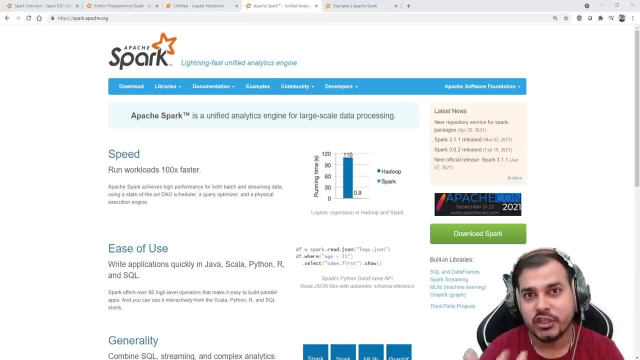 which will basically say that how you can apply machine learning, you know in Apache Spark itself, with the help of this Spark API called as PySpark libraries. and apart from that, we will also try to see in the future, once we understand the basics of the PySpark library, how we can actually 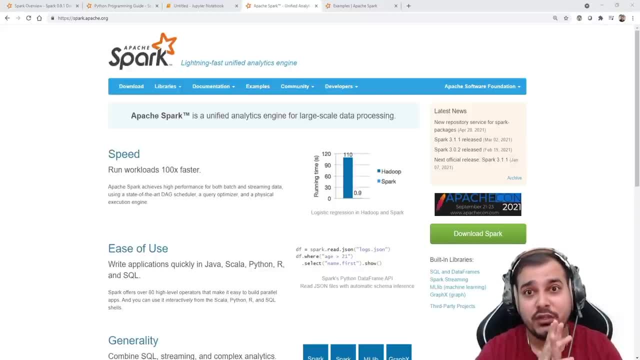 pre-process our data set, how we can use the PySpark dataset frames. we'll also try to see how we can implement or how we can use PySpark in cloud platforms like Databricks, Amazon, AWS, you know. so all these kind of clouds will try to cover. and remember Apache, spark is quite handy, let me tell you. 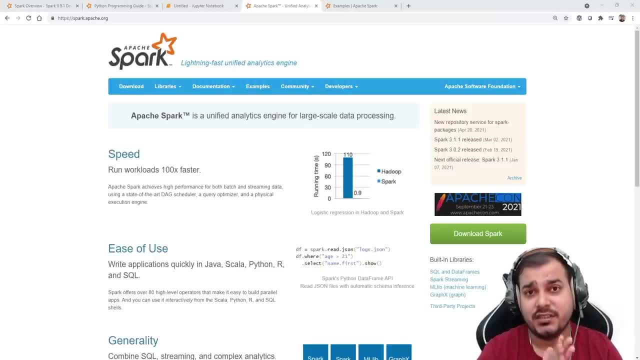 just let me just give you some of the reasons. so why Apache spark is pretty much good because understand, suppose, if you have a huge amount of data. okay, suppose if I say that I'm having 64 GB data, 128 GB data, you know, we may have. 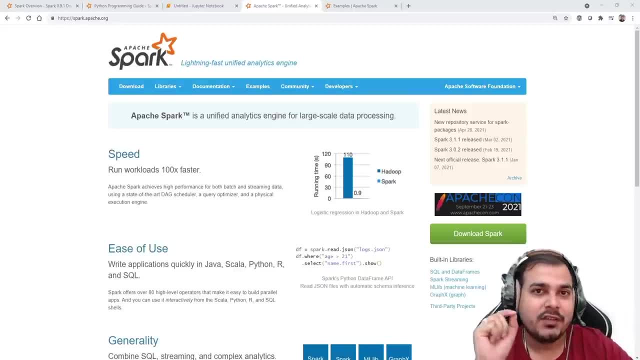 some kind of systems, of standalone systems. you know where we can have 32 GB of RAM, probably 64 GB of them right now in the workstation that I'm working in. it has 64 GB RAM, so max to max it can directly upload a data set of 32 GB 48. 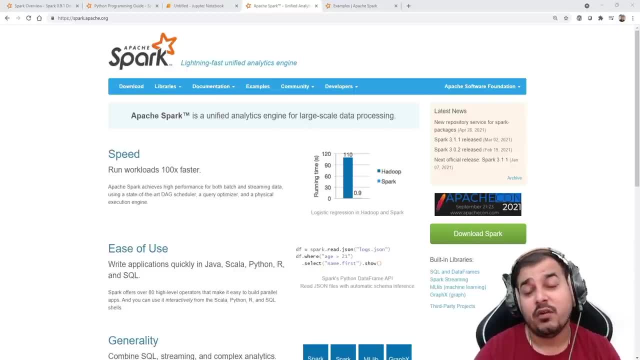 GB. right, but what if? if we have a data set of 128 GB? you know that is the time, guys. we don't just depend on a local system. we have to have a data set of 128 GB. you know that is the time, guys. we don't just depend on a local system. 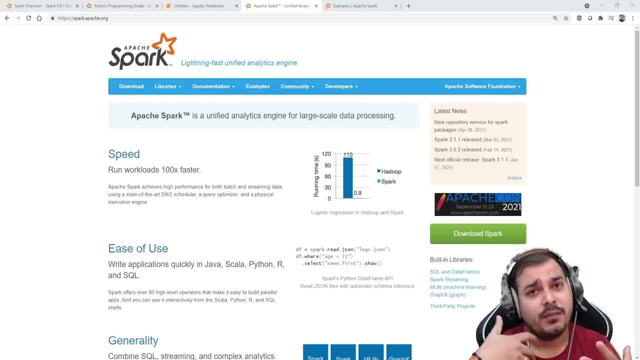 we'll try to pre-process that particular data or perform any kind of operation in distributed systems. right, distributed system basically means that all there will be multiple systems, you know, where we can actually run this kind of jobs or processes or try to do any kind of activities that we really 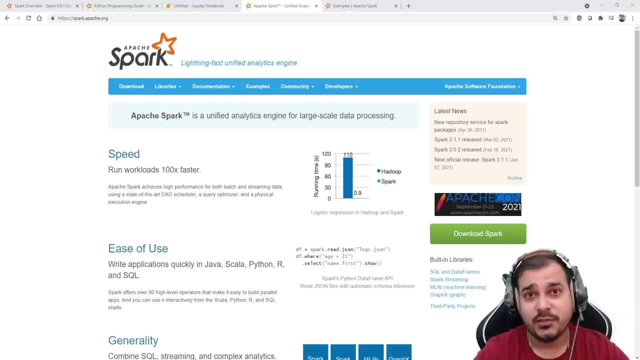 want, and definitely Apache spark will actually help us to do that, and this has been pretty much amazing and, yes, people wanted this kind of videos a lot. so how we are going to go through this specific playlist is that we'll try to first of all start with the installation. we'll 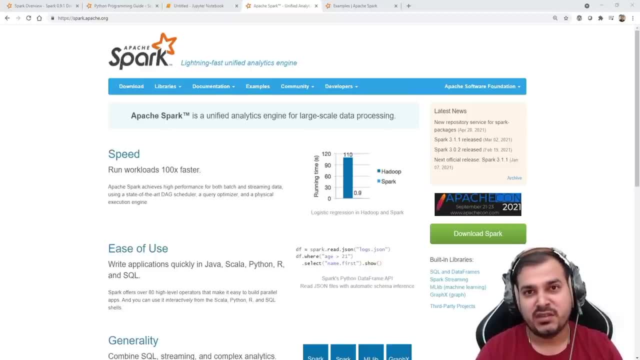 try to use PI spark, because that is also Apache spark is. it is a spark API with Python when you are actually working with Python. we basically use PI spark library and, yes, we can also use spark with other programming languages like Java, Scala, R and all right, and we'll try to understand from basics you know from. 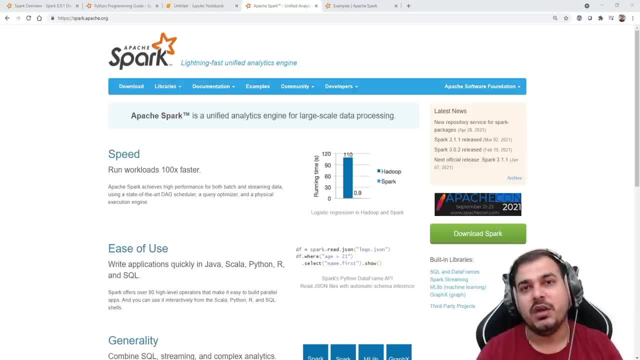 basics. how do we read a data set? how do we connect to a data source? probably, how do we play with the data frames. you know, in in this Apache spark, that is your PI spark also, they provide your data structures like data frames, which is pretty much similar to the pandas data frame but, yes, different kind of. 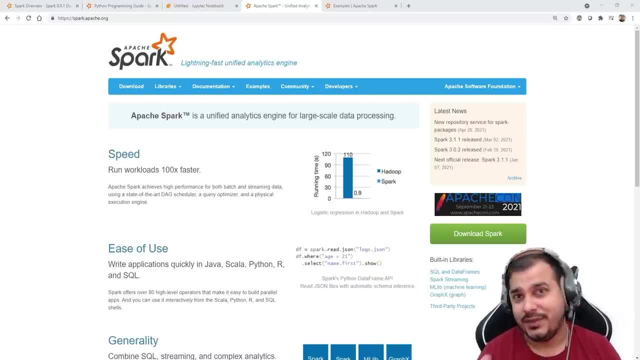 operations are supported over there which we'll be looking one by one as we go ahead, and then we'll try to enter into Mlib, the Apache spark Mlib- so basically it is called a spark Mlib- which will actually help us to perform machine learning, which will, where will be able to actually perform a lot of CHRISTOPHER. 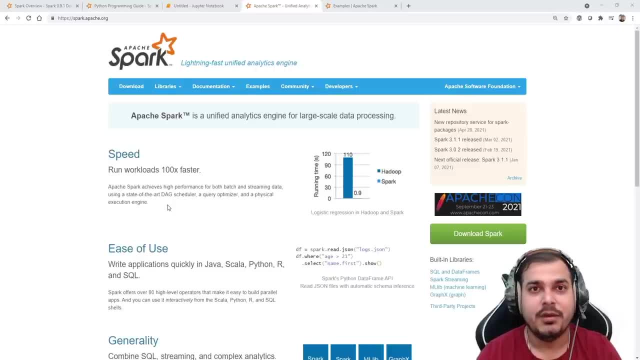 able to perform some machine learning algorithm task where we'll be able to do regression, classification, clustering, and finally, we'll try to see how we can actually do the same operation in cloud, where i'll try to show you some examples where we will be having a huge data set. we will 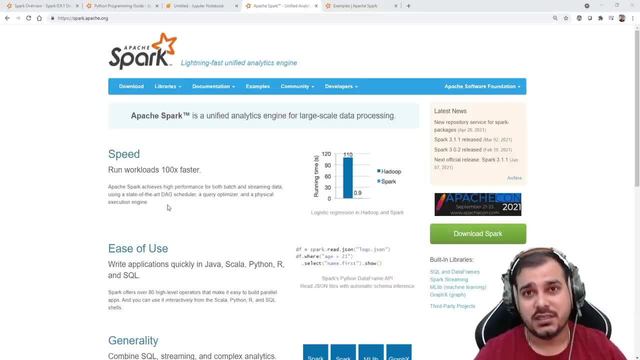 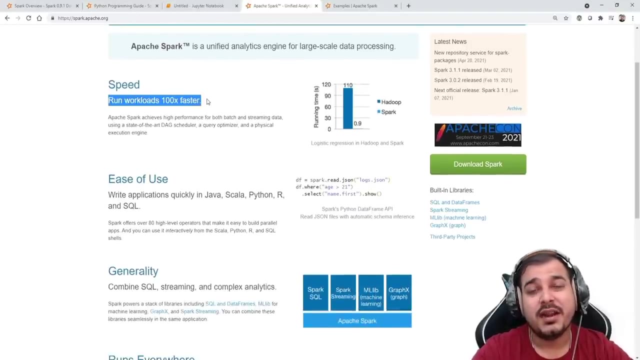 try to do the operation in the clusters of system, you know in a distributed system, and we'll try to see how we can use spark in that right. so all those things will basically get covered. now some of the advantages of apache spark and why it is very much famous because it runs workloads 100. 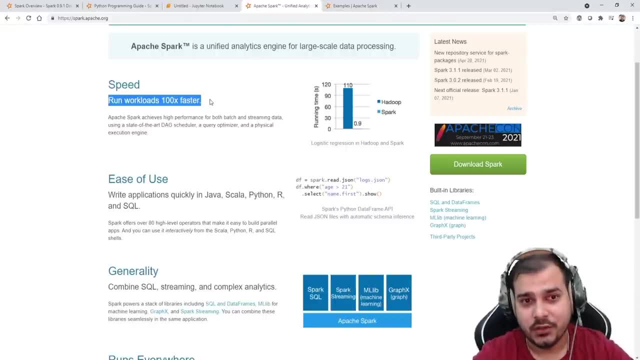 multiplied by 100 times faster. you know that basically means. and if you know about big data, guys, when we talk about big data, we're basically talking about huge data. set right and there. if you have heard of this terminology called as map, reduce right, trust me, apache spark is much more. 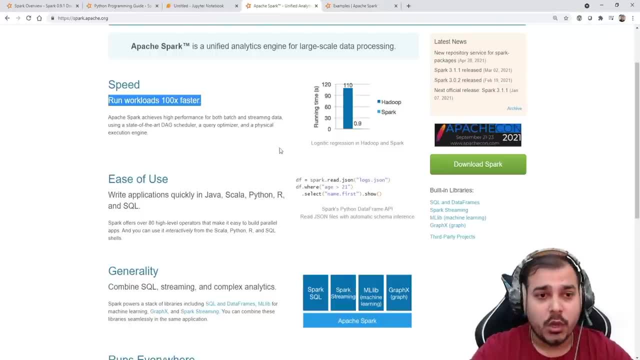 faster, 100 times faster than map reduce also okay, and it is, uh, some of the more advantageous and it has many advantages. so i'll just show you some of the advantages of apache spark and why it is very much famous because it runs workloads. 100 multiplied by 100 times faster you highest. 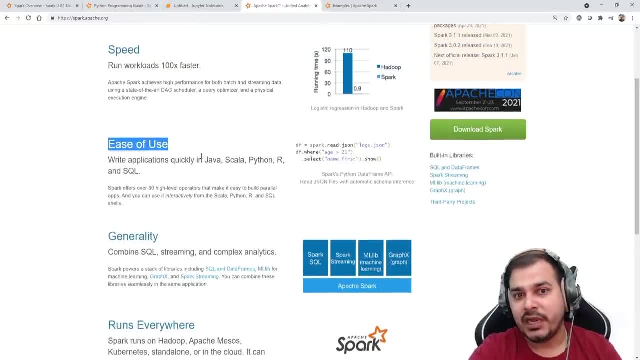 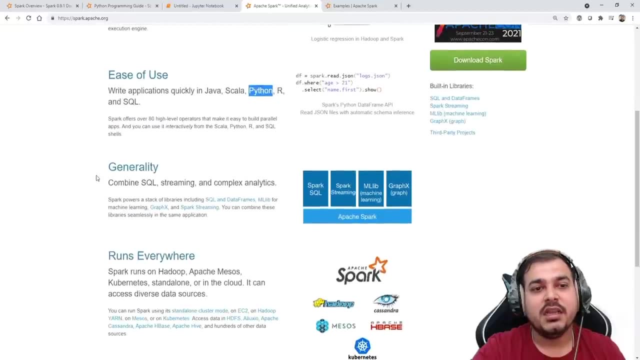 one thing is that it is ease of use. you can write application quickly in Java, Scala, Python or are, as I said, we'll be focusing on Python, where we'll be using a library called a spy spark. then you can also combine sequel streaming and complex analytics. when I talk about complex analytics, I'm basically talking 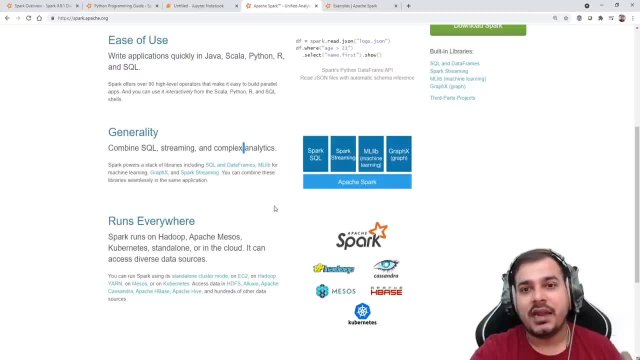 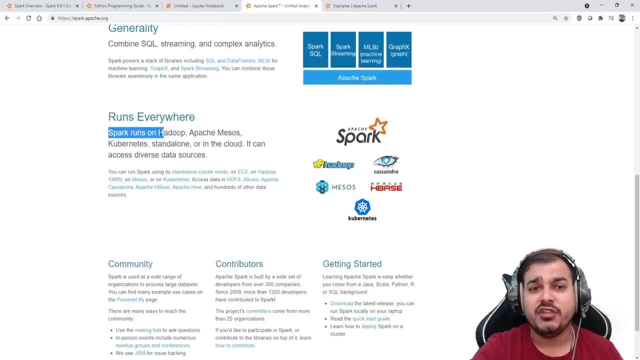 about this: MLib machine learning libraries. that will work definitely well with the Apache spark and Apache sparks can run on Hadoop, Apache resource kubernetes, standalone in or in the clouds cloud- different types of clouds. guys, when I talk about AWS, data breaks, all these things- we can definitely work. 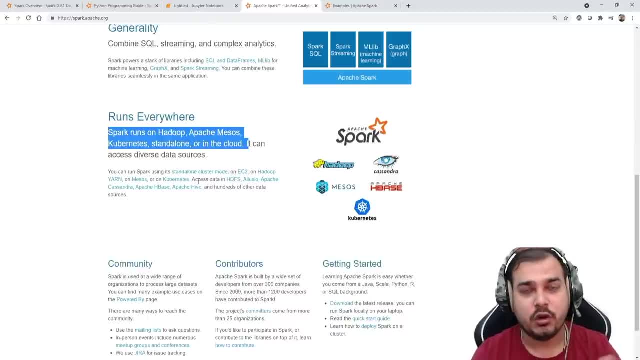 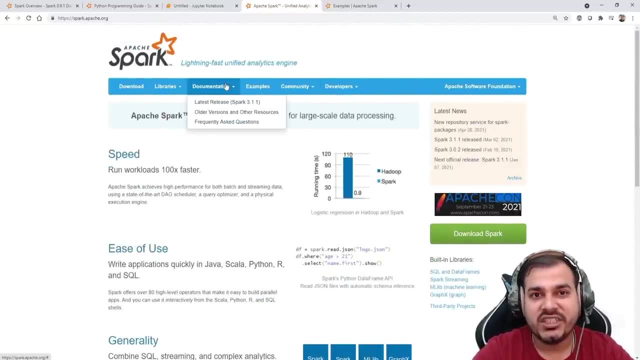 okay, and it actually runs in a cluster mode. cluster mode basically means in a distributed mode, right? so these are some of the examples. now, if I, if I go with respect to which version of PI spark will spark will be using plus proc 3.1 point one will be using will try to work. and if you just go and search for here, 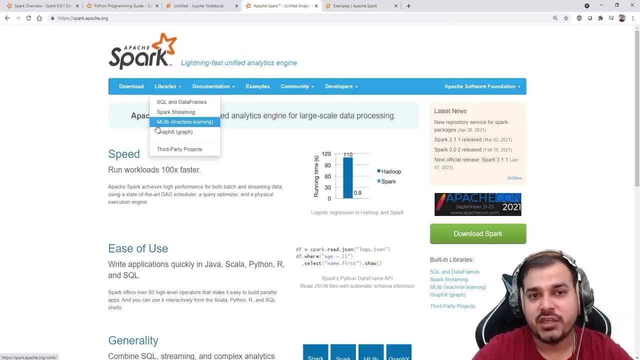 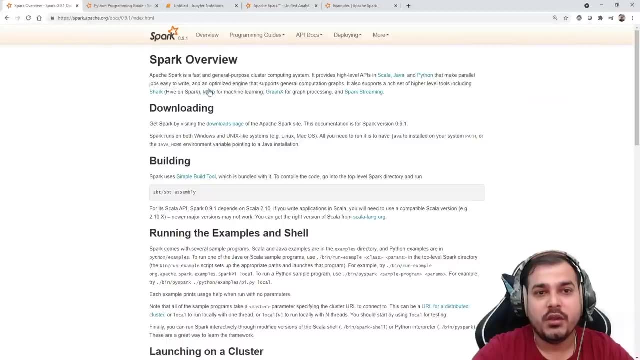 you can see sequel and data frames and all here. you can see spark streaming machine, MLib. that is called as machine learning and all right and apart from that, if I go and see the overview here, you can see that Apache spark is a fast and general-purpose cluster computing system. it provides high-level API's in 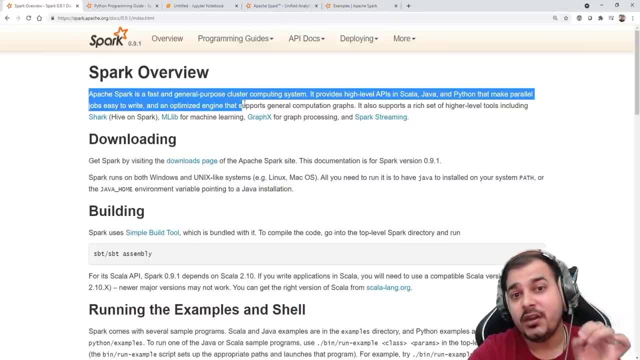 Scala, Java and Python. that makes parallel job easy. to write an optimized engine that supports general competition graph. so it is basically to work with huge amount of data. in short, you know, and that is pretty much handy. we'll try to work with that and that's it for today. thank you for watching and I'll see you in the next video. 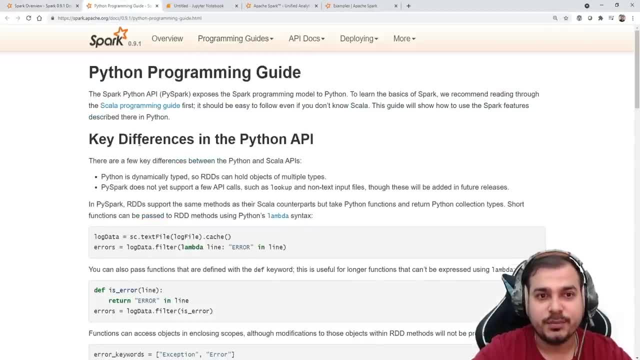 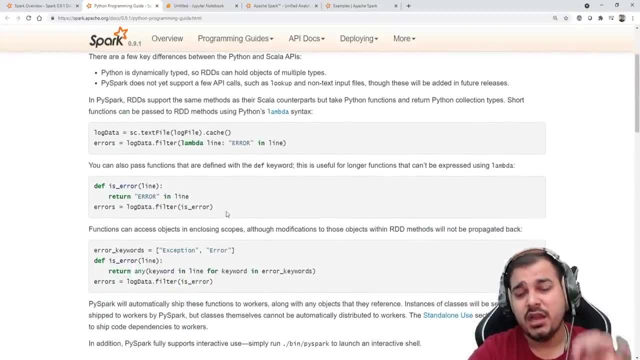 work. now, if I go and search for the spark in Python, you know this page will get basically go it open and this things will try to discuss how to install it and in this video we'll try to install the PI spark library. if I talk about PI, 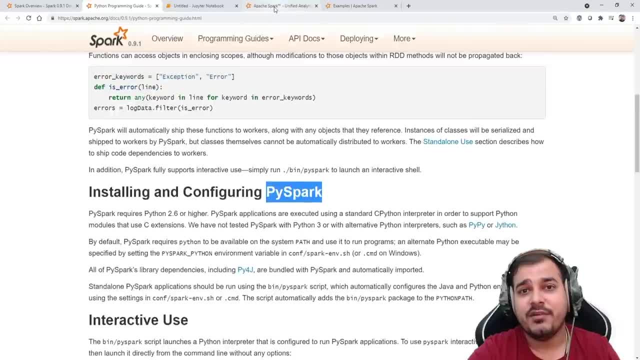 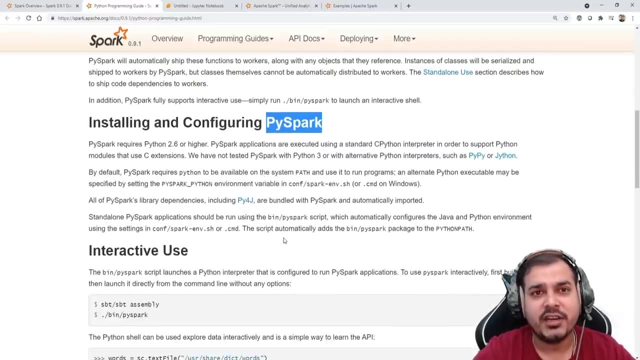 spark library, you'll be able to see that PI spark library is pretty much amazing. this library is, if you really want to work spa, if you want to work this part, functionality with Python. you basically use the specific library and let's proceed and let's try to see that how we can quickly- yeah, how we can. 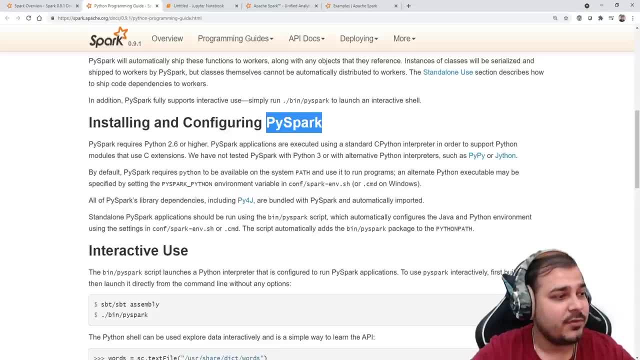 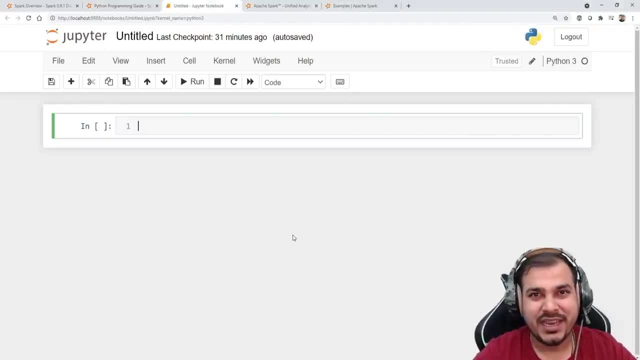 quickly, you know, install the specific libraries and check out like what all things we can actually do. okay, so all these things we'll try to see. so let's begin. please make sure that you create a new environment when you're working with PI spark. so I have created a new environment called as myenb here. first, 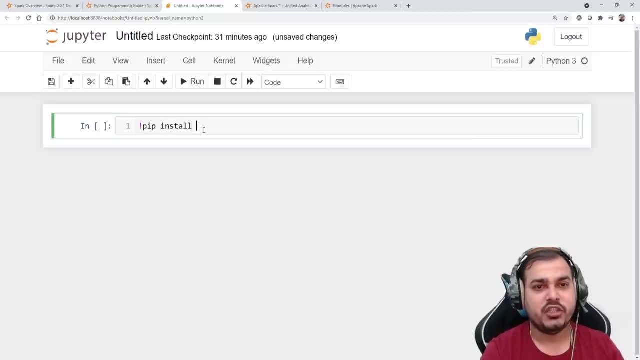 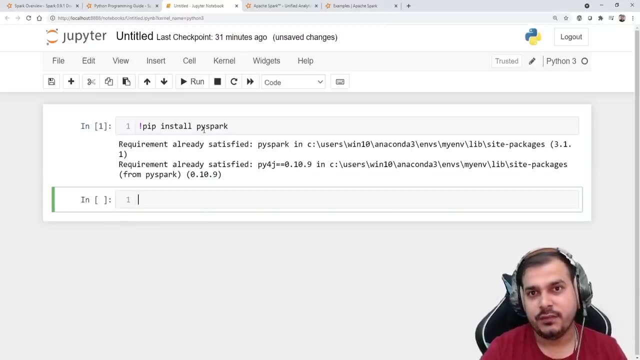 of all, I'll try to install the PI spark library, so I'll just write pip- install PI spark. okay, and let's see. in this we'll focus on installation, will focus on reading some data sets and try to see that what are things we can actually do. okay, and after doing this, 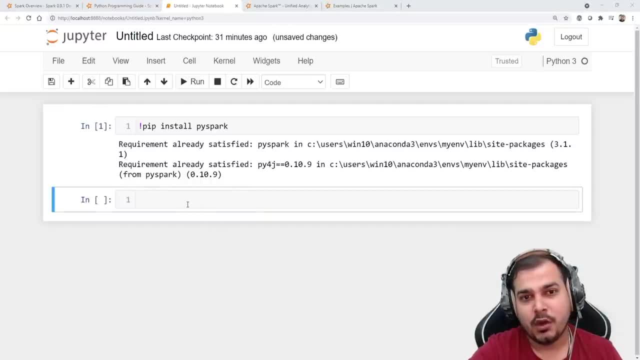 what we can actually do is that you can see that our PI spark has been installed. in order to check whether the installation is perfect or not, I'll just write: import by spark. so this, this looks perfectly fine, it is working. you know, we we are able to see that the PI spark is basically installed properly. now you may. 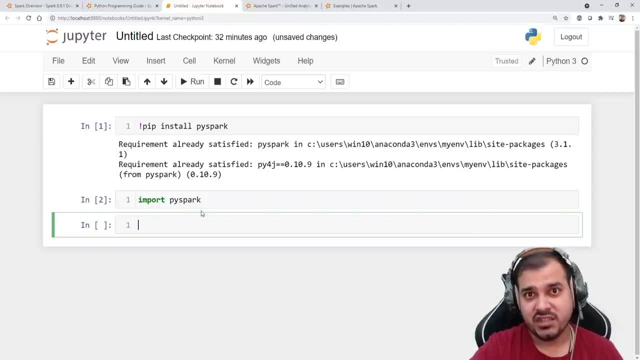 be facing some problems, guys. respect to py spark. so that is the reason why i'm telling you: create a new environment. if you're facing some kind of issue, just let me know what is the error that you're getting, probably writing in the comment section. okay, now let's do one thing. i'll just open a excel sheet. okay, and probably. 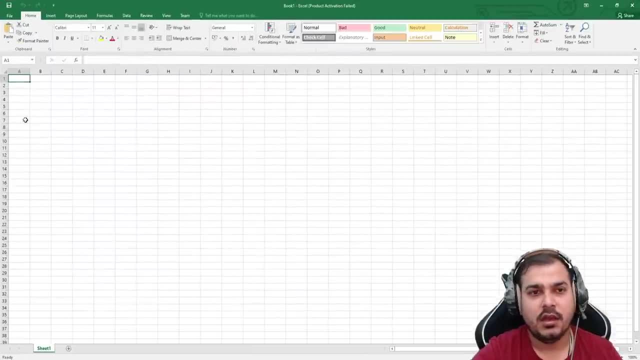 i'll just try to create, uh, some data sets. i'll say name, probably. i'll just say name and age, right, and suppose my name over here that i'm going to write is krish, and i'll say 31. i'm going to say sudan shu. 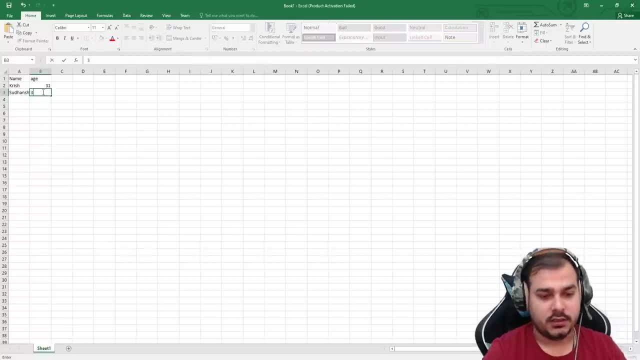 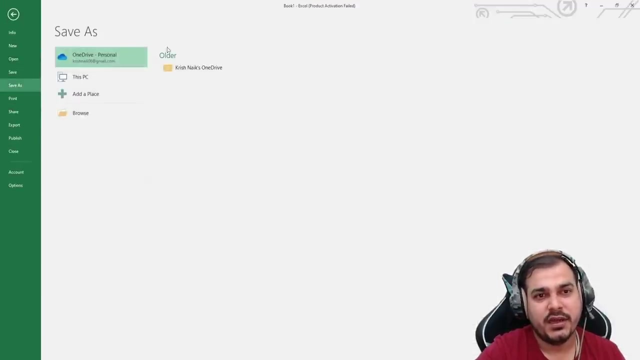 right, shudan shu. i will just say okay, 30, and probably i'll just write some more names, like sunny. probably i'll also give the data as 29. so this three data. we'll just try to see how we can read this specific file. okay, i'm just going to save it. uh, let's see, i'll save. 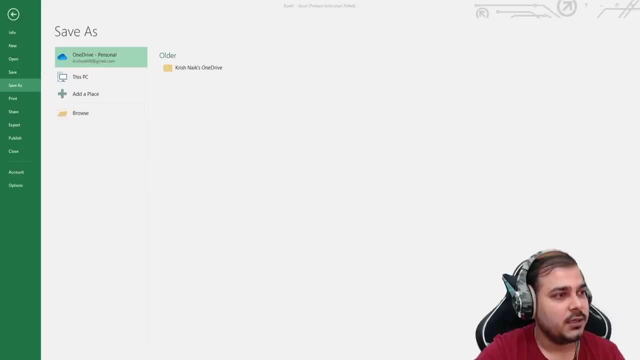 it in the same location where my jupiter notebook is. guys, uh, i created a folder. i guess you can save it in any location where your notebook file is open, right, so it is not necessary. i'm just, uh, uh, making sure that you don't see any of my files. 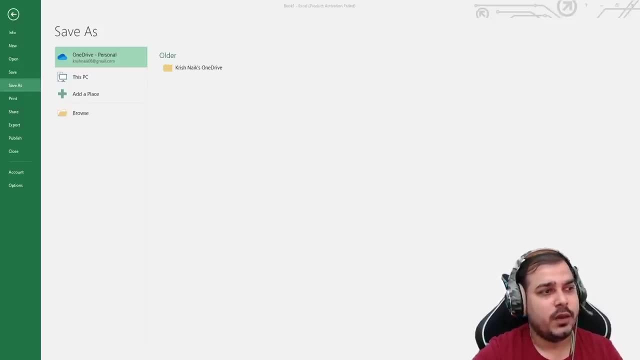 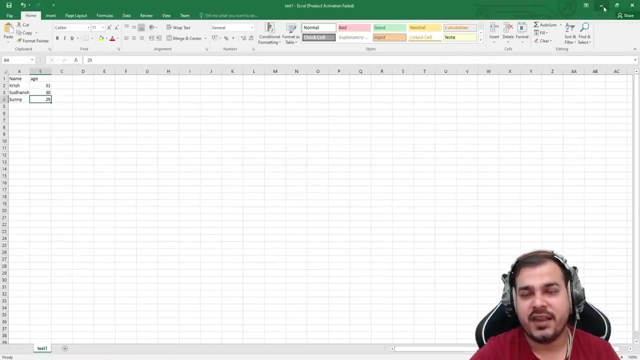 okay, and i'm just saving it. okay, i'm saving it as test one here. you can see, i'm saving it as test one, dot csv, so i'll save it. uh, let's keep this particular file saved, okay. now, If I probably want to, you know, read with the pandas. 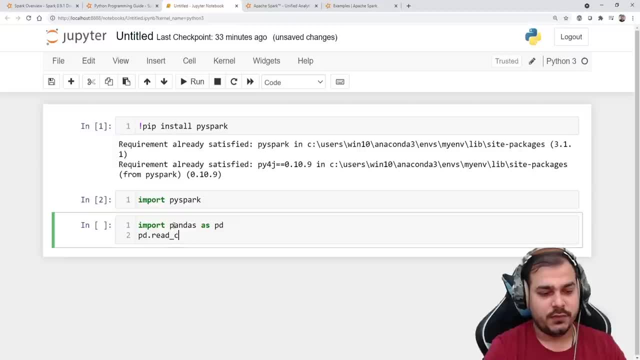 so what we write? we write pdread underscore csv right, And I basically use this particular data set. it's called as test1.csv right, So when I'm executing this here, you will be able to see the specific information. 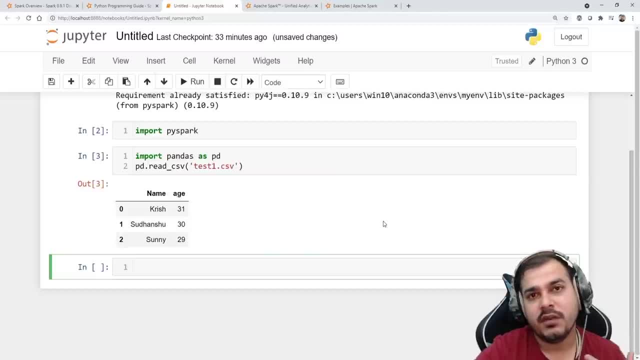 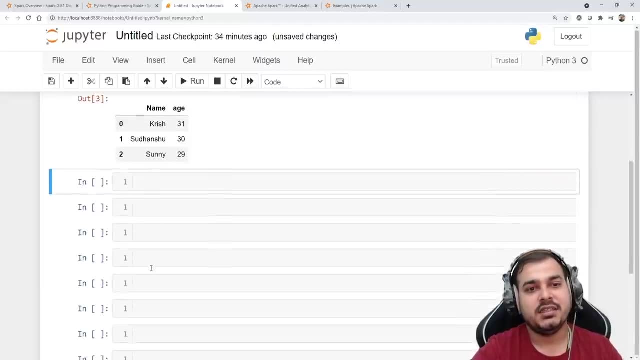 Now, when I really want to work with PySpark, always, first of all remember we need to start a Spark session. And in order to start a Spark session, first of all, let me create some more fields. Just see this. just follow these particular steps. 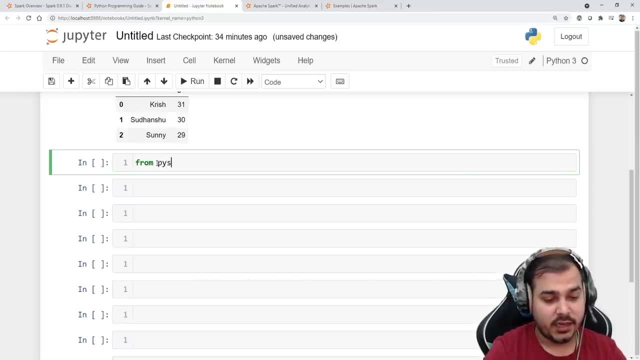 with respect to creating a path session. So I'll write from pysparksql import spark-session- okay, And then I'll execute this. You can see that it is executing, fine, Then I'll write. sorry, I don't know what has opened. 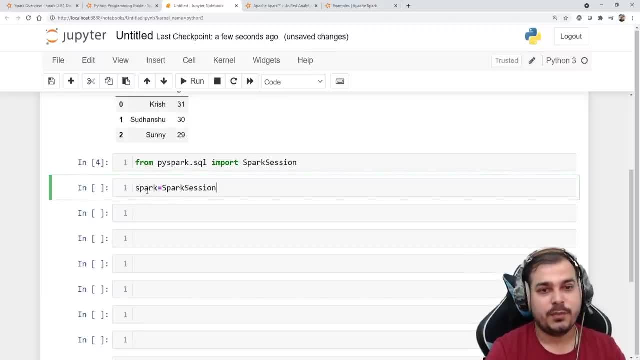 So I'll write, I'll create a variable called a spark, and probably I'll use the spark-sessionbuilder and I'll say app name and here I'll just give my session name. okay, So it'll be like practice. 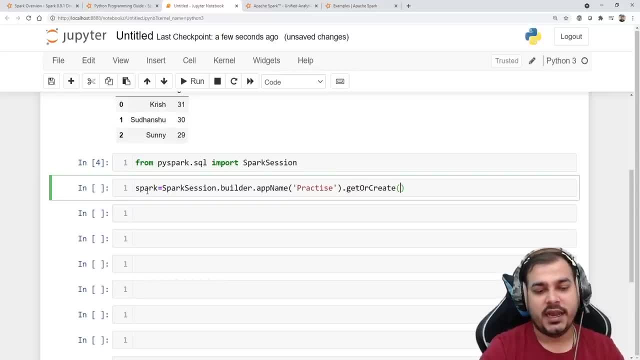 Suppose I'm practicing these things and then I can say get or create. So when I actually execute this you'll be able to see. a Spark session will get created And if you're executing for the first time, it'll probably take some amount of time. 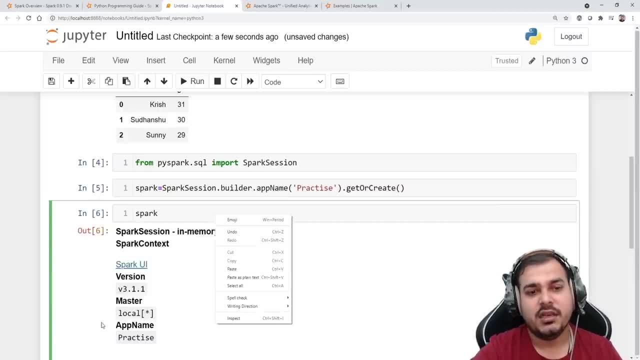 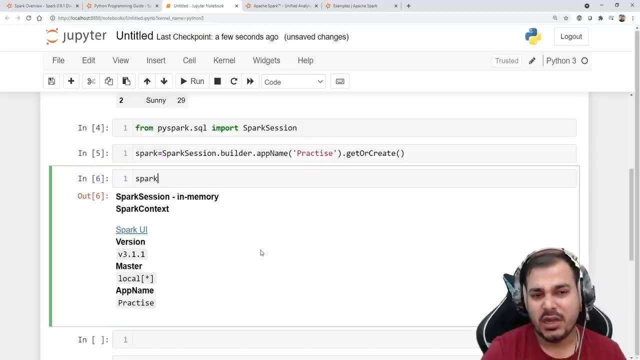 Other than that, if I've executed multiple times, then you'll be able to work it Now here. you can definitely see that in this, when you're executing in a local, there'll obviously be only one cluster. So you can see that in this, when you're executing in a local, there'll obviously be only one cluster. So you can see that in this, when you're executing in a local, there'll obviously be only one cluster. So you can see that in this, when you're executing in a local, there'll obviously be only one cluster, But when you are actually working in a cloud, 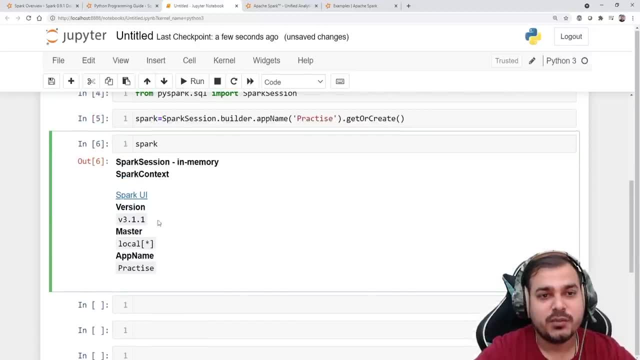 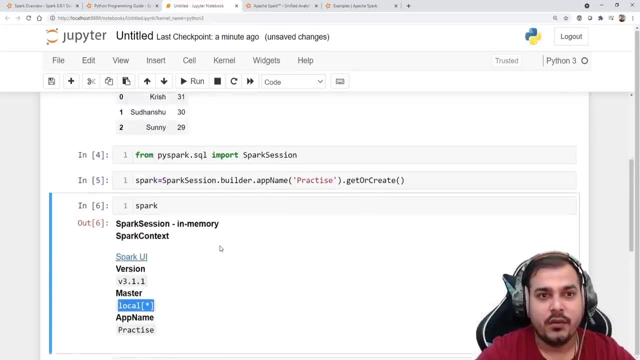 you can create multiple clusters and instances. okay, So the Spark version that you'll be using is v3.1.1.. Here you can see that this is basically present in the master. When probably you'll be working in multiple instances there, you'll be seeing masters and cluster one, cluster two. 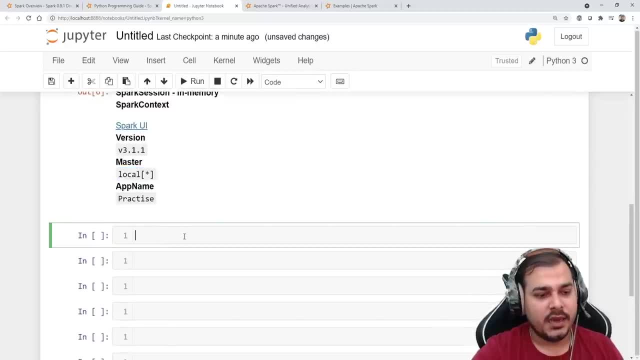 all those kind of information. okay, So this is with respect to Spark. Now let's, I'll just write df of PySpark, where I will try to read a dataset with respect to Spark, where I will try to read a dataset with respect to Spark. 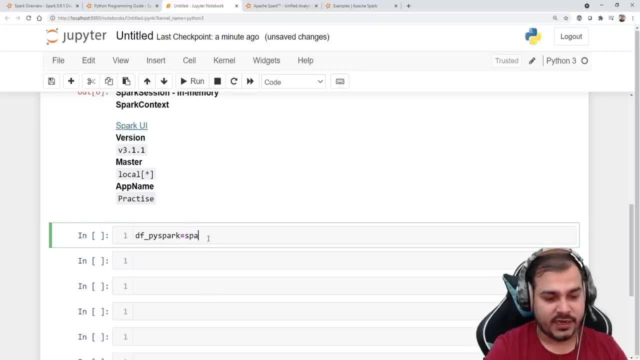 where I will try to read a dataset with respect to Spark. Now, in order to read a dataset, what I can write? I can write like this sparkread. I can write like this sparkread. There is a lot of options like CSV format, JDBC. 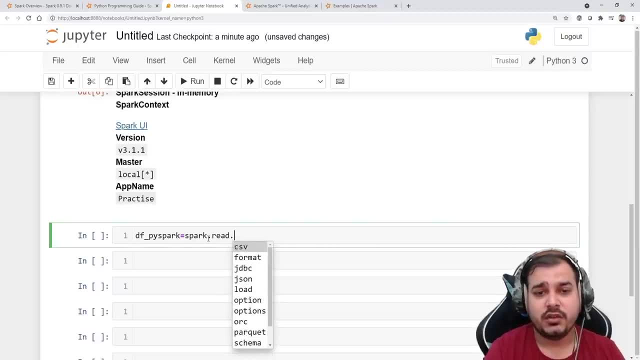 ParQ schema table text. a lot of options there. So here we are going to take CSV, and here I'm just going to write tips1.csv, right, and here I'm just going to write tips1.csv right. 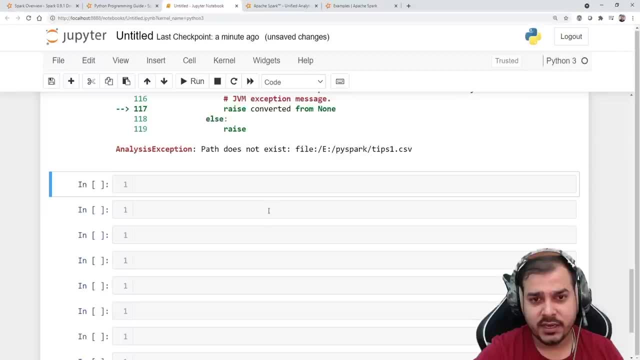 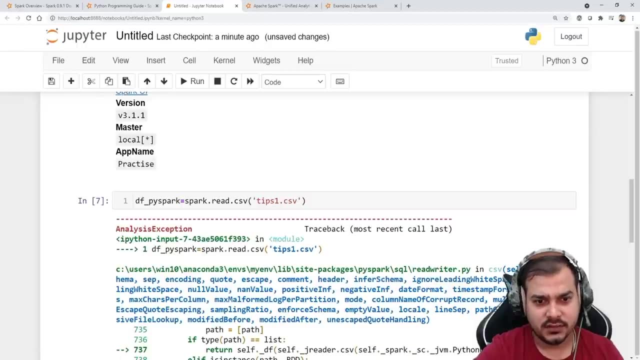 And if I just try to execute it here, I'm getting some error saying that this particular file does not exist. Let me see, I think this file is present. Just let me see, guys, Why this is not getting executed. Tips1,. 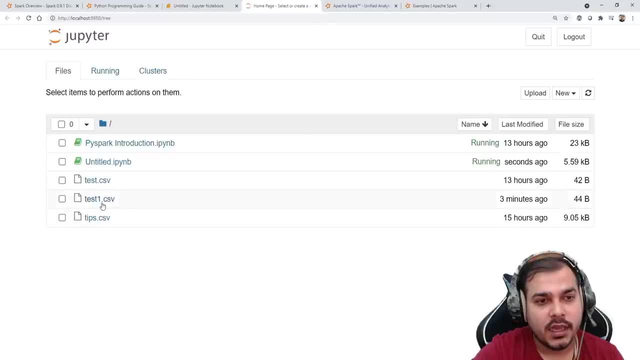 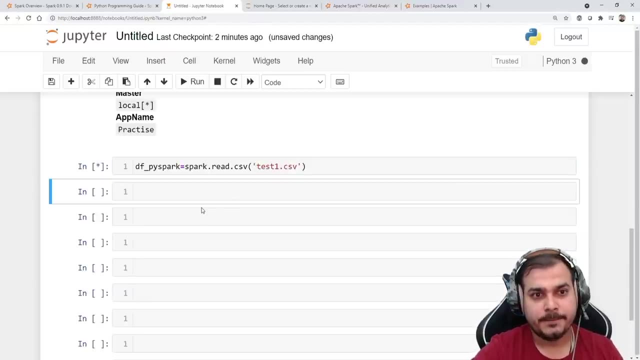 df file open. Here I can see test1.csv. Okay, sorry, I did not write the CSV file, I guess. Tips1.csv- Tips1.csv. Okay, this has now worked. Now, if I go and see dyspicepark. 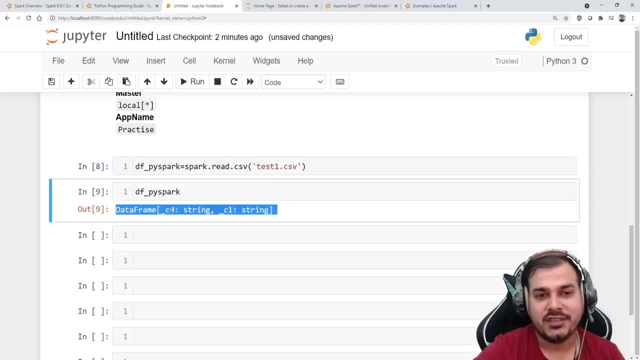 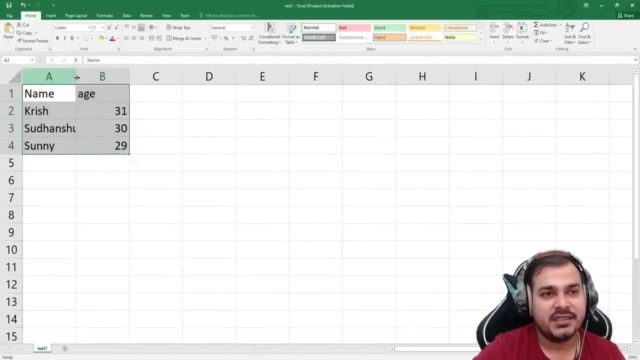 it is showing these two strings right, These two columns C0 and C1.. Now here you can see that, guys, I've created this particular CSV file, right, And it is just taking this AB as a default column probably. 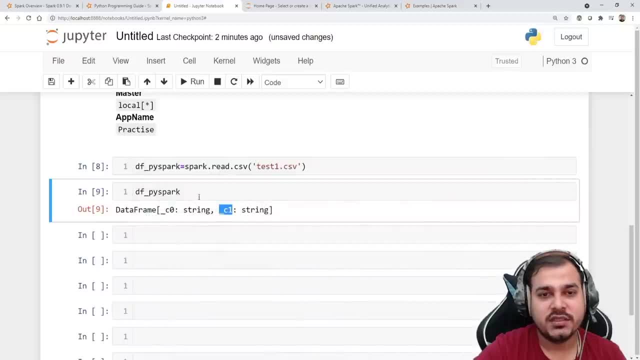 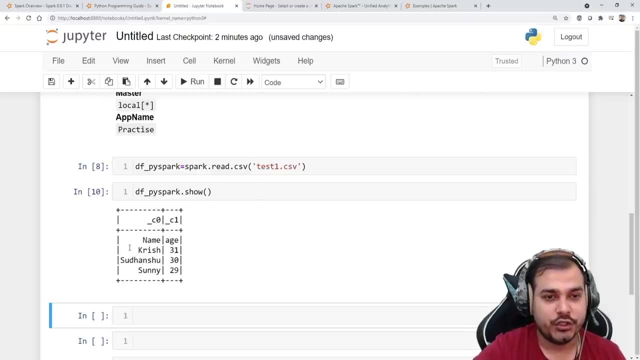 So it is saying C0 and C1.. So what we can actually do is that and probably, if you really want to see your entire dataset, you can basically see like this df underscore: pyspark dot- show. Here you'll be able to see name and age. 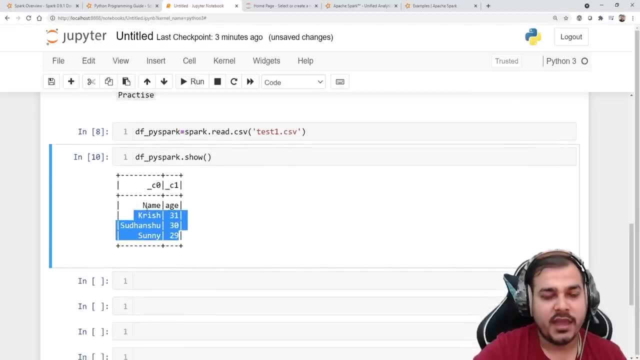 Chris, there's this information in there. I really want to make my column name or age as my main column right, But when I'm directly reading the CSV file, probably we are getting underscore C0, underscore C1.. So, in order to solve this, 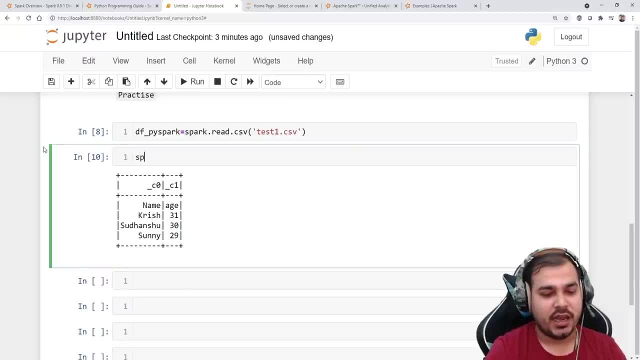 what I will do is that we have a different technique, So I'll write spark dot, read dot option. There is something called as option And inside this option, what you can basically give is that there'll be an option with respect to header, I guess. 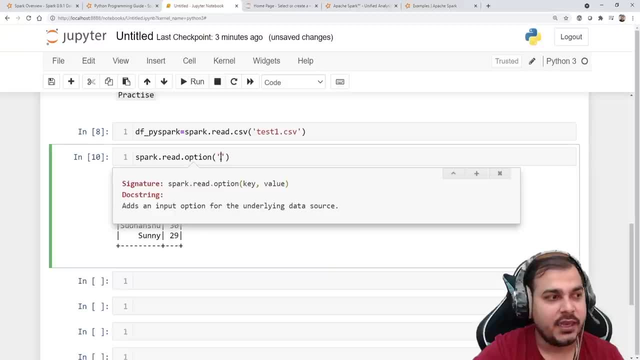 See, there'll be something like key value that you'll be providing in option. So what you can do, you can just write header comma: true. So whatever value, the first column, first row value will be there. that will be considered as your header. 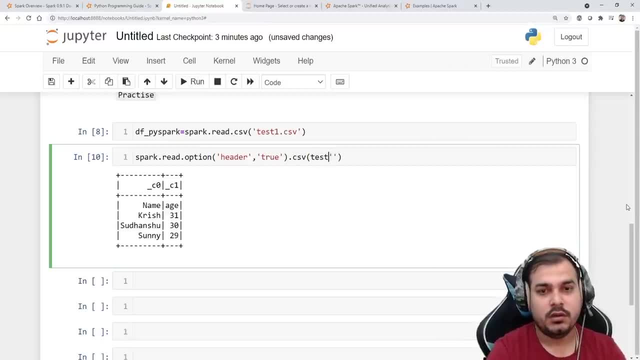 And if I write CSV with respect to test one now I'm just going to read this test: one dataset, Test one dot CSV. Now, once I execute this here, you'll be able to see that I'm able to get now name string, age string. okay. 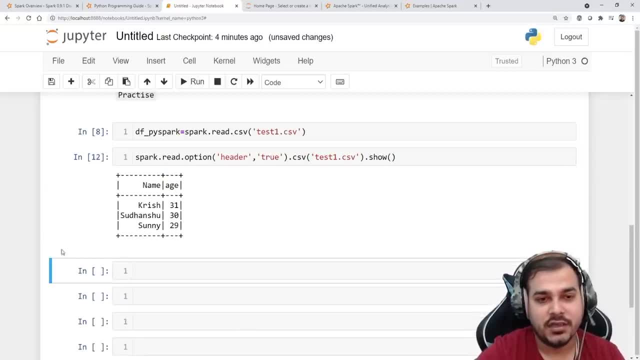 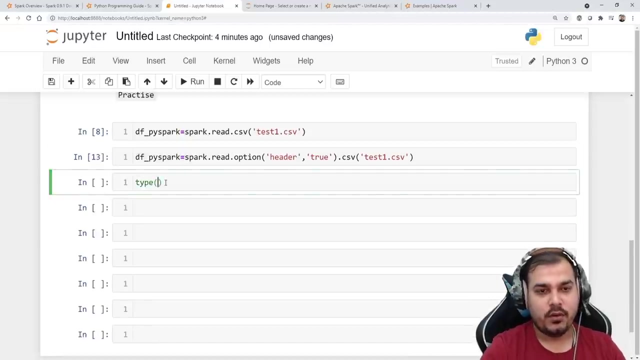 But let's see our complete dataset. So here, if I execute this now, I'll be able to see the entire dataset with this particular columns. okay, So let me just quickly save this in my df underscore, PySpark. okay, And now let's go and see the type of df underscore, PySpark. 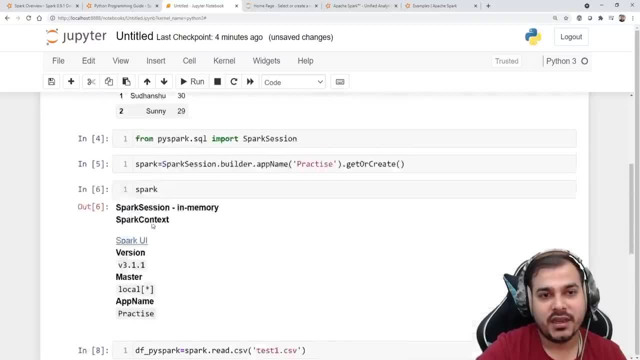 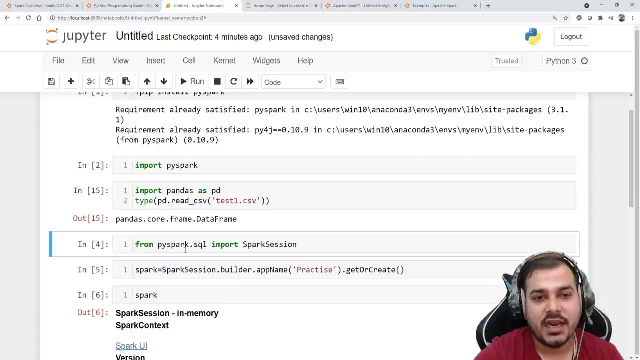 Okay, So once I execute this here, you'll be able to see, guys, when I was reading this df, right When I was. if I go and see the type of this with the help of pandas here, you'll be able to see that this is. 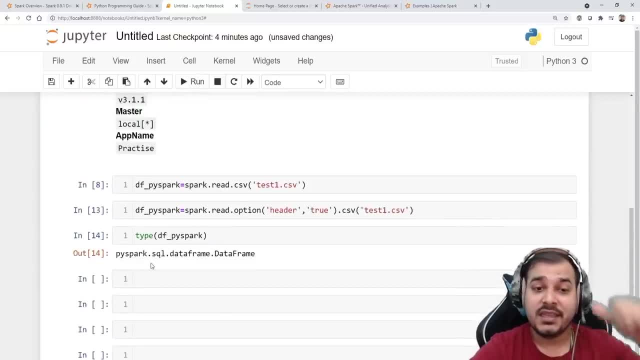 pandas dot code, dot frame, dot data frame. But here you'll be seeing that when you're reading this particular dataset, it is of type PySpark dot. SQL dot data frame, dot data frame. Yes, So that is pandas data frame. this is SQL dot data frame, dot data frame. 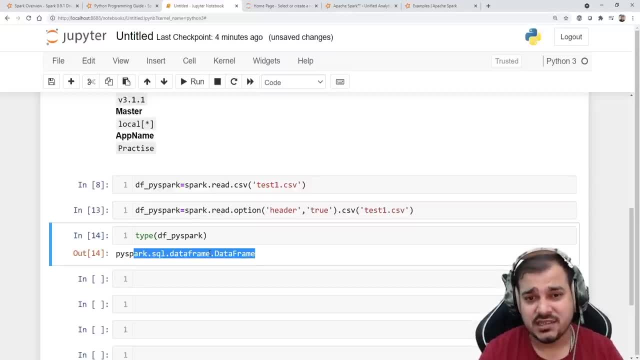 Yes, most of the APIs are almost same. The functionalities are same. There are a lot of things that we will be learning as we go ahead. If I quickly want to see my, probably I don't know whether head will work. Let's see. 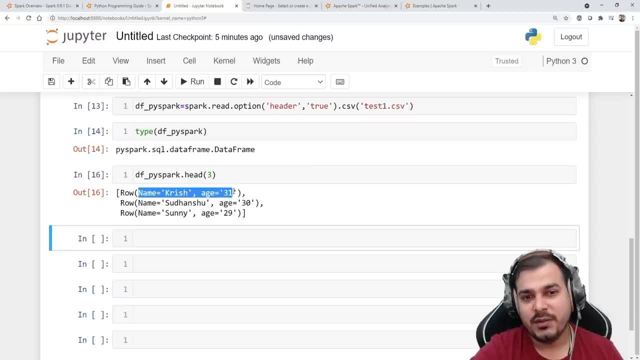 Yes, head is also working. So if I use dot head, probably you'll be able to see the rows. information are basically shown over here. Now, if I really want to see the more information regarding my columns, I will be able to use something called a sprint schema. 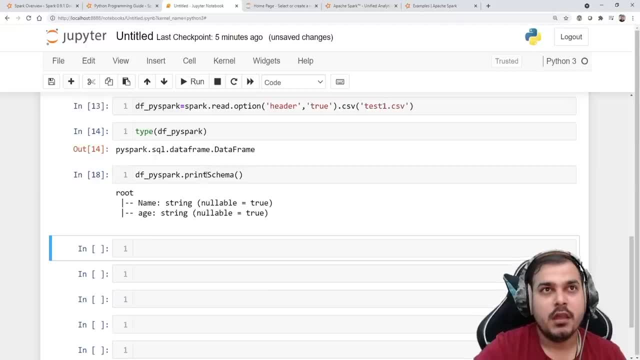 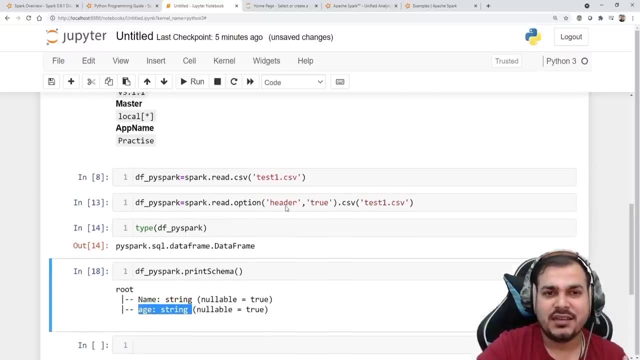 Okay, Now in this, this print schema is just like a, a DL PDF dot info which will actually tell about your columns, like name string and age string. All these are some basic operations that you have actually done after installation. Again, the main thing why I'm focusing on this is that 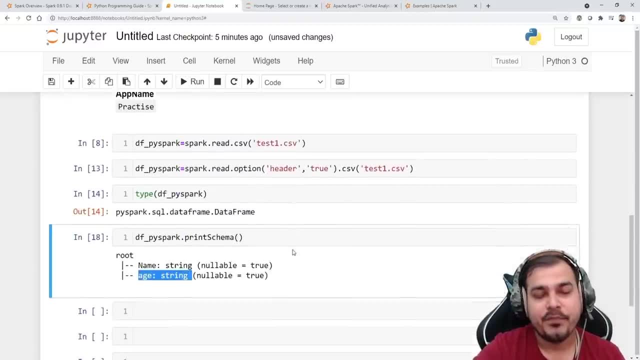 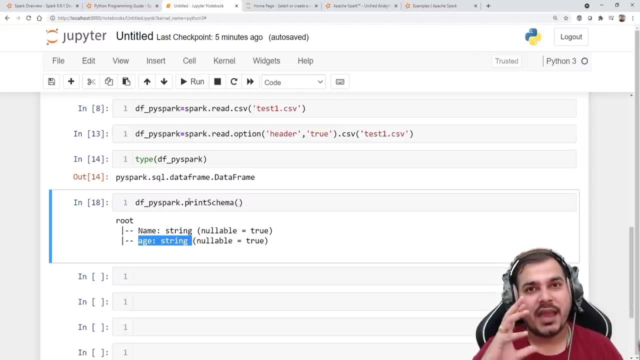 just try to install this PySpark and keep it ready. For my next session. I will be trying to show you how we can change the data type, how we can work with data frames, how we can actually do data preprocessing, how we can handle null values, missing values. 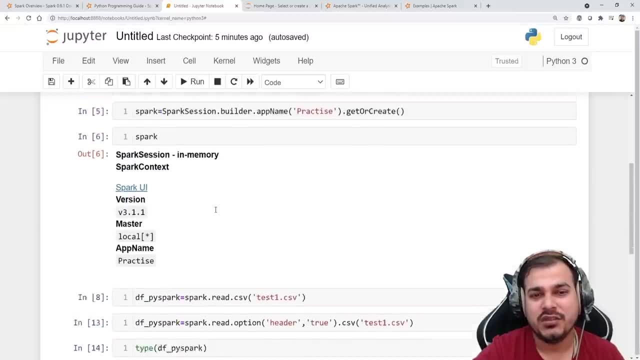 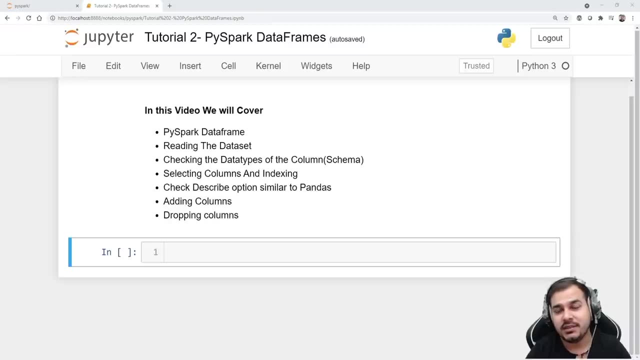 how we can delete the columns, how we can do various things. so all those things will basically we'll be discussing over there how to drop columns and all so, guys, we will be continuing the pi spark series and in this tutorial we are actually going to see what are pi spark data frames? uh, we'll try to read the data set, check the data types. 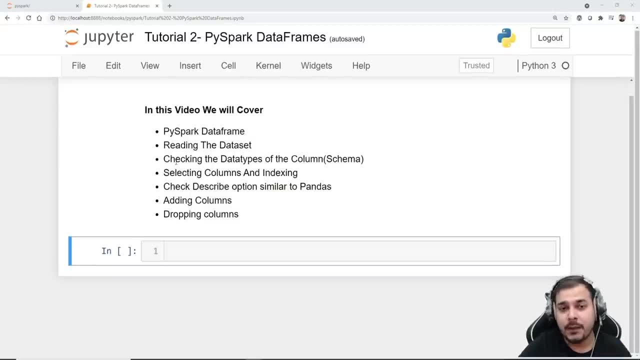 of the columns we basically see in pi spark called a schema. then we'll see that how we can select the columns and do indexing. uh. we'll see uh describe functionality that we have similar to pandas and then we'll try to see that how we can add new columns and probably drop columns. now this 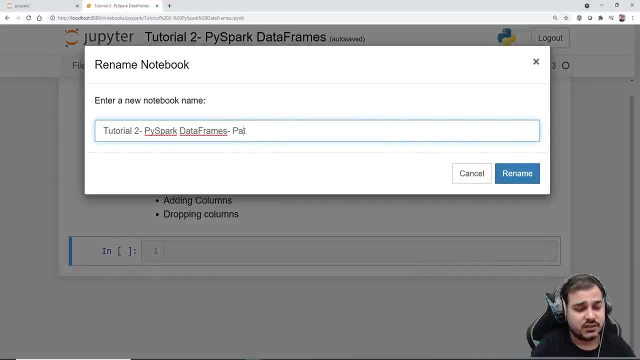 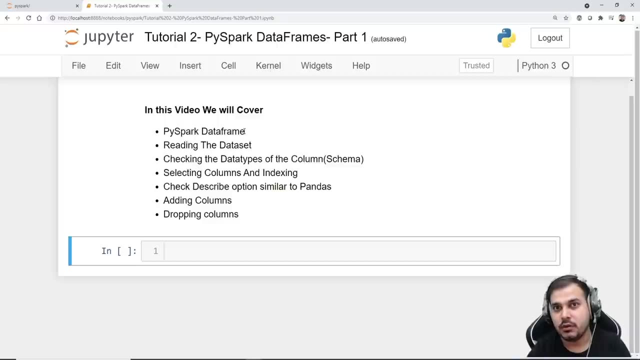 is just the part one, so let me just write it down as part one, because after this there will also be one more part. why this video will be important: because in pi spark also, if you're planning to apply emblem, you know the machine learning libraries you really need to do data pre-processing. 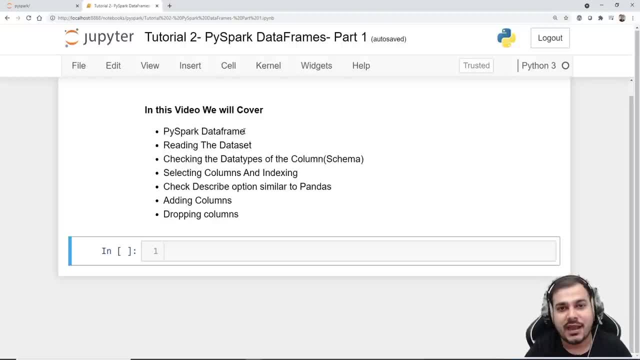 initially, you know, probably in the part two, we'll try to see how to handle missing values, and all uh. we'll try to see how to alter the rows, how we can probably put a filter condition, and all right. so let's proceed. before going ahead, what i'm going to do is that we will first of all, uh, you, i have a data set. 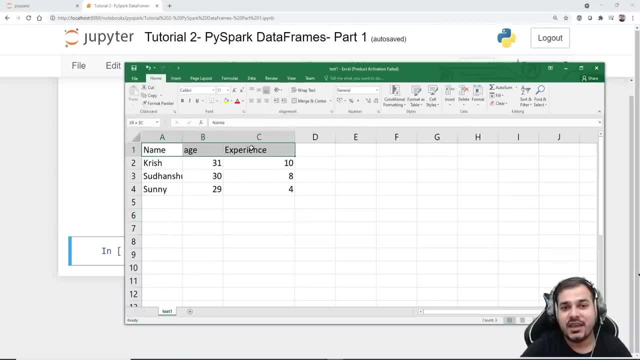 called as test one. so i have taken three columns: one is name, age and experience, and then i have a data set like krish 3110, like this: sudanshu sunny right. so this is some data set which i have saved in the same location. now, what i'm going to do first of all, as usual, uh, the first step with 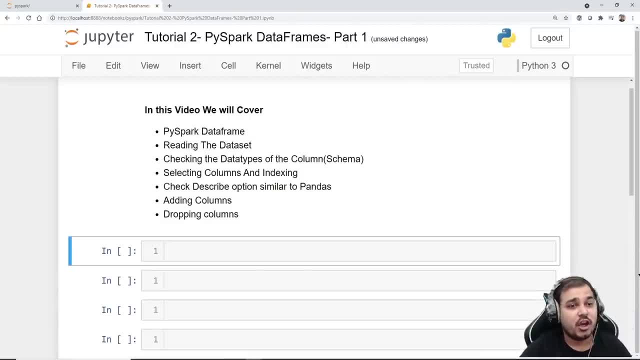 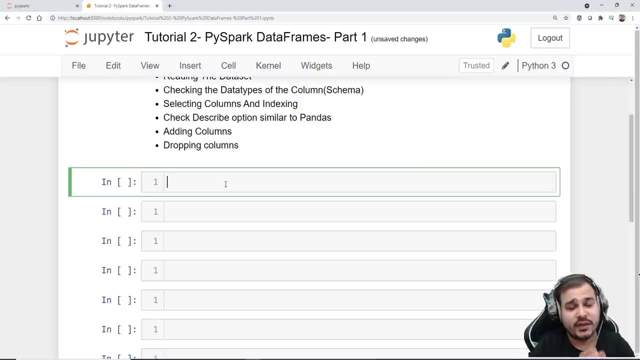 respect to pi spark is to build the pi spark session now. in order to build the pi spark session, i will uh write the code line by line to the pi spark session, and then i'm going to go ahead, and so please make sure that you also do along with me. it will definitely be helpful. so i'm going to 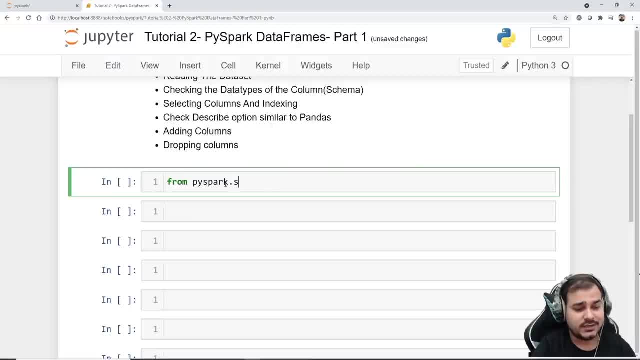 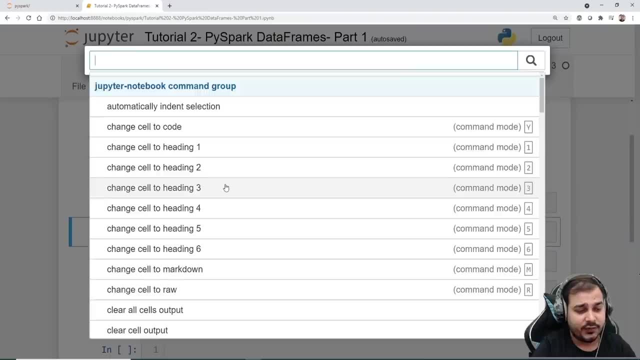 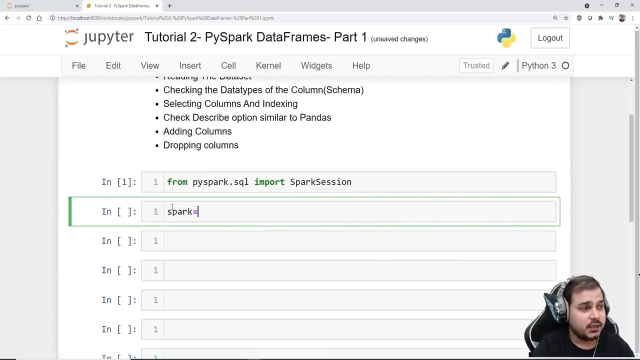 write from pi spark dot sql: uh. import spark session and then i'll create a variable. oops, sorry, then i'll start to create a variable regarding my session. so i'll write: spark is equal to spark session dot. we basically write builder dot app name, and here i'm just going to. 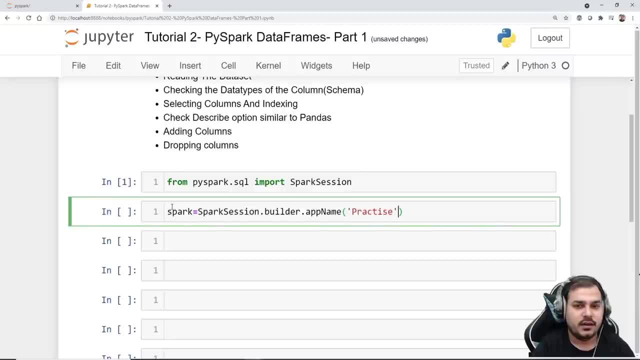 give my app name as practice, i can just say, or let me write, data frame practice or data frame right, something like this: since we are practicing data frame dot, uh, get or create function, and this is how you actually start a session. so, once and again, if you're executing for the first time, it 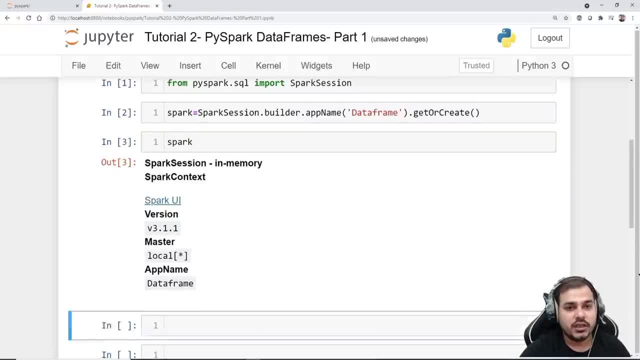 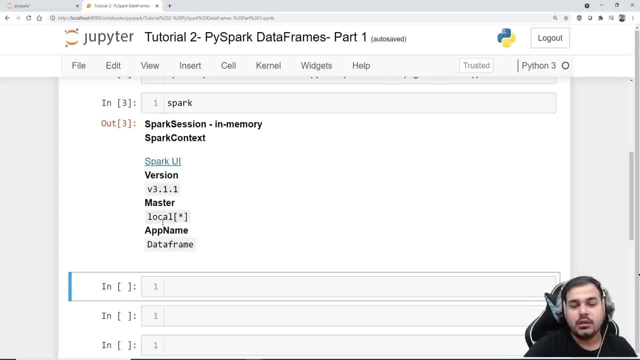 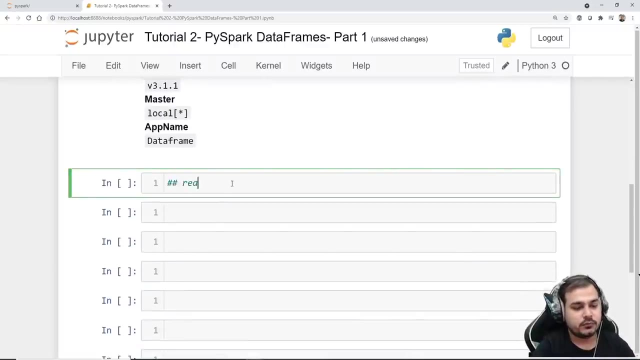 will take some time, otherwise it'll. it is perfect to go. so here is my entire spark. it is running in memory, uh, the version that it is running over here, and obviously, when you're running in the local you can see that the app name is data frame. so to begin with, uh, we'll try to read the data set again. 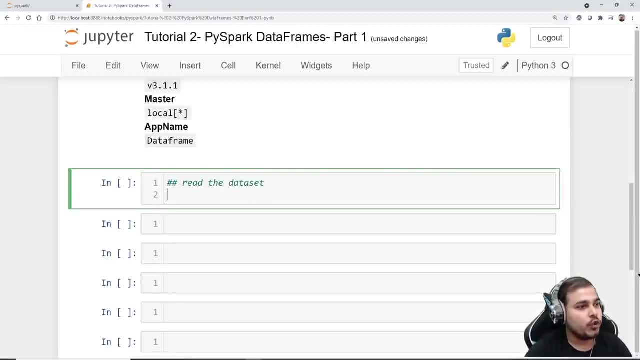 so let's read the data set now. reading the data set, i have already shown you multiple ways, um, one is through read option, one is to uh, and since this is a csv file, we'll try to read it first. first option: we'll try to see how we can actually rate it and then i'll show you multiple. 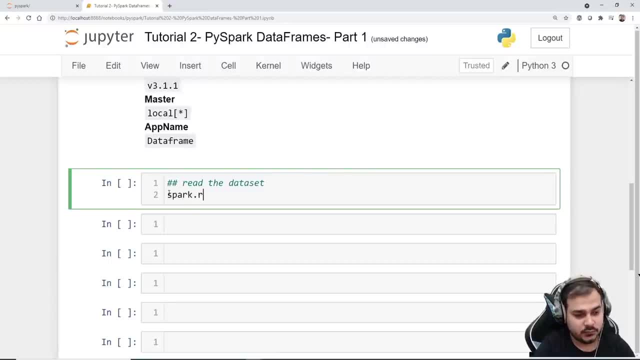 ways of reading it. okay, so i'll write spark dot. read dot options. we basically say key value, right? so here i'll just make it as header is equal to true, so that you know it should be considering my first row as the header, and here i'll write it as header as true. 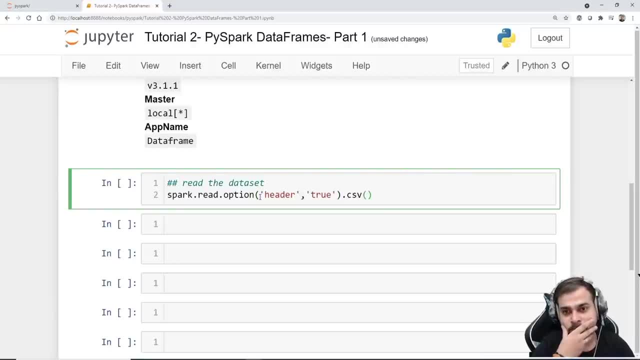 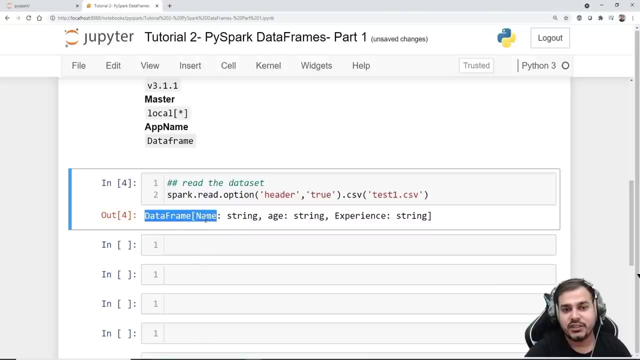 dot csv. inside the csv, i'll give my data set name that is called as test1 dot csv. right now, when i execute this, uh, probably, i think you'll be able to see the data set. so here you are able to see that if you have features like name, age, experience, right. so if i want to see the complete data set, 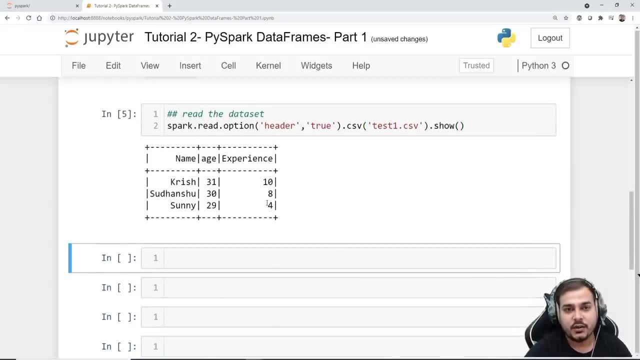 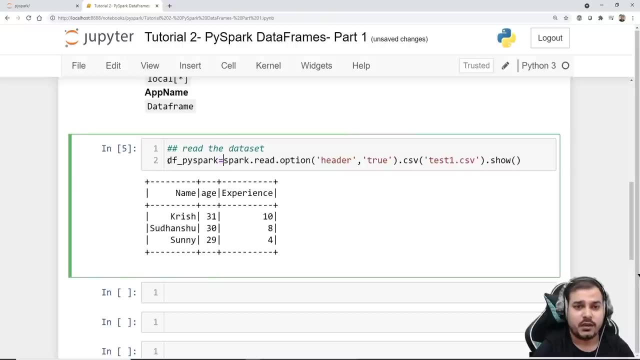 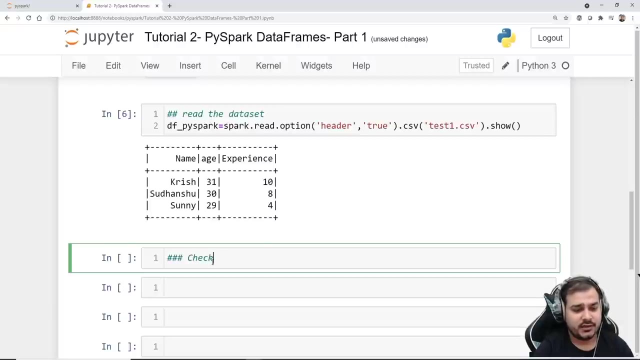 i'll just write dot show. so here is my entire data set over here. very clearly, i can see it now. uh, let me just save this in a variable called as df underscore, pi, spark. okay, so here is my entire data sets now. uh, first thing, uh, how do we check the schema? let's check the schema, okay. 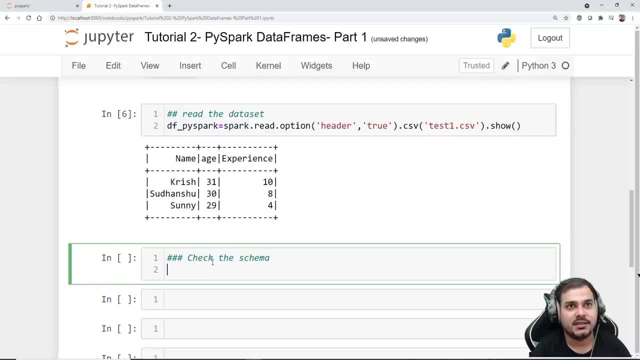 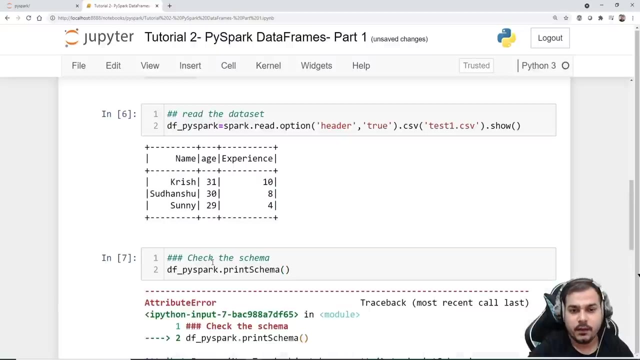 schema basically means the data types, like how we write in pandas, df, dot info. similarly we can write over here. so here you'll be able to see that i have written df underscore pi, spark dot print. i think it should work. print schema: oh, none type has spring schema. oh, sorry, so i had written dot showed and saved in a variable. 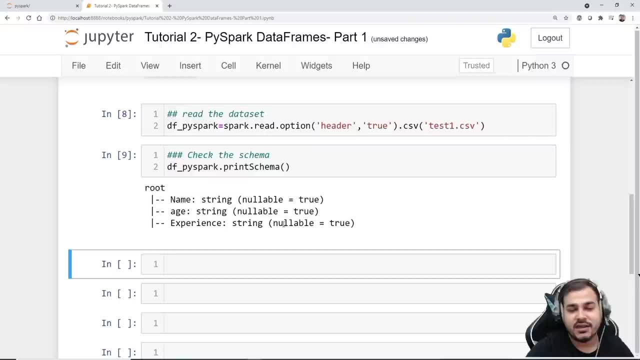 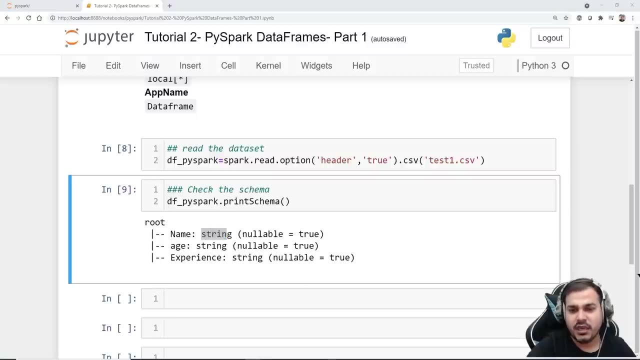 i'll remove this dot show. let me execute it once again. and now, if i write print schema here, you'll be able to see name, age and experience. but by default it is taking a string. even though in my first skew program i'm not going to do this yet as the aja planner, that should be what we have. 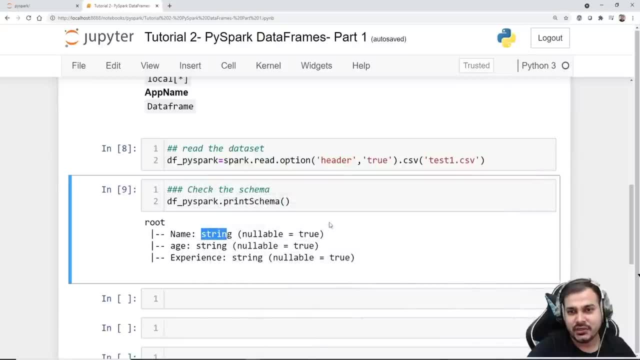 done is that we have written values. probably this should be string, this should be integers and this should be integers. but white is taking it as string. the reason it is probably taking at string, guys, because by default, unless and until we don't give one more option in csv. 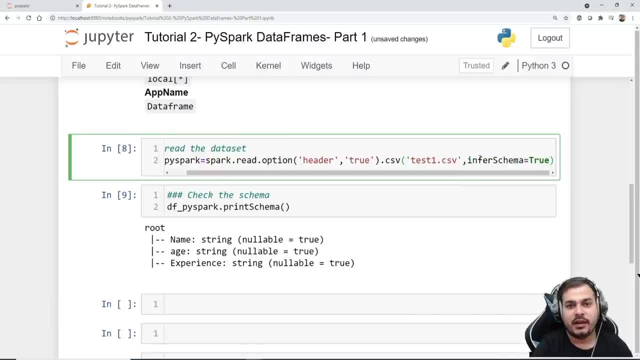 in this csv have one option called as infer schema. okay, if i don't make this as true right, it will by default consider all the features as, uh, you know, in the stream value. and now if i go and see df, underscore, pi, spark, dot print schema, you'll be able to see that i'm 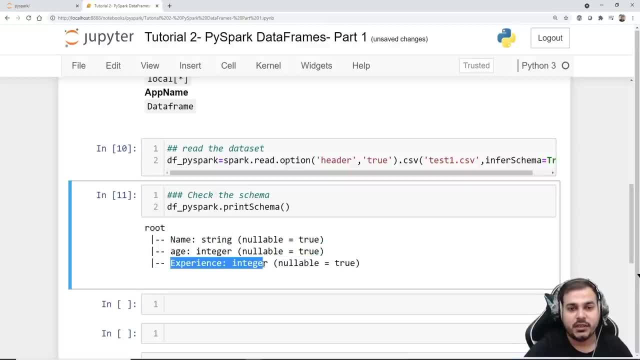 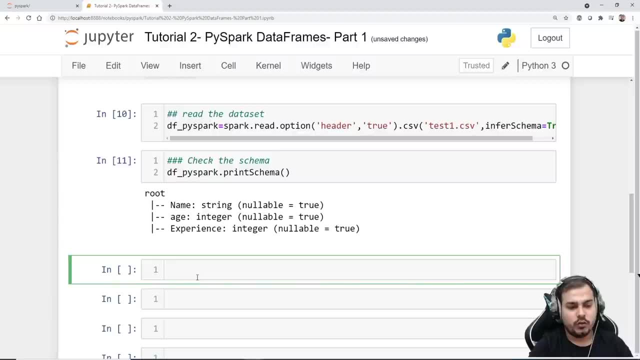 getting name and string, age as integer, experience as integer and the label is equal to two. that basically means it can have null values. okay, so this is one way of reading it. one more way i'll try to show you, which is pretty much simple, so i can include both header and info schema in one. 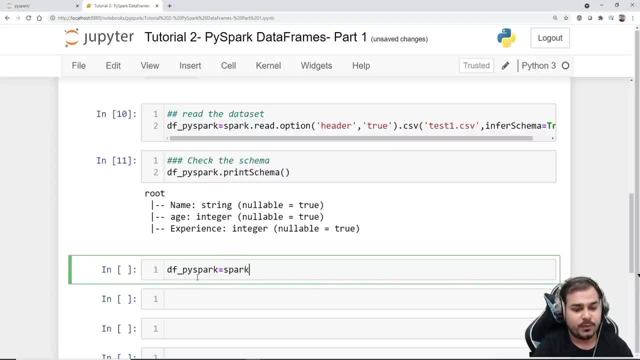 thing itself. so i'll write d f underscore pi, spark is equal to spark, dot, read dot csv and inside the csvl. first of all i'll provide my test file, csv, okay, and then here i will go ahead and write: header probably is equal to true and i can write info: schema is equal to so when i write like this: 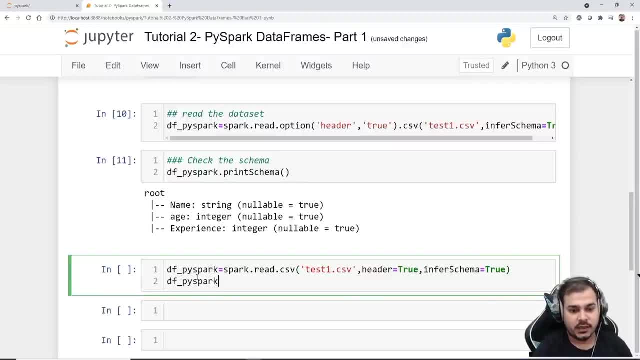 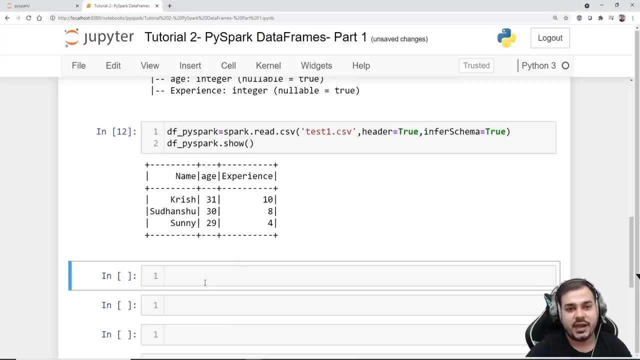 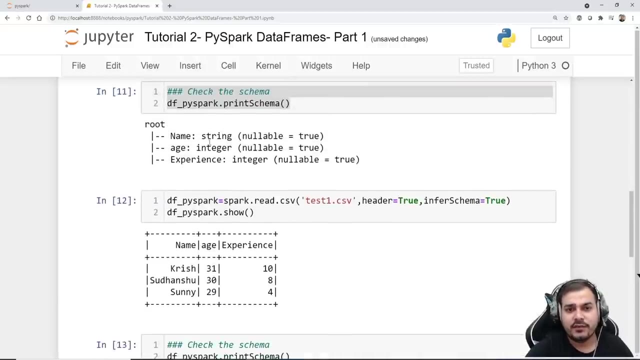 and if i write df underscore pi, spark, dot, show, here you'll be able to see all my data set. okay, so here is my entire data set. now, if i go and see and execute this schema again, it will probably give me the same way, like how we have we had over here. okay, so here you can see name. 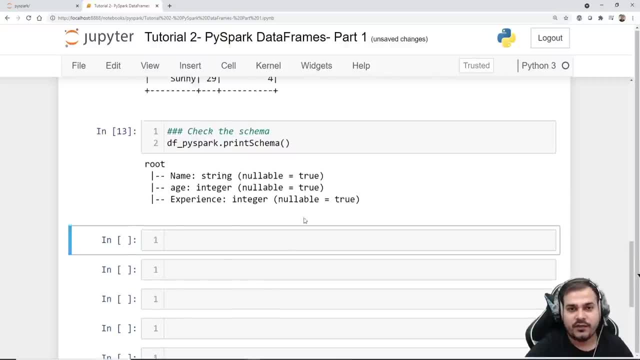 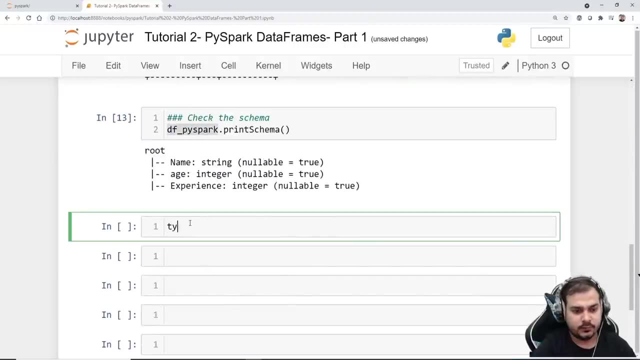 is equal to string, age is equal to integer, experience, integer, integer, perfect. so what? all things we have done? we have uh understood about this one and right, if i go and see the type of this, if i go and see the type of this, this is basically a data frame, uh pandas also have. 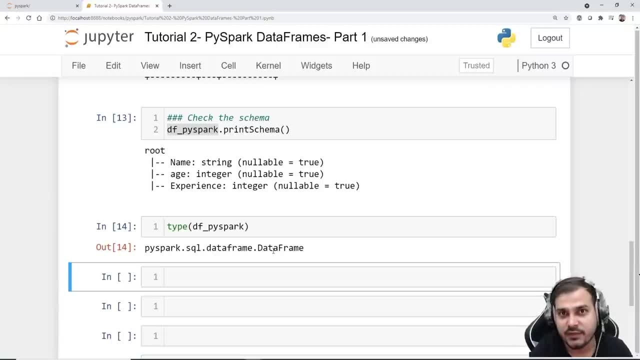 a data frame. so if somebody asks you an interview, what is the data frame, you can basically say that data frame is a data structures, you know, because in this you can perform various kind of operations. so this is also one kind of data structures. okay, so what all things we have actually done? uh, i've given an introduction of data frame reading. 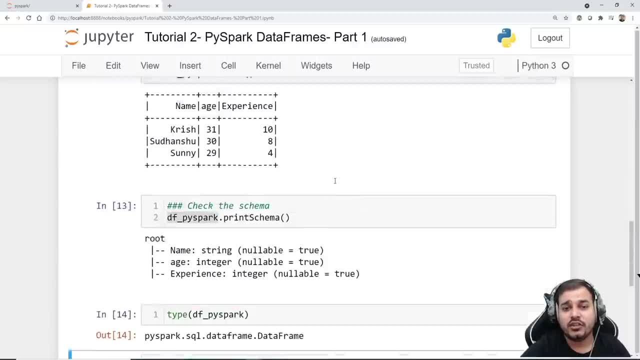 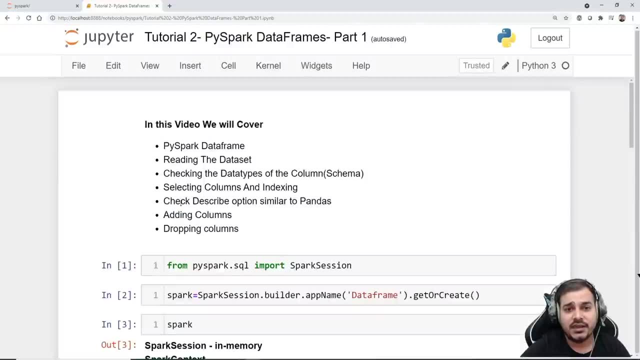 the data set. now checking the data types of the column. in order to check the data types of the column, we have already just written print schema. okay, now one more thing that i can do after this. let's see selecting columns and indexing. first of all, let's understand, uh, what all columns are. 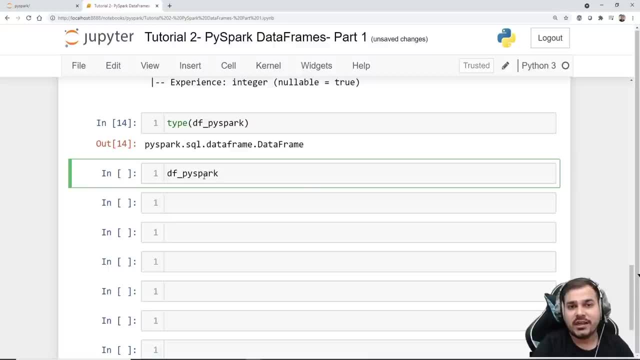 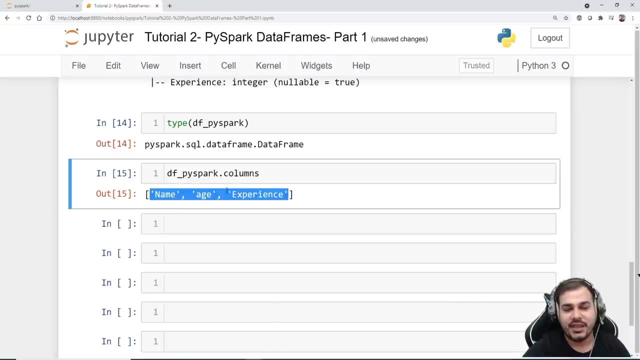 basically present how you can get all the column names. so, in order to get the column names, you can just write dot columns, okay, and when you execute over here you'll be able to get the column name like name, age, experience, perfect, this is perfectly fine. now, this is my df. now suppose, if i want to pick up some, 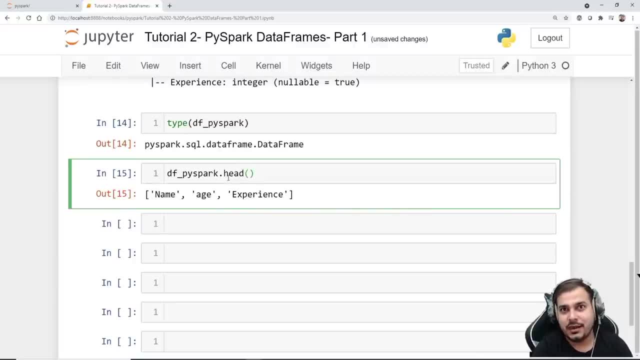 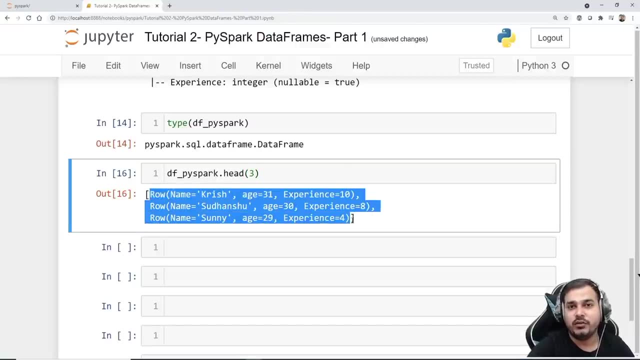 head elements also i will be able to pick up, because in pandas also you have an head suppose. i see i want to get the top three records. i'll be getting in this particular format in the list format. usually in pandas when we are using we usually get in a data frame format. so here you'll. 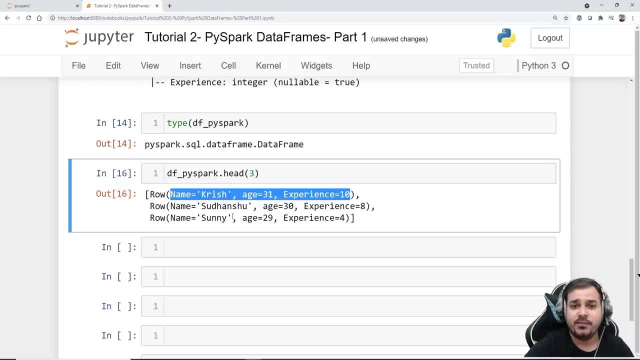 be seeing the combination of name, age and experience. okay, like this. this is my first row, this is my second row. this is my third row. okay, now, coming to the next thing that we are going to discuss now: how do i select a column? you know, i probably want to pick up a column and see all the elements right, like how we do it in pandas. 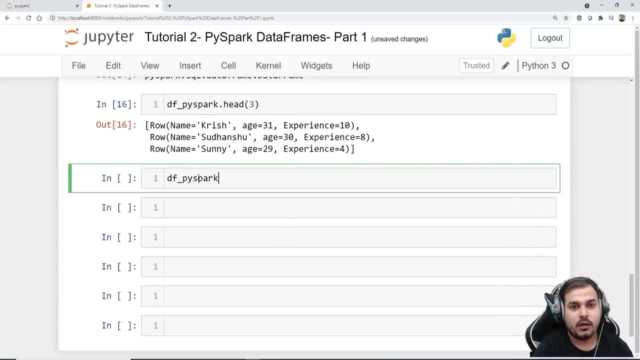 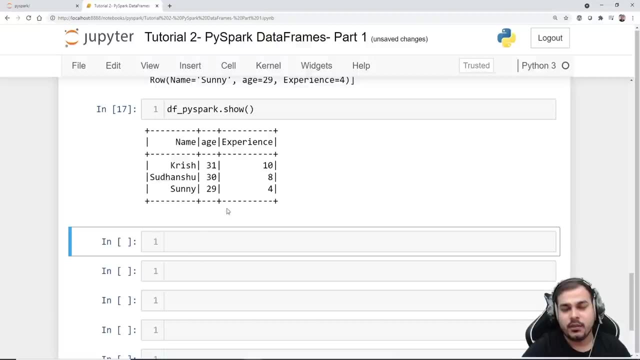 so, uh, first of all, let me just write it like this pi spark dot show: here you'll be able to see all the columns. now, if i really want to pick up only name column, okay, so how do i do it? okay, let's, let's actually see. 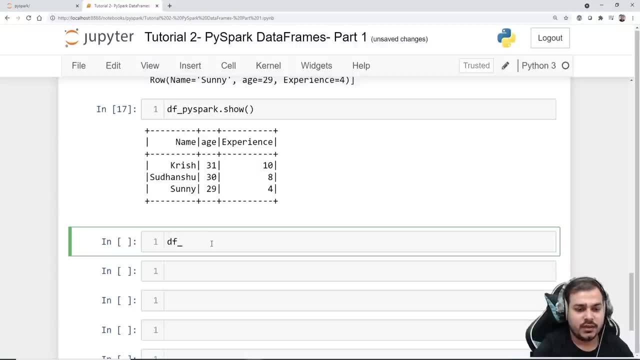 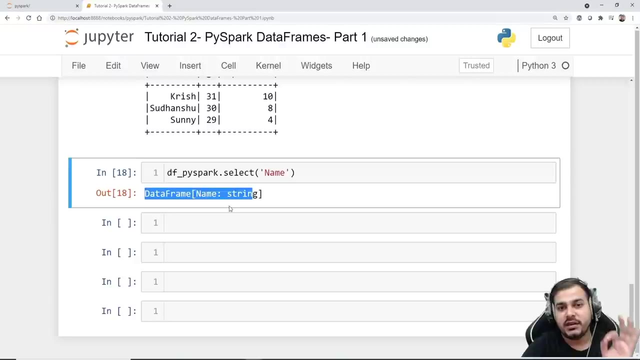 now, in order to pick up the name column, there is very simple uh functionality that we'll write, which is called as pi spark dot select, and here i will just give my name column. now, once i execute this, you'll be able to see that return type is data frame. okay, the return type is data frame. 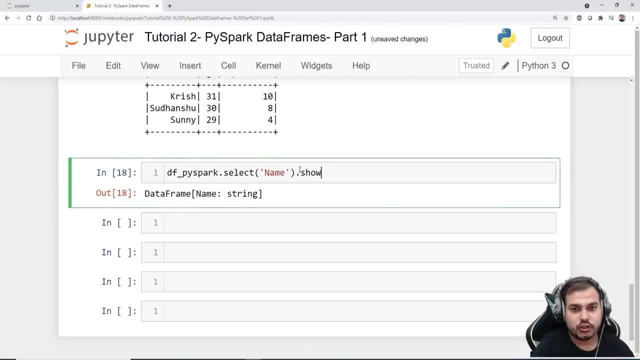 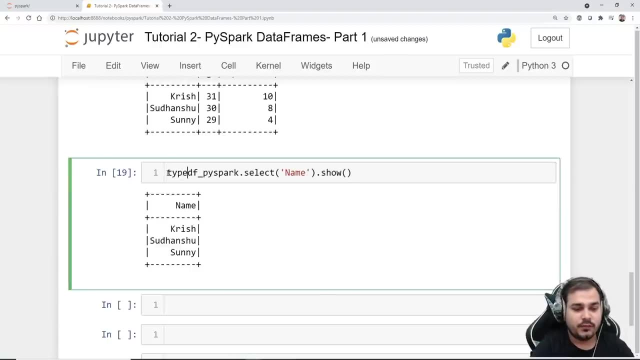 and name is basically a string. now, if i write dot show, i will be able to see the entire column. okay, so when i do this, i'll be able to see this and if i try to the type of this, so sorry, if i remove this dot show and see the type of this. this is basically. 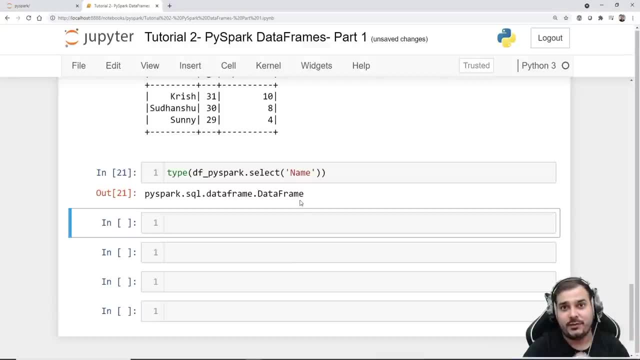 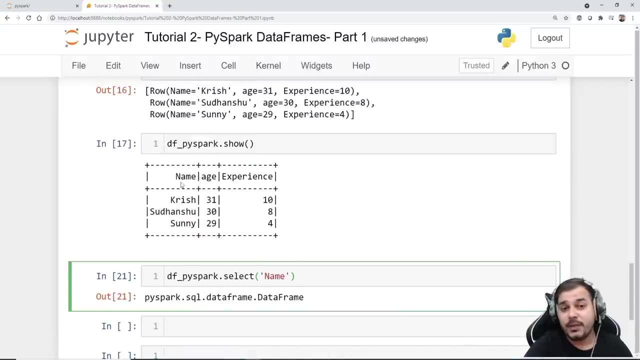 a data frame: pi spark dot sql dot data frame, dot data, not pandas dot data frame. okay, pretty much simple. now suppose i want to pick up multiple rows, like- sorry, multiple columns, like i want to pick up name and experience, probably two columns i want to pick up. so what i'll do? i'll just make one changes. 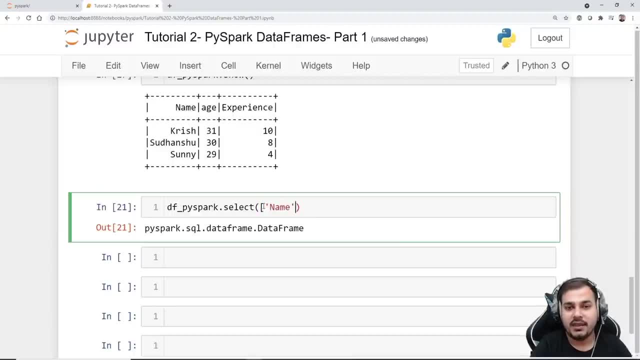 here. initially, i was providing my one column name like this. after this, what i'll do, i will provide another column which is like experience, and i'll execute this now. once i execute this over here, you can see that, guys, i'm getting a data frame with two features. one is name and experience. now, 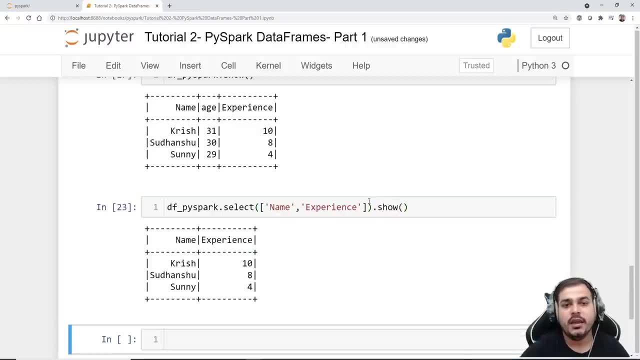 if i go and write dot show here, you'll be able to see my. all my elements are basically present inside this particular data frame. pretty much simple, guys. how do you select multiple rows and yes, uh, here slicing definitely will not work, because i tried doing slicing, it was not working. 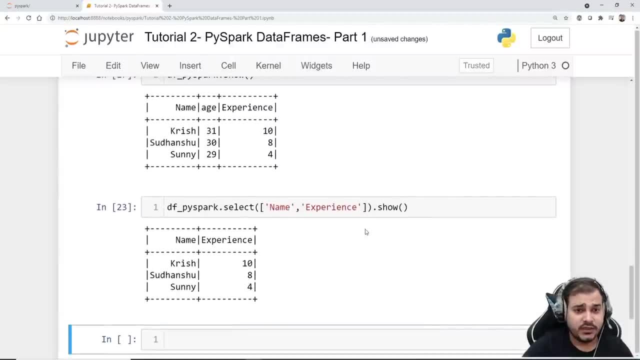 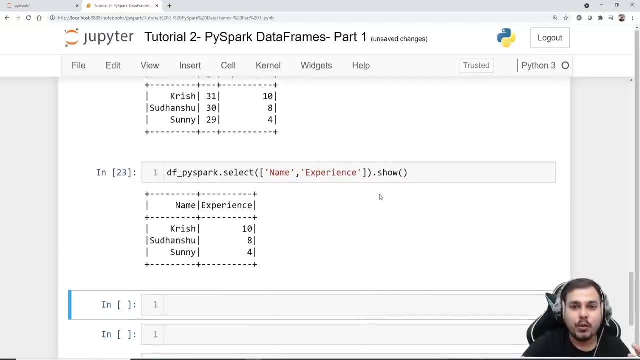 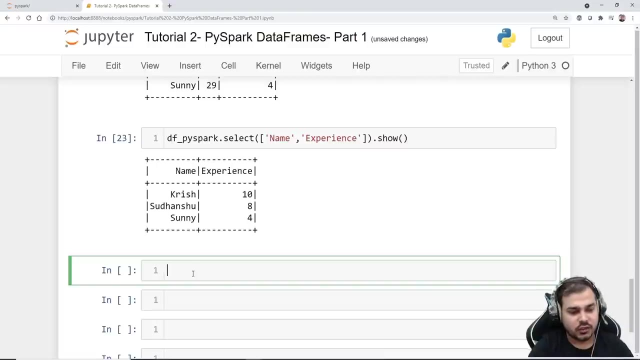 okay and okay. whenever you have any kind of concerns, try to see the documentation, the pi spark documentation, pretty much simple. okay, this is one way uh that, how we can actually select the columns and probably see the rows. okay, now let's show you if i just want to pick up, uh, there is also one way, like this: see if i write df of pi. 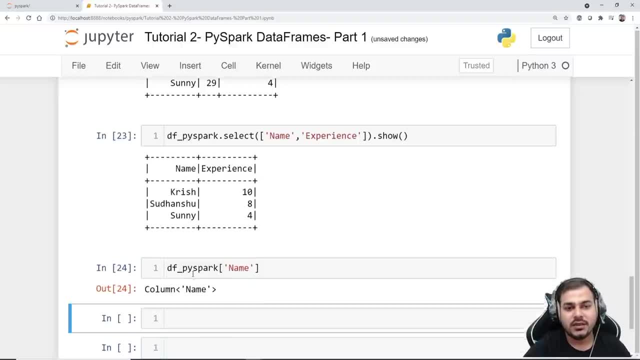 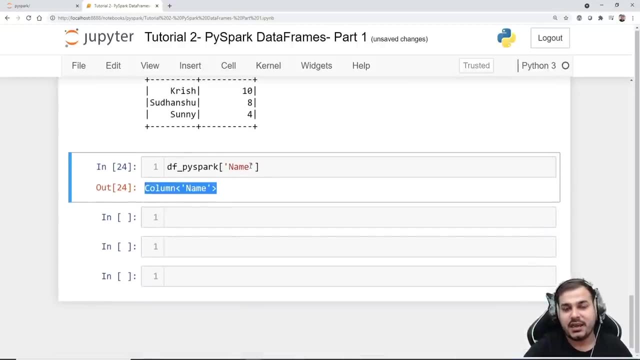 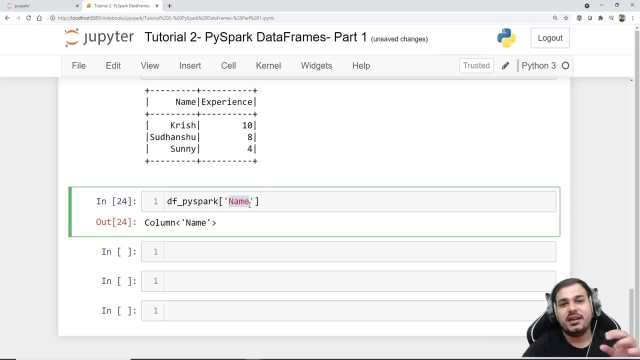 spark of name. if i execute this here, you'll be able to see column name. the return type will be column over here, if i'm directly picking, because in pandas we directly pick like this, right, and when we have this kind of columns, definitely we'll just not. uh, we are just able to understand what this particular feature. it is basically a. 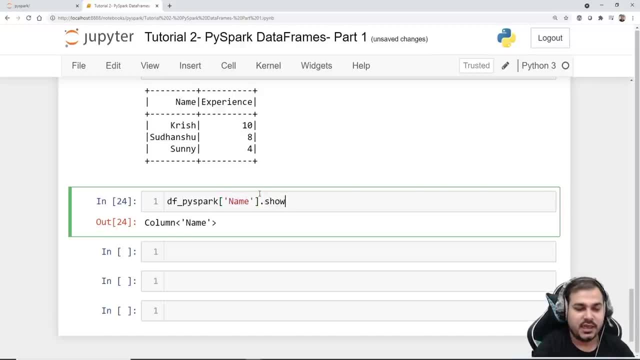 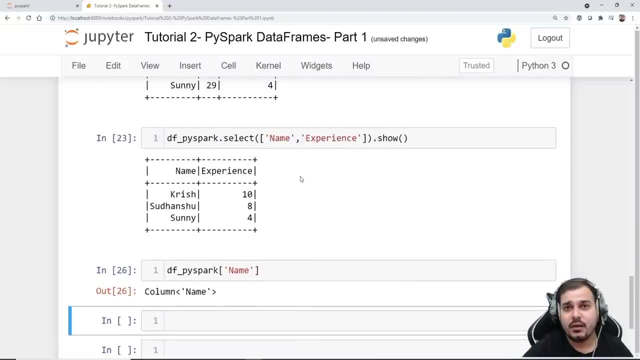 column. it is saying, okay, nothing more, we won't be able to get the data. see, there'll be no show function. it will be saying that, uh, it is an basically an error. so usually what we do, uh, whenever we want to get or pick up any kind of columns and try to see it, we basically need to. 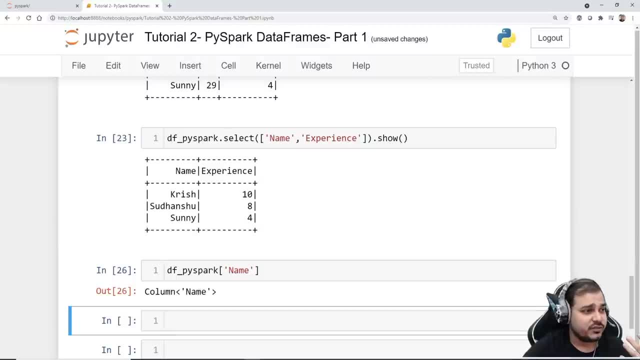 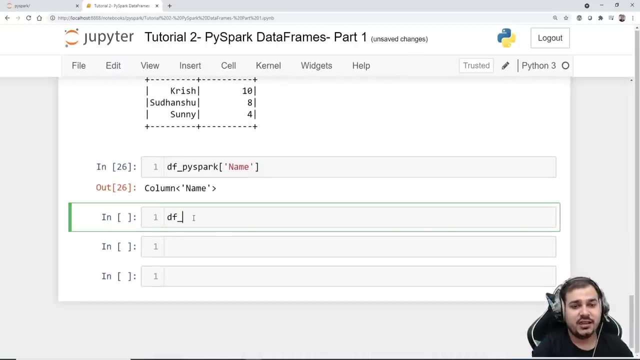 select, uh, using this particular select operation, which is my function. okay, so, uh, these all things have been done, guys. uh, what we try to understand now let's see how we can check the data types. so there is a functionality which is called d types, so here you'll be able to see name is 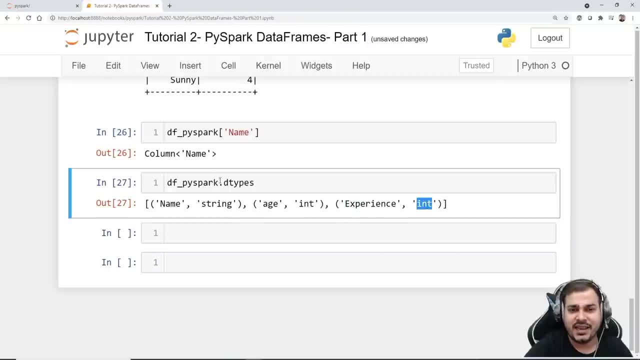 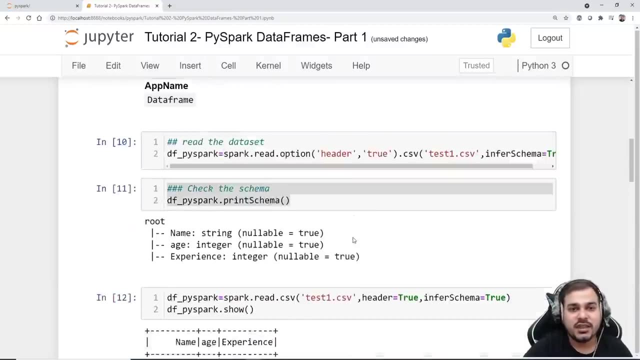 called the string. age is equal to int, experience is equal to int and again, d types is pretty much similar because we also use this in pandas. okay, most of the functionalities are similar to pandas, guys. so what are the things we have actually done? let's see. uh pi spark data frame reading. 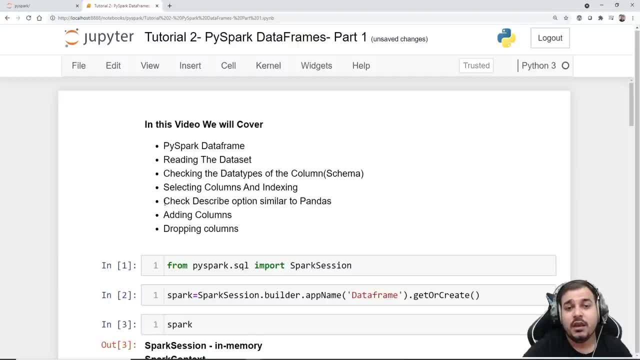 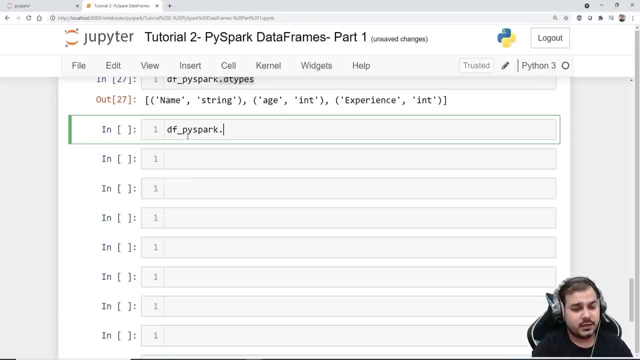 the data set, checking the data type, selecting columns and indexing. check the describe option, similar to panda, so we can also check out the describe options. so let's see pi spark dot describe and if i execute this, you'll be able to see. it will give you a data frame summary is: 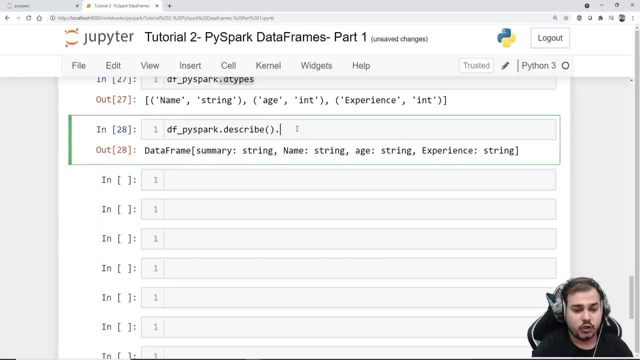 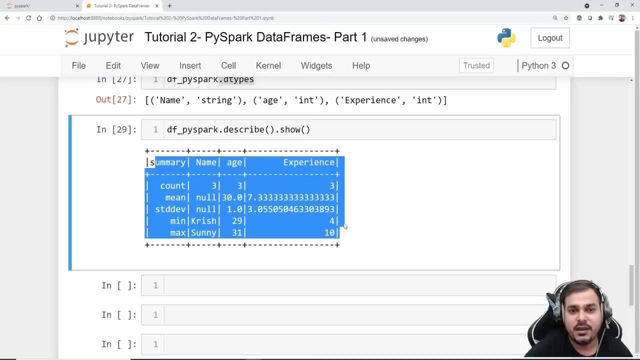 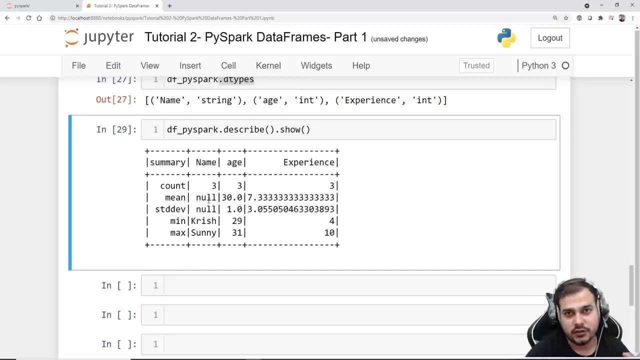 equal to string. this, this, this information is there now when i write dot show: okay, you'll be able to see all this. this is basically in the form of data frame. you may be thinking why this null value is coming, mean and standard division, because understand, even in this it will take the string column also, basically the values that are having the data type. 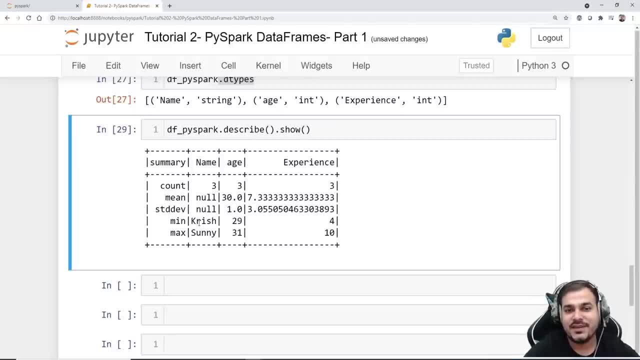 as string over here. obviously you don't have anything. so min and max is basically taken on the index. uh, because in the zero in the second index you'll be able to see trish is there and after that sun is there. okay, in the fourth index and remaining all this information are actually present, okay. 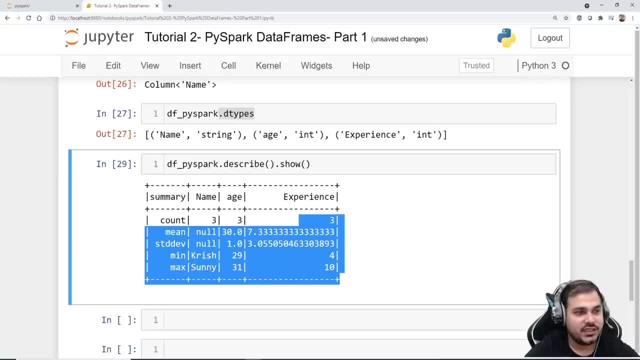 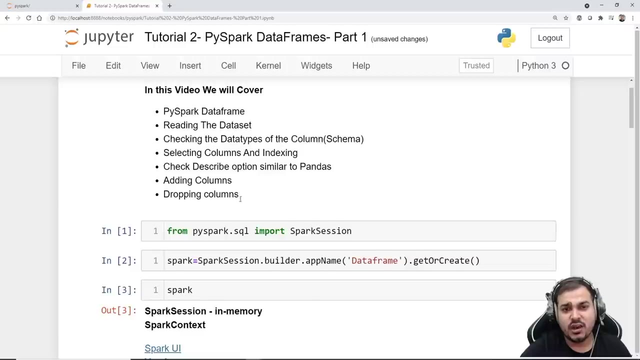 so this is basically the same, like the describe options that we had actually seen. um, you know, probably in- uh, our pandas, right. so, similarly, we have actually done that. okay, so describe option is also done. so now let's go and see adding columns, dropping columns. okay, adding columns and dropping columns. this is very, very much simple, guys. if we need to add the column, 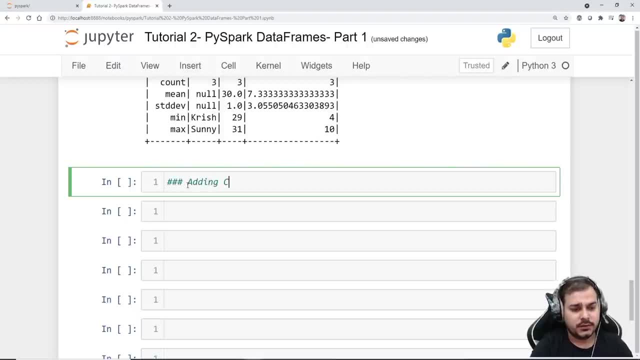 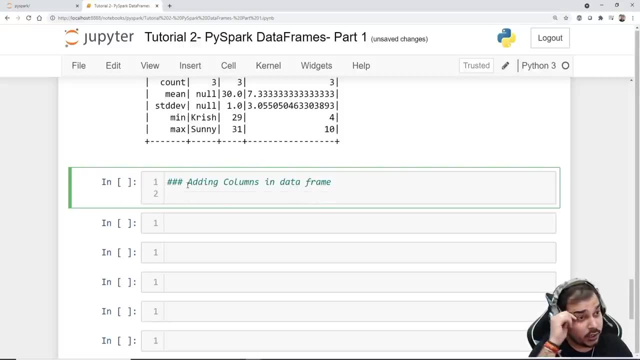 so i'm just going to write the comment over here adding columns in data frame, and this data frame is pi pi, uh, pi spark data frame. okay, now, in order to add the column. so we have an amazing functional function which is called as df pi spark dot. there's something called as width column, okay. 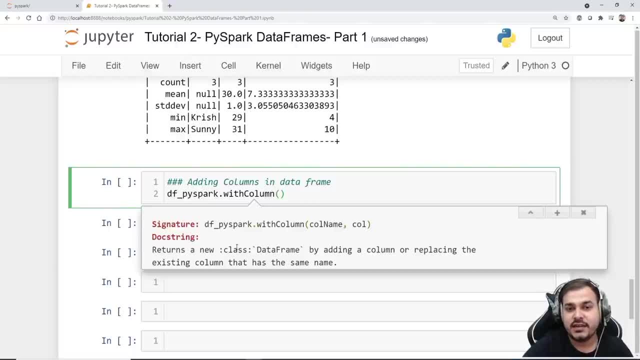 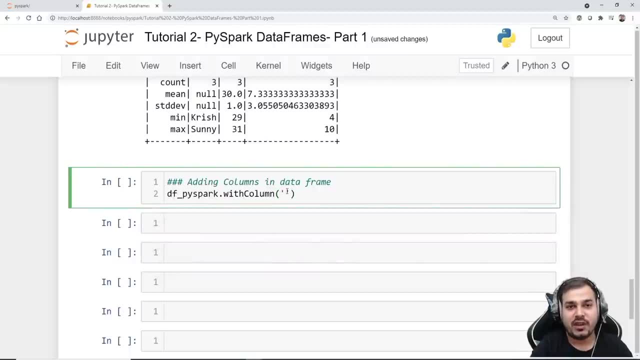 now this width column. if i see the functionality, it returns a new data frame by adding a class or replacing the existing column that has the same name. okay, so here, the first parameter that i'm going to give is my column name. suppose i want to pick up, let's see. uh, i'll pick up experience. 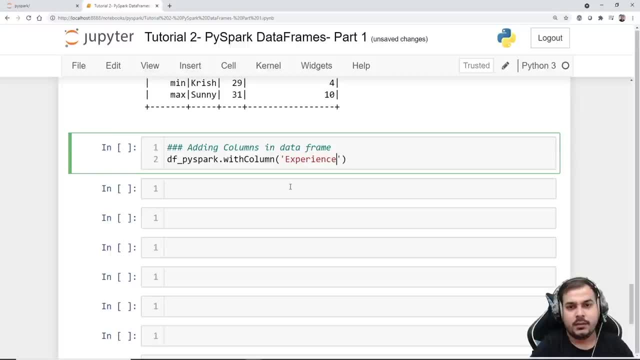 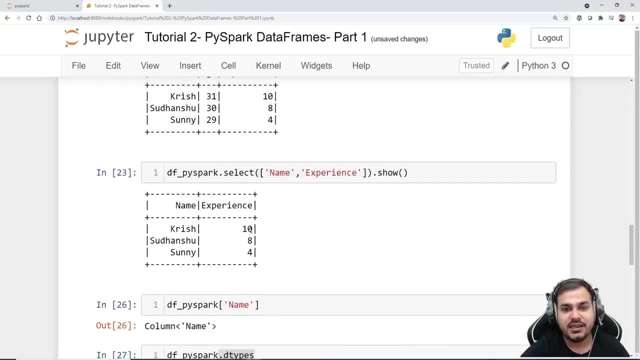 so i'll say experience, okay, and uh, probably this will be my new column- after two years. what will happen if experience after two years? you know, initially the candidate is 10 years experience, after two years it will become 12, right, so we'll try to put now the value. this is my new column. 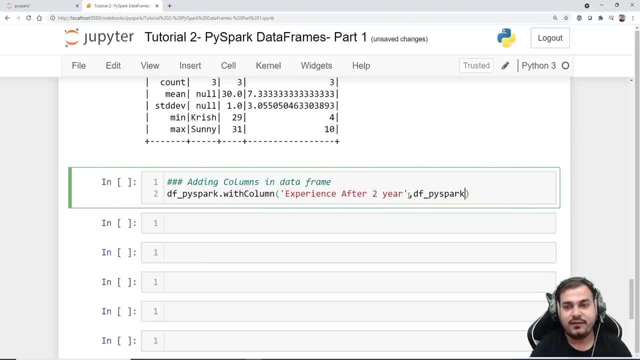 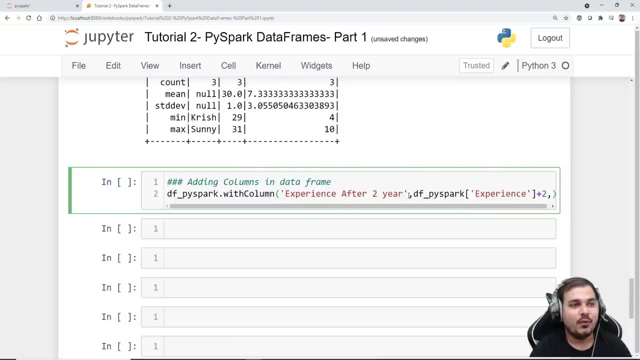 name and what value it should have. so for that i'll write df pi spark. and here i'll say: uh, probably i'll take that spam experience, i will multiply it by. i will add by two, because after two years the experience will get added by two. just i'm taking one, one way of actually solving this. uh, i can put. 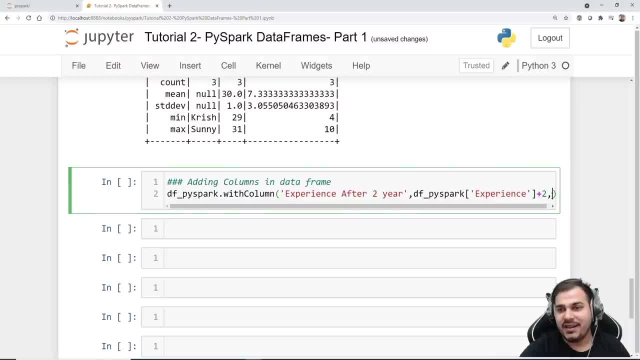 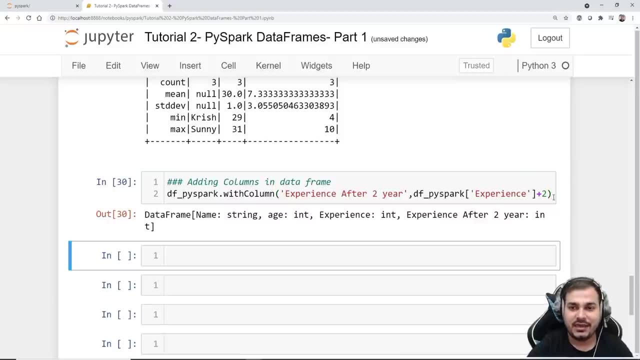 any values i want, guys, uh, it is up to you, okay, and you can actually check it out. okay, now, after this, uh, this is only the two things that is required, and now, if i execute it, you'll be able to see that some operation will happen. and now you, in this data frame, you have one, two, three and four feature. 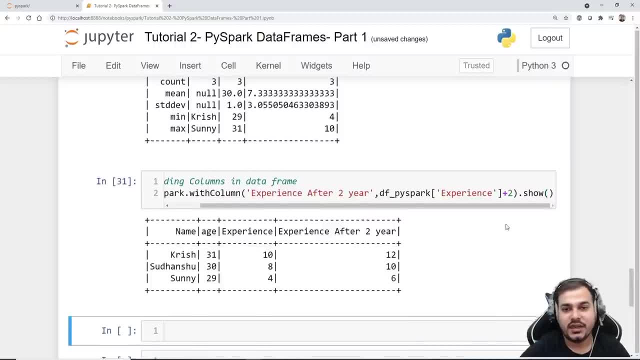 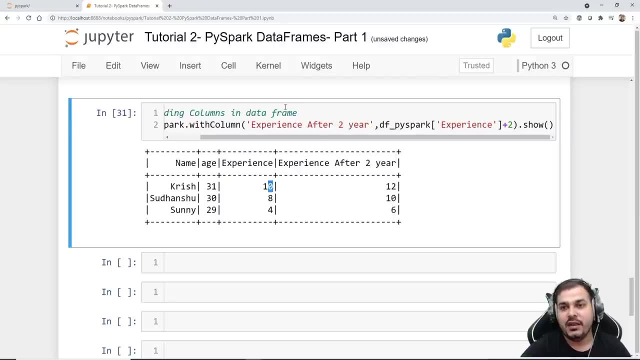 data set. i can write dot show. once i execute it now here you'll be seeing that experience after two years is nothing but 12, 10, 66, because 10 plus 2, 12. you have very, very simple guys, and this is what with column is basically: uh told, uh as, and you can also do different, different things with. 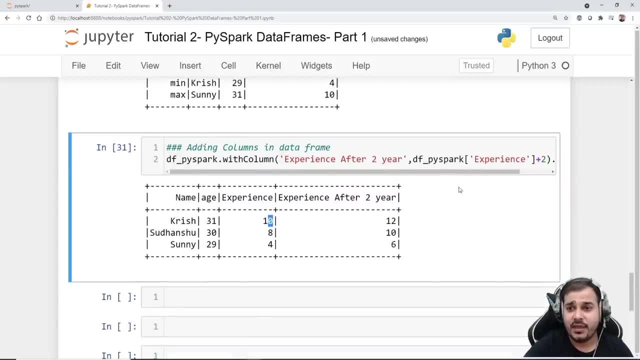 respect to this. so this is how you can add a column in a data frame. and again, guys, this is not an in-place operation. you basically need to assign it to a variable in order to get reflected. suppose? if i want to get it reflected, i really need to assign? 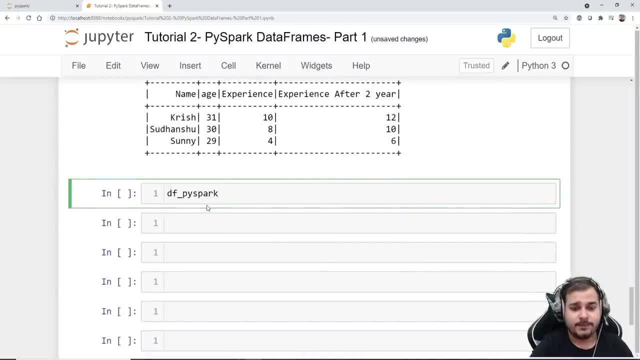 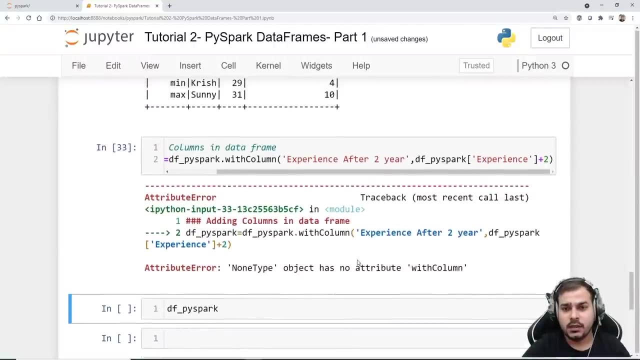 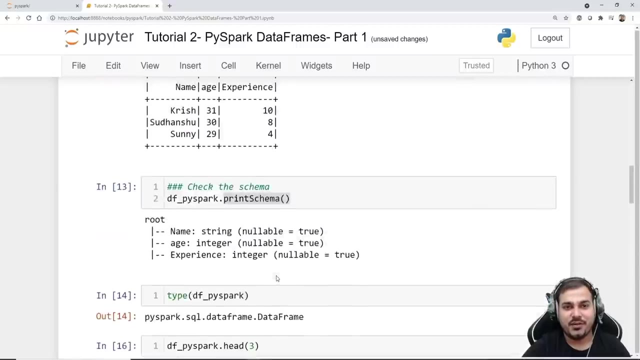 like this and here now, if i go and see my sorry, first of all, let me remove this show. the show will not give us proper result. okay, oh, has no attribute with column. okay, sorry. so this, there was a problem with respect to this. i'll read this data set, because i replaced it completely. 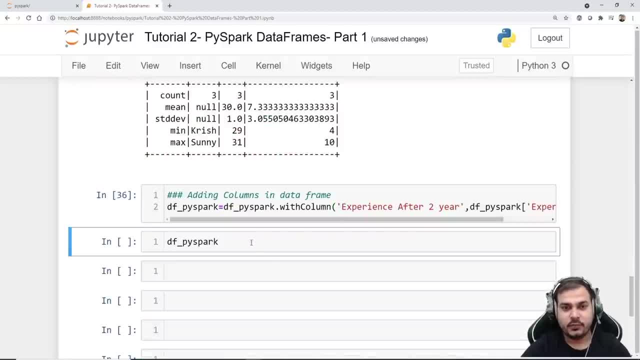 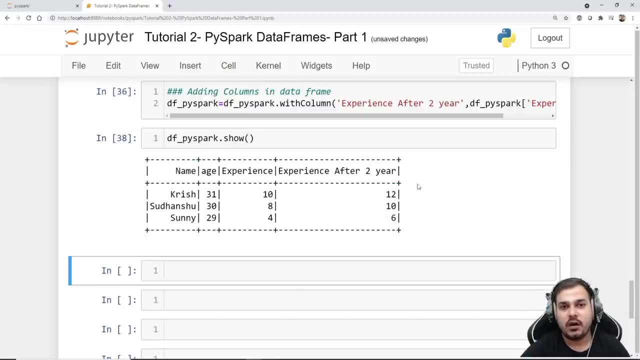 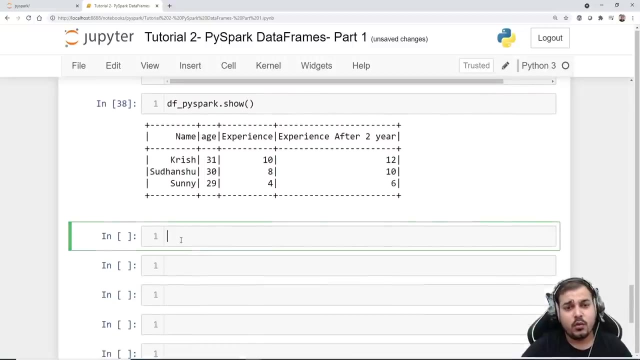 right now. i will execute it once again now. yes, fine, now if i go and write dot show here, you will see the elements all properly given now. this was with respect to adding the columns with data frame. now i probably need to drop the columns also. so drop the columns, let's see how we can. 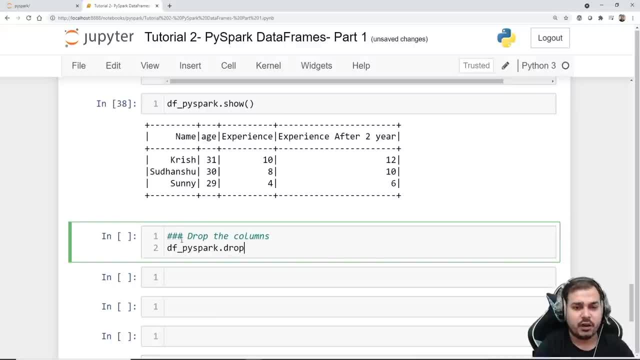 actually drop the columns. dropping the columns is pretty much simple, like how we usually drop this. drop functionality by default. take column names: you can give a list of columns. you can give a single column name. so suppose i'll say experience: after two years i want to drop this. 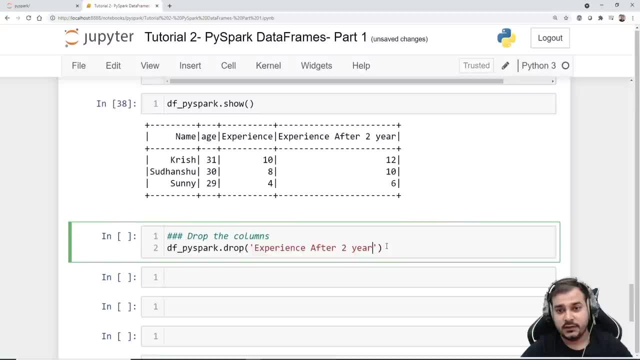 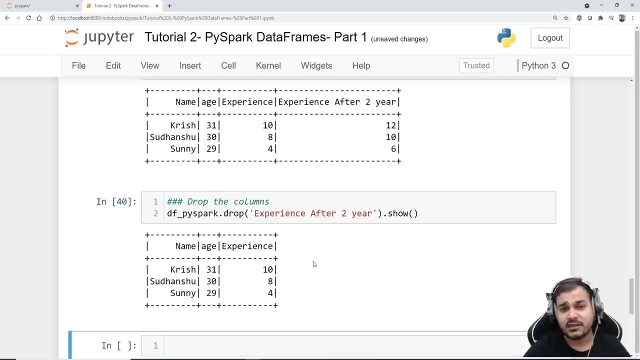 because who knows after two years what will happen. so let's drop this. in order to drop this, just execute like this and just go and see dot show here you will be able to find out without that specific column again. this is not an in place operation. you need to assign it to a variable. very much simple, so let me just assign it. 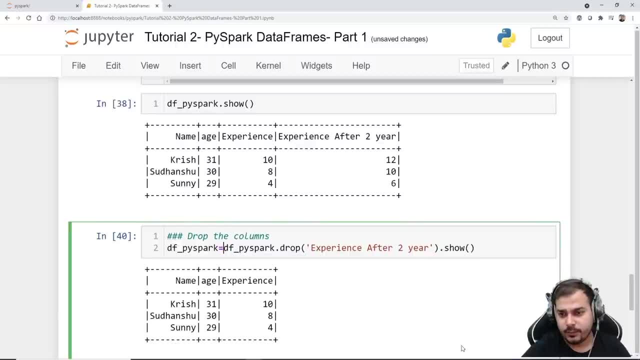 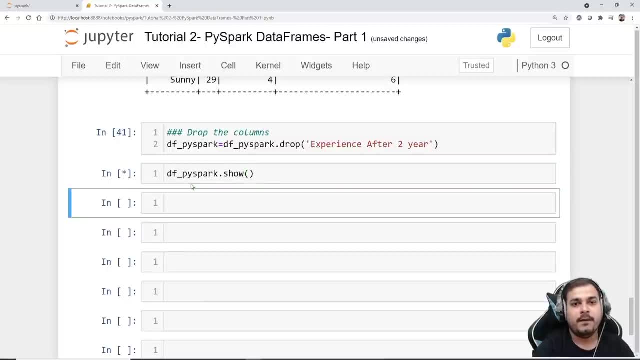 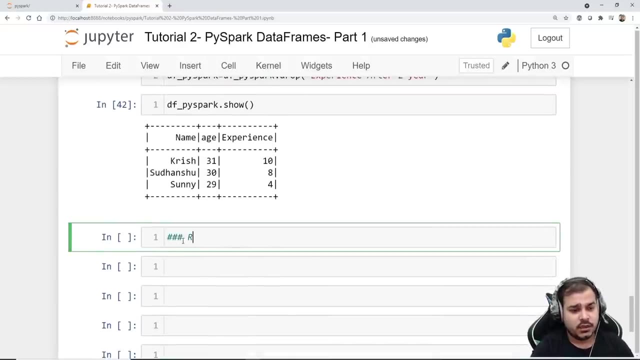 to a variable is equal to: and please make sure that you remove this dot show. dot show is the functionality right now. if i write this dot show here, you will be able to see all the elements. good, now let's go ahead and see how to rename the column. so we are just doing this, guys, because you really 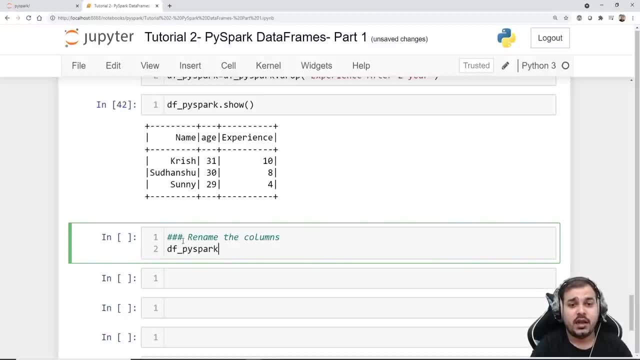 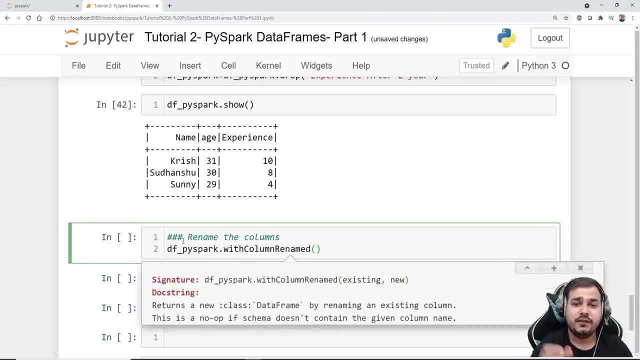 need to be very good at data pre-processing. okay, so i'll write dot. and there is another function which is called as with column renamed. okay, now in this you just give your existing and the new column name. suppose i have my existing column name over here. i'll say name and i'll say new name. 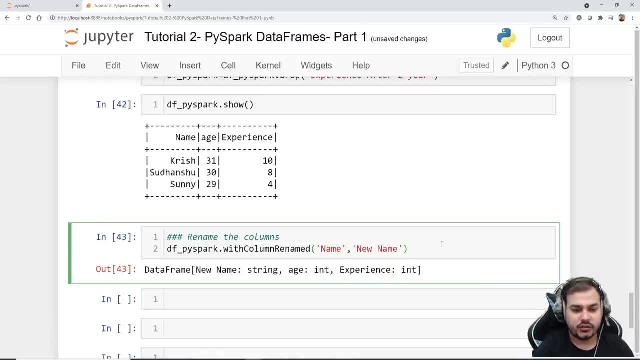 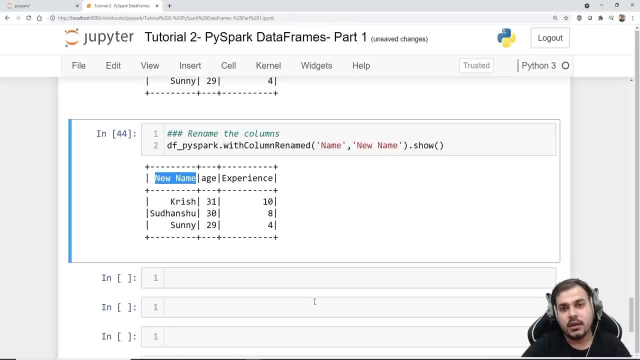 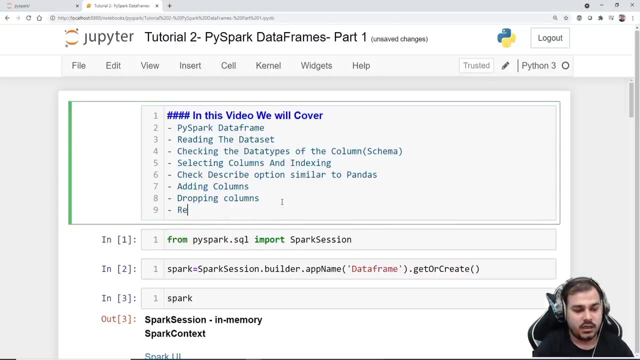 okay and just execute it. and now if i give this dot show- here it looks like this- and just write dot show, just complete it and finally complete the whole check portion, this is the goosebumps supervise filter option. okay, now, that's pretty much it right now. so now let's go and just write dot show and try to see the elements. 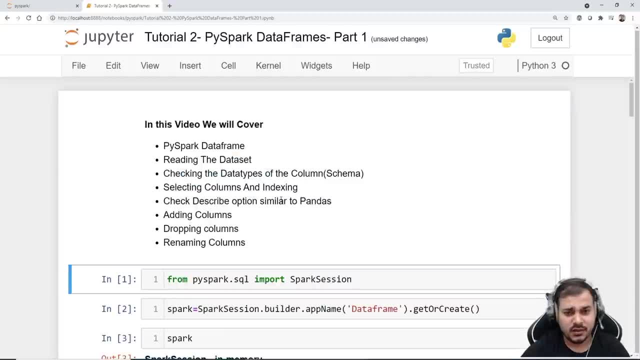 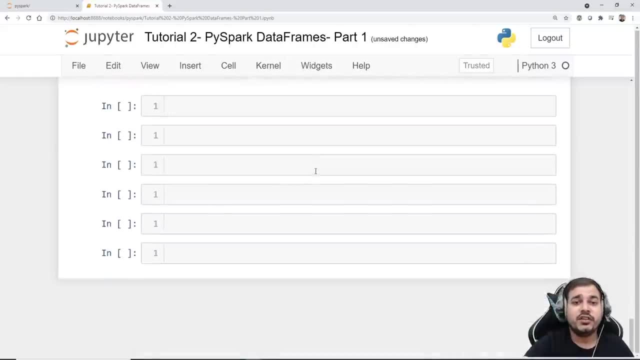 here you will be able to see, instead of name, there will be something called as new name. right now, this is what i had to actually discuss. i am just writing one more point over here. we have also discussed about renaming columns right now. uh, yes, this is just the part one of data frames. the part two will 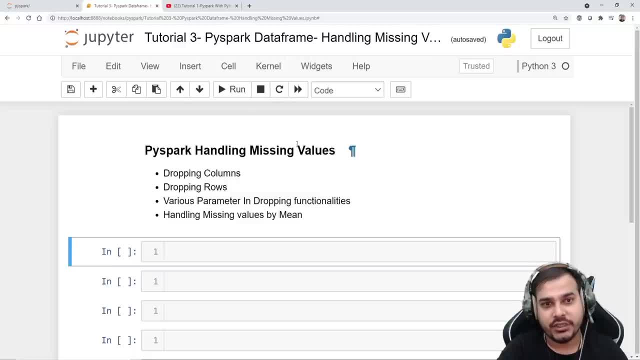 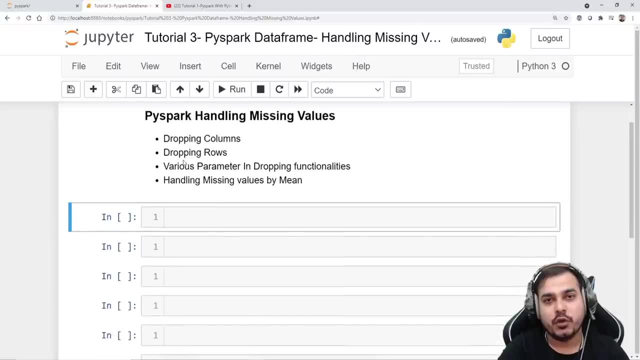 tutorial 3, which is the part 3 with respect to data frame operations. in this particular video, we are going to see how we can handle missing values, null values, you know. so, in short, this many things we'll actually try to do. we'll see how to drop columns, we'll see how to drop rows. 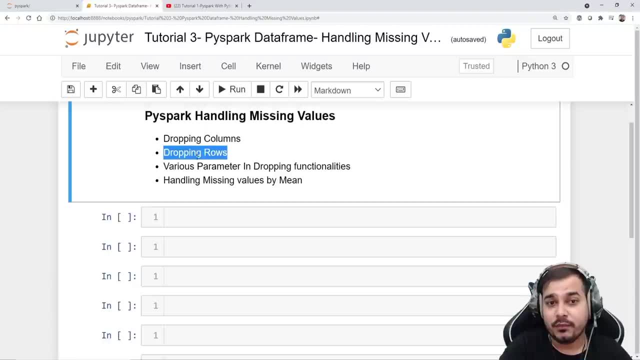 then we'll see when, when we are dropping rows, probably based on a null values, we'll try to drop a rows and then we'll try to see what are the various parameters in dropping functionalities and handling missing value by mean, median or mode. okay, so here i'm just going to write it as mean. 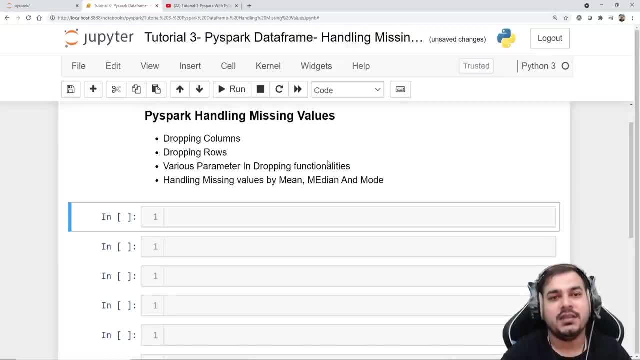 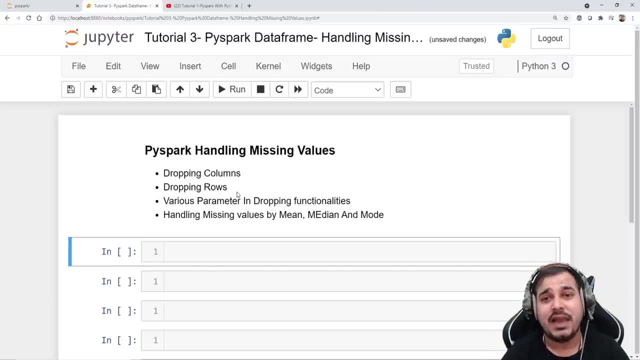 median and more probably right. so all these things we are actually going to see again. the main thing is that i really want to show you that how we can handle the missing values. this is pretty much important because in pandas and all also we try to do this in a skill on. we have some kind of 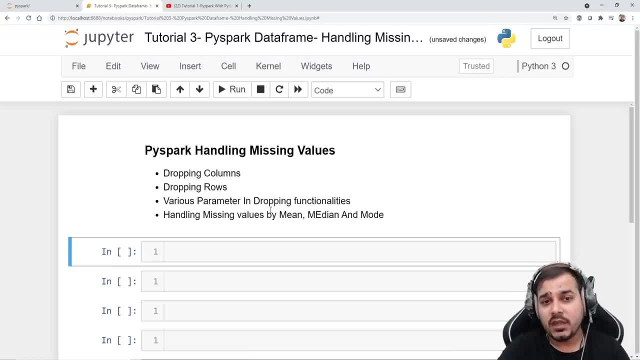 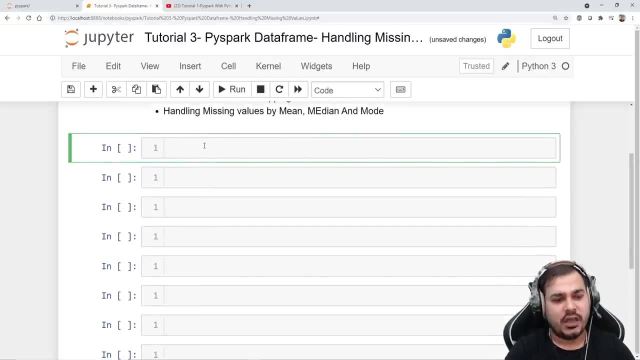 imputer function. so let's proceed up. whenever we usually start a pi spark, whenever we are working with pi spark, we really need to start a pi spark session. so i hope till now you all are familiar. so i'll write for pi spark dot sql. i'm going to import spark session, okay, and then i'm going to create a. 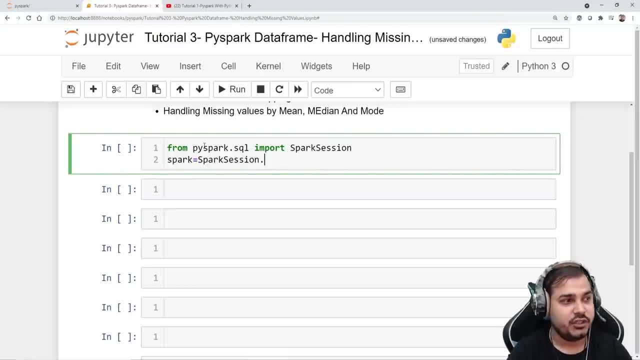 variable with spark. and then here i'm going to write spark session dot builder, not app name. okay, dot app name again. let me just keep this app name as practice, okay, and then we will just create a variable for this. we'll call it a get or create, because i'm just 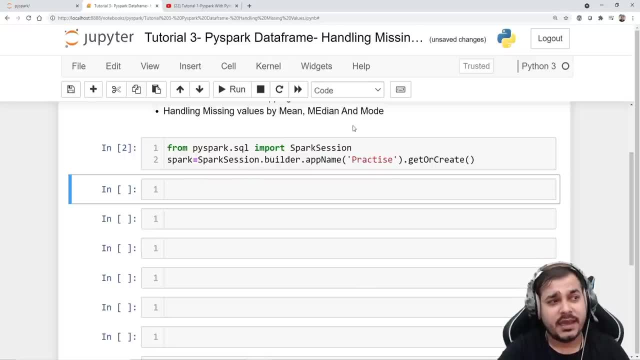 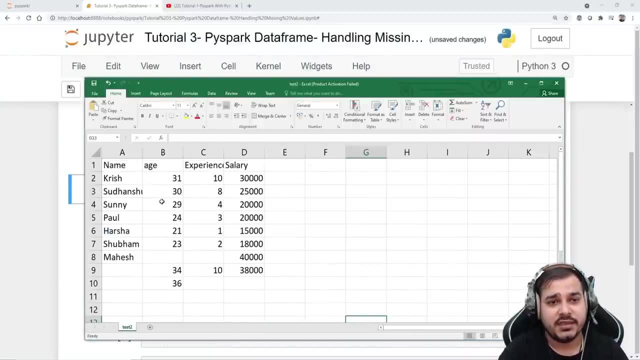 practicing things and then i write get or create and just execute this, so probably it will take some time to get executed. yes, it has got executed. fine, now for this. i've just created a very simple data set which looks like this. i have a column like name, age, experience, 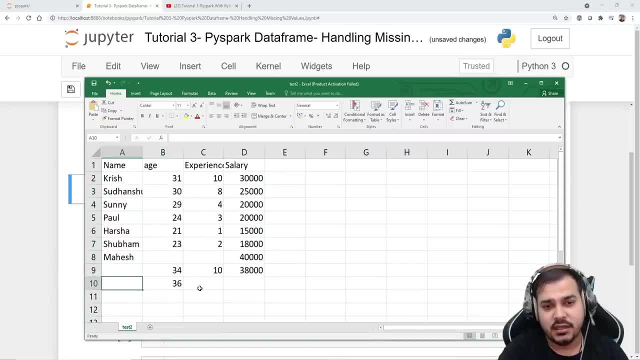 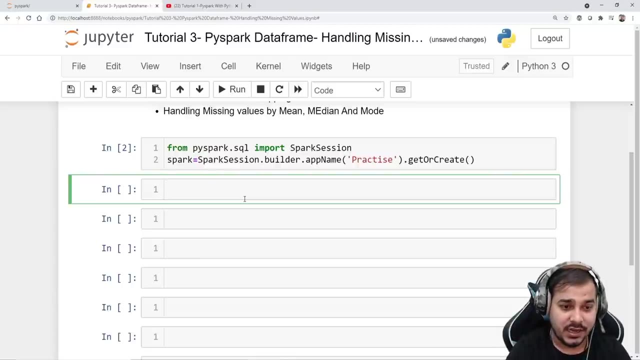 salary. so these are all my names, all the candidate names, and probably there are some values which are left blank. here you can see some values are left blank, null values or how to handle this particular missing values, and all okay, so let's proceed. so, first of all, in order to read the data set, I'll just 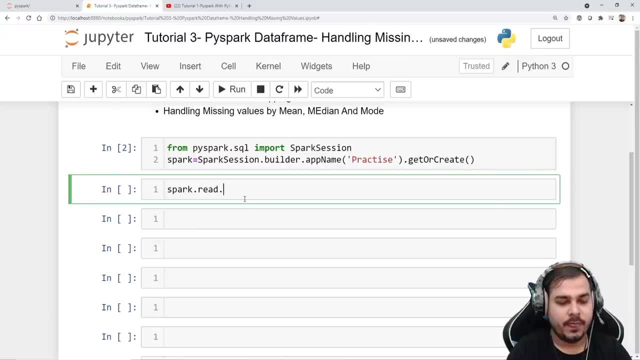 write spark dot. read dot CSV. and here I'm just going to use the CSV file name- test 2 dot CSV, and it is saved in the same location where this particular file is. anyhow, I'll be providing viewed in this github also, and I'm going to use 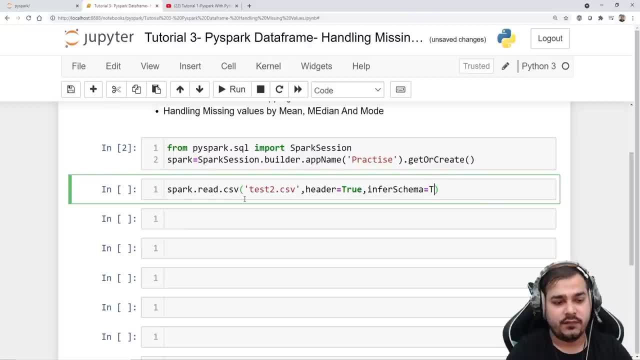 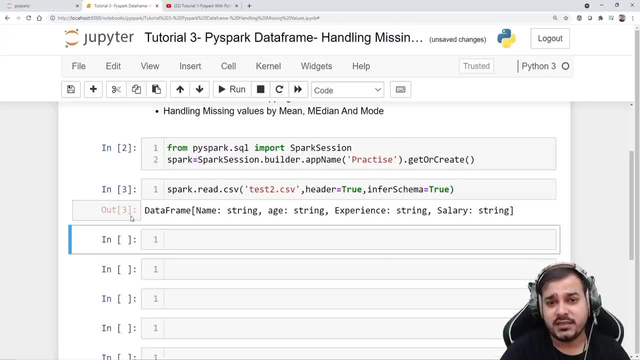 header is equal to true and probably there is also in first schema- is equal to true, so that I'll be able to get the data set properly. so probably when I'm reading this you'll be able to see: this is my data frame, that I'm actually. 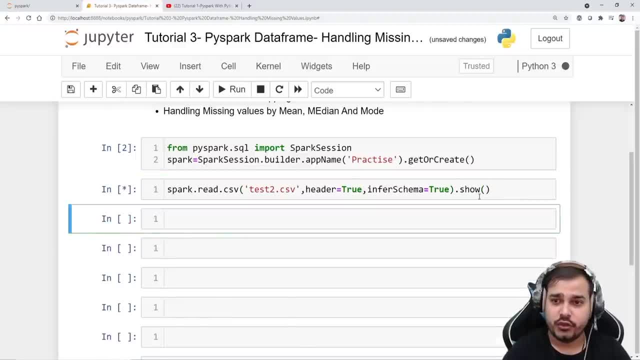 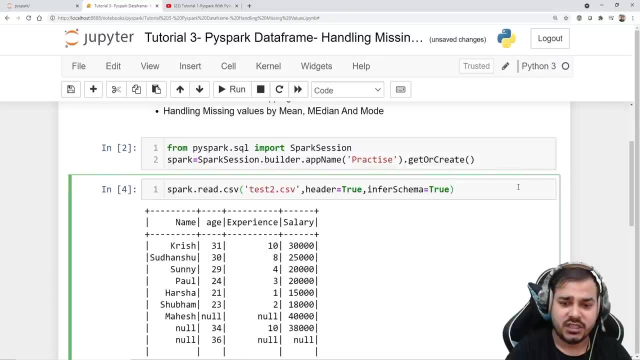 getting. if you want to see the entire data set, this will be like she used dot show and this is your entire data set. here you are having null values and all perfect. so what? let me do one thing. let me just save this in a variable, so I'll. 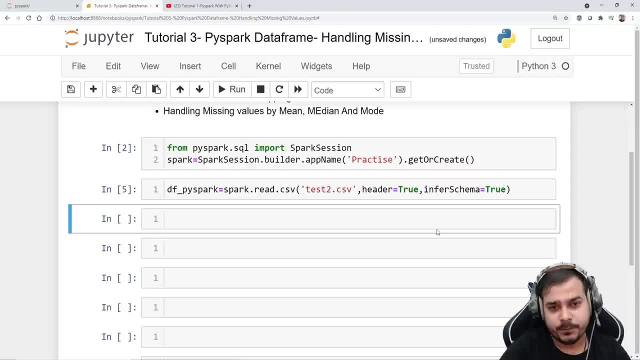 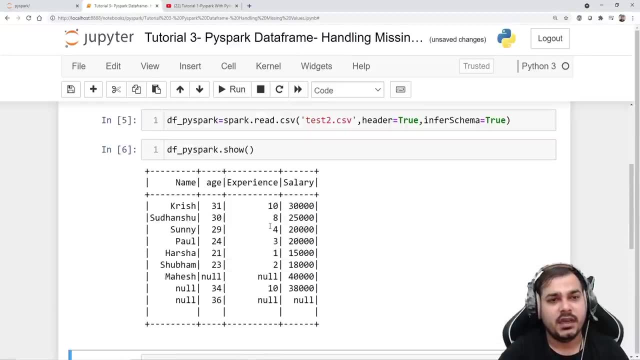 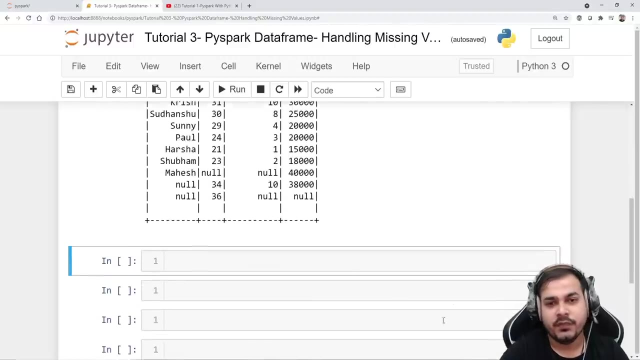 write DF underscore: PI spark. so if I go and now check dot show and this is my entire data set. okay, perfect, we are pretty much good till here. we are working fine with respect to this. we know we have actually read some kind of data set also. now, probably first let's 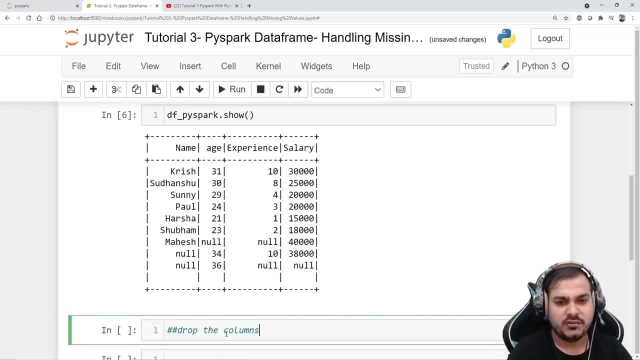 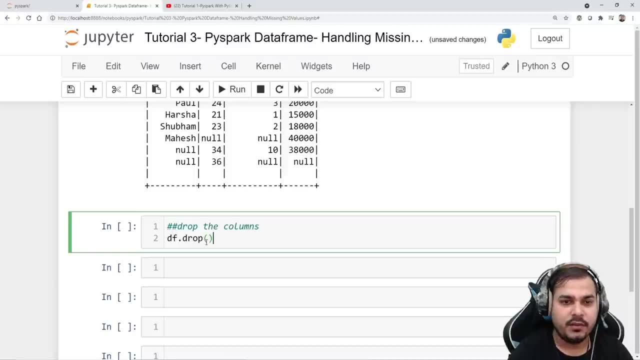 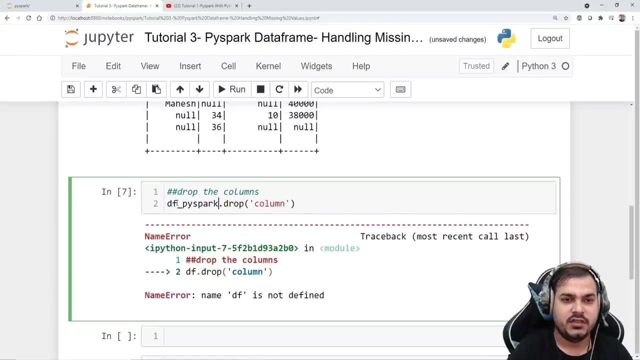 start. how do we drop the columns? dropping the columns is very, very simple, guys. suppose I want to drop name column. then I just use DF dot drop and provide my column name like this: right, so column, right, column name. suppose I'll write D, F, dot pi spark and here column name will. 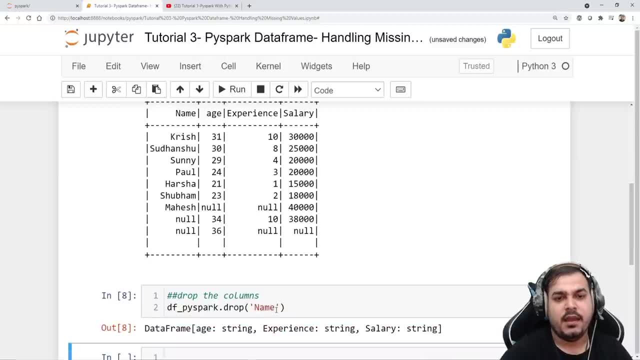 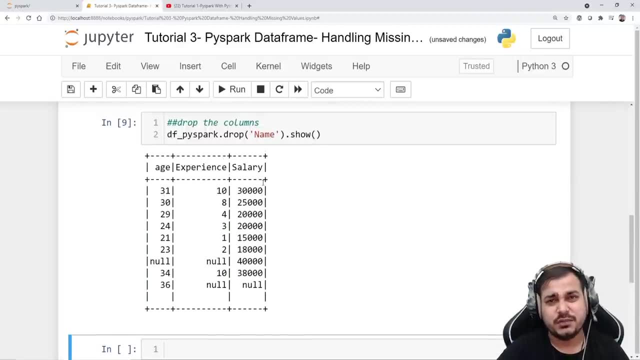 be name, so let me write it as name and I can basically go and check out my dot show and then you will be able to see all the features that are actually present. this is pretty much simple, which I also showed you, probably in the previous session also. okay, and this is how it is basically done, basically. 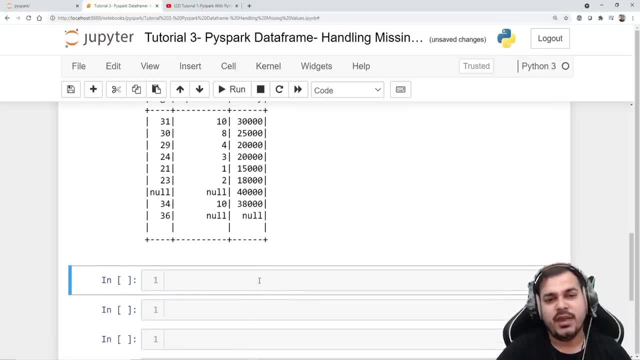 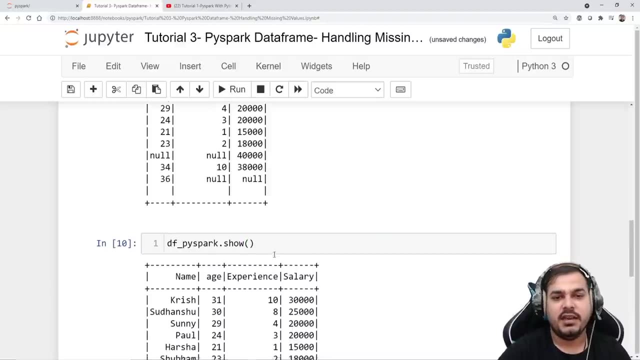 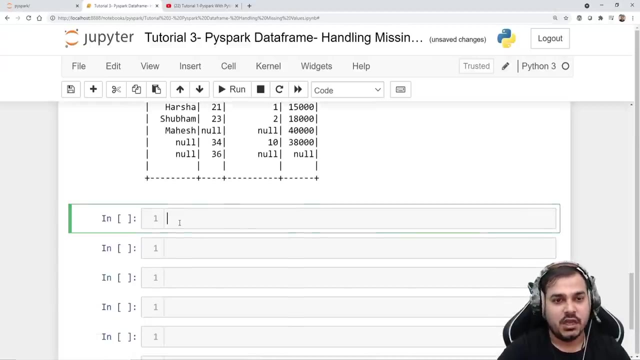 dropping your feature or columns, but our main focus is dropping the nan value. so right now, let me just write df dot by spark dot show. so this is my data set, right, uh, now let's see how to drop this specific rows based on the null values. so over here i'll just use df dot by: 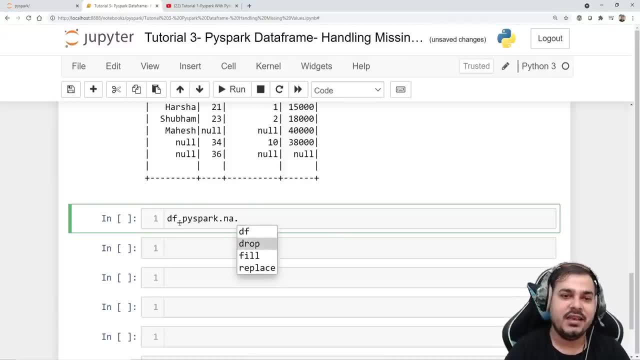 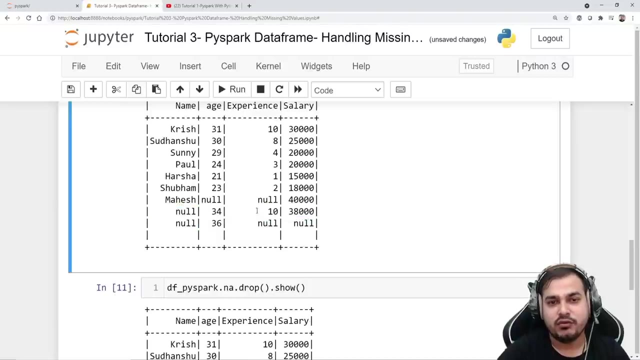 spark dot na. okay, there's something called as na, and then you have drop, fill and replace. so first of all, i'll start with drop. now, inside this particular drop, always remember, if i don't give anything okay and just execute it. here you'll be able to see wherever there is a null values those. 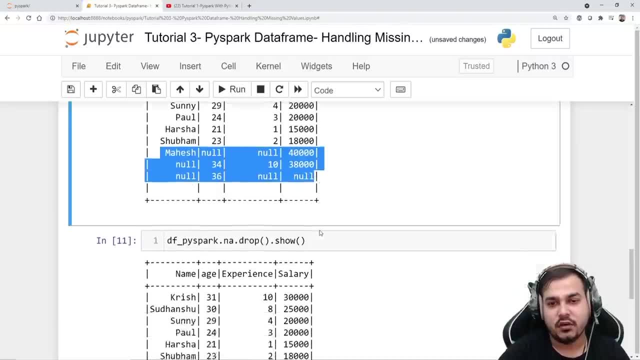 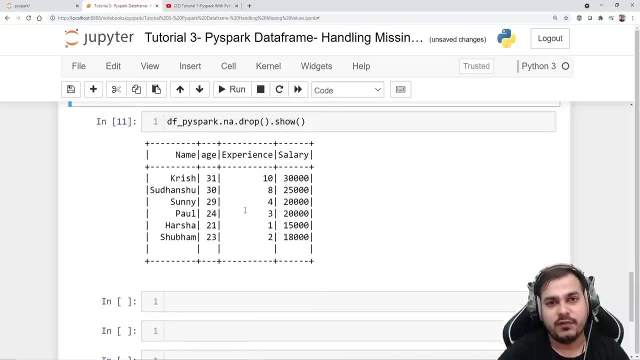 all rows will get deleted. so here you'll be, seeing that this last three rows are not present, right? so here you can see. till shubham, this particular value is present, demanding all the rows has been removed. perfect, right? so not a problem at all. so here you, in short, what you're. 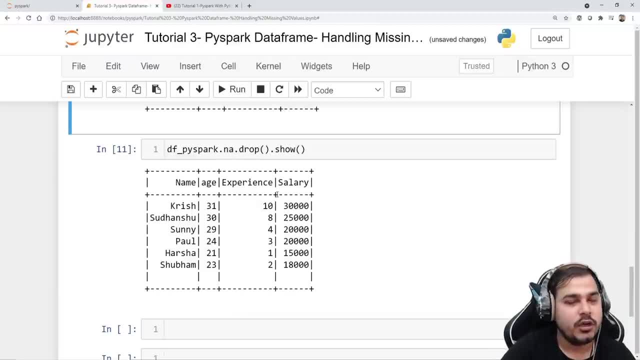 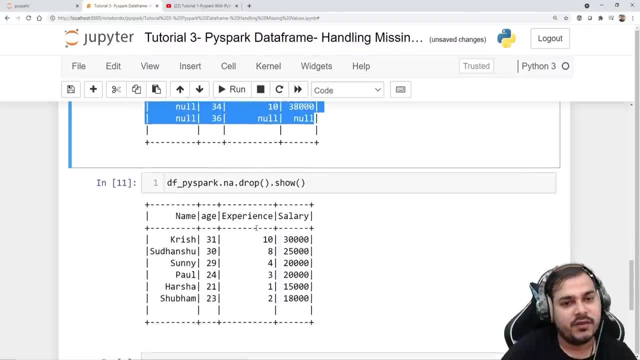 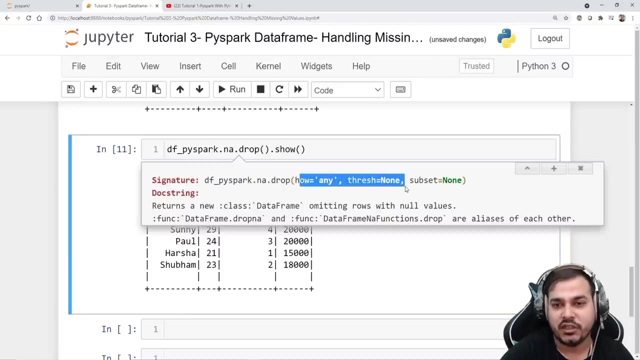 doing is that whenever you use dot na dot drop, it is just going to drop wherever. it is going to drop those rows wherever nan values are actually present or null values are actually present. okay, perfect, this much is fine. if i go and search in the drop, there are two main features: one is how and one is threshold, and then one is subset. so let's try to. 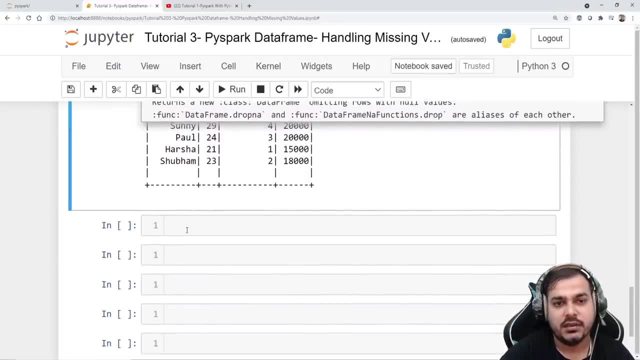 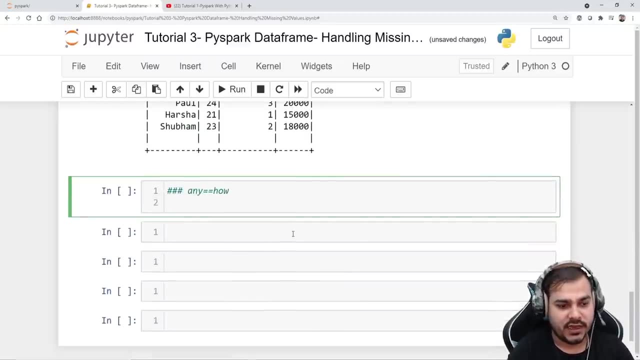 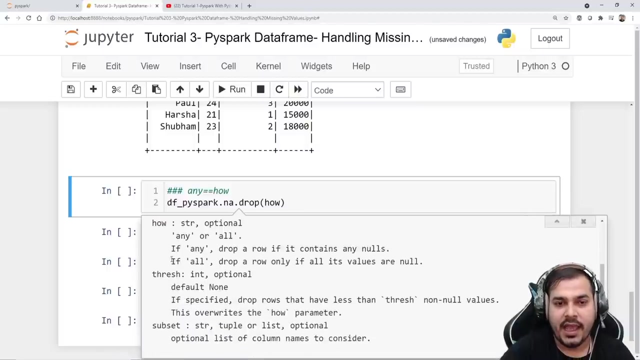 understand this particular features now. first i will start with how. any is equal to how. i'll just write like this: okay, so suppose if i write df dot by spark, dot na dot drop, and if my how, how, the how value can have two values. one is any, one is all okay, one is any, one is all any if the 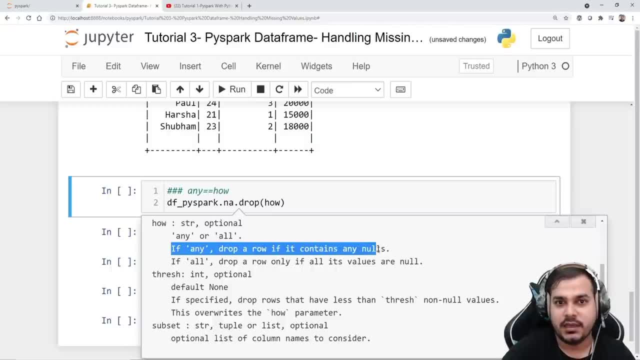 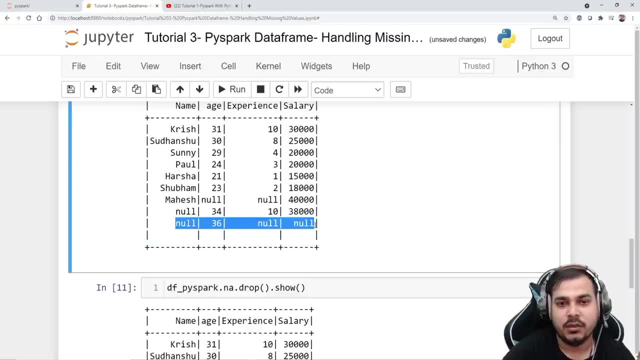 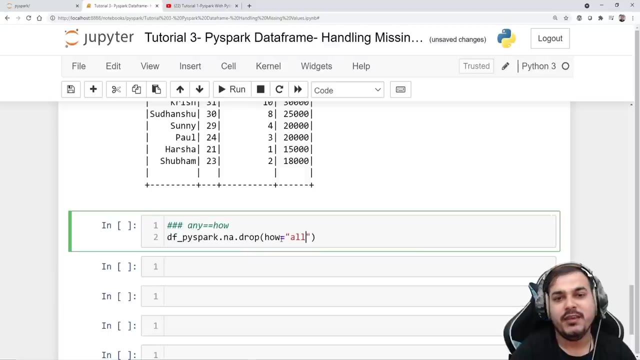 value selected as any drop or row. if it contains any nulls, like even though there is just one null, okay, one null, or there is two nulls, or there is entire nulls, you know, then by default it is going to get dropped. okay, but how is equal to all? when do we use all? that basically means suppose, if in 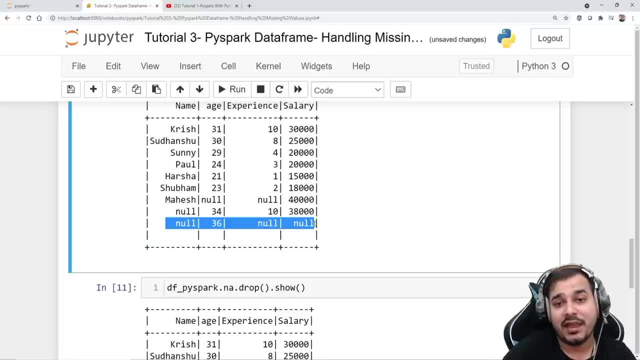 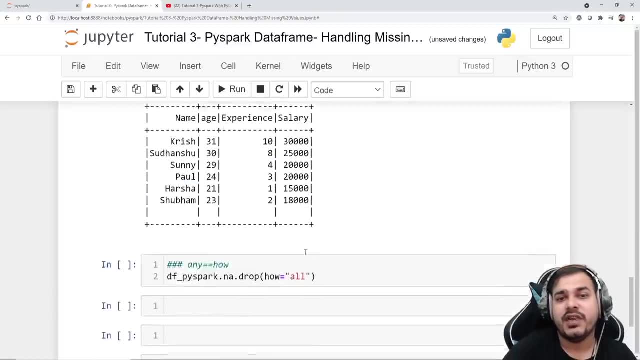 your feature you have. suppose if in your row you have all the values as null- in this case you have 36, one value- this will not get dropped. but if in a record you have all the values and null, then only it will get dropped. okay, so let's see whether this will work or not. definitely it's not going to work. 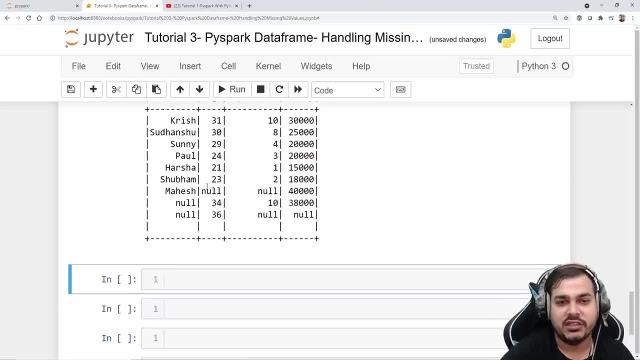 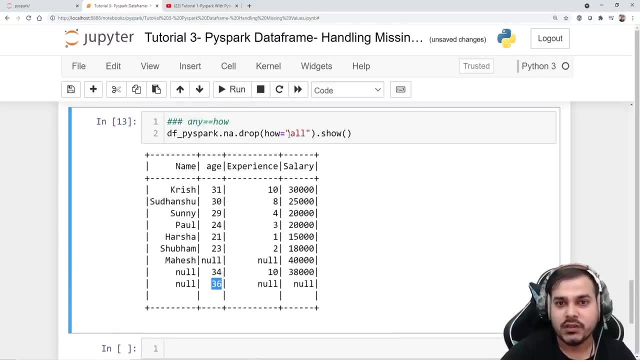 because i know all at least one values are at least there. see over here one values, uh, one one value. one non-null value is always there, right? if i'm using how is equal to all, it is going to drop those records, which is how is equal to all. 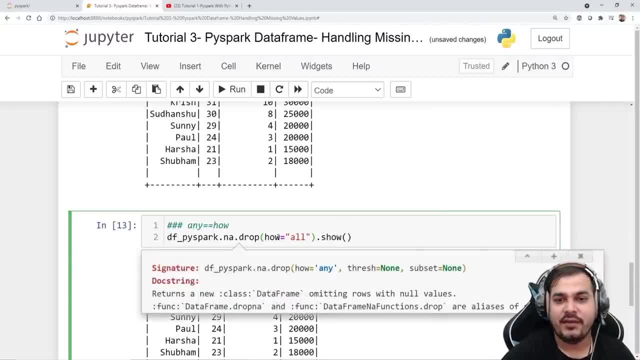 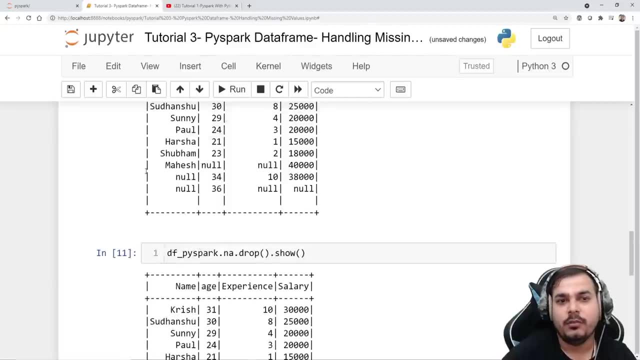 having completely, not by default. this how value should be having any right, so by default, it is any any. basically says that whether there is one null or two null, you are just going to drop it. drop those specific records, right. pretty much simple. this was what how was. now let's go ahead. 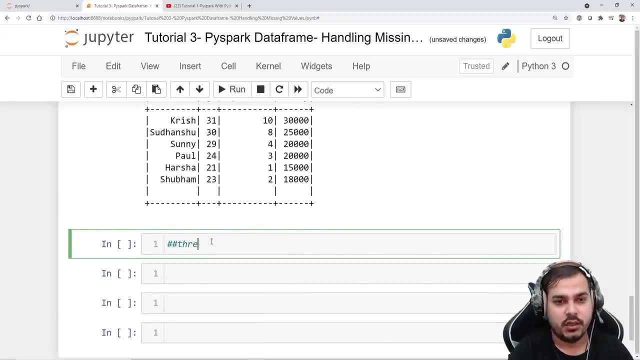 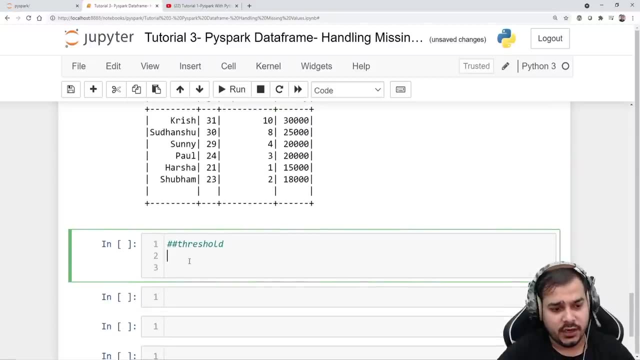 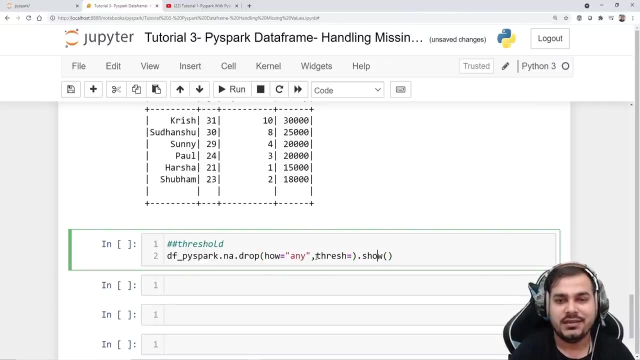 and try to understand with respect to threshold. what is this threshold? i'll tell you what is this threshold. now let me just use this. okay, i know how is any, but there is another one more option called as thresh. now, in thresh, what we do is that, suppose, if i write: let's keep the threshold as two? 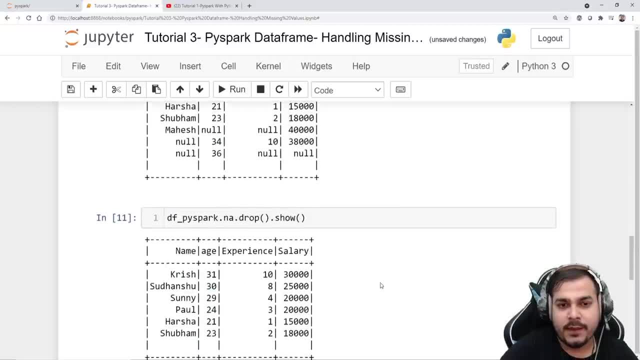 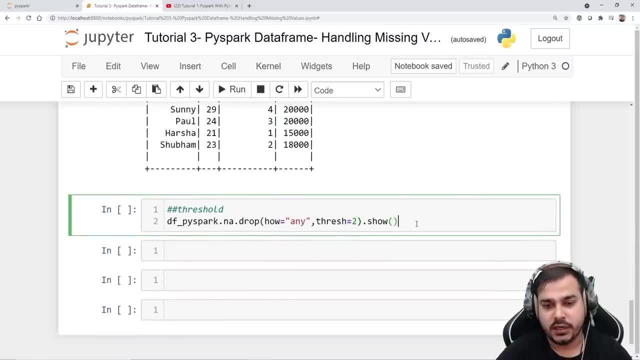 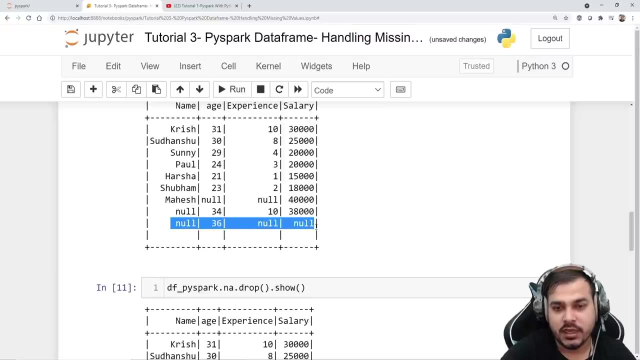 it basically says that suppose over here, in this particular case, if the threshold value is two, okay, let's. let's first of all execute it. you'll be able to see that the last column has got deleted over here. okay, the sorry, last row has got deleted. why it has got deleted? because we have kept the. 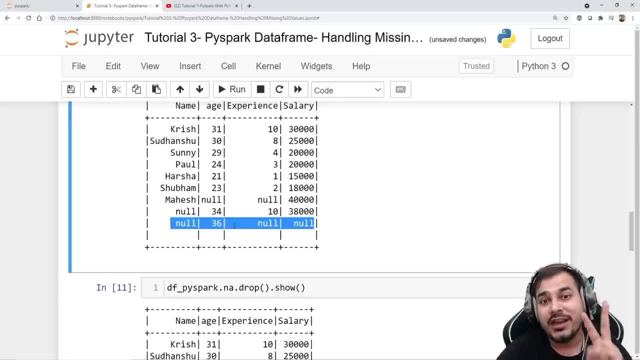 threshold value as two. it says that at least you have to keep the threshold value as two, so let's go ahead and do that. so at least two non-null values should be present. okay, at least two non-null values. now, here you have two non-null values like maish and forty thousand. okay, here you just have. 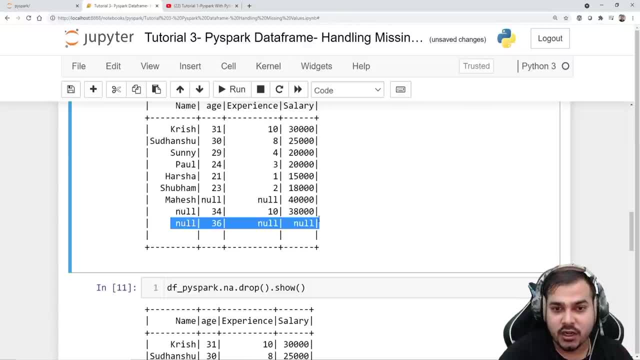 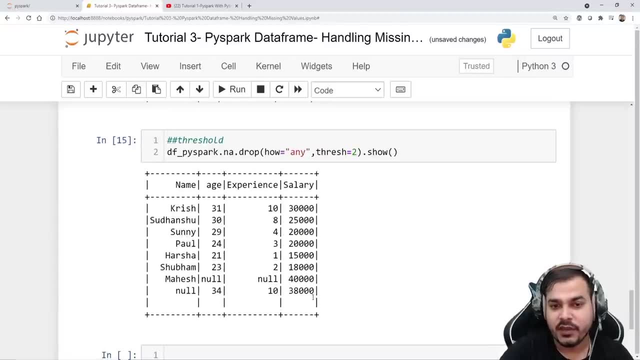 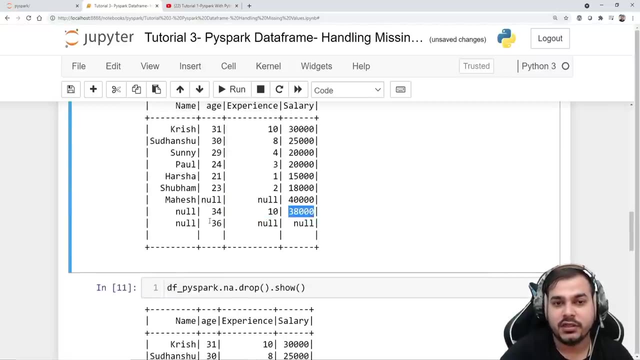 one non-null values. so because of that, it got deleted. suppose, if you had two non-null values over here, see 34 and 10, this is not got deleted. this is same over here: 34, 10, right, 34, 10. uh, you have. uh, if i go and show you 34, 10 over here and 38 000, they have at least two non-null values. 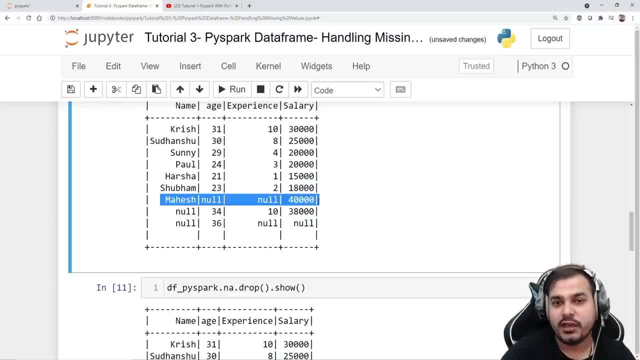 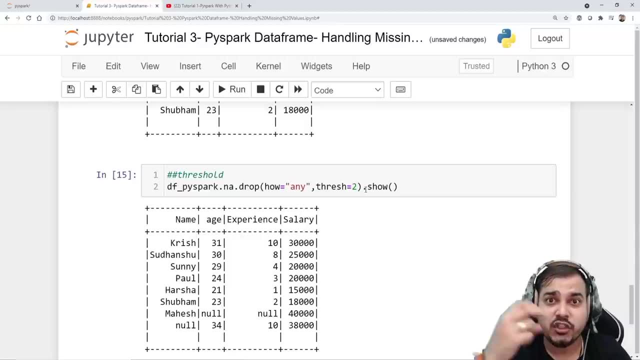 here you add three non-null values. here you add two non-null values. so here, whenever we give some threshold value as two, that basically means it will go and check whether in that specific row at least two non-null values are there. if it is there, it is just going to keep that row. otherwise, 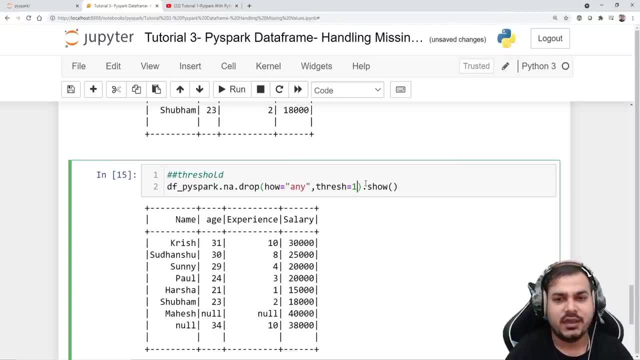 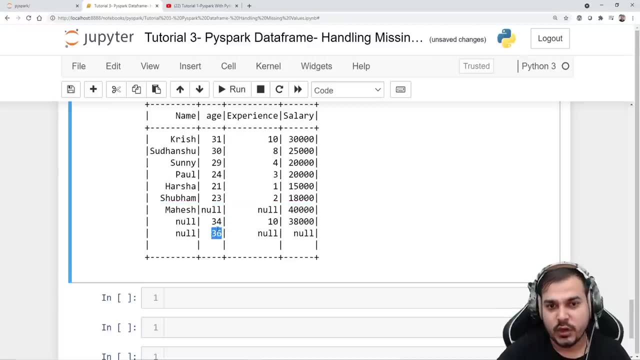 it is just going to delete it. that is what you can know. you can also check out with one. so if i go and see one, then you can see that all this particular rows are there, because it will just go and check. okay, here one non-null values are there. here it is there. if i make it as three. 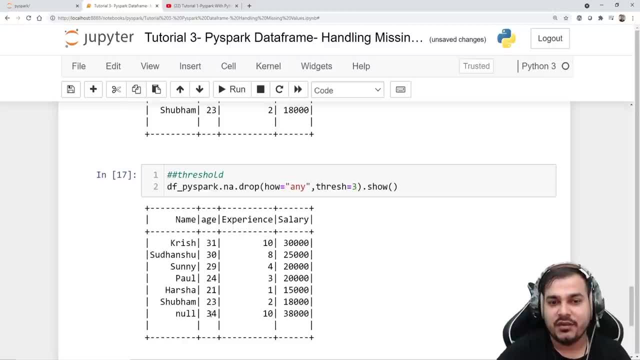 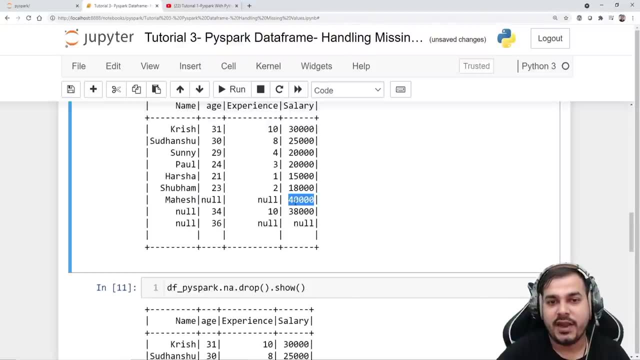 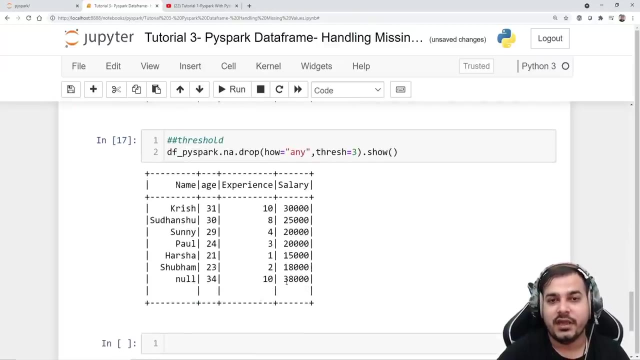 okay, let's see what it will come now. here you can see. at least this is there remaining. all has been deleted. right, see over here you had only two non-none values. here also here you add three. so this is there: 34, 10, 38 000 and null. so here you can see the value. that is the understanding with. 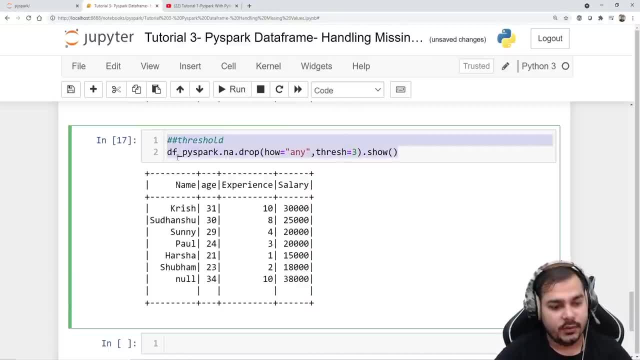 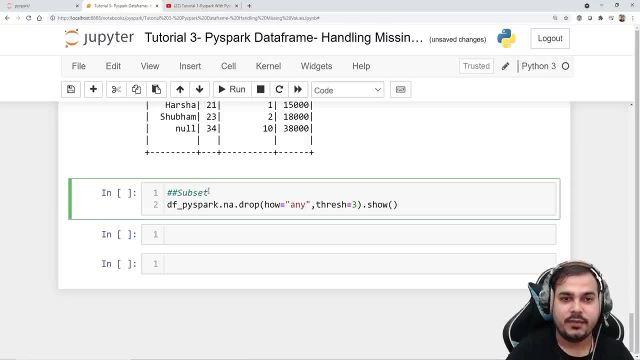 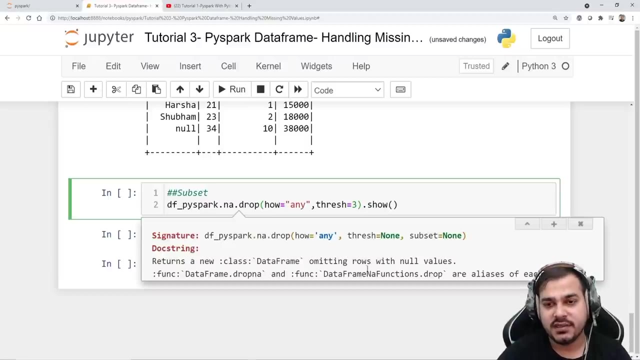 respect to threshold. now let's go ahead with the another one, which is called as subset. so here i'm just going to write it as subset, because this is the third parameter inside my drop feature. and remember these all features are pretty much simple with respect to, if you have worked with pandas, the same thing we are working over. 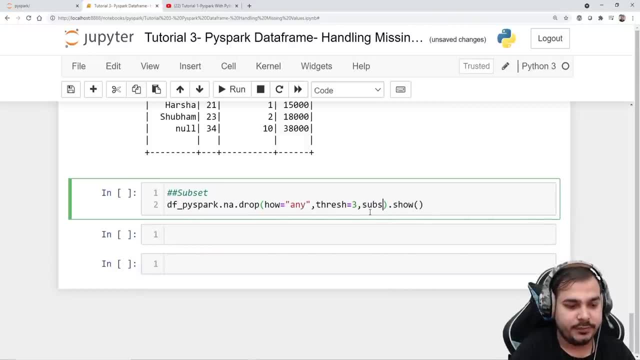 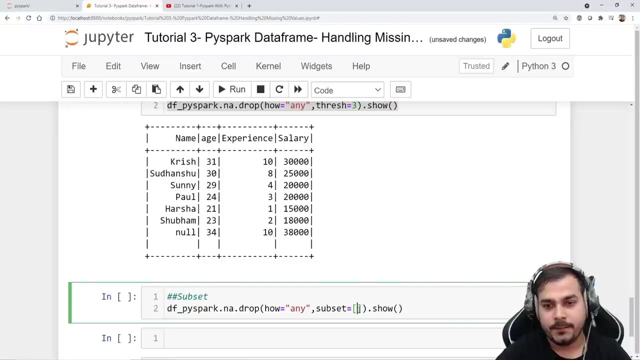 subset, in the subset we can actually provide. suppose i'll say in the subset: let's remove threshold, i don't want to keep any threshold. let's say i just want to drop nan values only from a specific column, probably only from experience column. then i can basically give. 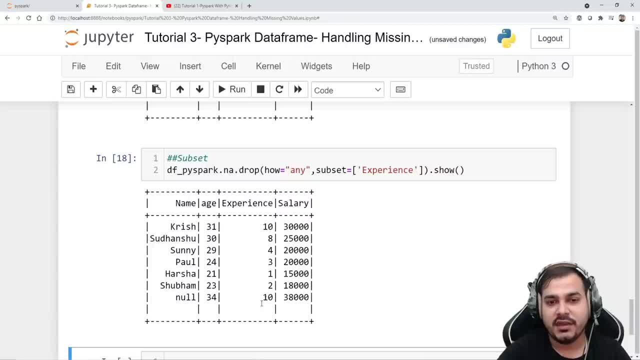 it as a subset. so from the experience column you can see that wherever there was nan values in the records, all those, that whole record has been deleted right. so like this you can apply with respect to this- suppose you want to apply it in age- you can also apply this right. wherever there was nan values, that whole record. 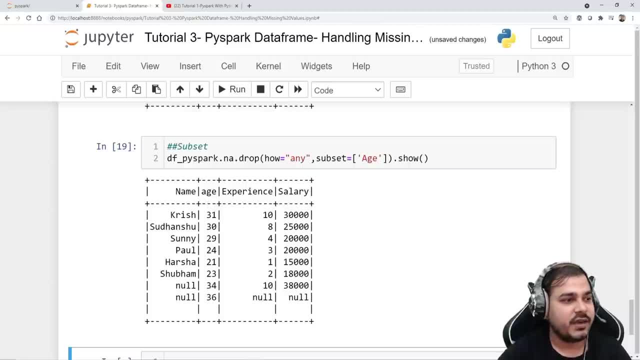 has got deleted in the age column also. so this is with respect to subset. so i hope you are getting an idea, guys, this is pretty much good because the same thing we are trying to do right we we are actually trying to apply whatever things we actually did in pandas, and this is very, very. 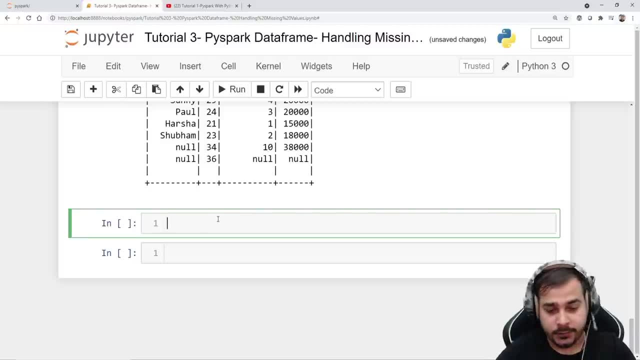 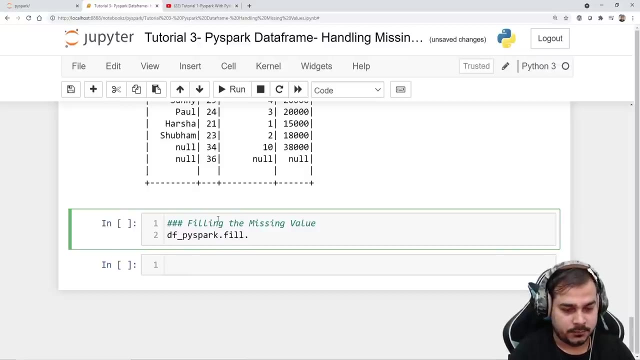 when you are working with missing data. okay, let's go with the next thing now. let's go and fill the missing value. filling the missing value now. in order to fill the missing value again, i'll be using df by spot: dot fill, dot. okay, sorry, na dot fill, okay. and inside this, this fill will take. 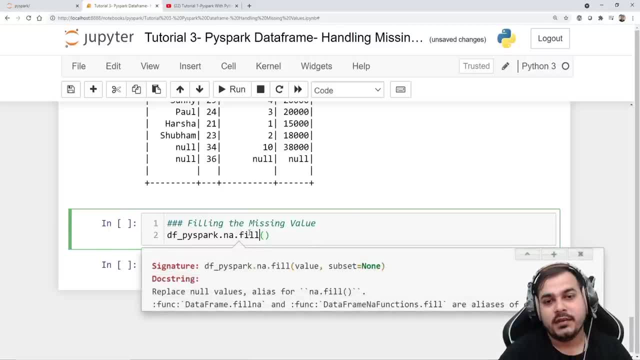 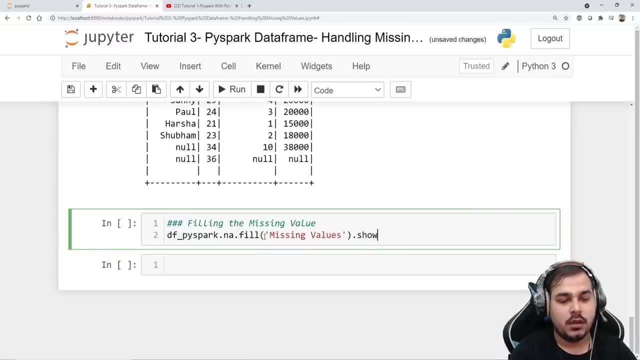 two parameters: one is value and the one is subset. okay, now suppose, if i go and give value like this, suppose i say missing value, and if i go and write dot, show then what it is going to do: wherever there is a nan value, it is just going to replace with missing values. so here you. 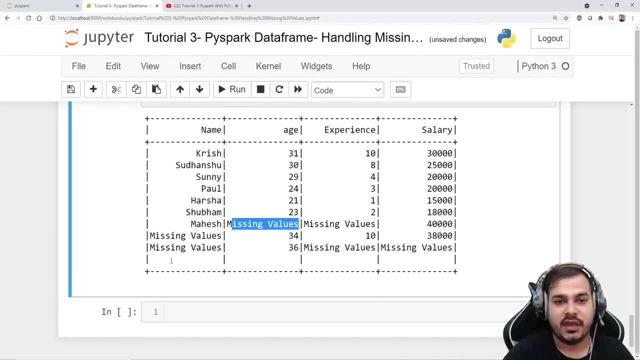 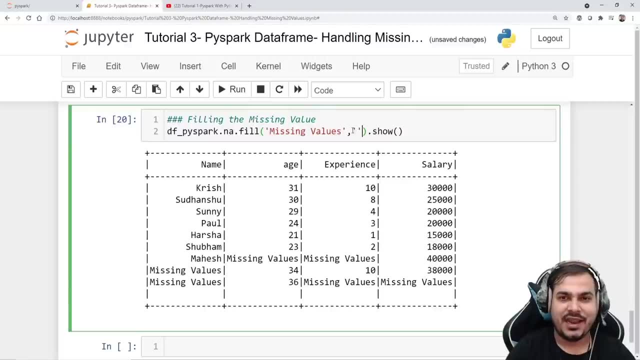 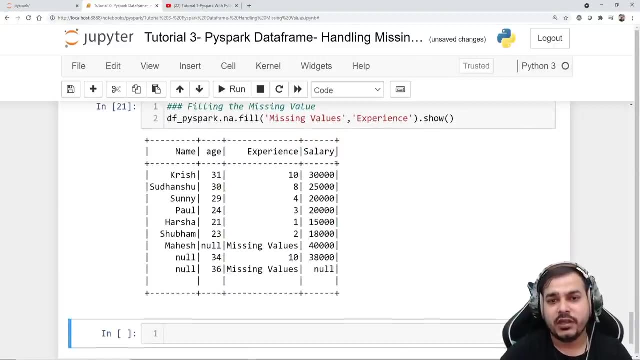 can see here, the null value is there. so missing value, missing value, missing value, suppose. if you really want to perform this missing value handling in only a specific column, then you can basically write your column name also like this. so this will be my subset. okay, i can also give multiple. 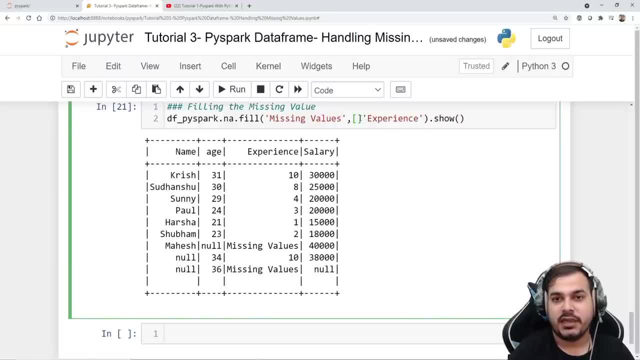 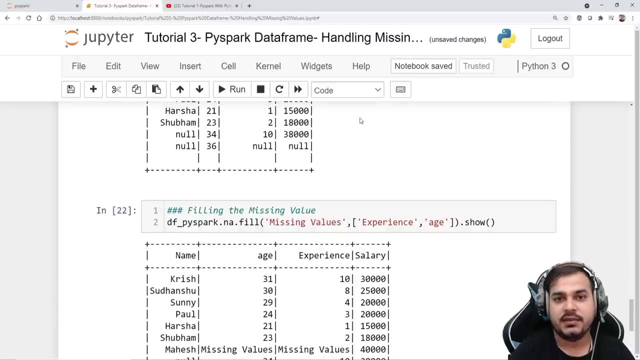 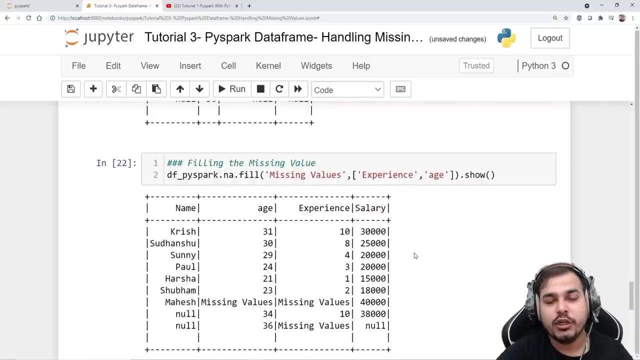 like this: see, i can also give multiple like experience comma, probably age comma, age in call in list right. when i give like this, then it this kind of functionality will happen in two columns, right. pretty much simple. so, guys. now next step. what we are going to do is that. 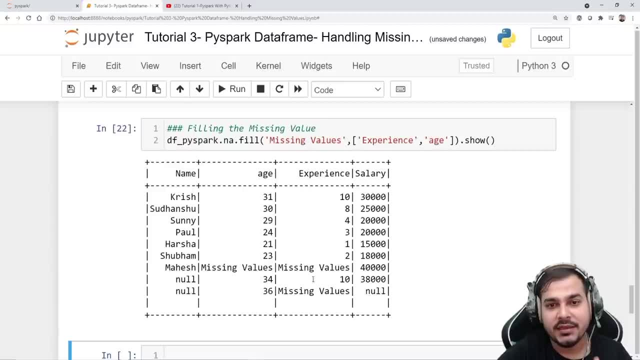 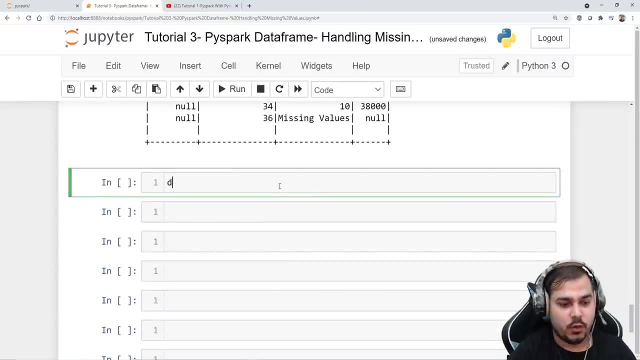 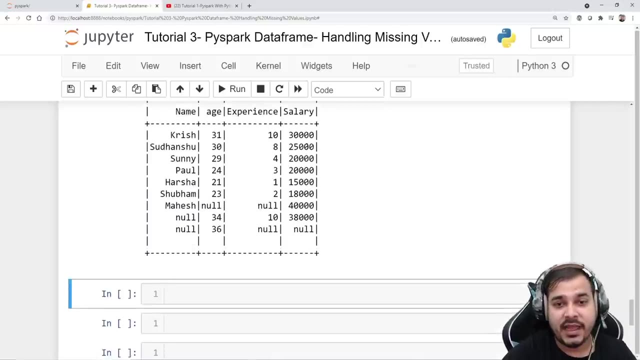 we are going to take a specific column and probably we are going to handle the missing values with the help of mean of that specific column or median of that specific column. so right now, if i go and check out my df dot spy spark here, if i go and see my dot show value, uh, this is my entire. 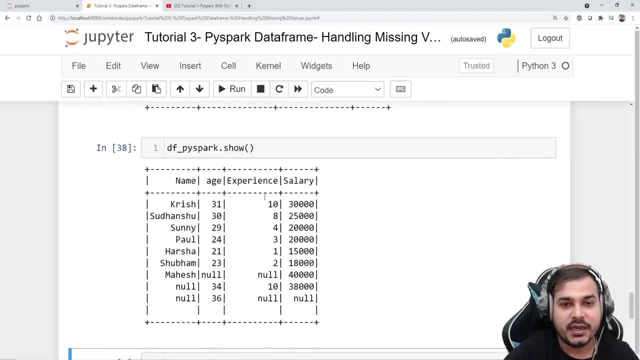 data set over here. now, what i'm going to do is that i'm going to take this particular experience column and probably replace the null values with the mean of the experience itself. so, in order to do this, i'm going to use an imputer function and, guys, if you know about imputer function, 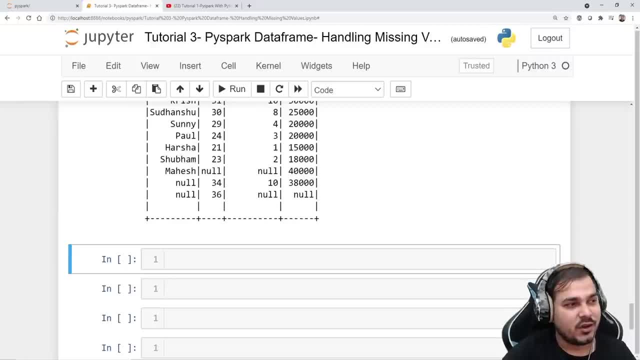 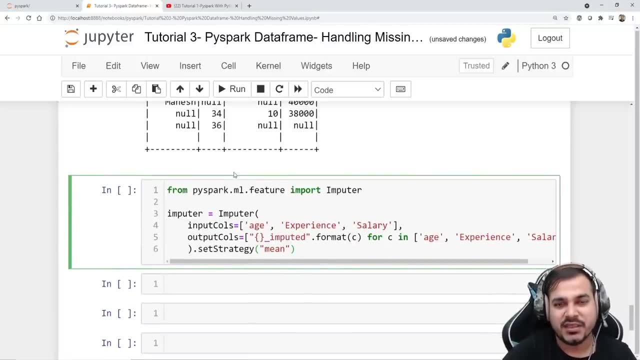 um, we basically use that with the help of this data set over here and we're going to take this model with the help of sklearn also. in pi spark also, we have an imputer function, so i'm just going to copy and paste the code over here to make it very, very much simple. from pysparkml feature. 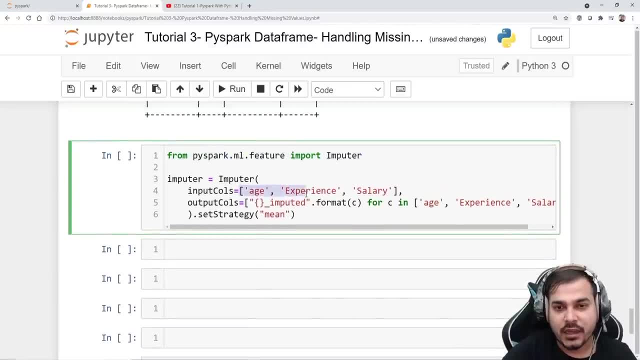 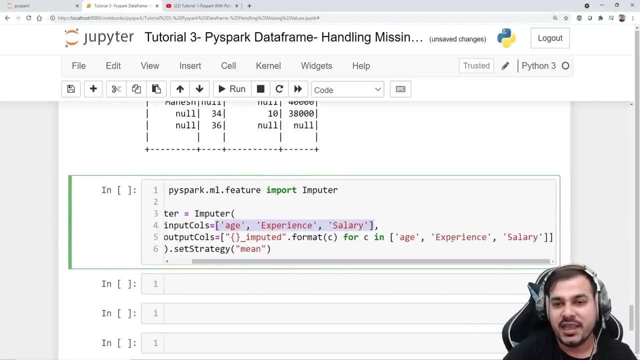 import imputer here i'm just going to give my input columns, that is age experience salary. probably i want to apply for every column over here and then i'm just saying that for age experience salary. i'm just going to find out this dot formatc output columns and then i'm going to keep the strategy as mean you can also. 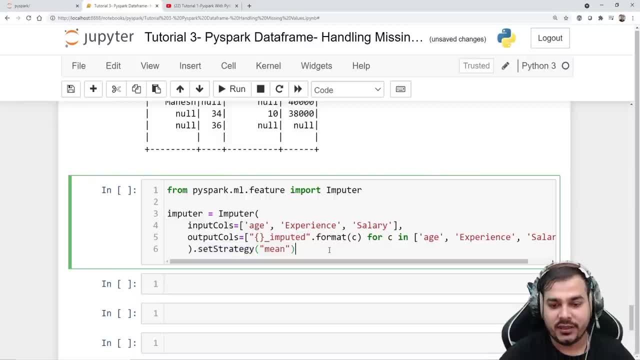 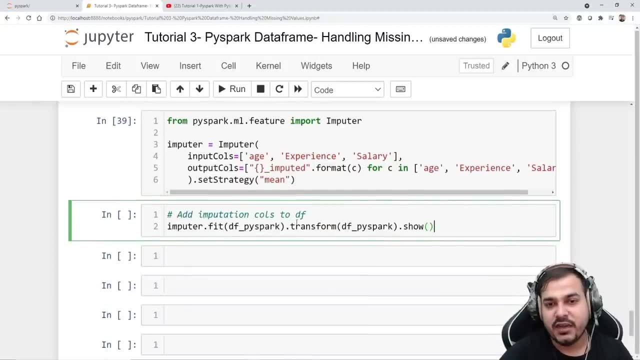 change the strategy just because you're already in the pipeline mtl. so i'll keep the strategy as men, as median mode and everything. so i'll execute this. this has got executed fine, and then we are just going to write fit and transform. so imputed or fit df of pi spark dot transform. so once i. 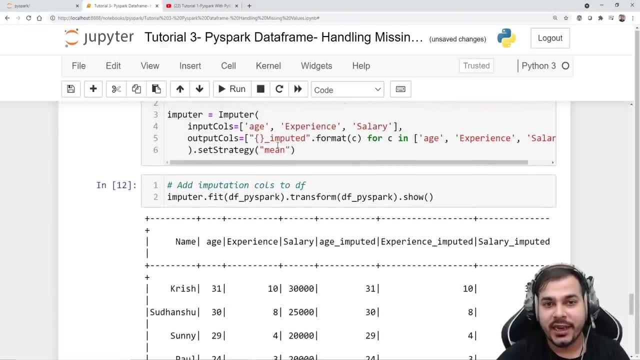 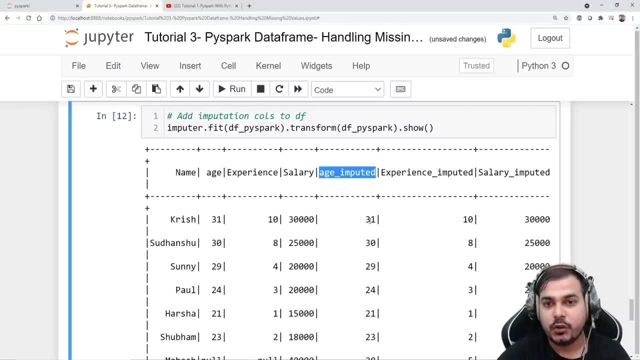 execute this, guys. here you'll be able to see that we are going to create multiple columns with underscore imputed as this name. so here you can see age underscore imputed. in short, what we have done. we have tried some kind of- uh mean functionality over here. that basically means the null value has. 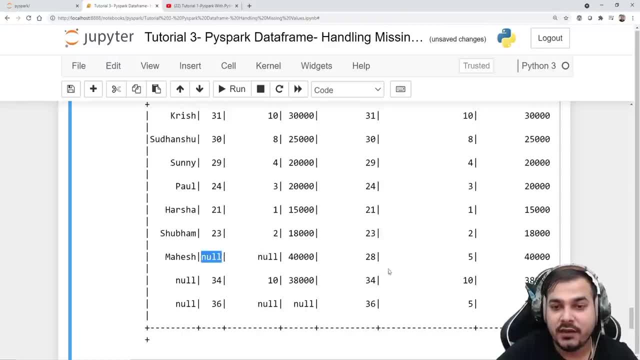 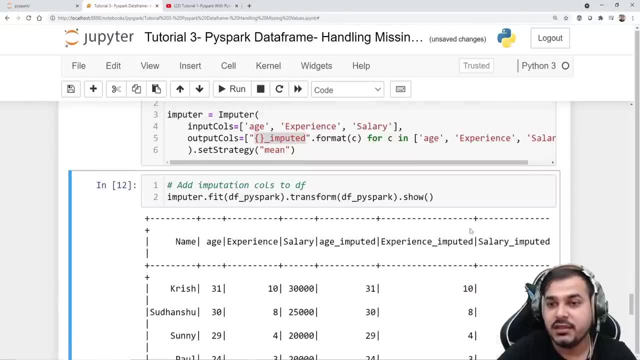 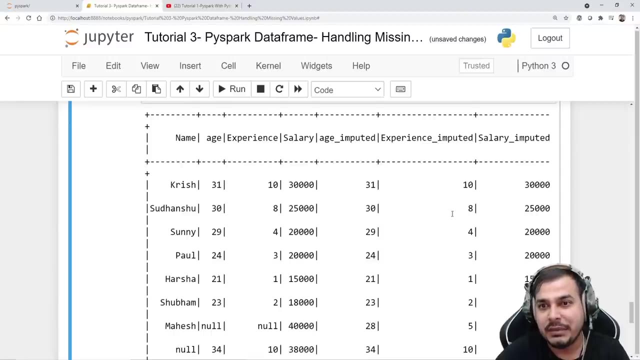 been replaced by mean. so over here you can see, this null value is replaced by 28. similarly, this two null value is replaced with 10 and 5. sorry, 5. this is what is the experience imputed column. over here you'll be seeing that wherever there is a null value, it is being replaced by the mean of. 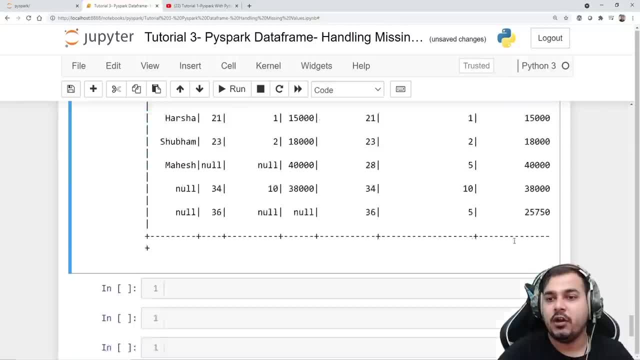 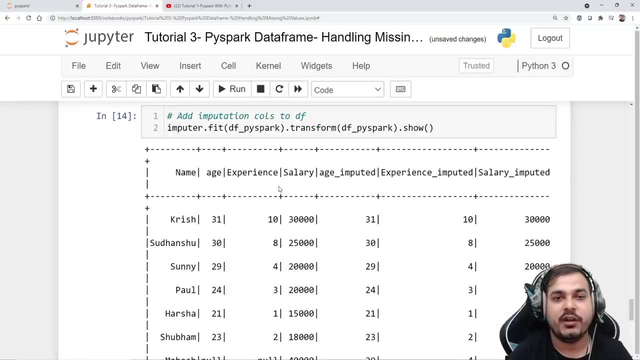 the experience column, the mean of the age column and mean of the salary column. and this way you'll be able to do it. if you really want to go ahead with median, just go and change this mean to median and just try to you execute it here. now you'll be able to see the median value. and here is your initial null columns. 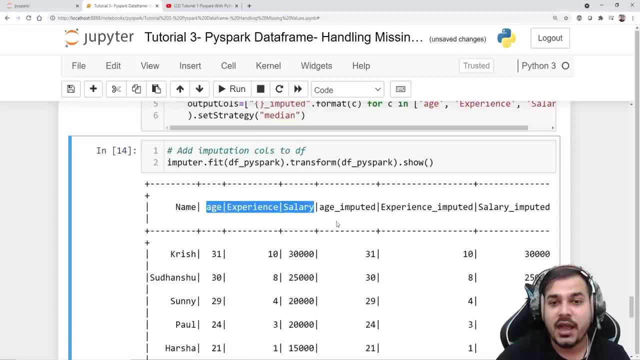 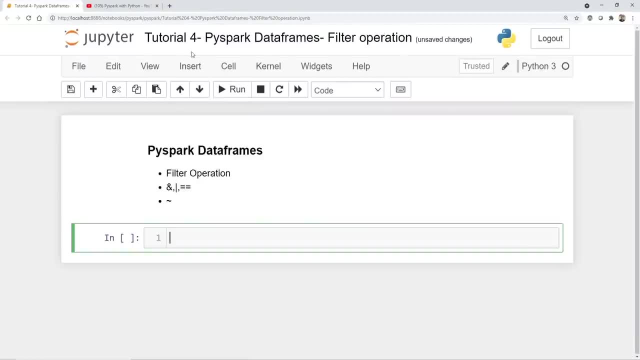 which have- sorry, here are the columns which has null values and here are all the columns which has basically the imputed values right with respect to mean median. so, guys, today we are in the tutorial for of pi, spark data frames, and here, in this particular video, we are going to discuss 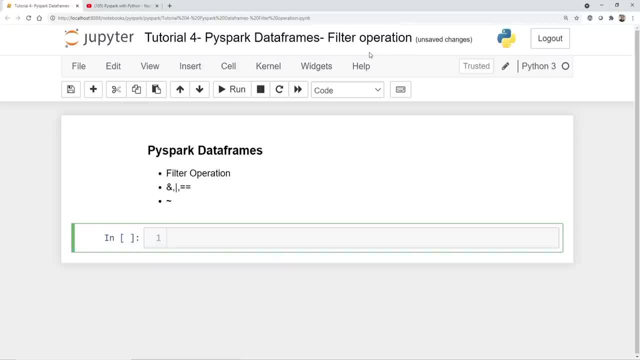 about filter operation. a filter operation is pretty much important for data pre-processing technique. if you want to retrieve some of the records based on some kind of conditions or some kind of boolean conditions, we can definitely do that with the help of filter operation. now, guys, please make sure that you follow this particular playlist with respect to 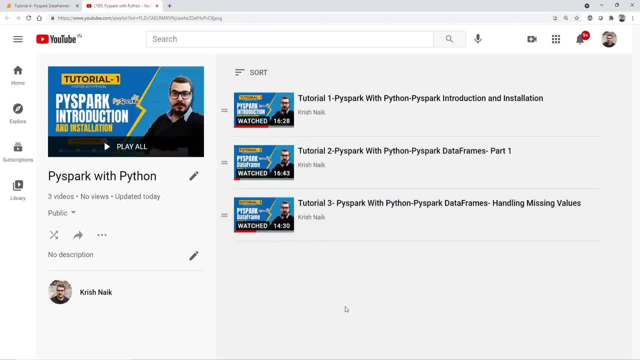 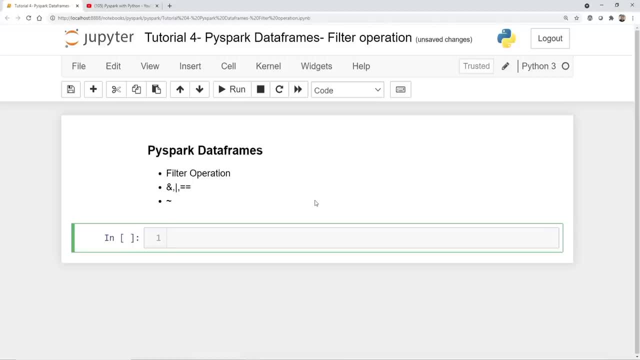 pi spark. i will be uploading more and more videos as we go ahead. and remember one more thing: there was a lot of complaint from people telling to upload sql with python. don't worry, parallelly i'll start uploading sql with python. i'm extremely sorry because of some delay, because i was doing. 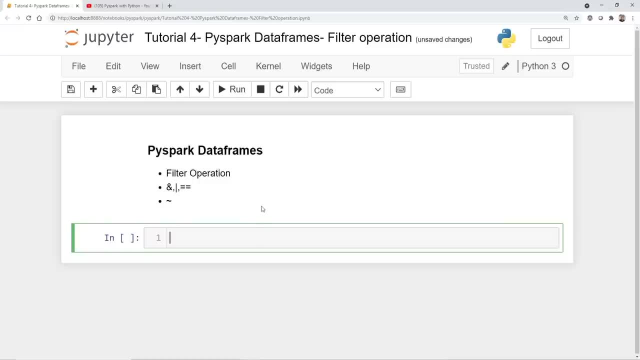 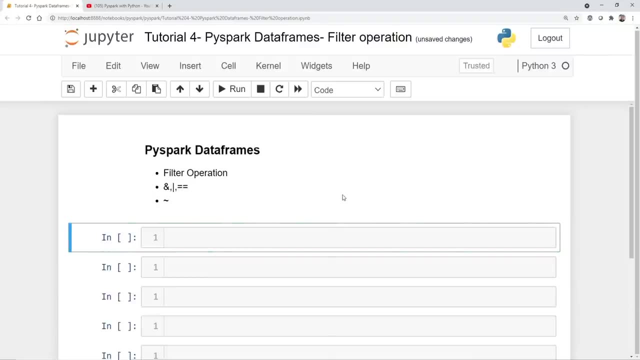 some kind of work, busy with something, but i'll make sure that i'll try to upload all the videos so parallelly. sql with python is going to be a lot of work, so i'm going to try to upload all the videos. so let's proceed now. first of all, let me go and make some cell now, today. for this i've taken a. 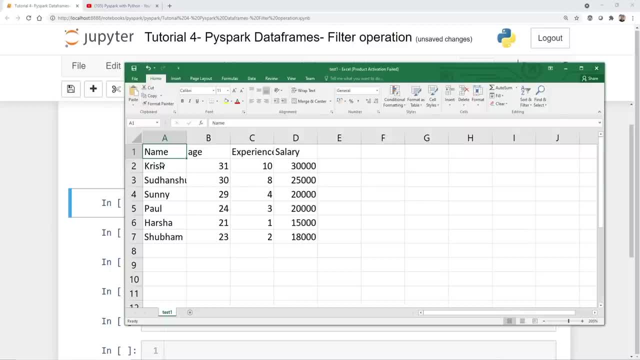 data set, a small data set which is called as test1.csv. here i have some data set like name, age, experience and salary, and i'm just going to use this and try to show you some of the example. with respect to filter operation, initially, whenever you want to work with pi spark, you have to make 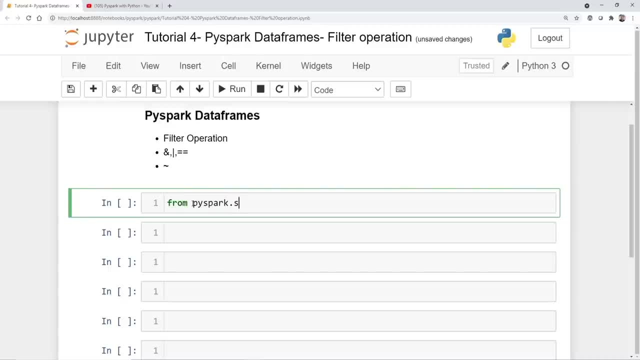 sure that you install all the libraries, so i'm going to use pi sparksql. import spark session. actually help us to create a spark session, right, and that is the first step whenever we want to basically work with uh uh, pi spark, right, so we'll be using spark session. dot builder, dot app name. 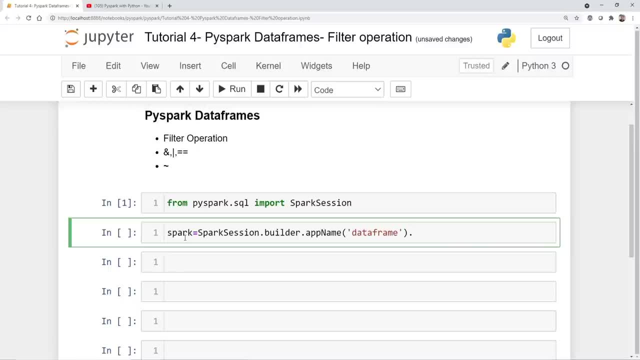 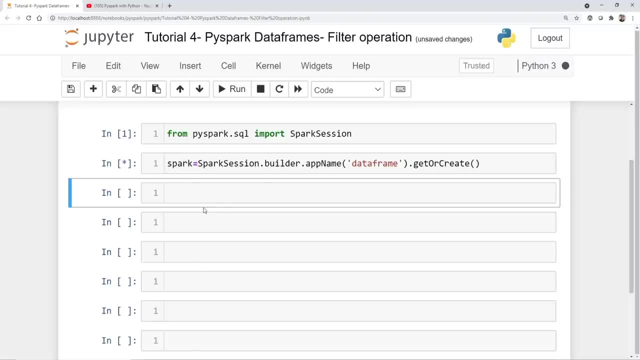 uh, then i'm just going to create my app name as data frame and basically write get or create function, which will actually help me to quickly create a spark session. i think this is pretty much familiar with every one of you. now let's proceed and let's try to. 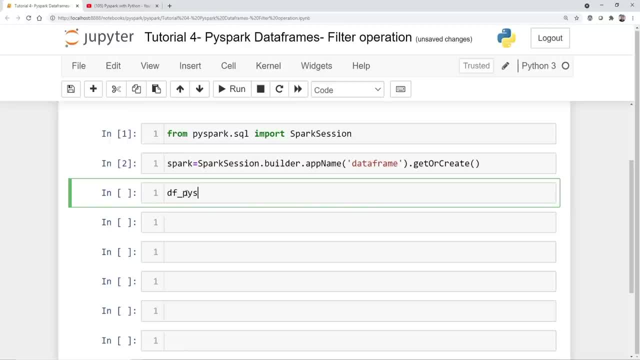 read a specific data set. so over here what i'm going to do, i'm just going to create a variable, uh, df, underscore pi, spark, and i'm going to use the spark variable, dot read or dot csv. and here i'm just going to consider my data set, test1.csv. and uh, here i'm just going to make sure. 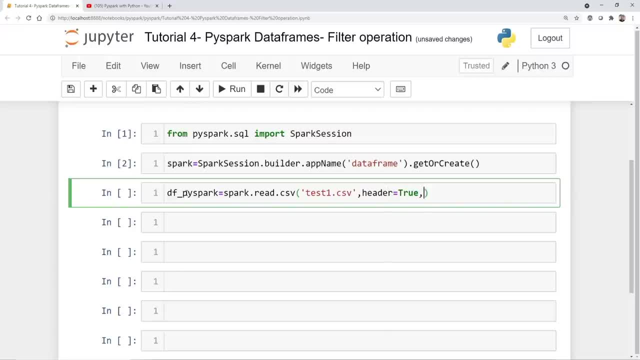 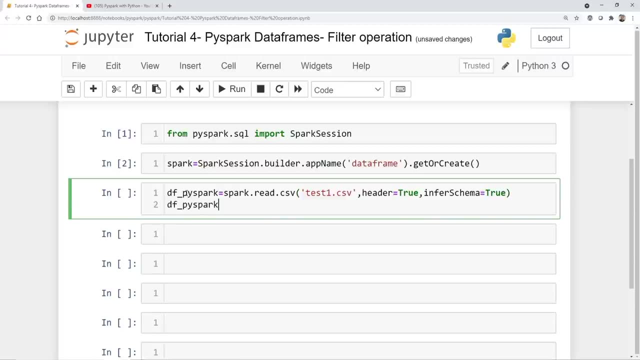 that we have this particular option. selected header is equal to true and infer schema is equal to true. i think this all i've actually explained you. you can see that i've actually explained you and i've actually explained you and i've actually explained you and i've actually explained you. then if i write dfpl. 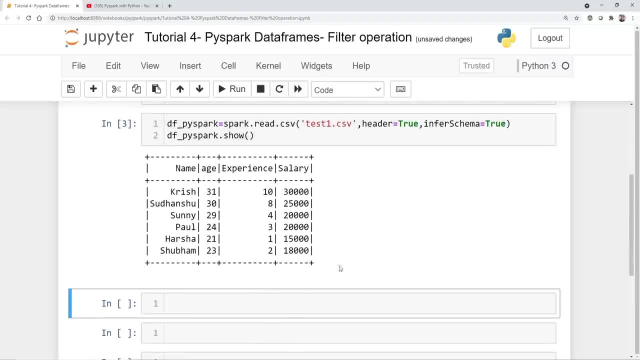 your dataset. okay, so it is reading Veggie die output. now, guys, as i showed you that we will be working on filter operation and we try to retrieve some of the records based on some conditions, remember filters also are available in pandas. but there you try to write. 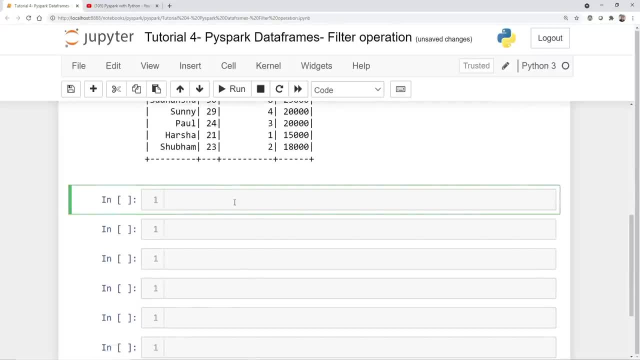 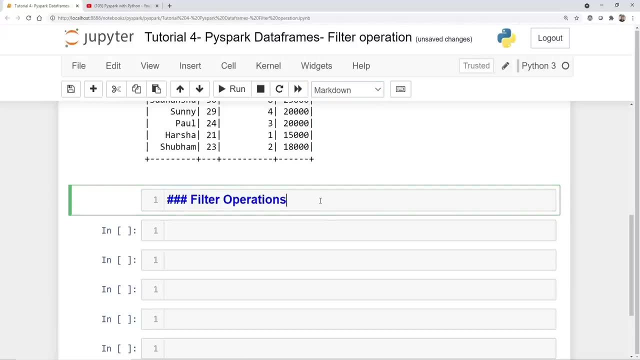 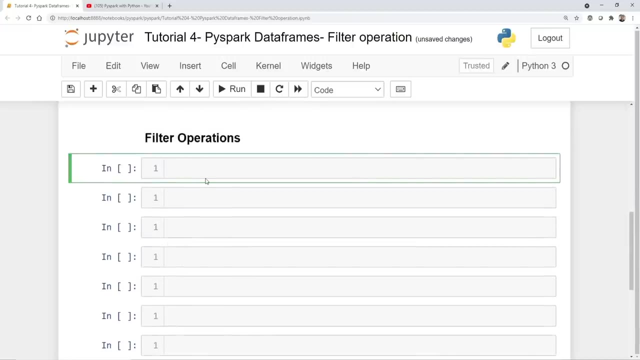 in a different way. let me just show you how we can perform filter operation by using by spark. okay, so filter operations. let me make this as a markdown. so it looks big, it looks amazing. uh, let me make some more cells. perfect now, first step: how do i do a filter operation? 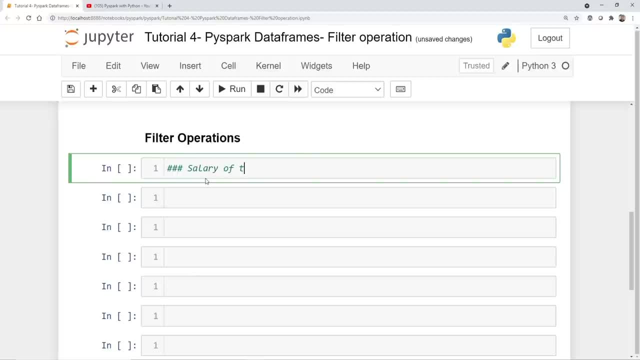 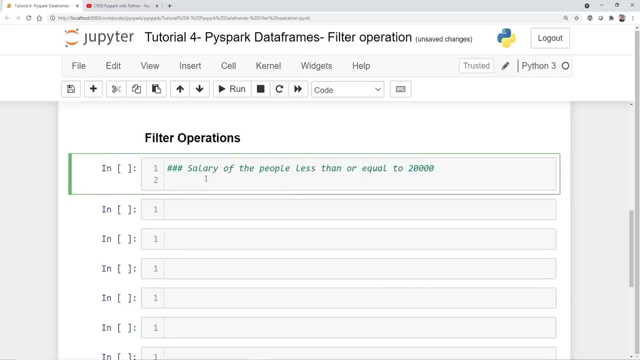 suppose i want to find out salary of the people who, less than probably 20 000- okay, less than or equal to 20 000 again write like that: less than or equal to 20 000. now for this there are two ways how we can write it. first way, i'll just try to use the filter operation, so you have like dot. 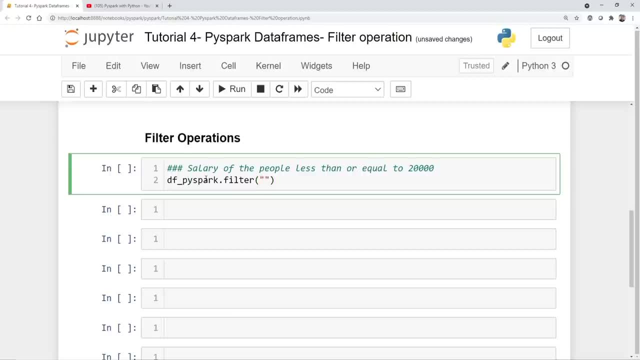 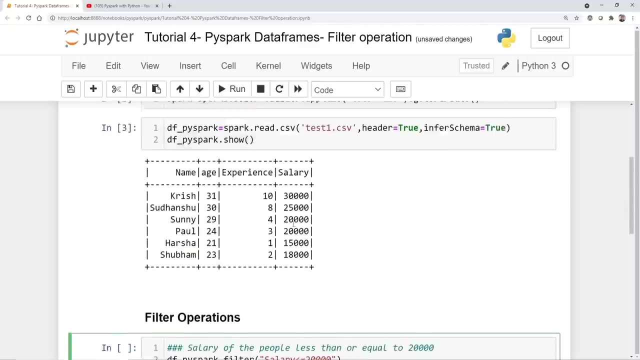 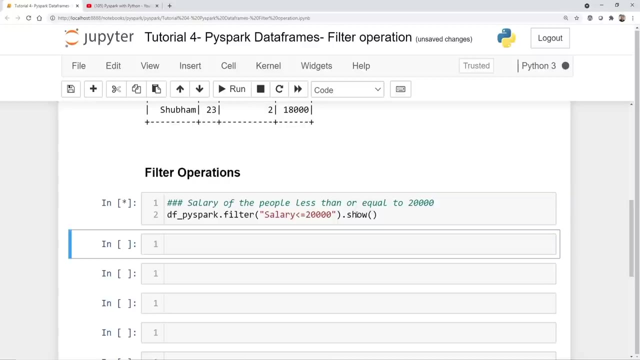 filter and here you just have to specify the condition that you want. suppose i'll write: salary is less than or equal to 20 000. remember this salary should be the same name of the column over here right, and when i write dot show, you will be able to see this. specific records and. 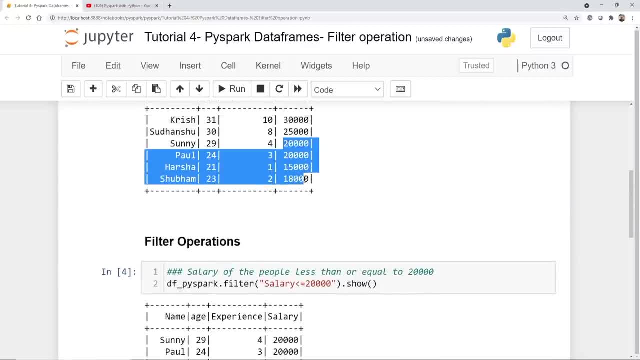 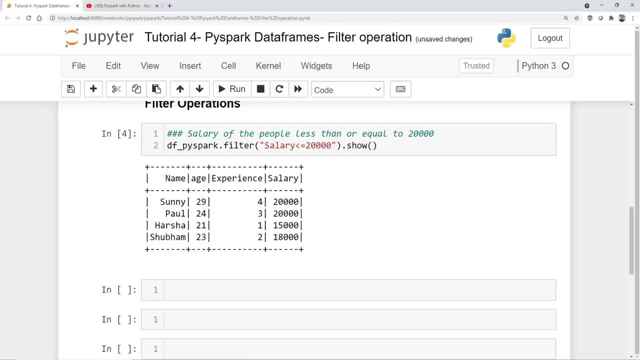 you'll be able to see. okay, less than or equal to 20 000 is this form for people: sunny, paul, harshan. so here you'll be able to see all these things along with experience. right now, this is one way, probably. i just want to pick up. uh, after putting this particular condition, i want to pick up two. 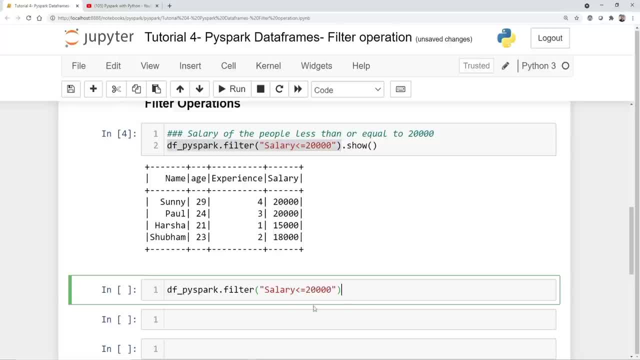 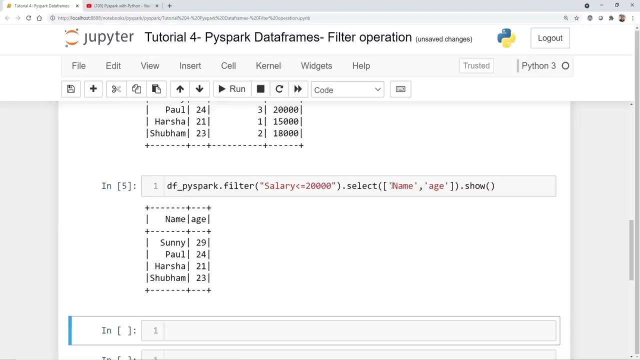 columns. so what i can do. i can use this and then i can basically write dot select, and here i'm going to specify my name. probably i want the name and age, name comma, age, so dot show. i'll do this now. this is how you can actually do it again. over here you can see that name underscore age is. 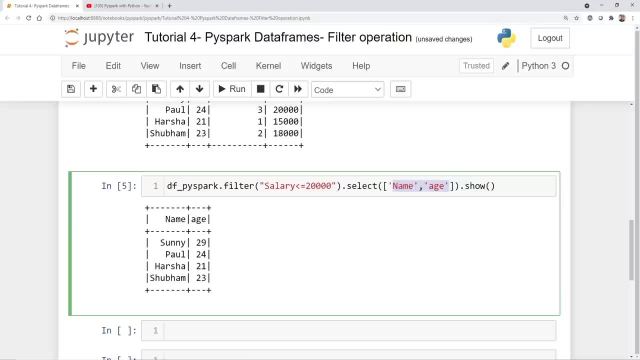 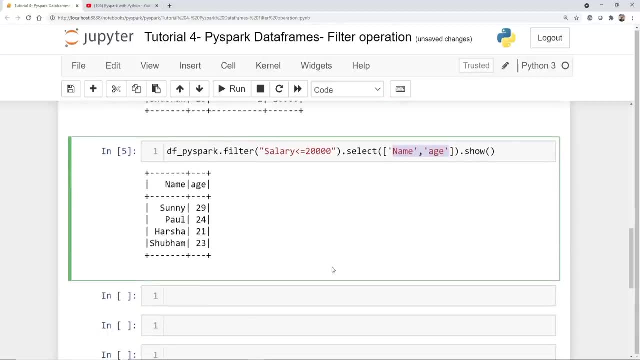 actually there and you are able to get that specific information after this. uh, probably i want to do some of the operation. you can actually do less than greater than whatever things you want. probably i want to put two different conditions, then how should i put it? let's see, let's see for. 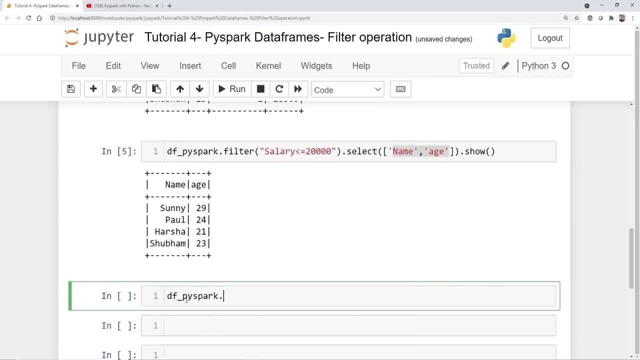 that also. so i'll write d by uh df pi spark dot filter. and here i am going to specify the condition. i'm going to specify my first condition, suppose? uh, this is one way. uh, this is one way by using filter operation also. guys, and this conditions that i'm writing. i can also write something like: 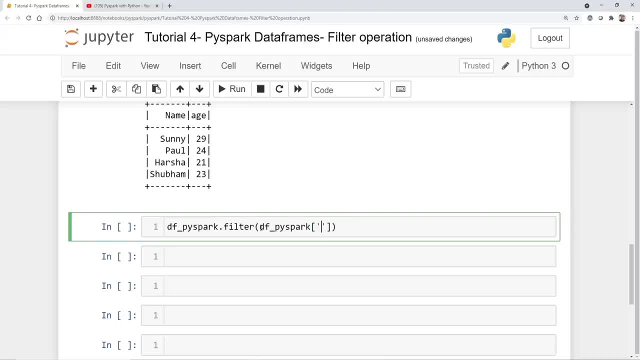 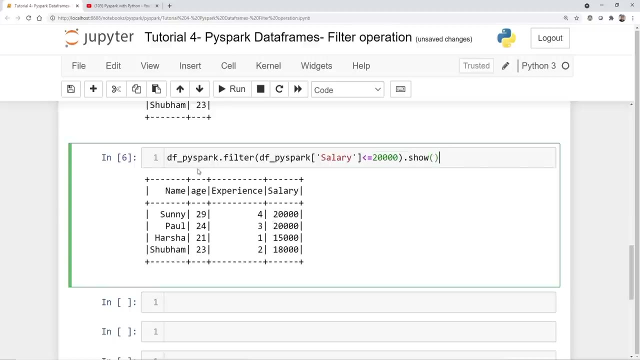 this. see this: suppose: if i write df pi, spark of salary, suppose salary is less than or equal to 20 000, i can also write like this: i will also be able to get the same output. so here you'll be able to see the same output over here. now suppose i want to write multiple conditions. how do i write? 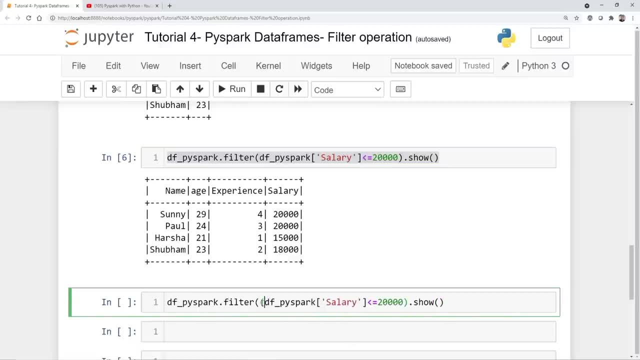 i will take this. this is first. this is one of my condition, so i'm just going to use this condition, and i can also use an and operation, you know, so i'll say and, or or any other kind of operation that you want. uh, probably, i want to uh say that df underscore pi, for salary is great, less than. 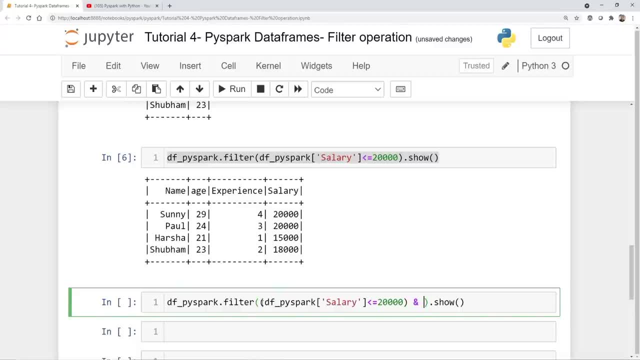 or equal to two thousand, um, twenty thousand, uh and uh, probably i want a df pi spark of salary- salary greater than or equal to fifteen thousand, so i'll be able to get all those specific records. okay, and again, i'll try to put this in another brackets. make sure that you do this, otherwise. 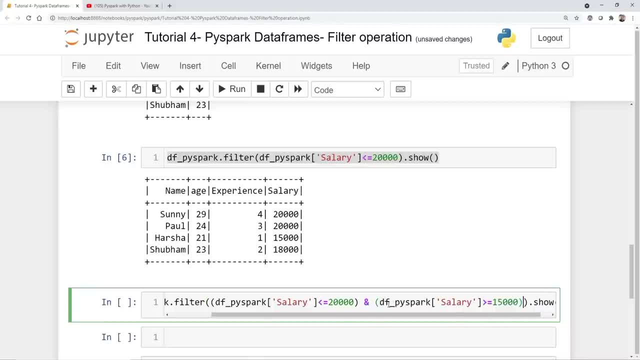 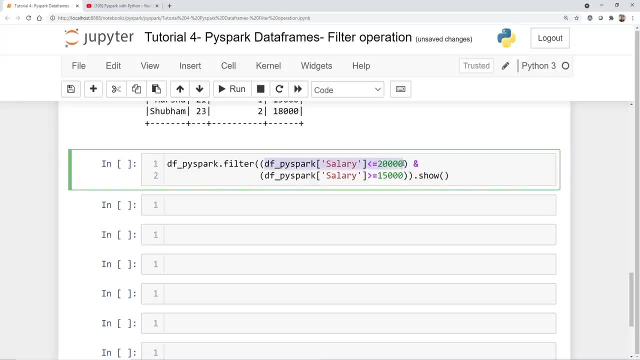 you'll be getting an error. okay, very, very simple, guys. so let's see how i've actually written. it is something like this: df underscore pi spark dot filter. df for pi spark of salary is less than or equal to twenty thousand, greater than equal to fifteen thousand. if i execute, you'll be able to. 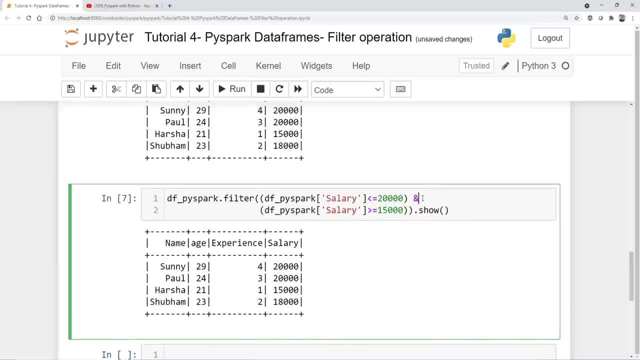 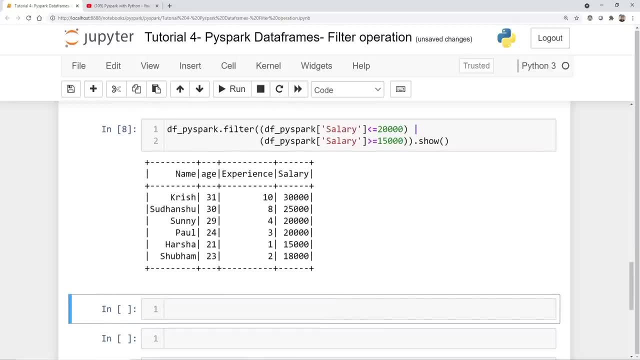 see between fifteen thousand to twenty thousand. you'll be able to filter it. so i'm going to find out. you can also write, or then you'll be able to get all the different, different values. now this is a kind of filter operation that you can basically specify. remember, this will be pretty. 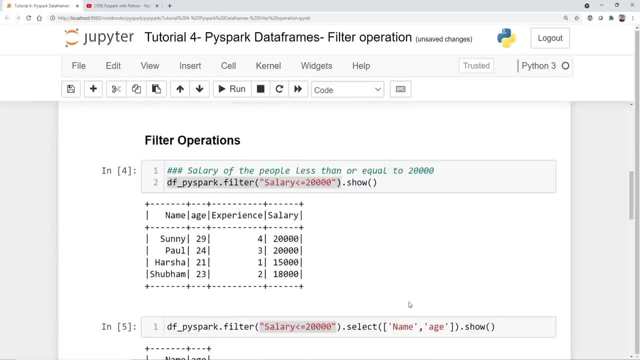 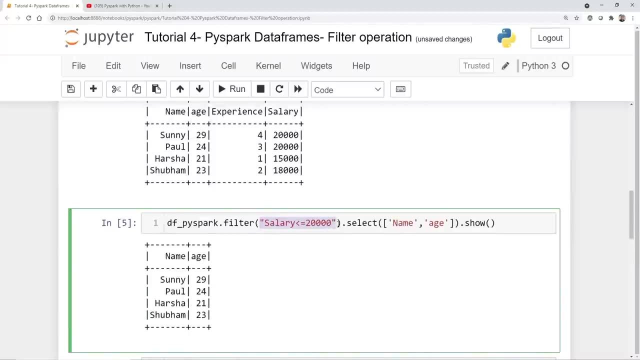 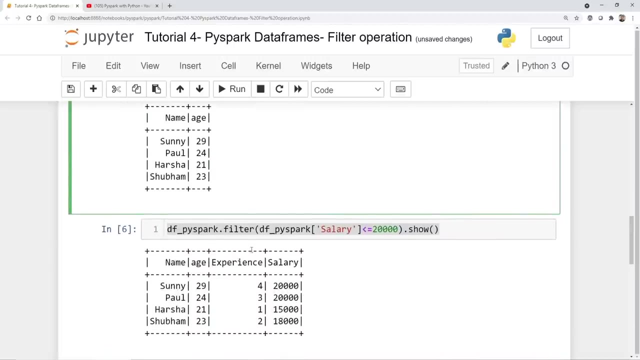 much handy when you are probably retrieving some of the records with respect to any kind of data sets, and you can try different, different things. see, this is one way where you are actually directly providing your column name, uh, and putting a condition internally. this pi spark- actually pi spark- data frame understands it and you'll be. 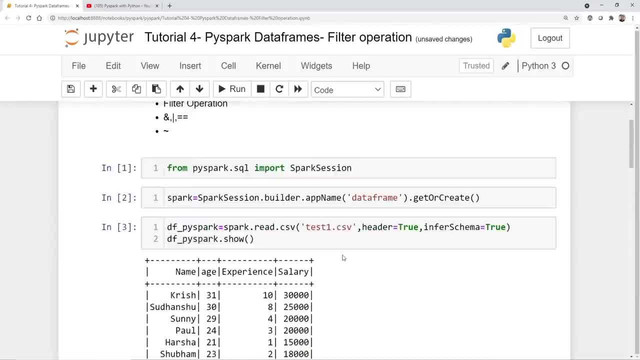 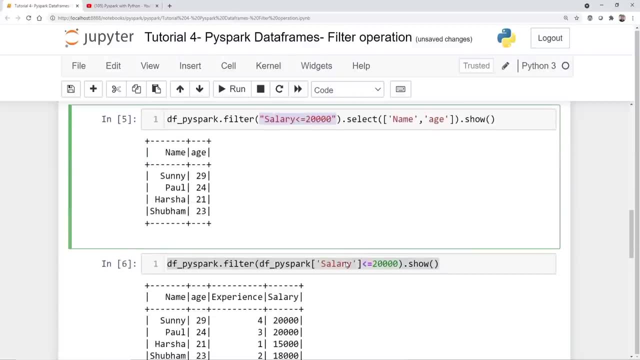 able to get the output right. so, yes, this was it all about this particular video. i hope you like it. i hope you like this particular filter operation. just try to do it, uh, from your side. okay, one more operation is basically pending. uh, i can also write like this. see this, everybody. i can basically say: 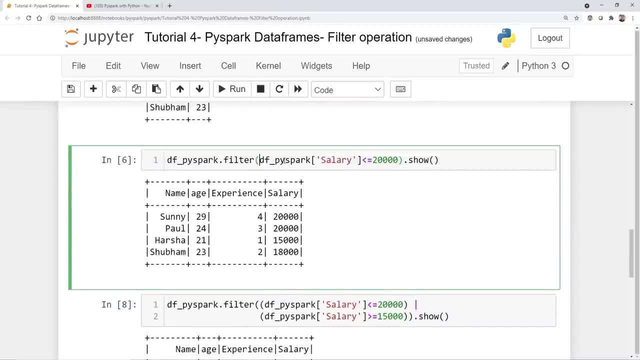 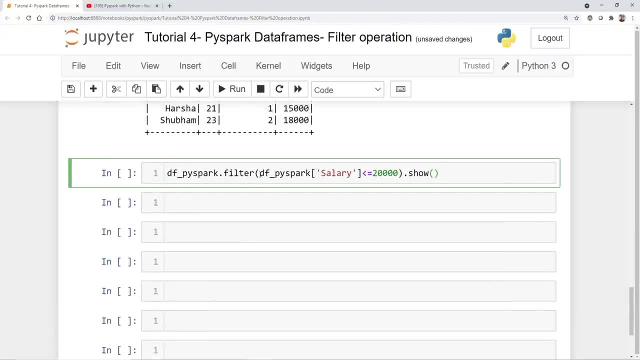 that okay, um, probably i can use this operation which is called as not operation. let's see how this not operation will be coming. okay, basically the inverse condition operation. we basically say: so i'll be using this, okay and this, and inside this i can put a not condition which like this. so i'll say this is a. 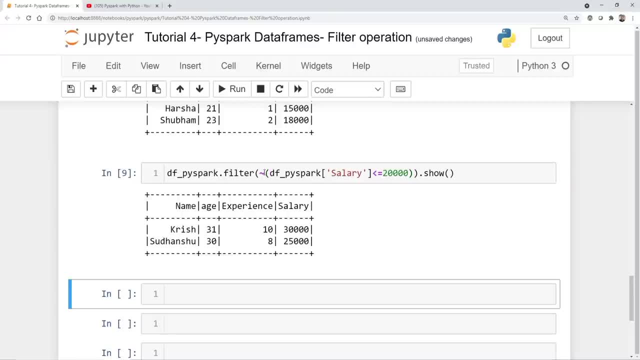 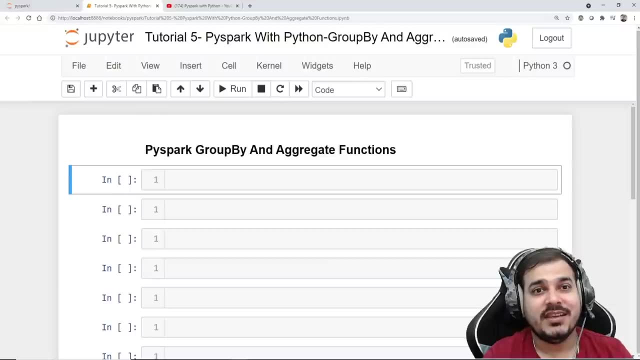 not of df, of pi spark salary is less than or equal to twenty thousand, so anything that is greater than twenty thousand will be given over here. okay, so inverse operation, you can say inverse filter operation. guys, we will be continuing the pi spark series and in this particular video we are going 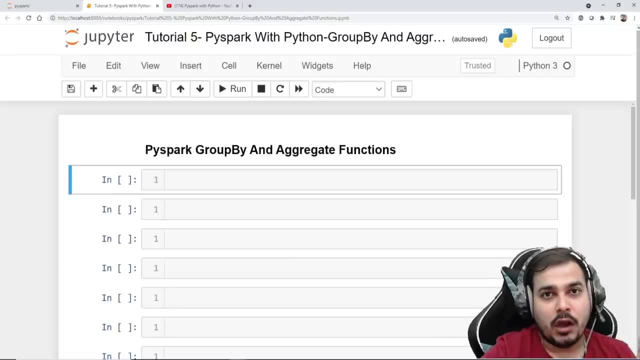 to see group by an aggregate function. already i have actually created somewhere around four tutorials on pi spark. this is basically the fit tutorial and again, this is a part of a data frame why we should actually use group by an aggregate functions again for doing some kind of data pre-processing. so let's begin for this particular data set for. 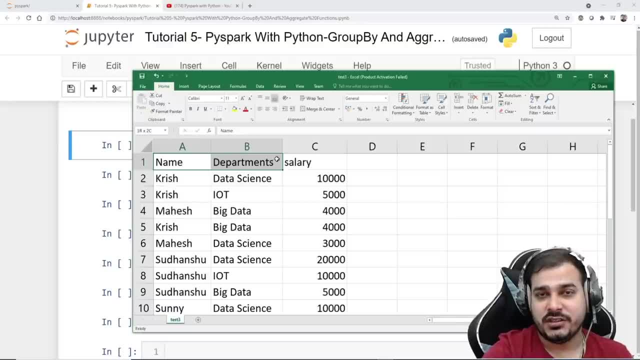 this particular problem. i've created a data set which has three features like name, departments and salary, and you have some of the data, like krish data science- uh, salary right, something like this. so over here, in short, if i want to basically understand about this particular data set. 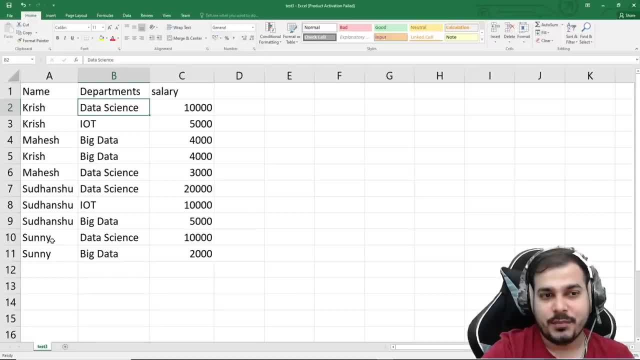 there are some departments probably where krish and other people teach and based on different, different departments they get a different, different salary. so let's see how we can perform different, different group by an aggregate functions and see how we can pre-process or how we can get some or retrieve some kind of results from. 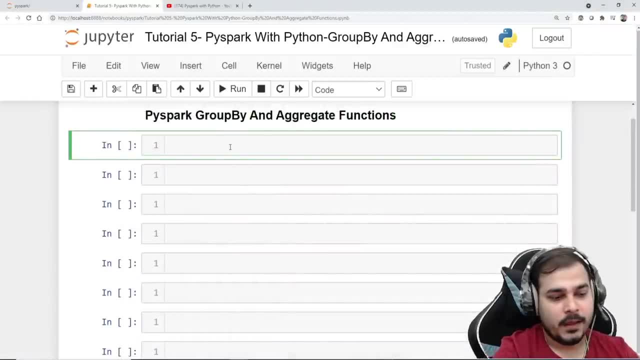 this particular data. so, to begin with, what we are going to do, we are first of all going to import pi, spark sql, import spark session. as usual, we have to create a spark session. so after this, what we have to do, i'll create a spark variable. so i'll use spark session dot. builder dot. 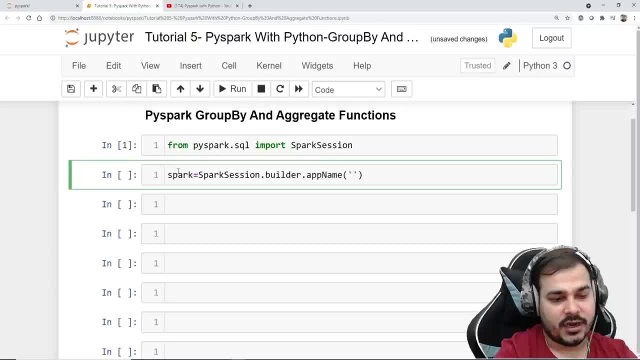 app name. i think everybody must be familiar with this, but again i'm trying to show you this one, so let me write it as aggregate dot: get or create. so now i've actually created a spark session. okay, probably this will take some time now if i go and check. 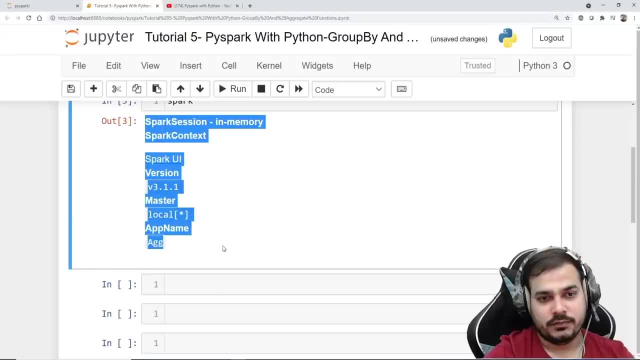 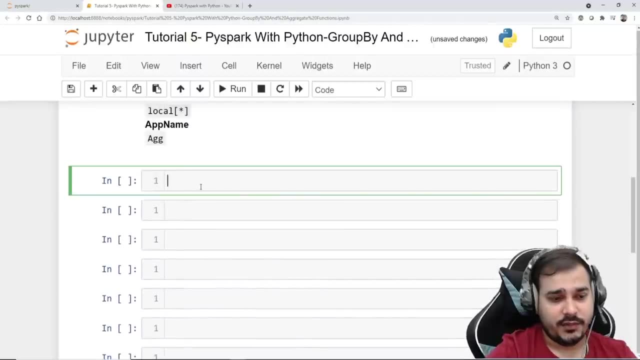 out my spark variable. so here is your entire information. okay, with respect to this part, i am going to use this particular spark variable. now let's go ahead and try to read the data set. now i will just write df, underscore, pi, spark, and then here i'll write spark, dot read. 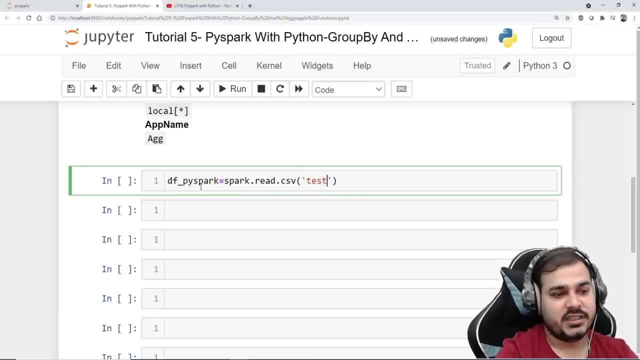 dot csv. the csv file name is basically test 3.csv. and remember i'll be giving this particular csv file in the github also and then i'll be using. header is equal to true comma in first schema. now this is my df underscore by spark. now what i'll do in the next statement i will write df. 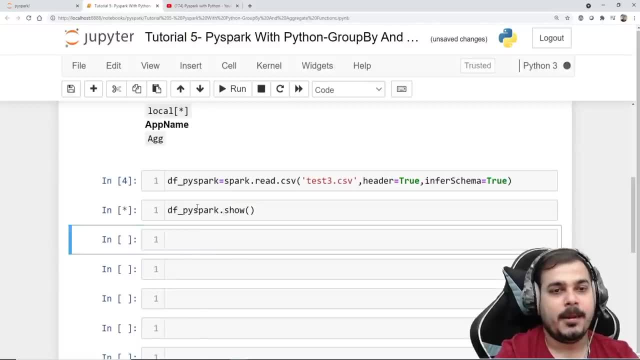 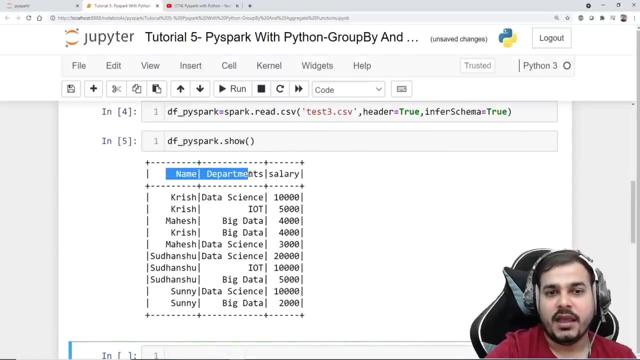 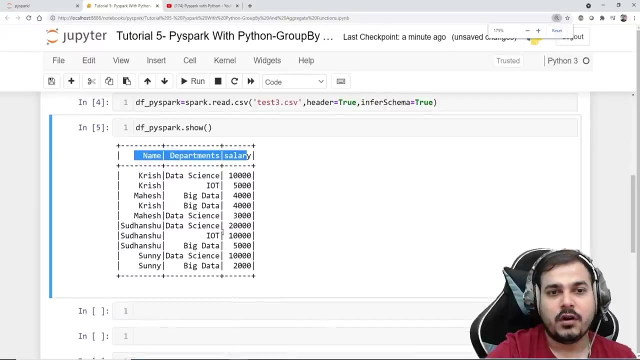 underscore by spark dot show right now. here you'll be able to see that i'm actually being able to see all the data sets here. i have name, departments and salary. on all this particular information, if i really want to see the schema or the columns like which- all columns where it belongs to, 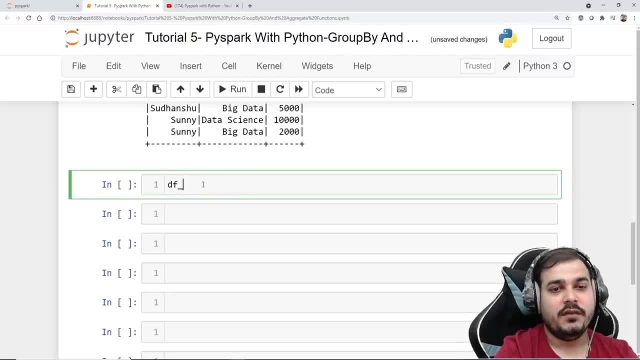 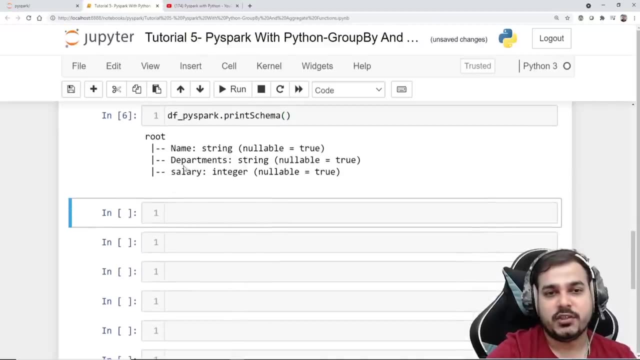 just like a data types. i can definitely use df underscore by spark dot print schema. right and now. here you can see: name is a string, department is string and salary is basically an integer. okay, now let's perform some group by operation. first. we'll start by group by operation. 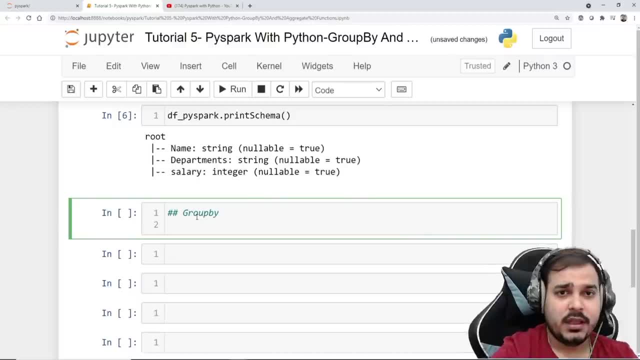 probably. i want to group by name and probably try to see what will be the mean average salary, you know, or what will be the mean average salary. what will be the mean average salary, what suppose? let's? let's take a specific example over here. so i'll write: df dot, underscore by spark. 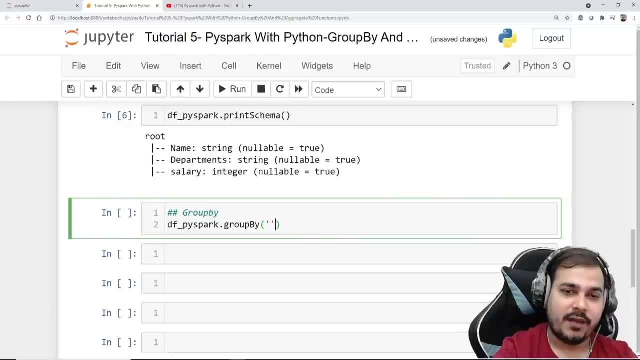 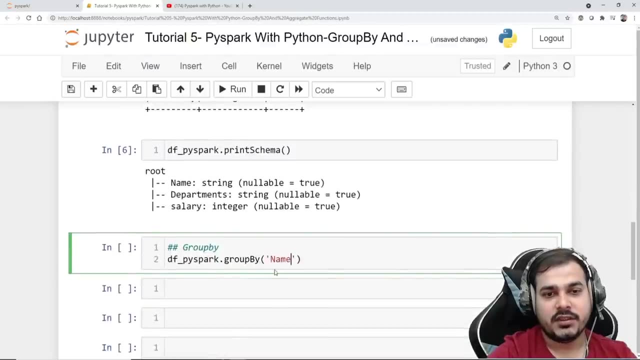 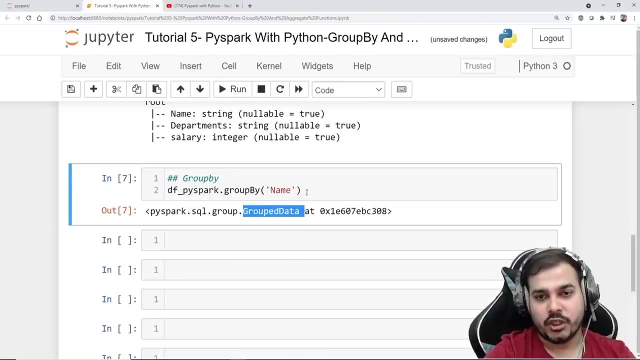 dot group by suppose i want to go and check who is having the maximum salary out of all these people that are present in this particular data set, so i'll first of all group by name. if i execute this, you can see that we will be getting a return type of group data at some specific memory location. 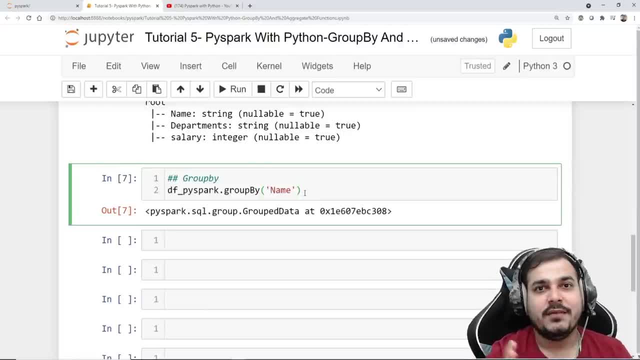 and you should always know that guys, group by an aggregate functions works together. that basically means first of all we up, we need to apply a group by functionality and then we need to apply an aggregate function. so aggregate function, if you really want to check, just press dot and press tab. 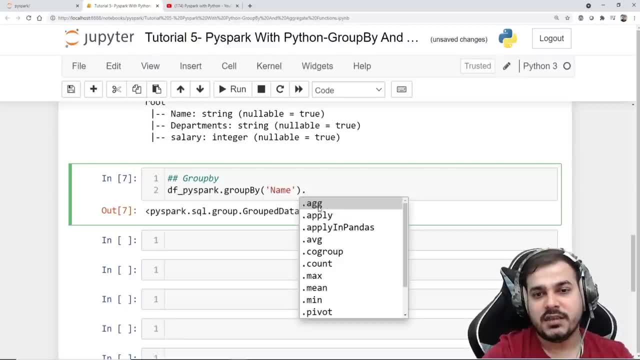 so here you'll be able to see a lot of uh, different, different function examples like aggregate, average, count, max, mean, pivot and many more. right now, what i'm going to do, i'm just going to use this dot sum because i really need to find which is the maximum salary now from out of all this particular employees. 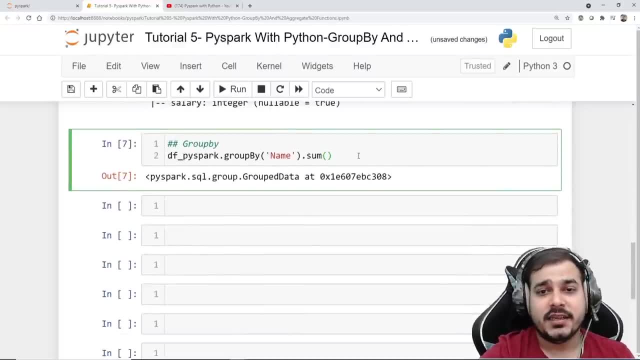 so what's the maximum salery is having the maximum salary. so here i'll say dot sum and if i execute it you'll be able to see that we are getting a sql dot data frame which has name and sum of salary. this is very much important, guys. 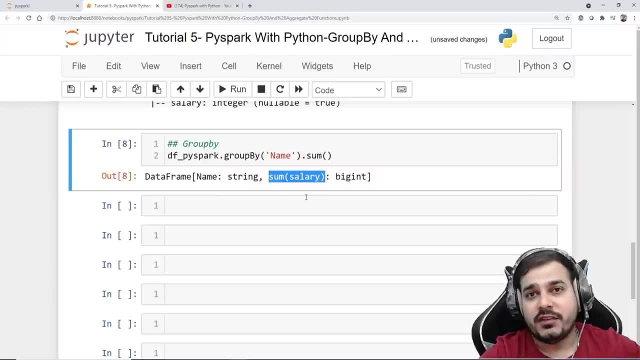 sum of salary, because i really want to have the sum of the salary. remember we cannot apply sum on the string, so that is the reason it has not done over here. it is just giving you the name, because we have group by name and this dot sum will just get applied on this particular salary. 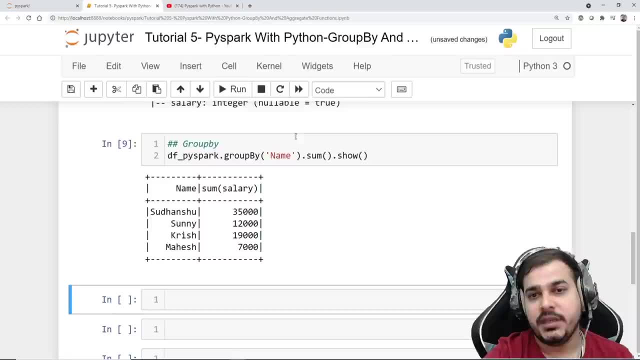 now, if i go and write dot show here, you'll be able to see sudhanshu over here is having the highest salary of 35 000, sunny has 12 000, krish has 19 000, mahesh has 7 000. so if you go and see, 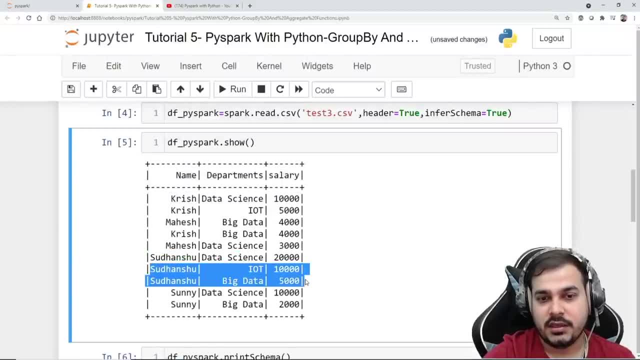 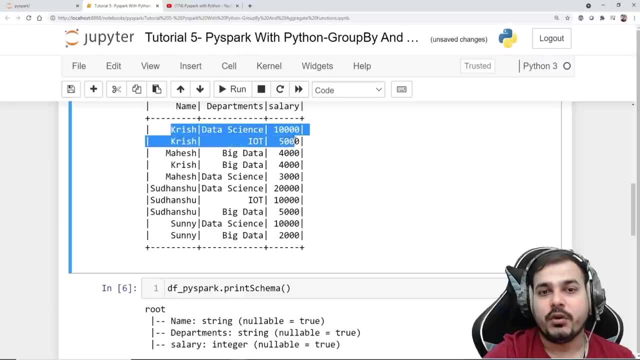 over here. sudhanshu is basically present here here and in big data, so overall his salary should be 35 000 if you compute it. similarly, you can go and compute my salary over here, over here, by just calculating my salary over here and i'll just calculate my salary over here and i'll just 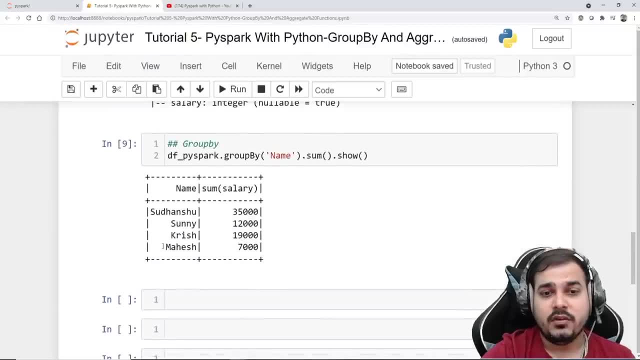 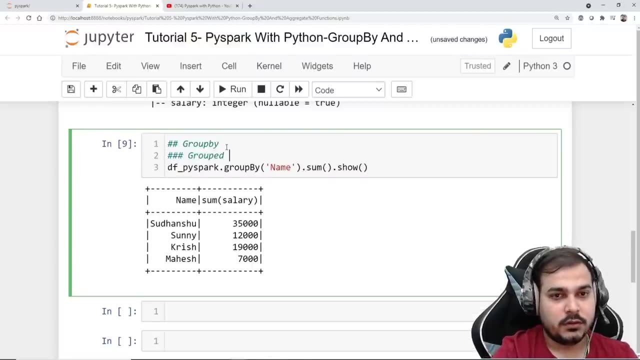 calculating this and then you can also compute sunny salary and you can also see mahesh salary. so this is one, just an example. so here i'll just write: we have grouped to find the maximum salary and definitely over here from this entire observation we can retrieve that sudhanshu. 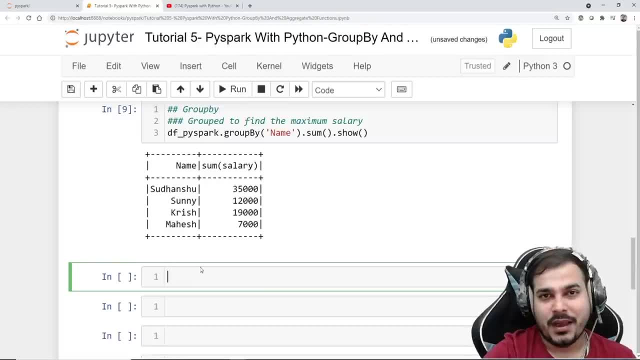 is having the highest salary. okay, now let's go to one step ahead. one more step ahead. now we'll try to group uh by departments to find out which is the highest salary of sudhanshu and which is the highest salary of sudhanshu. okay, so we are going to do a group by departments which gives maximum. 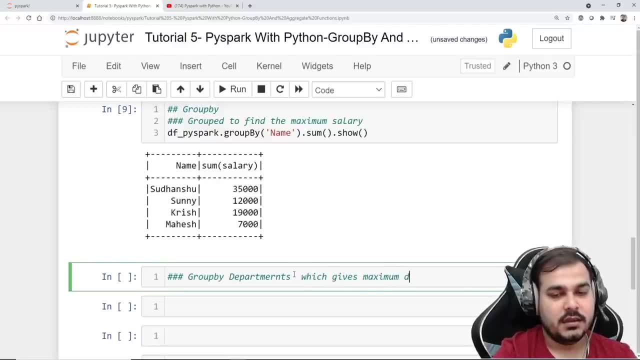 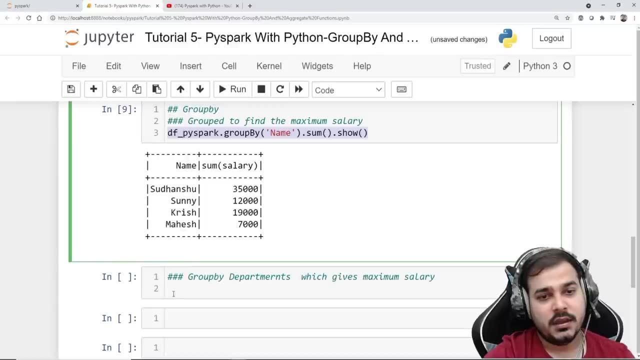 salary. suppose this is my, this is my requirement, okay, and different, different types of requirement may come. i'm just trying to show you some examples, so i'm just going to copy this: i'm going to use this department, okay, and then i'm basically going to say: dot, sum, dot, show, if i 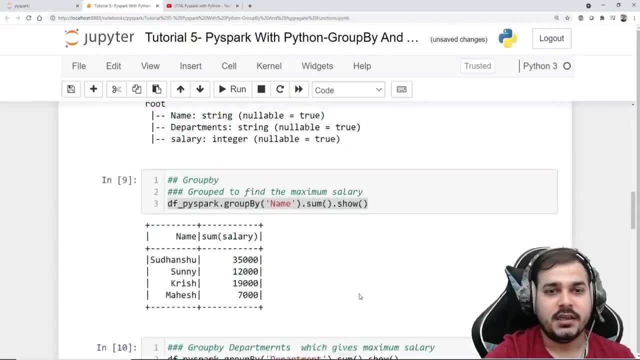 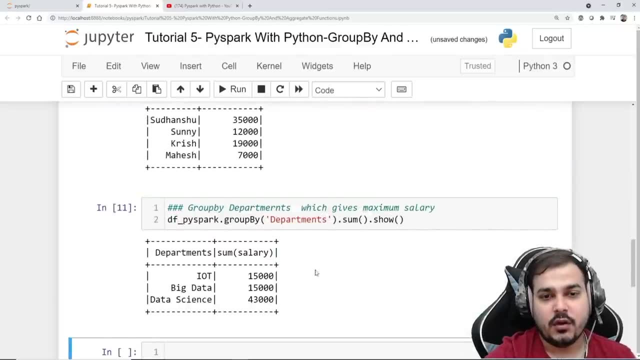 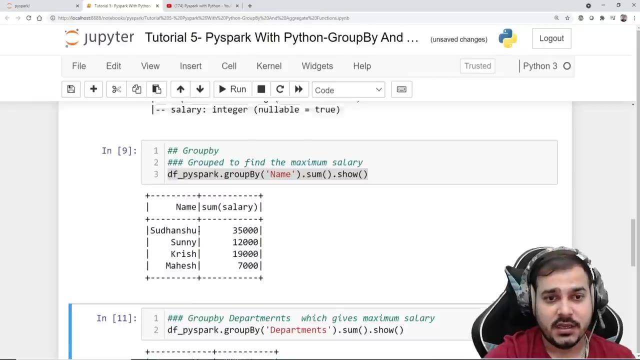 execute it. uh, let me see. department is a wrong uh column name so i'll write departments. it is departments, so let me write s. now, if i go and see iot over here gives some salary around one fifteen thousand to this employees, to all the employees right combined, because we are doing the sum big data gives. 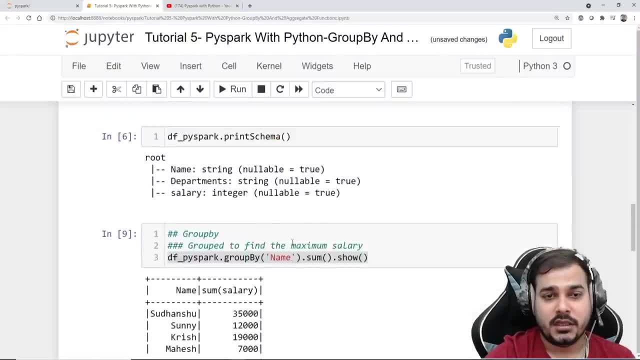 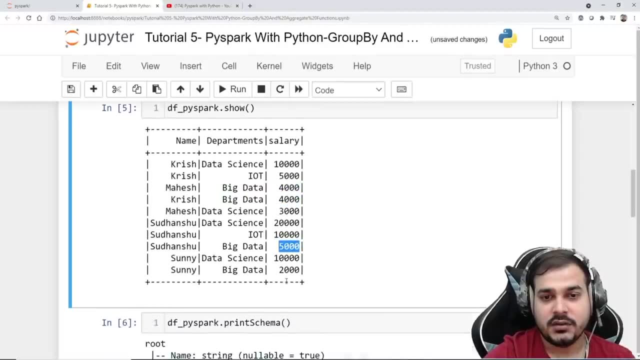 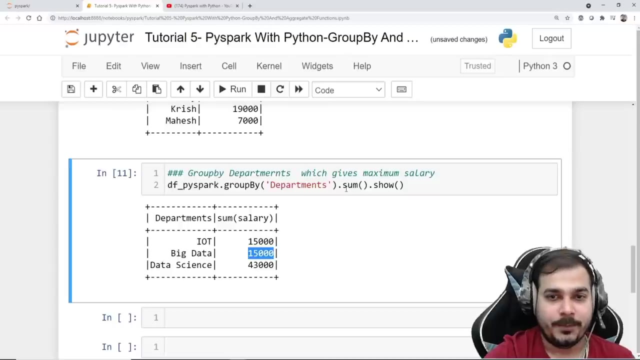 somewhere around fifteen thousand. data science gives around forty three thousand. now suppose, if i go and see big data over here, four thousand four thousand, eight thousand eight thousand and thirteen thousand, thirteen thousand fifteen thousand, so i hope i'm getting. yes, big data is actually giving us fifteen thousand, so you can go and calculate it. suppose. if you want to find out the mean, you can. 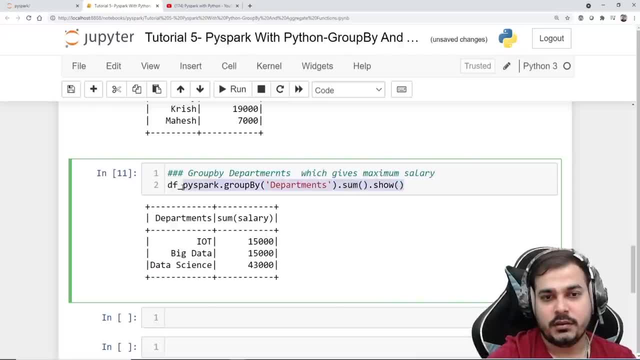 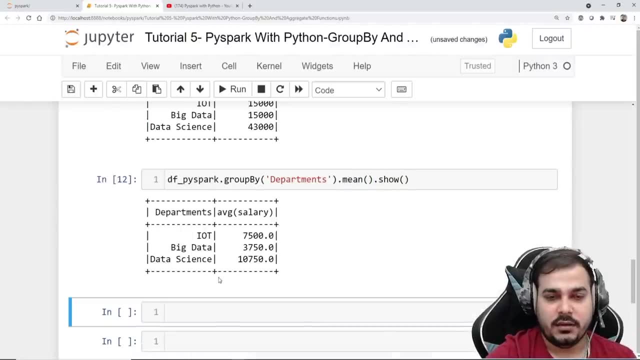 also find out the mean. okay, so let me just write it over here, just copy this entire thing, paste it over here and let me write instead of: instead of sum, i'll try to write mean. so by default, the mean salary here. you can see that for a particular employee somewhere, for iot it is 7 500, because this mean will be. 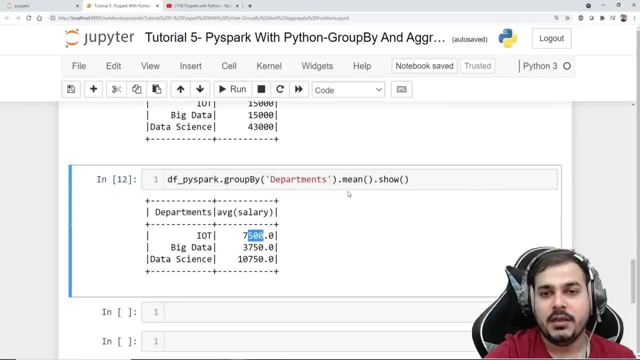 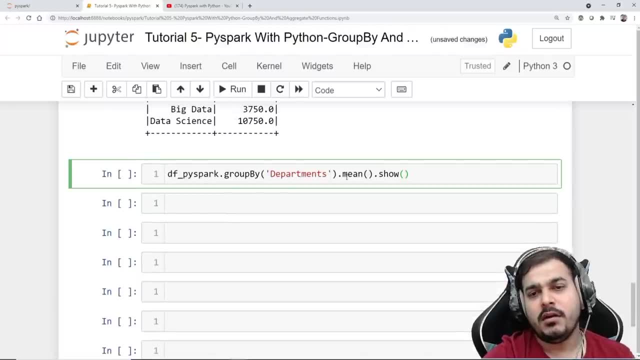 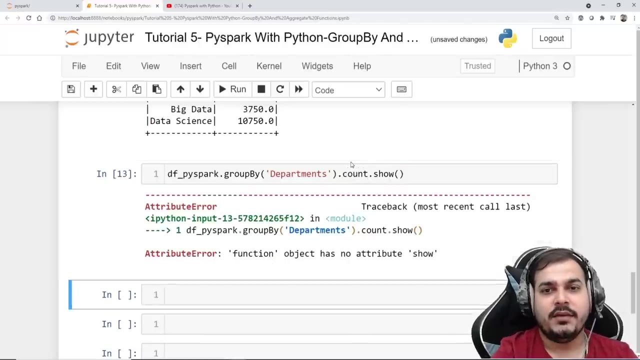 based on how many number of people are working in the department, right? so like this you can actually find out. now i can also check one more thing, guys. i can copy this. i can try to find out how many number of employees are actually working, based on the department. so i can use dot count and then if 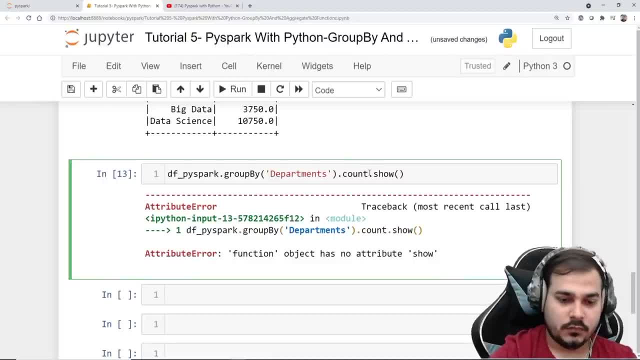 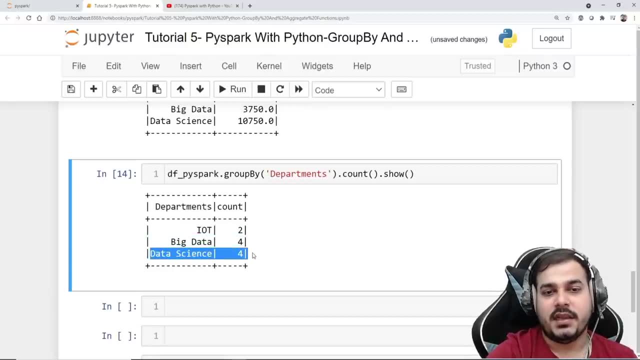 i go and execute this. probably this is a method. okay, now, here you'll be seeing that in iot there are two people, in big data, there are four people in data science. they are four people. so four plus four plus eight, total employees that are present over here is basically 10. now one more way that i 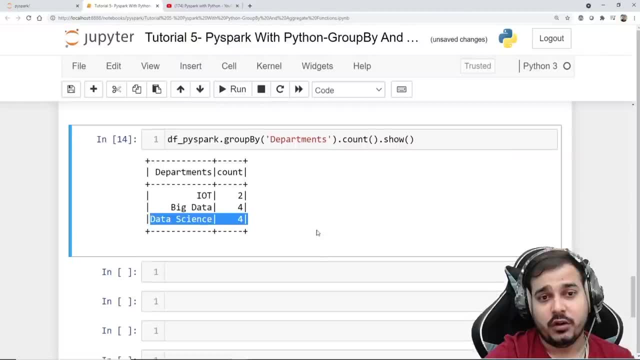 can basically apply a directly aggregate function also. now see, these are all some of the examples, and again you can do different, different group, by- let me use df, by spark. suppose i say dot aggregate, okay, and inside this i will just give my key value pairs like this, suppose i say: let me say that: 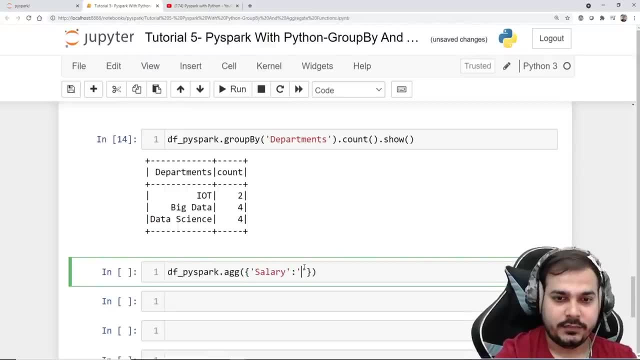 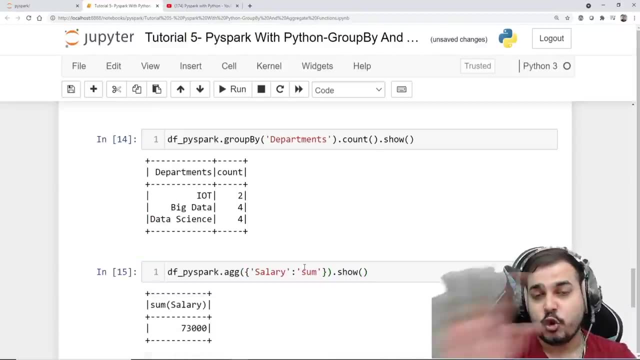 salary. i want to find out the sum of the salary. i want to find out the sum of the salary. i want to find out the sum of the salary. i want to salaries the overall salary that is basically given to the entire total expenditure. insert, so the total expenditure that you will be able to see somewhere around 73 000. all right, so we can. 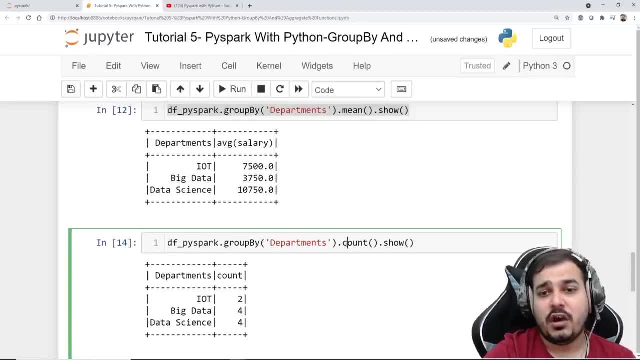 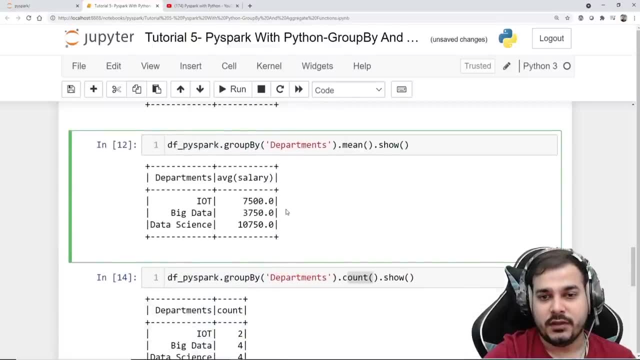 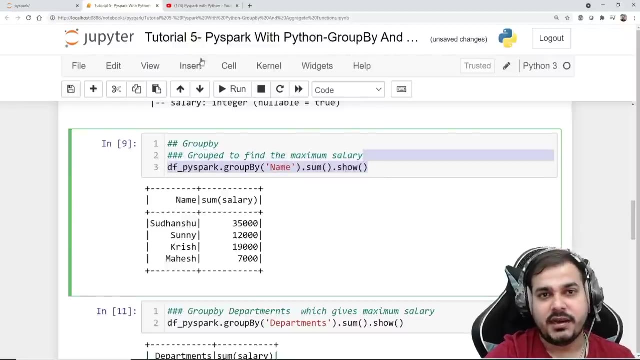 also apply direct aggregate function, otherwise this, all are also aggregate function, which we basically apply after after, um, you know, applying a group by function. now, suppose these are probably the salary i want to find out. suppose i'll take this example: i want to find out the maximum salary. 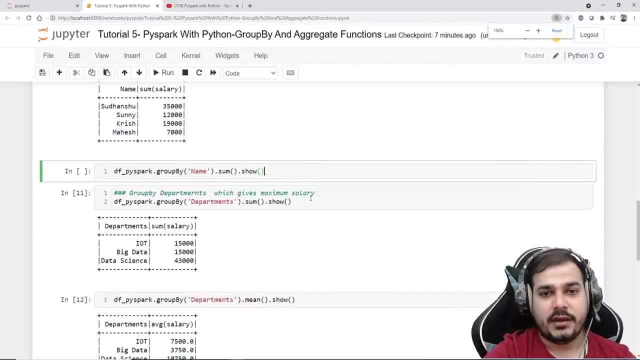 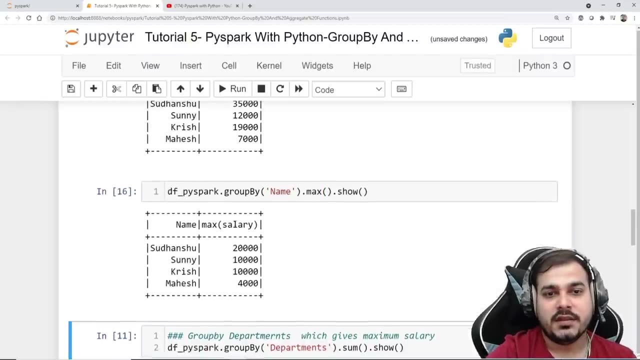 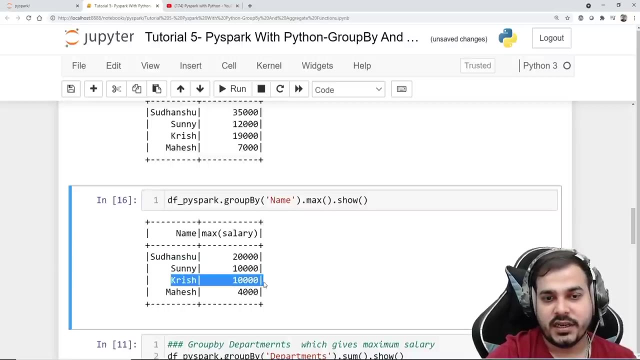 that the person is basically getting who is getting the maximum salary. sorry so here, instead of writing dot sum now, i'll write max dot show now. here you can see: uh, sudanshu is basically getting 20 000 now over here, 10, 10 000 krish is getting 10 000. maesh is getting for 4 000. right. 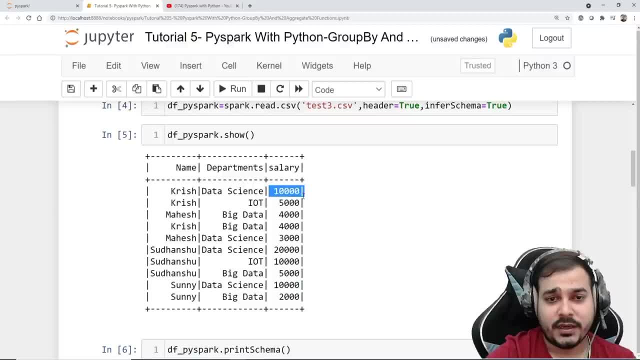 so all this particular data is there. see, krish is basically getting, with respect to, you know, the salary that the person is getting. so here you can see that the maximum salary that the person is getting- uh, data science over here- 10 000. so it has basically picked up. it is not. 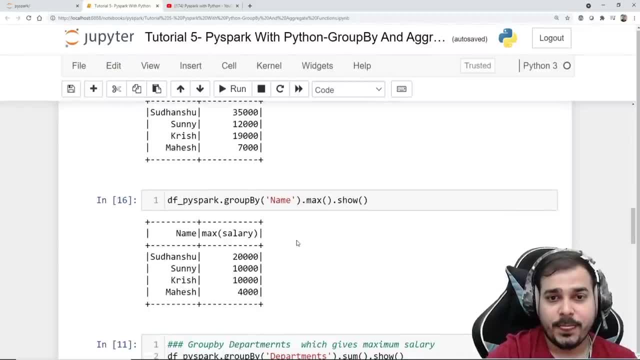 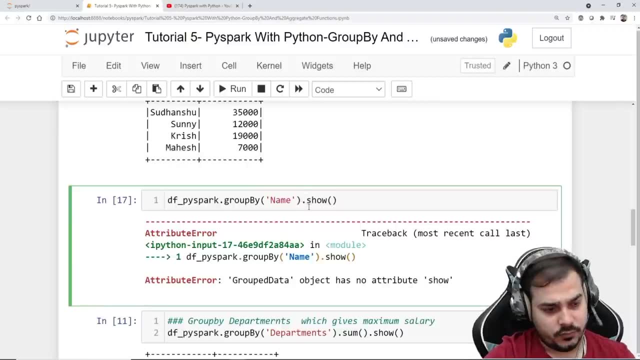 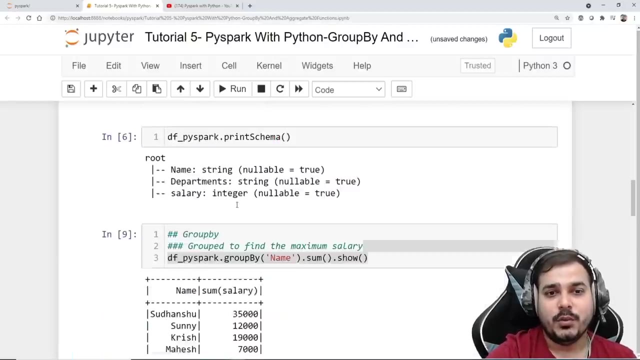 picking up both the records. but at least when it is grouping by name and then it is showing, uh, this particular data, that time you will be able to see it. let's see whether i'll be also able to see this or not. so, group by if i score and write min. so here you will be able to see minimum value with. 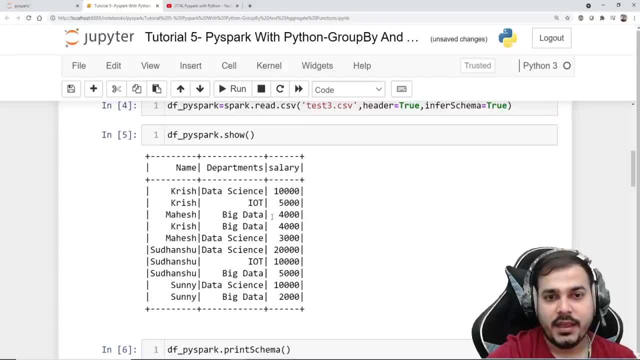 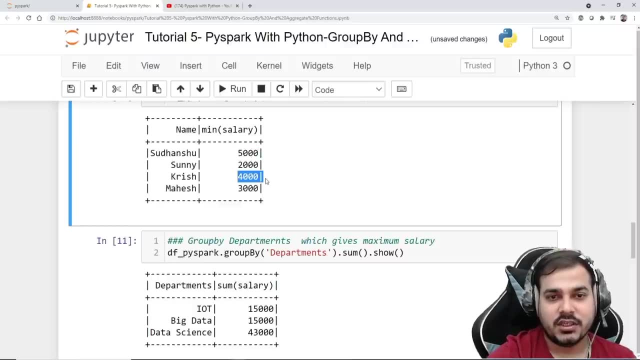 respect to different, different records. when i'm grouping by here, you'll be able to see that: uh, sudanshu, oh sorry, sudanshu is getting a minimum salary of five thousand two thousand krish, is getting a minimum salary of four thousand. right, we can also get that particular information now. 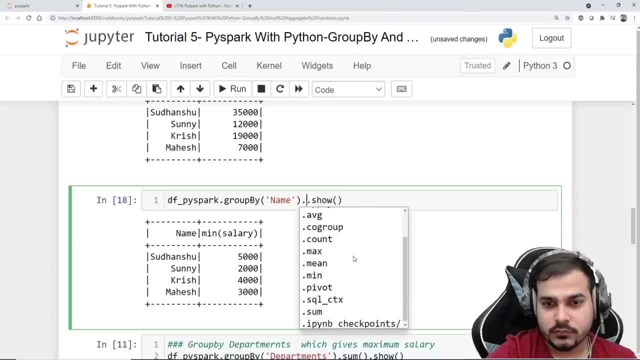 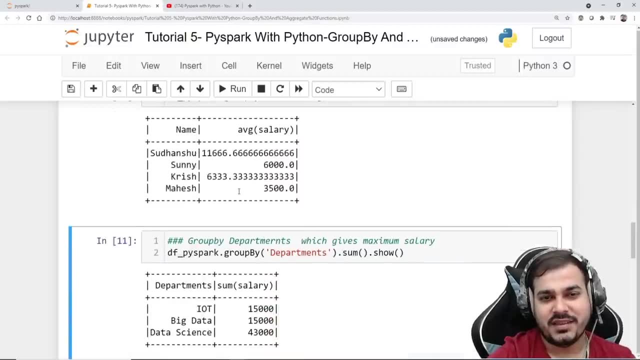 let's see what all different different types of operation are there. average is also there. so if i write avg, it's just like mean, only guys. so this is basically the mean salary that probably you're getting again. you can check out different, different functionalities. why these all? 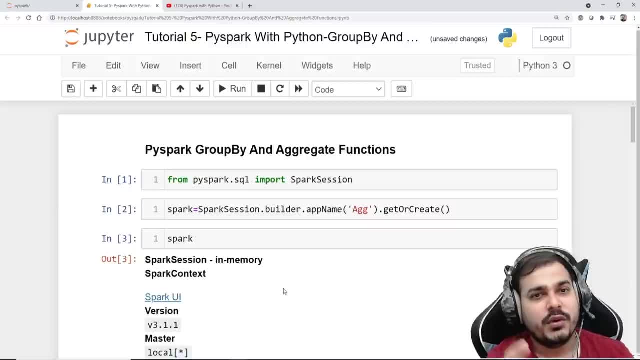 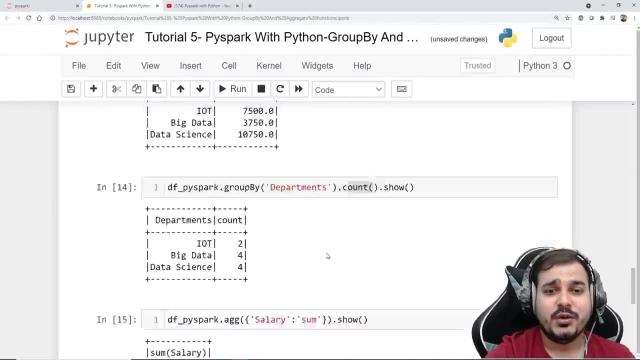 things are basically required. understand one thing is that you really need to do a lot of data pre-processing, a lot of retrieving skills. that you basically do. you can check it out this one and you can do different, different functionalities as you like. spark mlib also has. 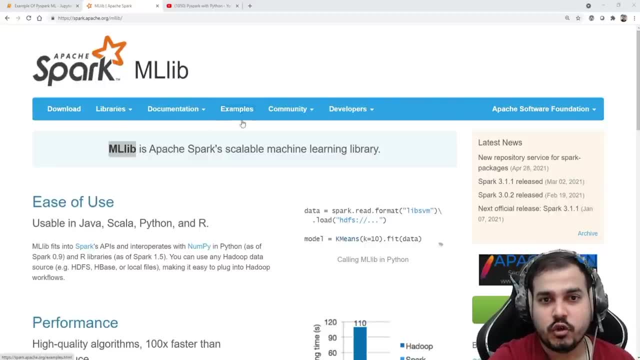 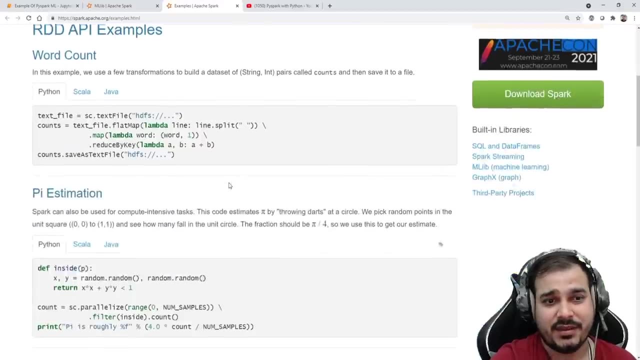 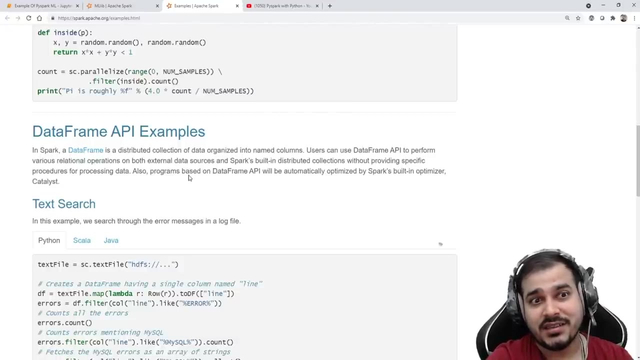 an amazing documentation with respect to various examples. so here you can go and click on examples and basically check out this particular documentation. you can actually see different, different kind of examples how it is basically done. but with respect to spark ml, there are two different techniques. one is the rdd techniques and one is the data frame apis. now what we are going to. 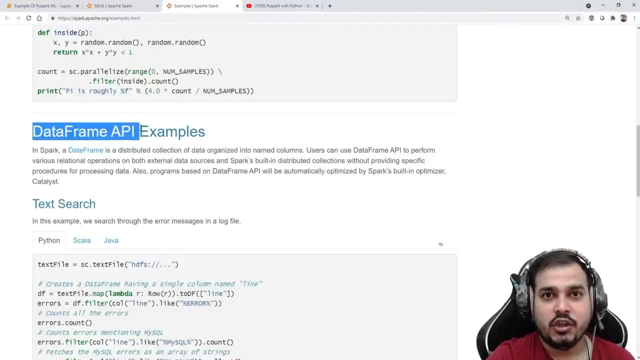 do guys? data frame api is the most recent one you know and it is pretty much famously used everywhere. so we'll be focusing on data frame api. that is the reason why we learned data frame in pisepak very much nicely. so we'll try to learn through data frame apis and we'll try to see. 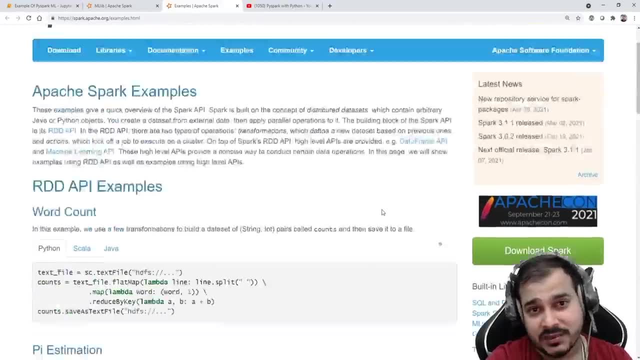 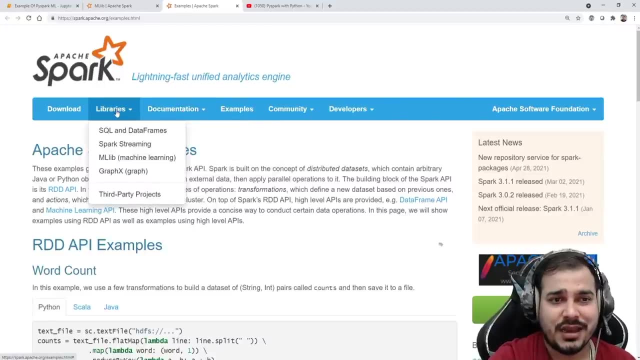 the technique, how we can basically solve a machine learning use case. now let's go and see one very simple example, guys, and always remember: the documentation is pretty much amazingly given. you can actually check out over here and try to read the documentation. you can actually check out over here and try to read the documentation. you can actually check out over here and try to. 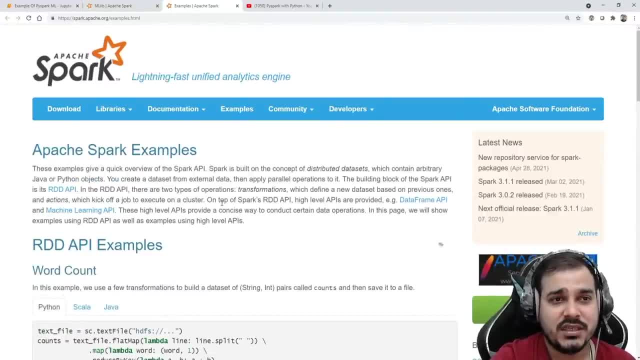 read all these things. okay, so let's proceed and let's try to see, uh, what are things we can actually do in this particular example. i'm just going to take a simple machine learning problem statement. so let me just open a specific data set for you all, and then probably we'll try to do it. 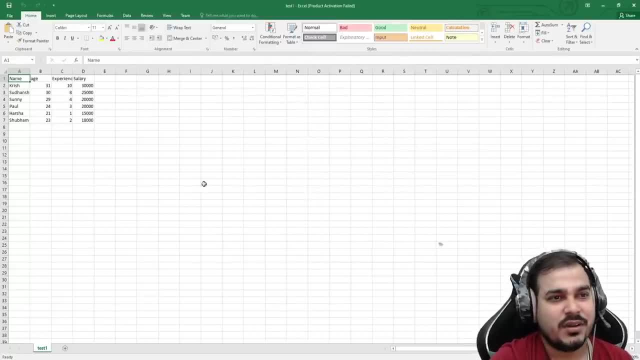 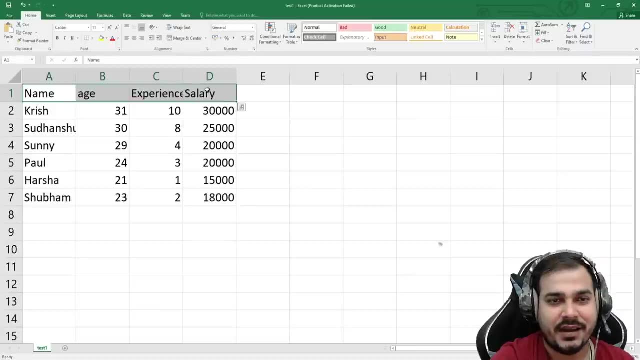 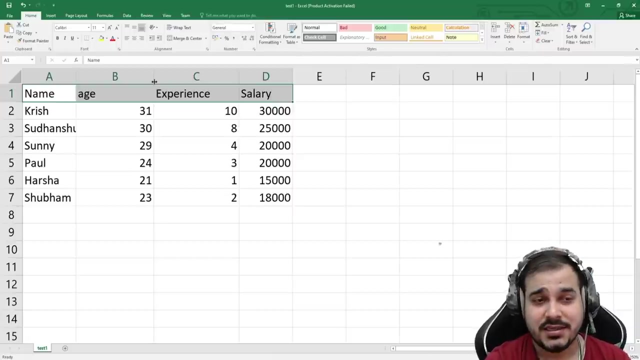 okay so this is my data set. guys, i know there are not many records over here. okay so i have a data set which has like name, age, experience and salary, and this is just a simple problem statement to just show you that how powerful a spark actually is with respect to an envelope library, just to show. 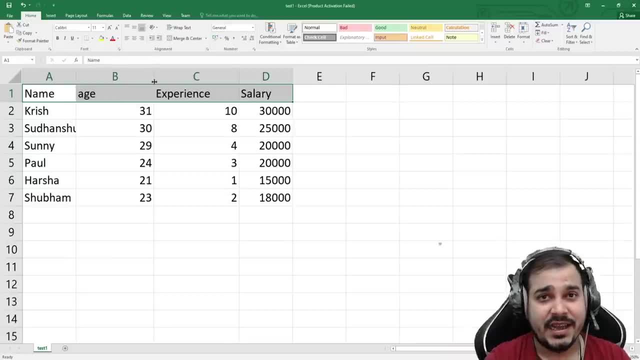 you a demo from the next video. i'll be showing you detailed explanation of the regression algorithms, how we can basically do the implementation and all theoretical and all guys i have already uploaded you can see over here i'll be doing. see after this: tutorial 5: this is basically the 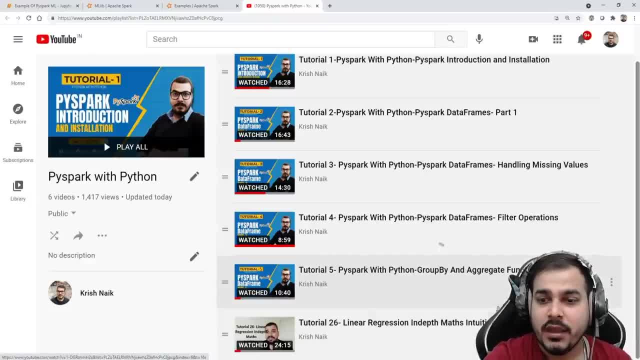 tutorial 6. i'll try to add it after this and then whenever i will be uploading the linear regression algorithm. before that, please make sure that you watch this maths intuition. okay, i've uploaded this specific video also in the same playlist. so after this, tutorial 26: see why it is saying tutorial 26. 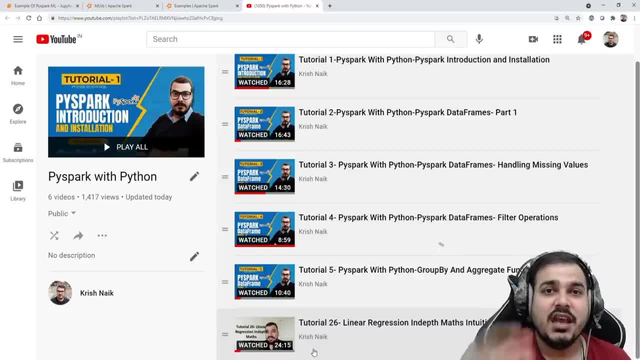 because i have also added this in my machine learning playlist. so after this, you'll also be able to find out, when we'll be discussing about linear regression, how we can implement in depth that video will also get uploaded. so let's proceed. and here is my entire data set. guys, this is my 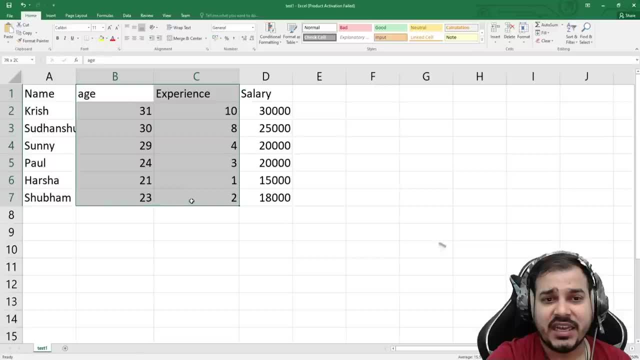 data set. now what i have to do is that, based on age and experience, i'm going to show you how i can predict the salary. based on age and experience, i need to predict the salary. very simple use case: not not much data pre-processing, not much transformation, not much standardization and. 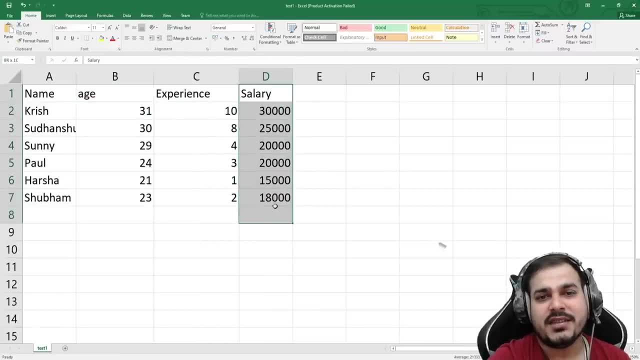 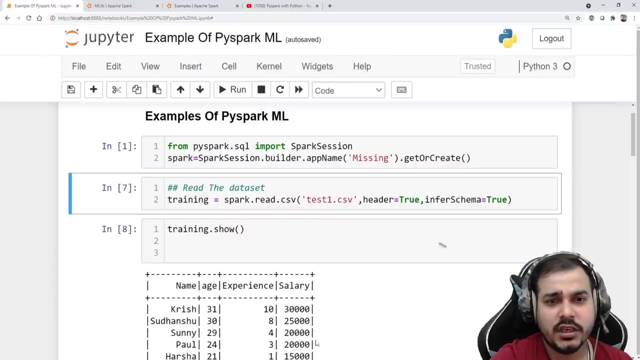 all, okay, i'm just going to take up this two independent feature and i will be predicting the salary of this particular uh person based on age and experience. okay, so this is what i'm actually going to do. so here is a perfect example. again detailly, i'll try to show you how to. 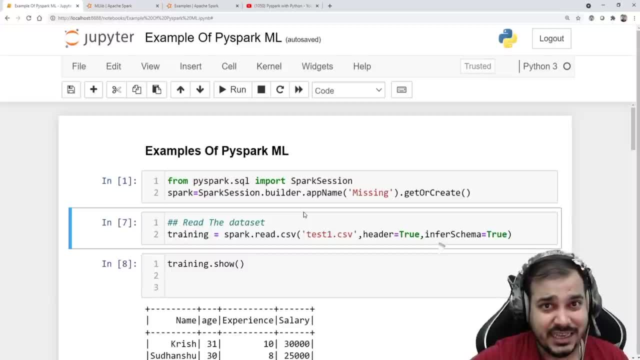 basically implement line by line, probably from the upcoming videos where i'll be doing the tutorial 6, discussing about linear regression and all. and if i go see this particular problem, this is also a linear regression example. okay, so let's go over here. uh, first of all, as usual, i will be creating 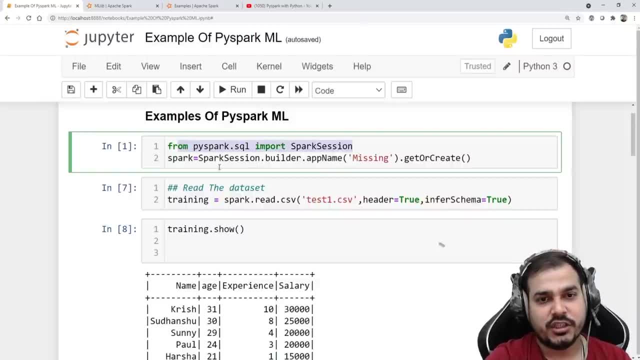 a spark session. so i'll use from five spark dot sql import spark session and then i'm going to use spark session dot builder, dot app name. here i'm actually creating a spark session on missing. let me execute it. i think this is pretty much familiar. you're familiar with this. uh, then what? 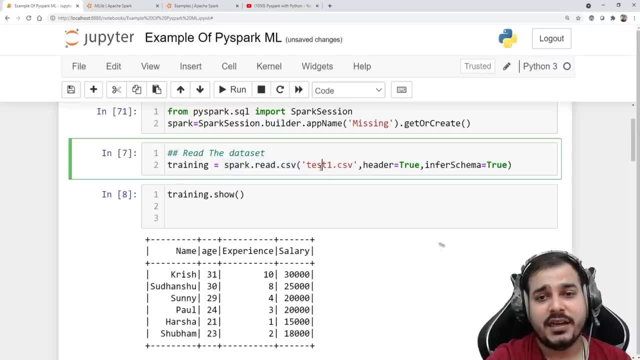 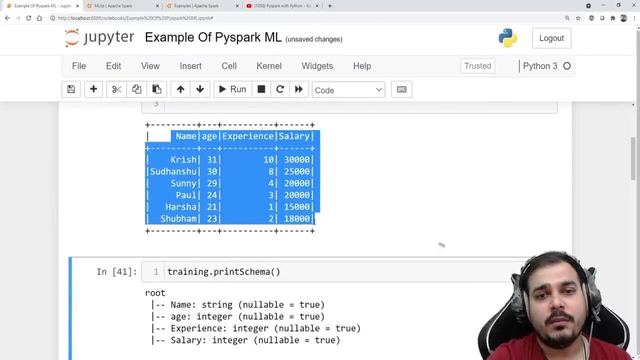 i'm going to do over here is that we are just going to read this particular data set with csv: header is equal to true and infer schema is equal to true. so when i go and see my training dot show, these are all my features over here. perfect, i'll be giving you this data set also. 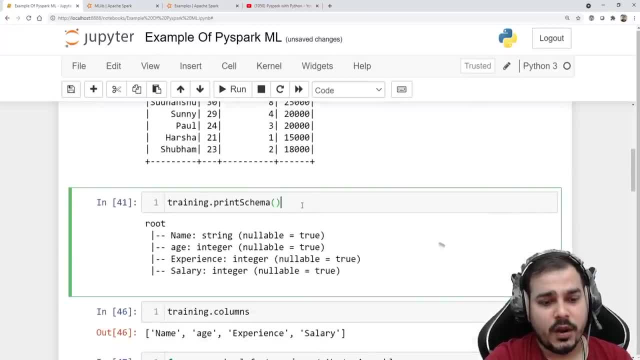 don't worry now, from this particular data set. if i go and check out my print schema, so here you'll be able to see that i'm getting this particular information. this is my entire print schema. over here i have features like name, age, experience and salary. now 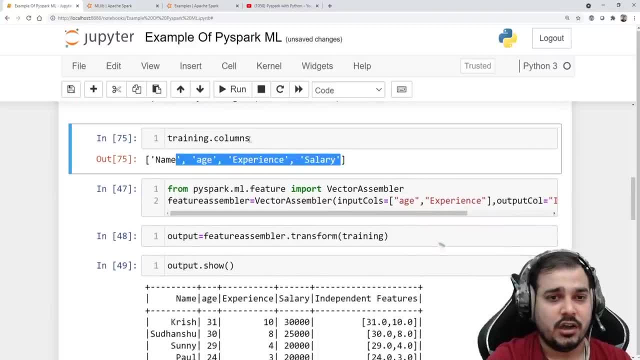 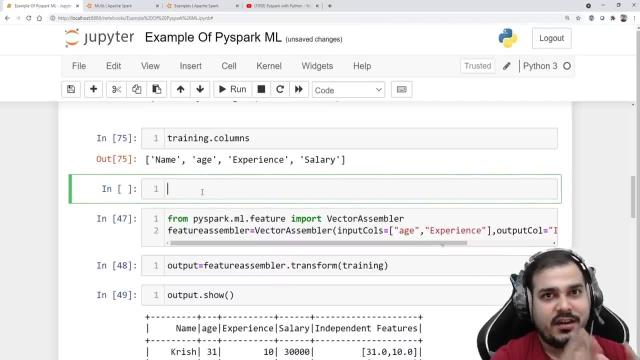 if i go and see training dot columns- this is my training dot columns now- always remember guys in spark we use a different funda or mechanism or a kind of data pre-processing before. see, usually what we do is that in on by using machine learning algorithms that are available in escala. we 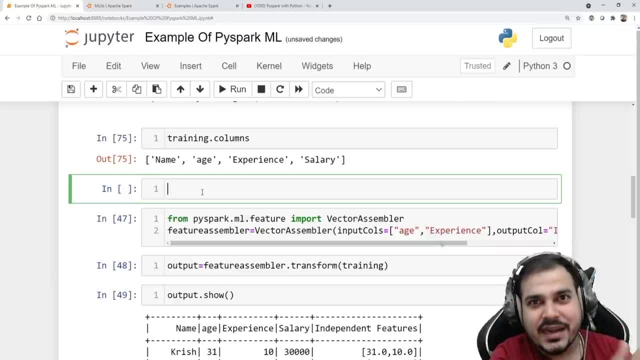 basically do a train test split, right, and then we first of all divide that into independent features, dependent features, right, which, uh, we use an x and y variable, and then we do train test plate by doing this in, in, in pi spark. we just do some different techniques. what we do is that, yes, we have. 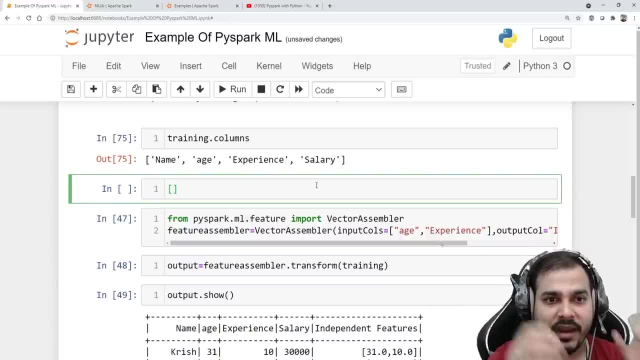 a very unique seit ワでsa, like all of my features. physically, we can actually do that um. uh, as you know, a lot of people think not all of it is them if um for revision, i think that i- let's say like i do it, i do so many certain kits. 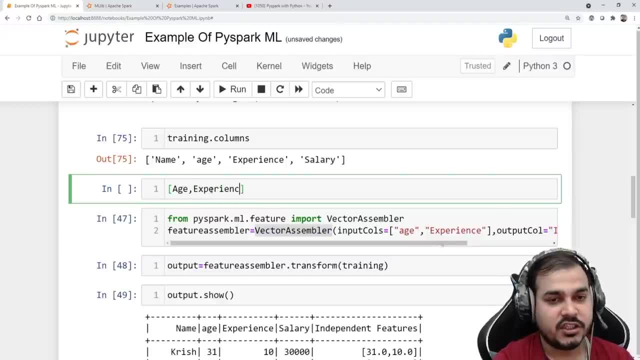 in my experience. so basically, i will basically create a way where i can group all my independent features. so probably i'll try to create a vector sampler. we basically say it as a vector assembler. see over here the class i've actually used. the vector assembler will make sure that i have all my 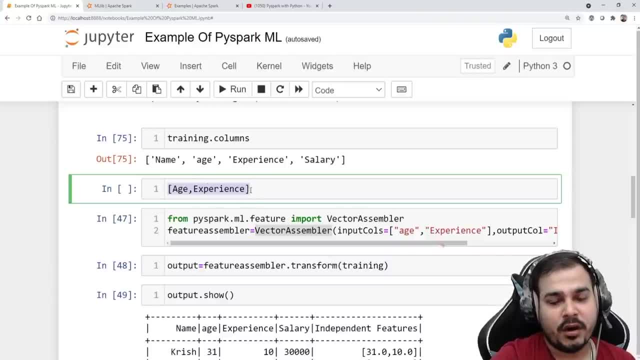 for every record, it will be grouped like this: okay, for every record, it will be grouped like this, and then what i will be doing is that i will be treating this grouped as a different feature. so this will basically be my new feature. right, and remember, this new feature is my independent. 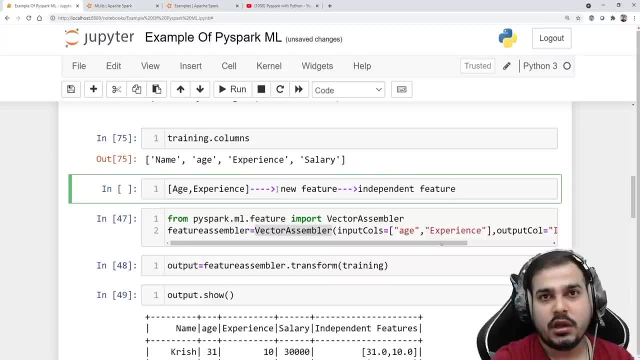 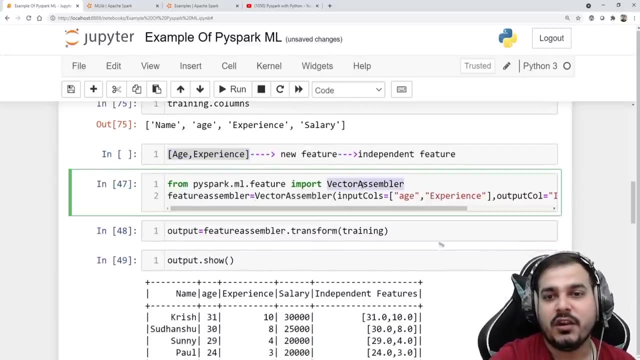 feature. so my independent feature will look like this: in a group, of age comma, experience, which will be treated as a new feature. and this is exactly my independent feature. so i have to group this particular way. so in order to group this, what we do is that in pyspark we use something called 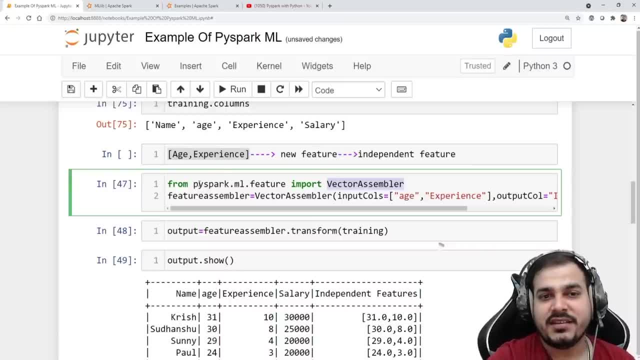 as vector assembler. so in this vector assembler it is basically present in pysparkmlfeature. we use this vector assembler. we use two things. one is input column, which all column we are basically taking to group it. so two columns: one is age and experience. right, we don't have to take. 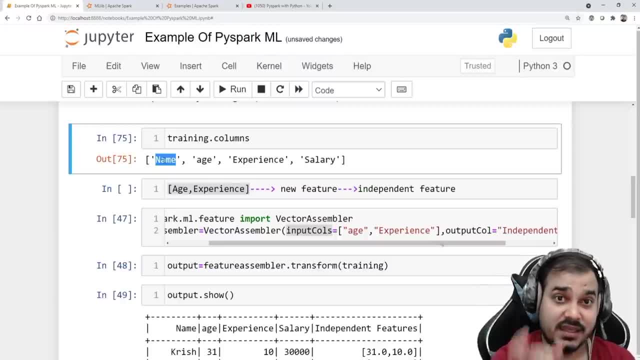 name, because name is fixed, it is a string. yes, if category features are there, what we do, what we need to do, we will convert that into some numerical representation that i'll be showing you when i'm doing some in-depth implementation in the upcoming videos of linear regression, logistic regression and all 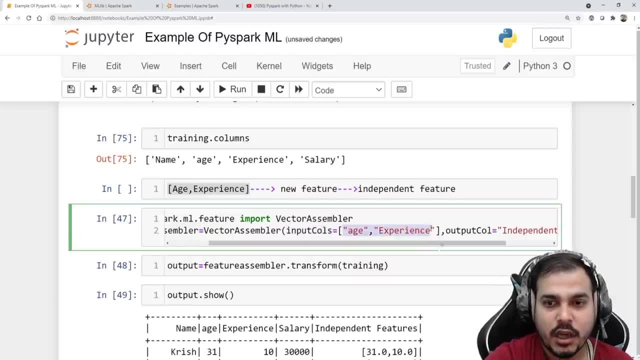 but here you'll be able to see that i'm going to take input columns- age comma, experience- in the form of a list, and then i will try to group this and create a new column which is called as independent feature over here. right, that is what i'm actually doing. so if i go and execute this, 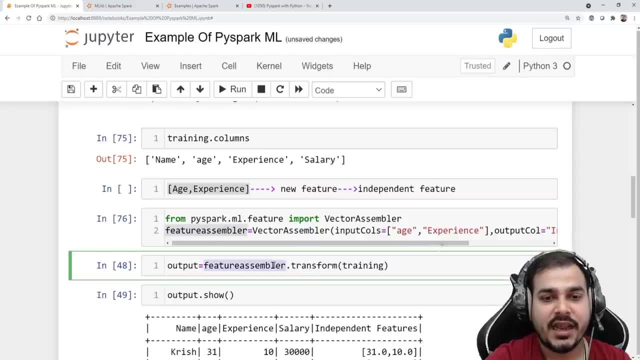 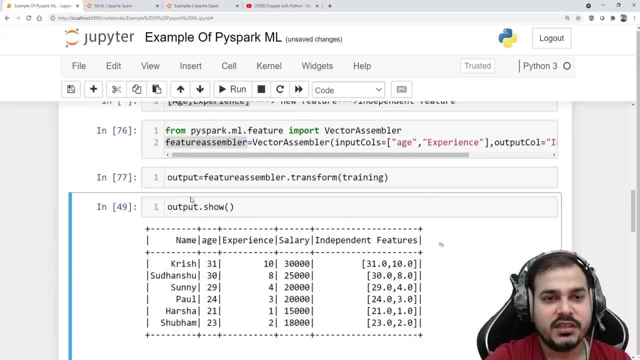 vector assembler. so here i've got my feature in assembler and then i do dot transform. i do dot transform on my training data. so this is basically my training data. when i do this and when i do output dot show. here you'll be able to see i had dissolve features and a new feature has been created which is called. 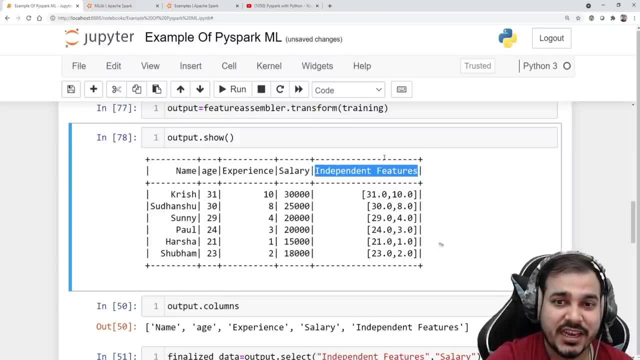 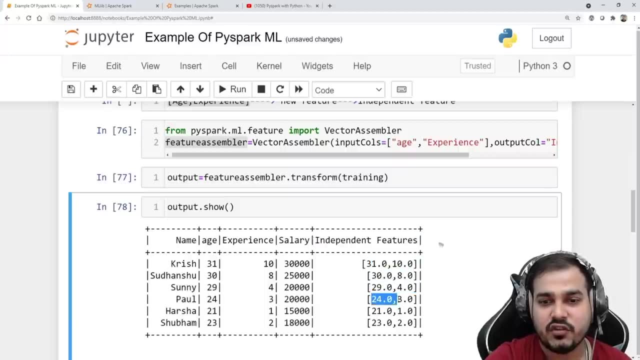 as independent features. okay, so we have actually created an independent feature and you can see over here age and experience, age and experience, age and experience. so this is my grouped roles that i've actually got. in short, what i've done, i've actually grouped members. so this is why do i call them? 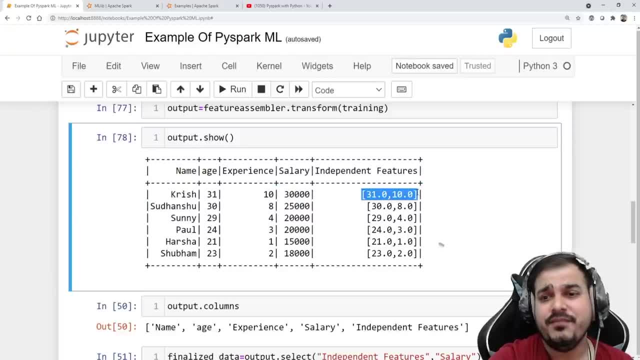 in design, as the new Stephens have, just, i guess, orfuncals rather people. so instead of joining the tool, i've combined this two column and made it as a- uh, a single independent feature. okay, now, this will be my input feature. okay, and this will be my output feature, and we'll try to train the model. 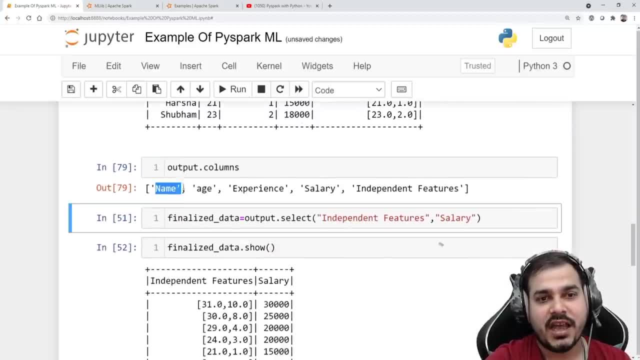 okay, so over here now, if i go and see output dot columns, i have name, age, experience, salary, independent feature. now what i'll do out of this, let's take which all data set i'm actually interested in. so out of this i will just be interested in this: two data set right, independent. 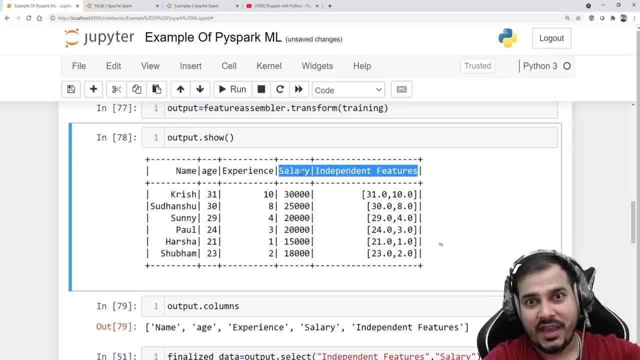 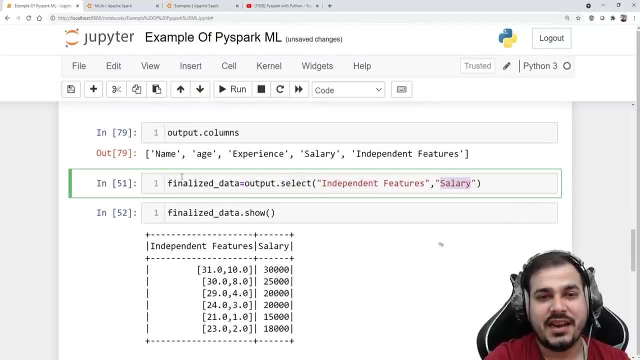 features and salary. salary will be my output feature, the y variable right and this will be my input feature. so what i'm going to do, i am going to select output dot, select independent features and salary and i'm going to put that in my finalized underscore data. that is what i'm 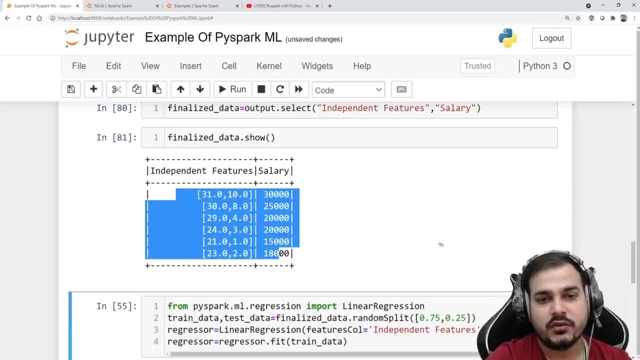 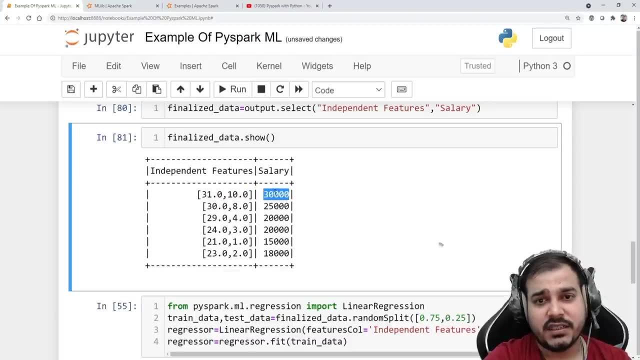 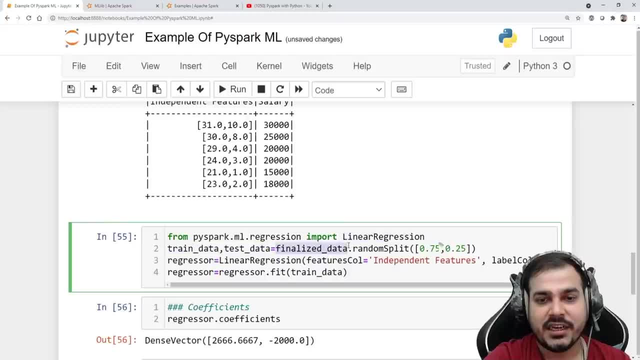 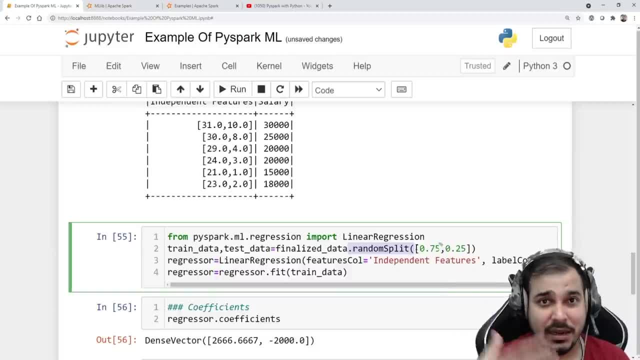 inside my finalized data, which is called as random split. remember guys, i'll try to explain you line by called as random split. remember guys, i'll try to explain you line by called as random split. remember guys, i'll try to explain you line by line, by implementing it when i'm doing a. 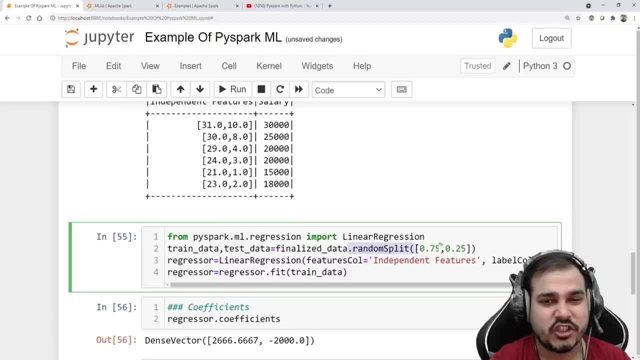 line, by implementing it when i'm doing a line, by implementing it when i'm doing a bigger project right now, since this is bigger project right now, since this is bigger project right now, since this is just an introduction session, i really just an introduction session, i really 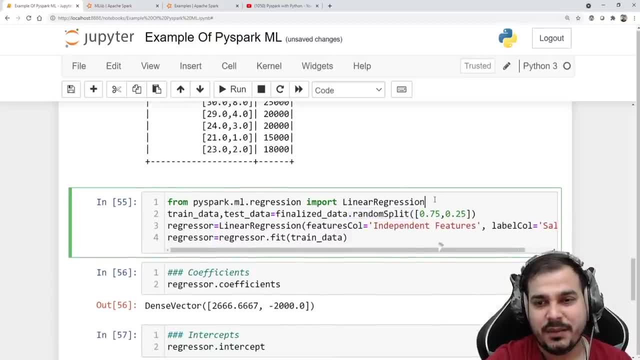 just an introduction session. i really want to explain you how things are, want to explain you how things are, want to explain you how things are actually done. so this is basically my actually done. so this is basically my actually done. so this is basically my train test split. so here let me write it. 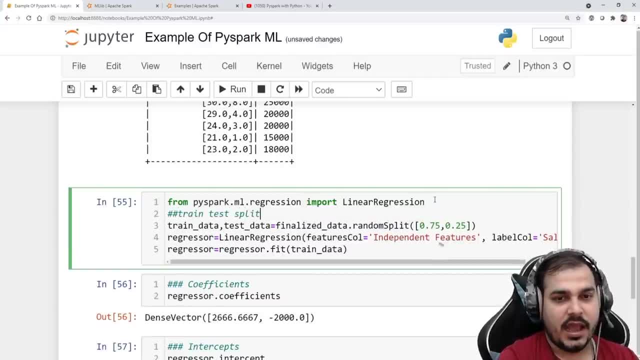 train test split. so here let me write it: train test split. so here let me write it down, the comment down, the comment down, the comment. train test split. train test split. train test split, and i will be using the linear and i will be using the linear and i will be using the linear regression, like how we import a class. 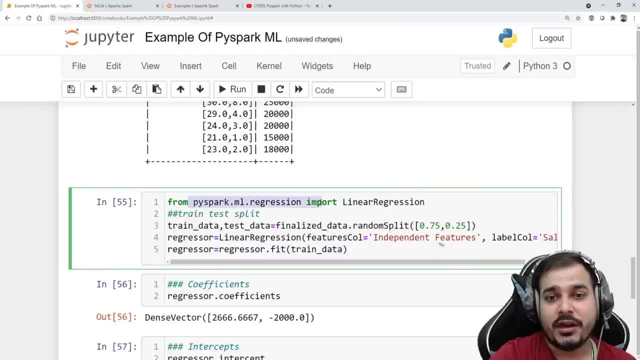 regression like how we import a class regression like how we import a class from sklearn, similarly uh, by using from sklearn, similarly uh, by using from sklearn, similarly uh, by using pysparkmlregression: import linear pysparkmlregression, import linear pysparkmlregression, import linear regression. and then i'm doing a random. 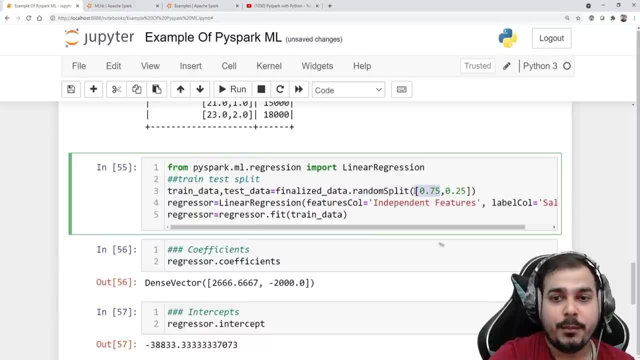 regression and then i'm doing a random regression and then i'm doing a random slip of 75 to 25. that basically means my slip of 75 to 25. that basically means my slip of 75 to 25. that basically means my training data set will be having 75. 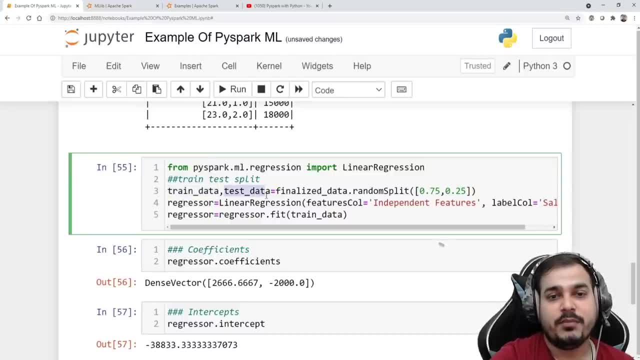 training data set will be having 75 training data set will be having 75 percentage of the data and my test data percentage of the data and my test data percentage of the data and my test data set will be having 25 percentage of the set will be having 25 percentage of the. 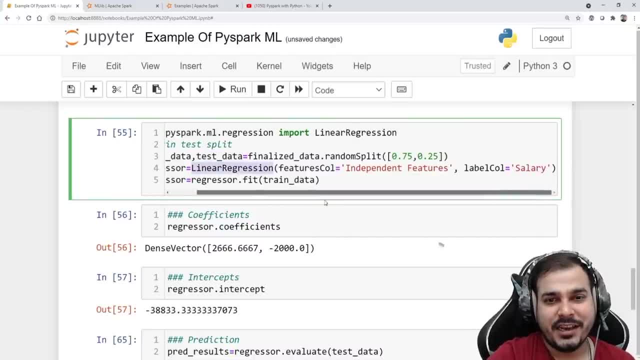 set will be having 25 percentage of the data right data, right data right. then after that i'll be using this, then after that i'll be using this, then after that i'll be using this linear regression in this you have two linear regression in this, you have two. 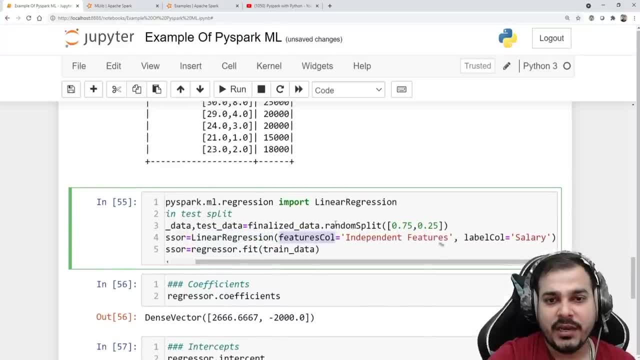 linear regression. in this you have two important variables that we need to give, important variables that we need to give, important variables that we need to give. one is feature columns, one is feature columns. one is feature columns. how many number of feature columns are? how many number of feature columns are? 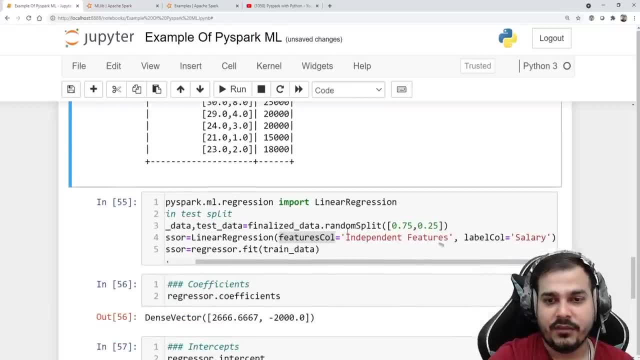 how many number of feature columns are there that is completely present in this there, that is completely present in this, there, that is completely present in this independent feature, independent feature, independent feature. so i'm giving it over here, similarly in. so i'm giving it over here, similarly in: 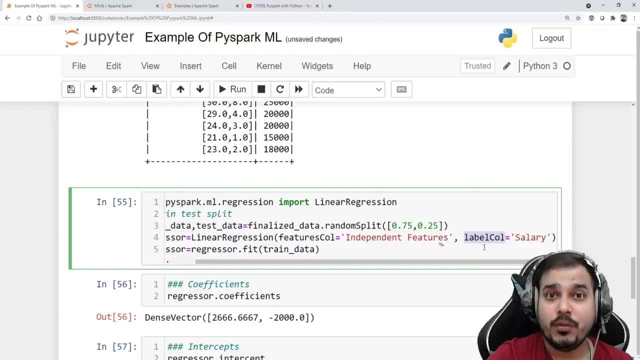 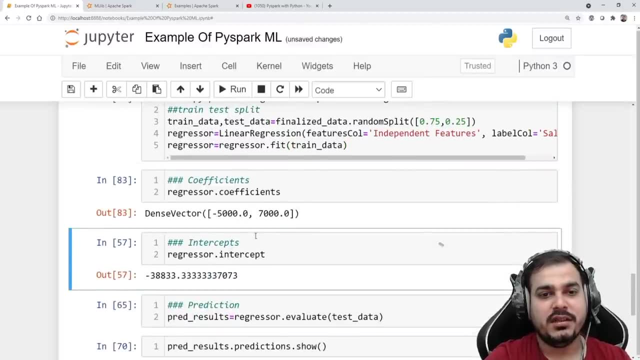 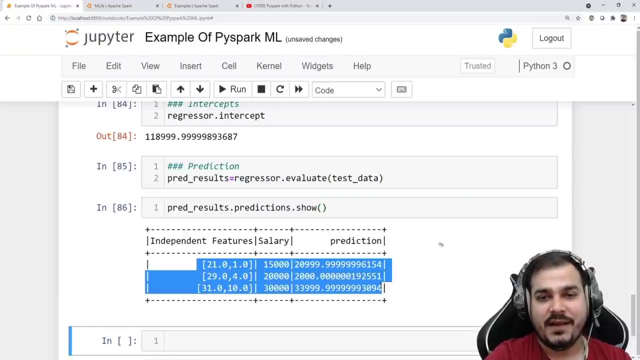 so i'm giving it over here. similarly, in label column: this is my second feature, label column. this is my second feature, label column. this is my second feature that i have to give. this is my that i have to give. this is my second feature that i have to give. this is my second feature, my output right. so by using this, 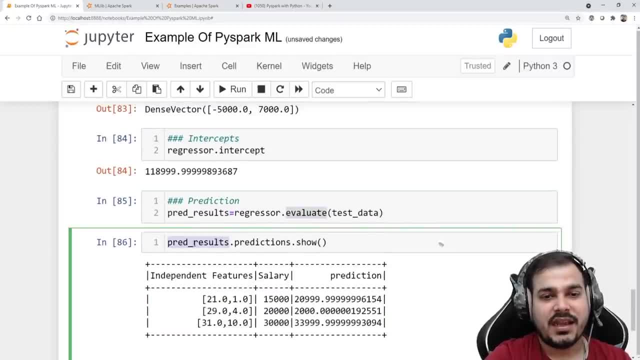 my output right. so by using this, my output right. so by using this evaluate function, we will be able to see evaluate function, we will be able to see evaluate function, we will be able to see the output, and inside this there will be the output and inside this there will be. 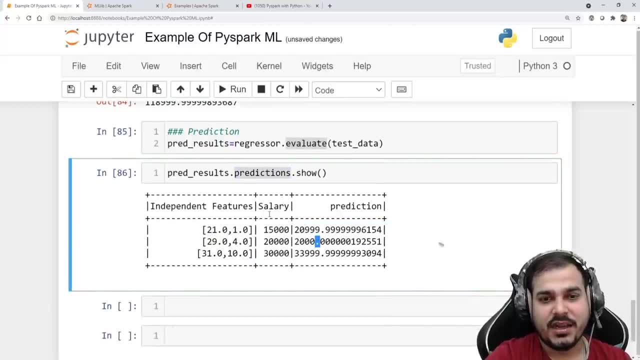 the output, and inside this, there will be a prediction variable which will have the, a prediction variable which will have the, a prediction variable which will have the output. okay, so this is my prediction output. okay, so this is my prediction output. okay, so this is my prediction. this is my salary. the real value, this is. 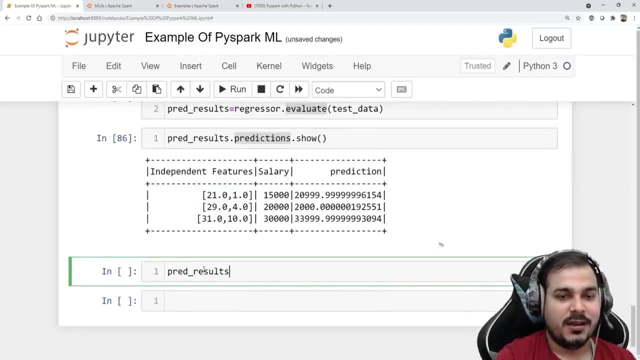 this is my salary, the real value. this is: this is my salary, the real value. this is my other thing now, if i really want to my other thing now, if i really want to my other thing now, if i really want to find out the find out the other important parameters or metrics. 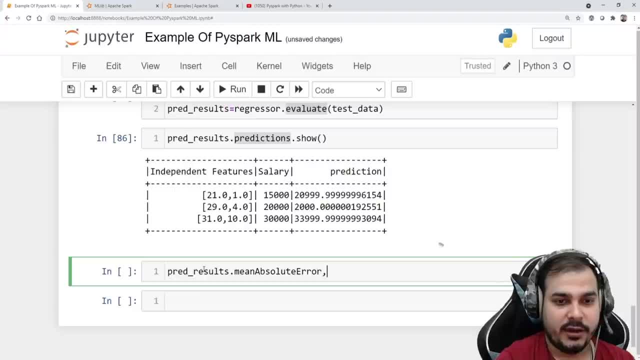 other important parameters or metrics. other important parameters or metrics. let's press tab here, you'll be able to. let's press tab here, you'll be able to. let's press tab here, you'll be able to see mean absolute error: um spread. see mean absolute error: um spread. 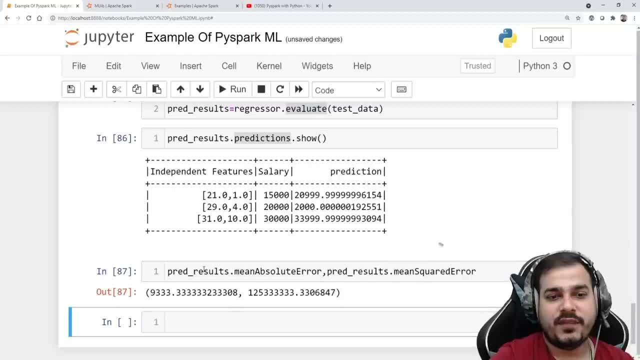 see mean absolute error. um spread. underscore result: dot mean squared error. underscore result: dot mean squared error. underscore result: dot mean squared error. suppose if i do see this particular word, suppose if i do see this particular word, suppose if i do see this particular word value, you'll be able to understand that. 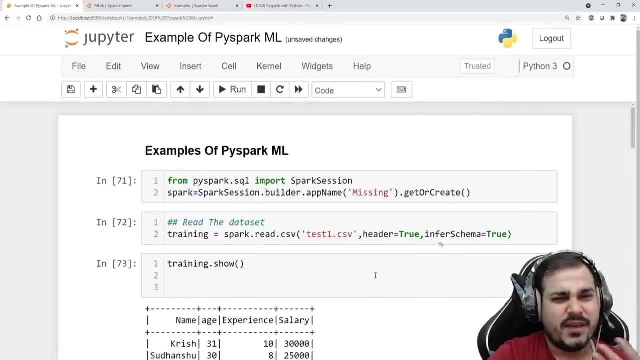 value. you'll be able to understand that value. you'll be able to understand that how the model is actually performing, so how the model is actually performing, so how the model is actually performing. so that's just a very. that's just a very, that's just a very, a very simple example. guys, don't worry. 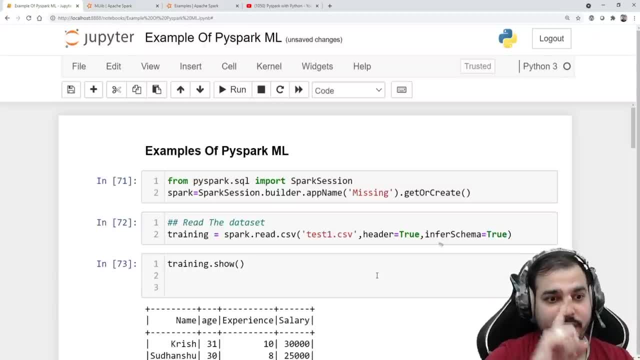 a very simple example, guys, don't worry. a very simple example. guys, don't worry, i'll be explaining you in depth. i'll be explaining you in depth. i'll be explaining you in depth, probably in the upcoming videos. when- probably in the upcoming videos, when- probably in the upcoming videos- when we'll be starting from linear regression. 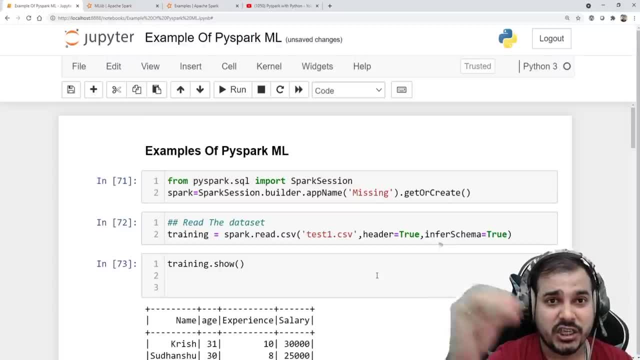 we'll be starting from linear regression. we'll be starting from linear regression now. remember, the next video is about now. remember, the next video is about now. remember, the next video is about linear regression implementation: in-depth linear regression implementation. in-depth linear regression implementation. in-depth implementation. right to help you know. 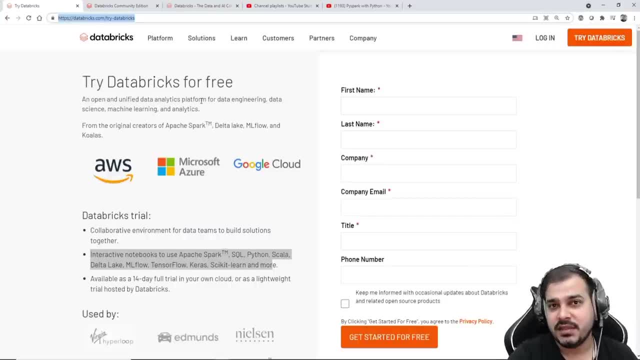 implementation right to help you know implementation right to help you know what exactly is a databricks platform. what exactly is a databricks platform? what exactly is a databricks platform? and this is an amazing platform where- and this is an amazing platform where- and this is an amazing platform where you can actually use. 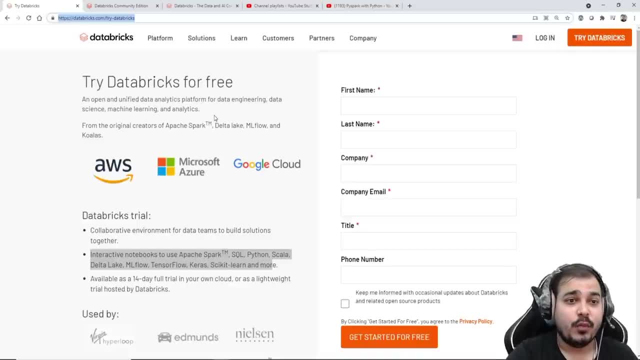 you can actually use. you can actually use spy spark. or you can work with apache spark- spy spark, or you can work with apache spark- spy spark, or you can work with apache spark. and one more amazing thing about this, and one more amazing thing about this and one more amazing thing about this particular platform, is that they also 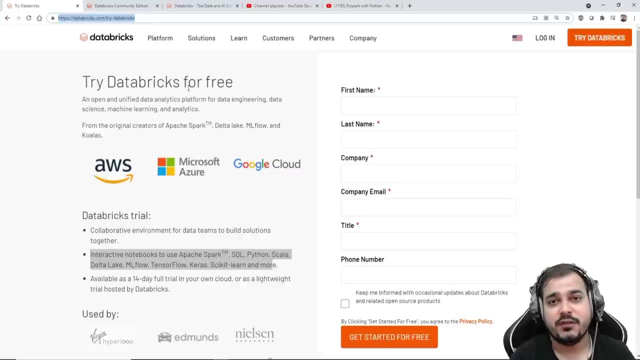 particular platform, is that they also particular platform is that they also provide you, provide you, provide you cluster instances. so suppose if you have cluster instances. so suppose if you have cluster instances, so suppose if you have a huge amount of data set, a huge amount of data set. 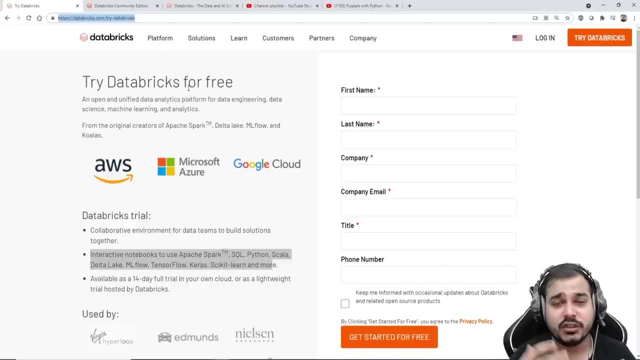 a huge amount of data set. probably you want to distribute the. probably you want to distribute the. probably you want to distribute the parallel processing, or probably want to parallel processing, or probably want to parallel processing, or probably want to distribute it in multiple clusters. you distribute it in multiple clusters. you. 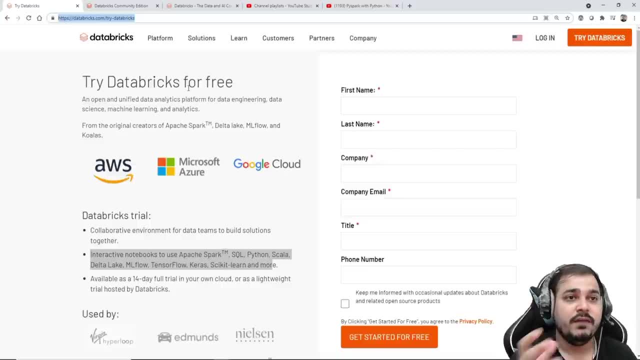 distribute it in multiple clusters. you can definitely do with the help of, can definitely do with the help of, can definitely do with the help of databricks, databricks, databricks. now, if i really want to use this now, if i really want to use this now, if i really want to use this particular platform, there are two ways. 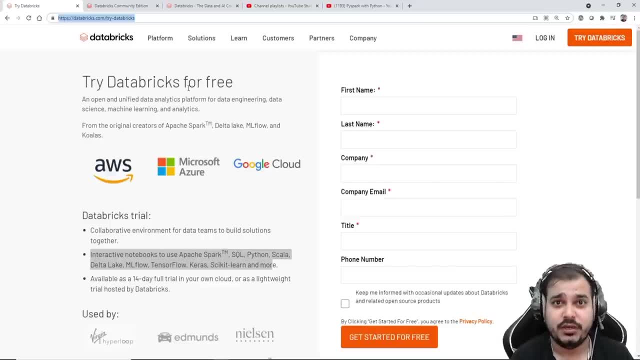 particular platform: there are two ways. particular platform: there are two ways: one is for community version and one is one is for community version and one is one is for community version and one is for the paid version, which is like azure. for the paid version, which is like azure. 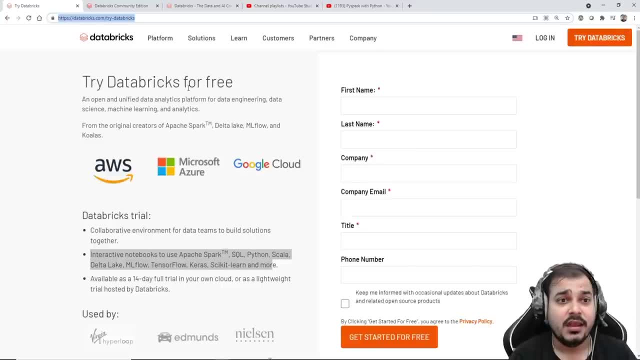 for the paid version, which is like azure or aws cloud. you can actually use in the or aws cloud. you can actually use in the or aws cloud. you can actually use in the backend, backend, backend. uh databricks also helps you to, uh databricks also helps you to. 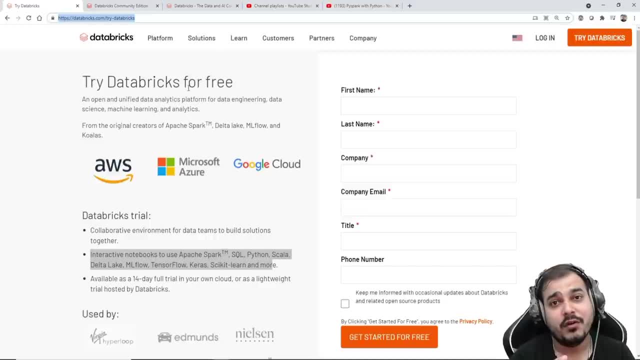 uh databricks also helps you to implement ml flow. okay, and this ml flow implement ml flow, okay. and this ml flow is with respect to the cicd pipeline, so is with respect to the cicd pipeline, so is with respect to the cicd pipeline, so you can also perform those kind of. 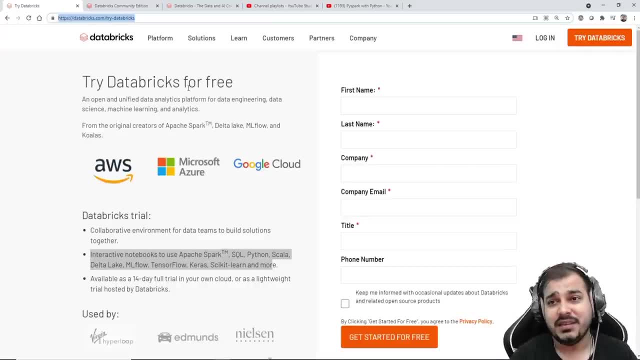 you can also perform those kind of. you can also perform those kind of experiments also. experiments also, experiments also. all together an amazing platform. what i all together an amazing platform. what i all together, an amazing platform. what i will be focusing in my uh youtube will be focusing in my uh youtube. 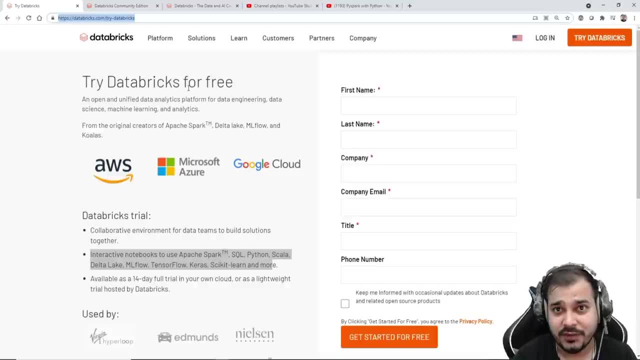 will be focusing in my uh youtube channel. is that i will try to show you channel? is that i will try to show you channel? is that i will try to show you, both with the community version also and both with the community version also, and both with the community version also, and in the upcoming videos we'll try to. 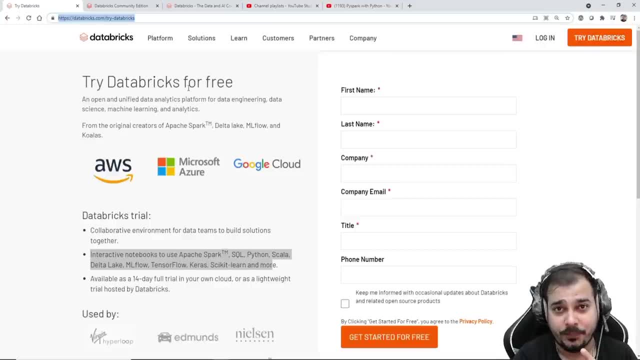 in the upcoming videos, we'll try to. in the upcoming videos, we'll try to execute, execute, execute, try to execute with both aws and azure. try to execute with both aws and azure. try to execute with both aws and azure. when we are using aws and azure, what? 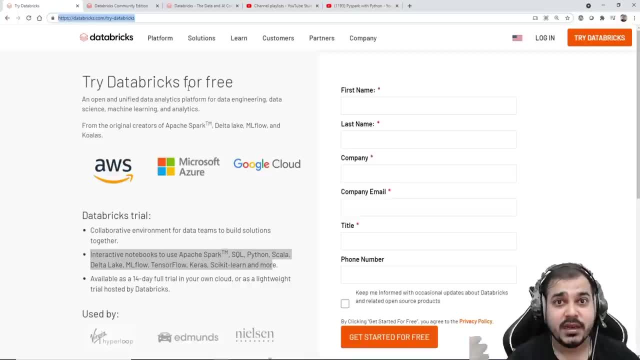 when we are using aws and azure. what when we are using aws and azure? what we'll try to do is that, whenever we we'll try to do is that whenever we we'll try to do is that, whenever we create the instances, multiple instances, create the instances, multiple instances. 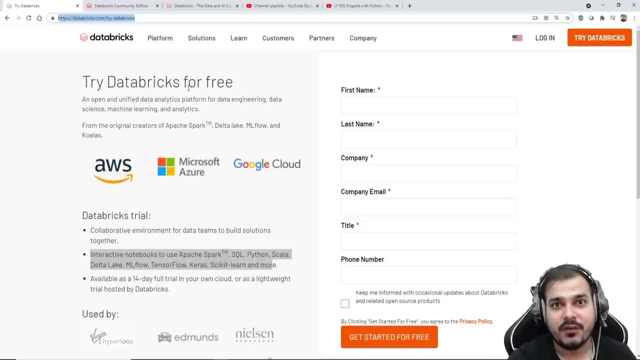 create the instances, multiple instances. you know that we'll try to create in. you know that we'll try to create in. you know that we'll try to create in this particular cloud platform. we'll this particular cloud platform, we'll this particular cloud platform. we'll also try to pull the data from s3. 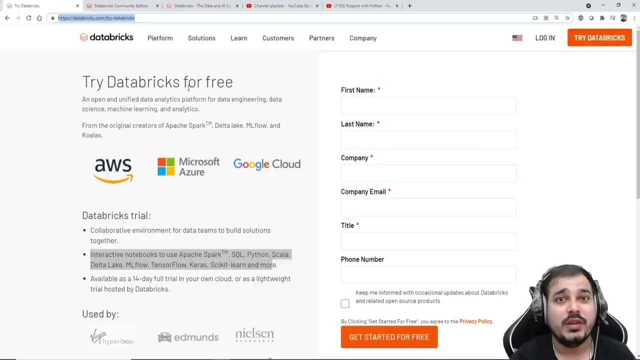 also try to pull the data from s3. also try to pull the data from s3 bucket, which is the storage unit in aws bucket, which is the storage unit in aws bucket, which is the storage unit in aws, and try to show you that, how we can work. 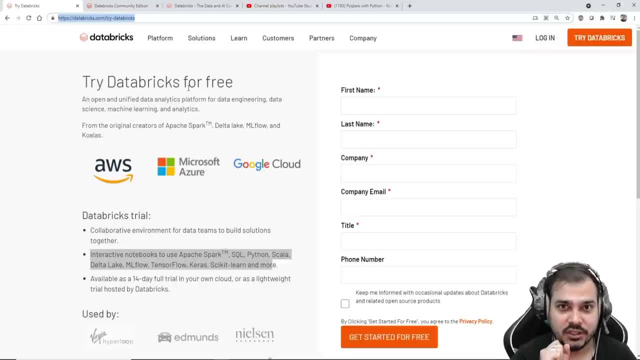 and try to show you that how we can work, and try to show you that how we can work with huge, huge data sets, with huge, huge data sets, with huge, huge data sets. right, all those things will be actually right. all those things will be actually right. all those things will be actually showed as we go ahead. 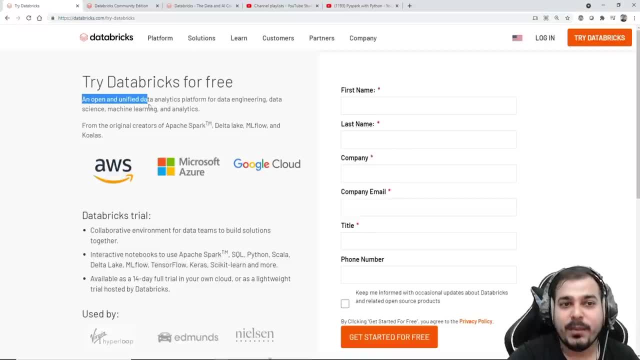 showed as we go ahead. showed as we go ahead. now let's understand what this databricks. now. let's understand what this databricks now. let's understand what this databricks is. it is an open and unified data. is it is an open and unified data? is it is an open and unified data analytics platform for data engineering. 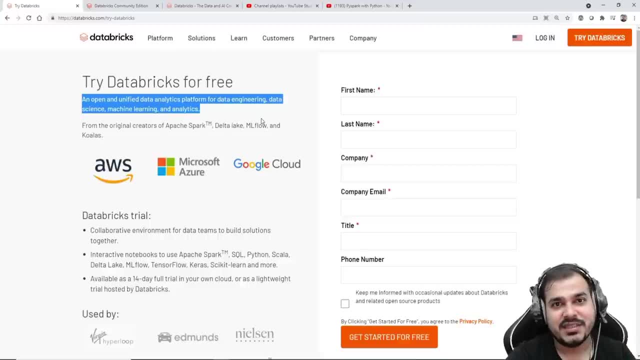 analytics platform for data engineering. analytics platform for data engineering, data science and machine learning, data science and machine learning, data science and machine learning. analytics. remember guys, databricks. analytics platform for data engineering. analytics, platform for data engineering. do it, and probably it supports three. do it, and probably it supports three. 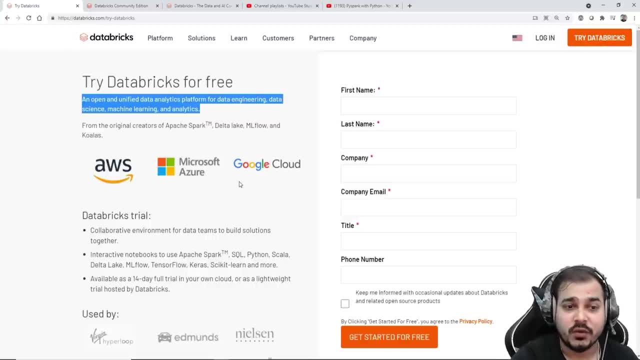 do it and probably it supports three kind of platform cloud platforms. one is kind of platform cloud platforms. one is kind of platform cloud platforms. one is aws- microsoft azure and google cloud. aws, microsoft azure and google cloud. aws, microsoft azure and google cloud. now, if you really want to start, 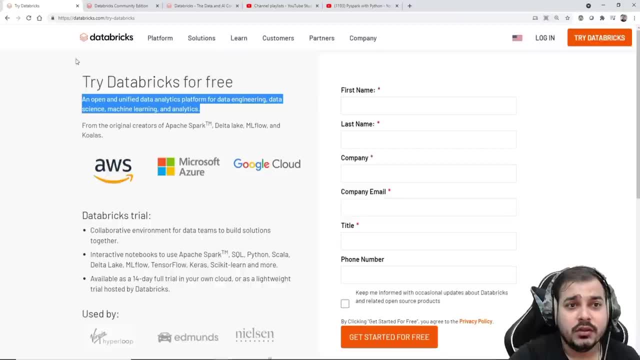 now. if you really want to start now, if you really want to start, start with this, we'll start with the start with this. we'll start with the start with this. we'll start with the community version, community version, community version, and you just have to go into this. 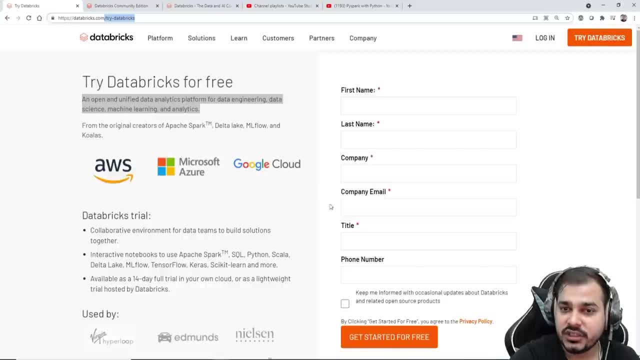 and you just have to go into this. and you just have to go into this particular url and just type try particular url and just type try particular url and just type: try databricks. and then you just enter all your details to get registered for free. now, once you are registered, when you, once you get started, 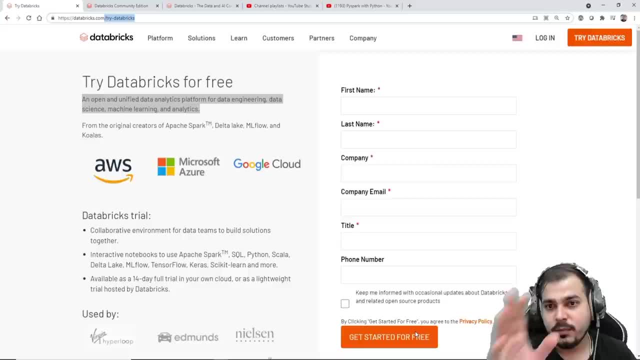 for free. you'll get two options over there. on the right hand side, you'll be seeing the community version, which you really want to use it for free, and in the left hand side, you will be having an option where they'll tell you that you need to work with this three cloud platforms and you can. 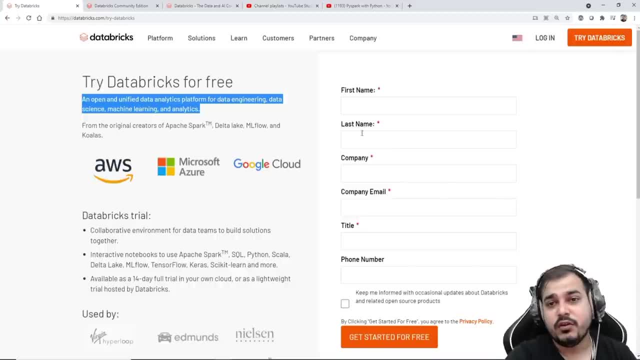 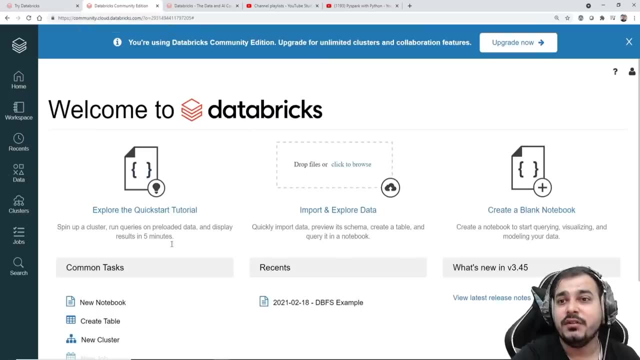 select that also. so for right now, i will try to show you a community version, which will be very simple, very, very easy. so let's go to the community version. so this is how the community version actually looks like. if you really want to go into the cloud version, you just, you can just click on. 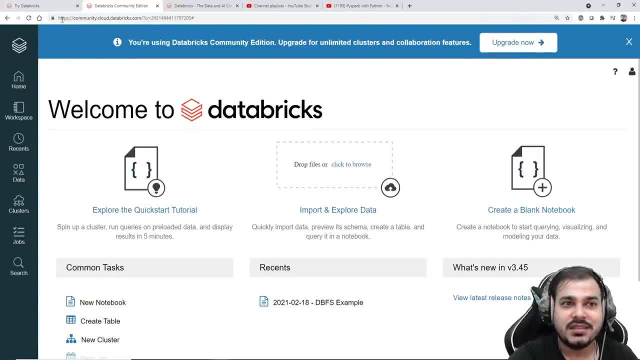 upgrade. okay, so just click on upgrade and this is the url of the community version, and this version of this url you'll be able to get when you register for the community version tomorrow. you think that you probably want to work with the cloud. you just have to click on this upgrade now. 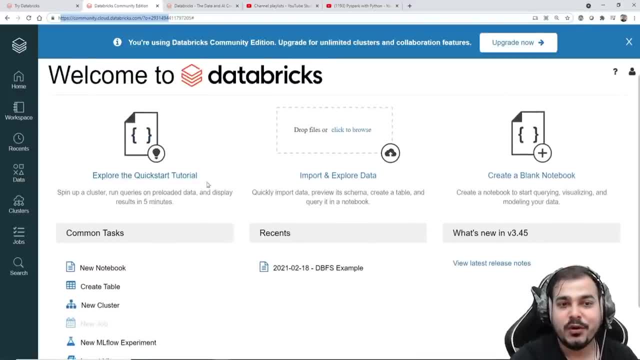 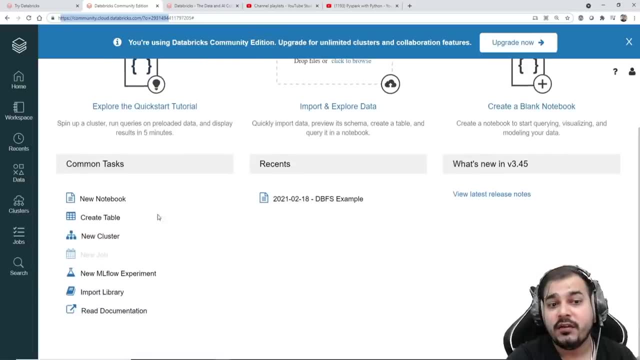 now. in this you'll be able to see three things. one is explore to the. explore the quick start tutorial, import and explore data, create a blank notebook and many more things over here- what all kind of tasks you'll be able to do in the community version one. 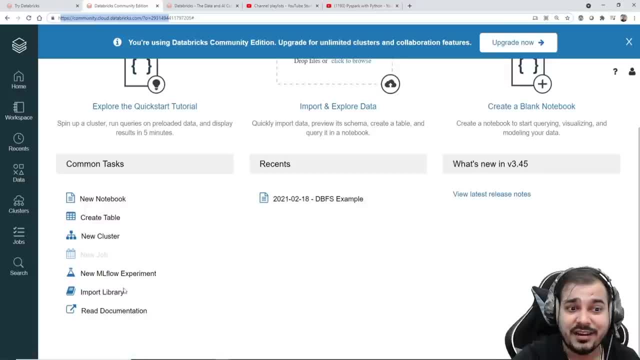 is: you can create a new notebook, you can create a table, create a cluster, create new ml flow experiments. i hope i have actually showed you ml flow experience. we can also create this ml flow experiment, uh, by combining uh to a database in the backend. okay, then we can import libraries. 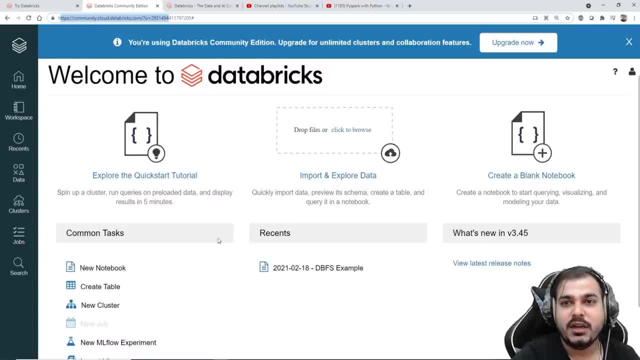 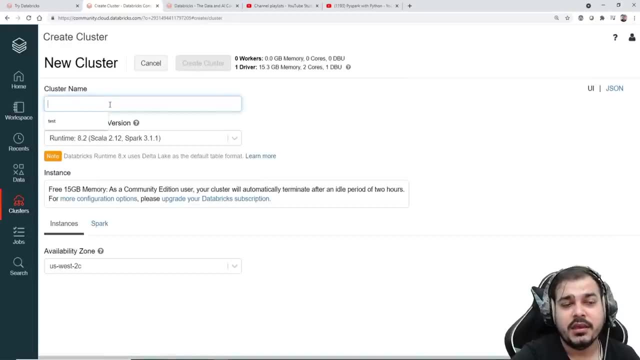 read documentation, do a lot of tasks now. first of all, what we need to do is that probably i'll create a cluster. now, in order to create a cluster, i will click on this: create a cluster. here you can basically just write down any cluster name. suppose i'll say apache, or i'll just say 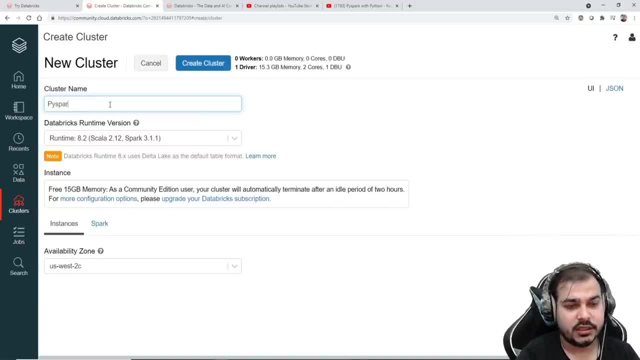 pi spark cluster. suppose this is my cluster that i want to basically create? okay, and then here by default- uh, over here you can see 8.2 scalar. this one, spark 3.1.1, is selected. so we'll be working with spark 3.1.1. if you remember, in my local also, i actually created a cluster and i'll 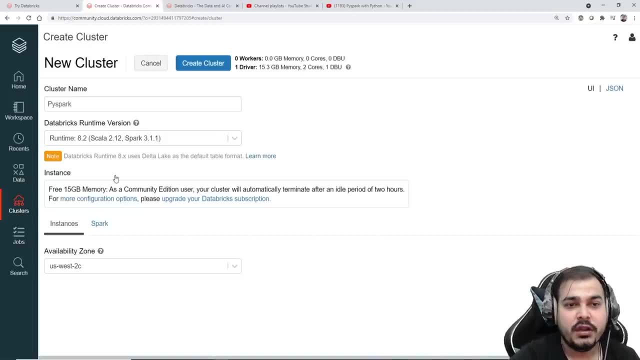 install this particular version only. okay, by default. uh, you'll be able to see that they will be providing you one instance with 15 gb memory and some more configuration. if you really want to upgrade your configuration, you can basically go and click over here. okay, and remember, in the free. 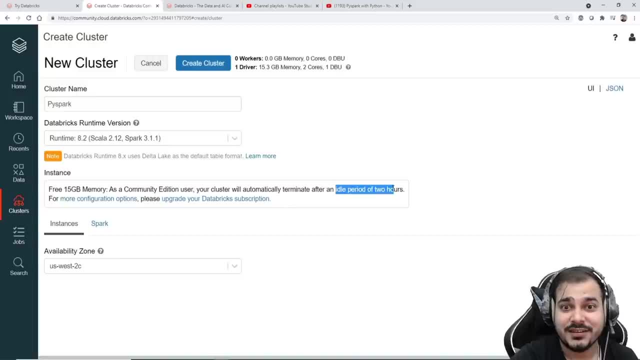 version. you will be able to work in an instance unless and until it is not idle for two hours, otherwise it will get disconnected. so over here you can see one driver: 15.3 gb memory, two cores- all these things are there. you can also understand what dbu is. dbu is nothing but a data. 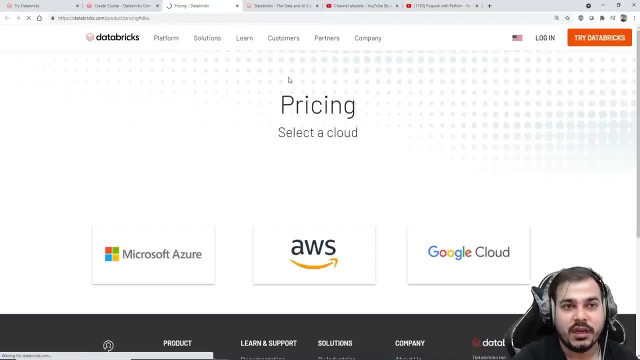 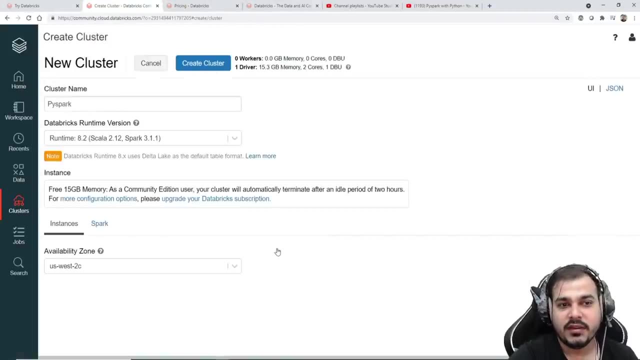 bricks unit. if you want to click over here, you'll be able to understand what exactly dbu is okay, and you'll be able to select a cloud and basically work with that. perfect till here. everything is fine. let's start. let's create the cluster now. once you, you will be seeing that the cluster 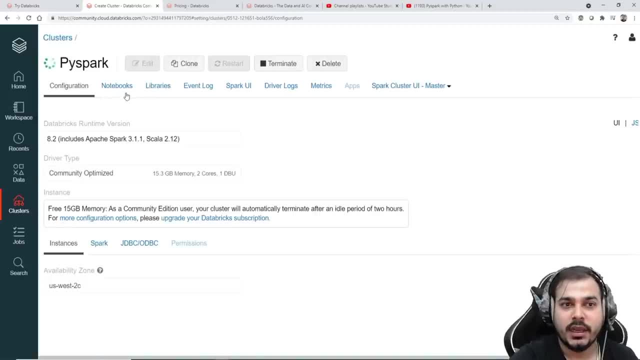 is basically getting created. you also have a lot of options over here, like notebook libraries, event logs, spark ui driver logs and all. it's not like you just have. you'll be able to work with python over here here. you have a lot of options, okay. so suppose, if 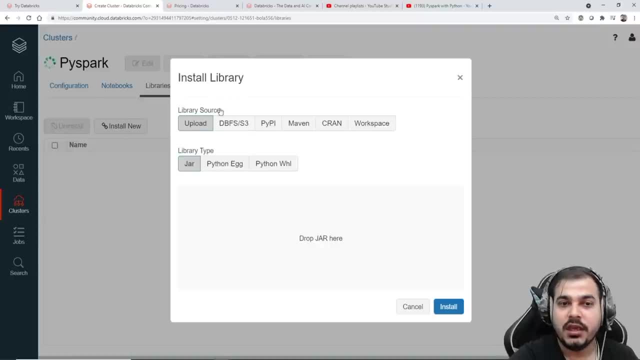 i go and click on libraries and if i click on install new, here you will be having an option to upload the libraries. you can also install the libraries from pi pi, from maven, which we basically use along with java, and then you have different, different workspace. so here what i'm going to do. 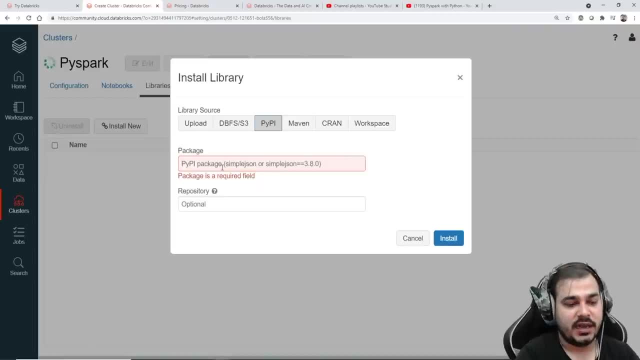 is that? suppose, if you select pi pi and suppose you want to install some of the libraries like tensorflow, or probably you want to go with keras, you can basically write like this: probably i want sk learn, you know. so i can just give comma separated and start installing them. 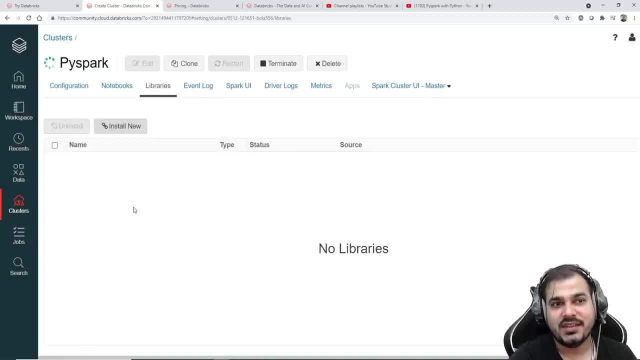 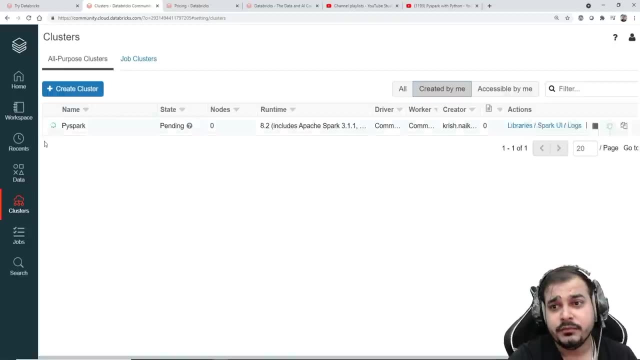 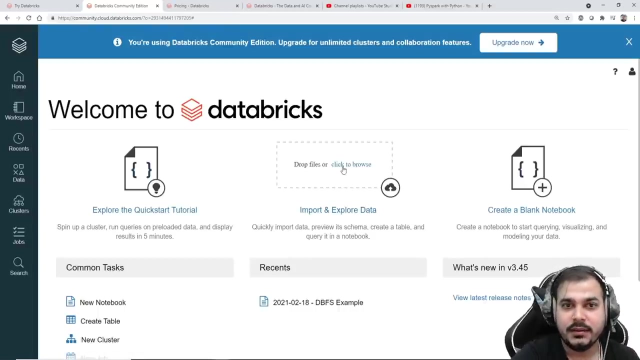 okay, but by default, i know i'm going to work with pi spark, so i'm not going to install any libraries, so let's see how much time this will probably take. this is just getting executed over here and let's go back to my home. so, apart from this, here you'll be also able to upload the data set. 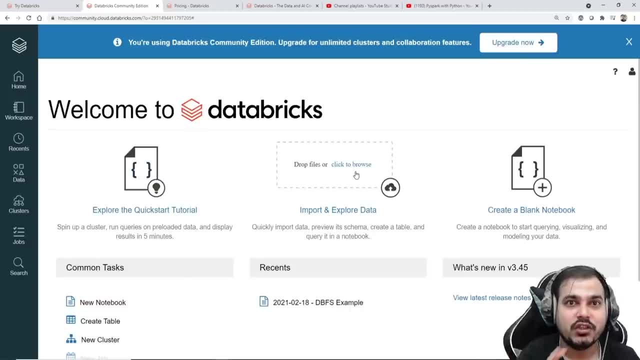 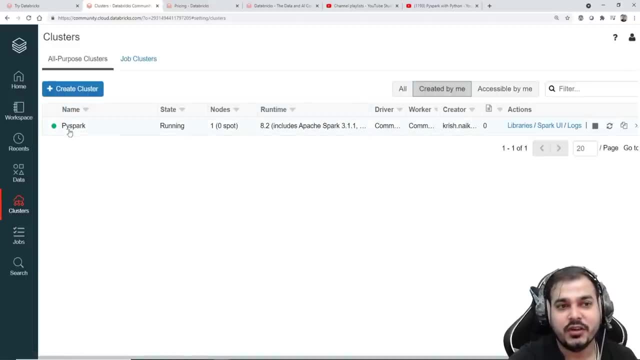 and that particular data will give you an environment like how you're storing the data in the do. okay, so before the cluster is getting created. okay, now the cluster has got created. here you can see pi spark, it is in running state now. and remember, this cluster only has one instance if 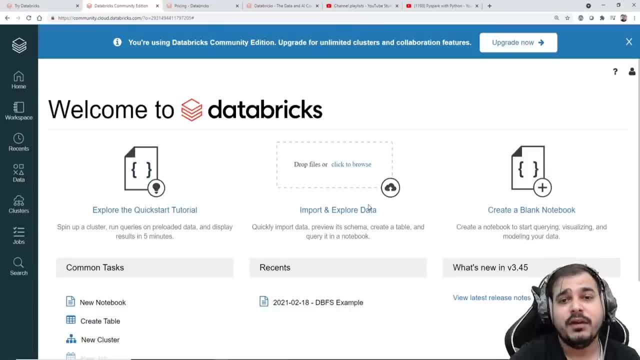 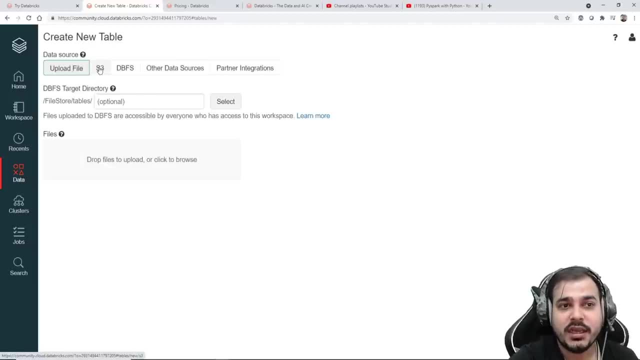 you want to create multiple clusters, we have to use the cloud platform, one which will be chargeable, okay, so here i'm going to click on export the data. now see, guys, you can upload the data. you can also bring from s3 bucket. okay, you can also, then, bring from s3 bucket. 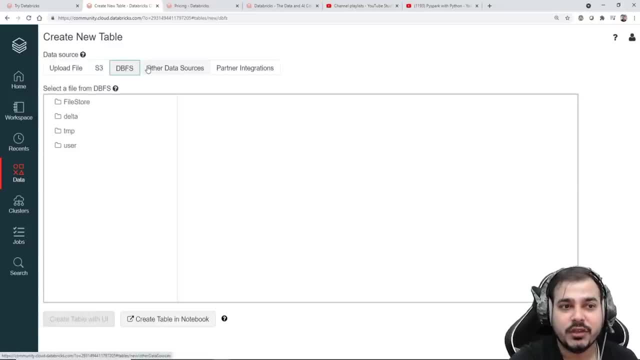 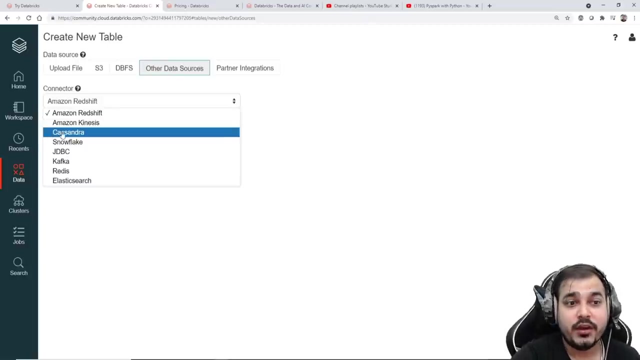 these all things i'll try to show you. then you also have dbfs, you know, and dbff you will basically be storing inside this particular format. then you have other data sources like amazon redshift, amazon kinesis. amazon kinesis is basically used for live streaming data. okay, then you have cassandra. 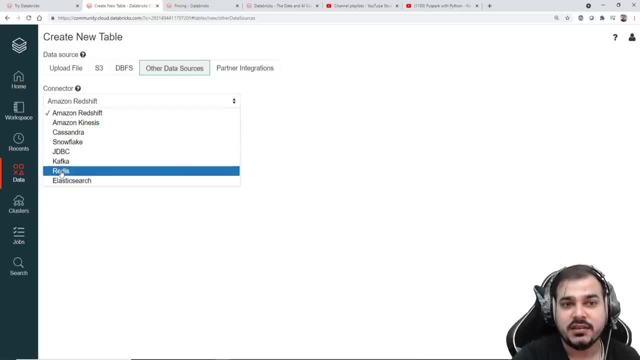 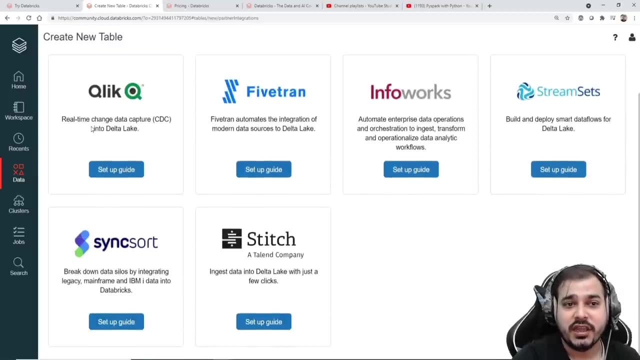 cassandra is also a no sql database and jdbc elastic search. so different, different data sets, data sources, are also there. we'll also try to see with respect to partners integration. so they are also like real-time capture, uh, in the delta lake and many more things are there. so you can definitely 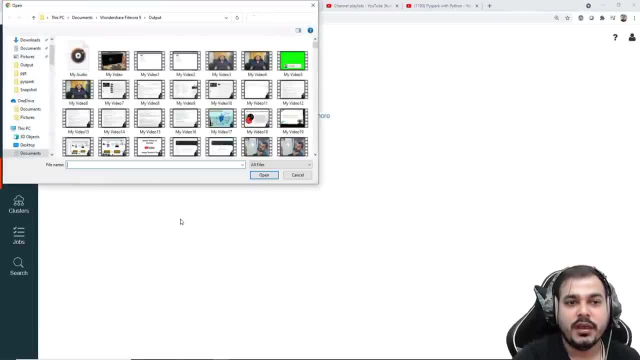 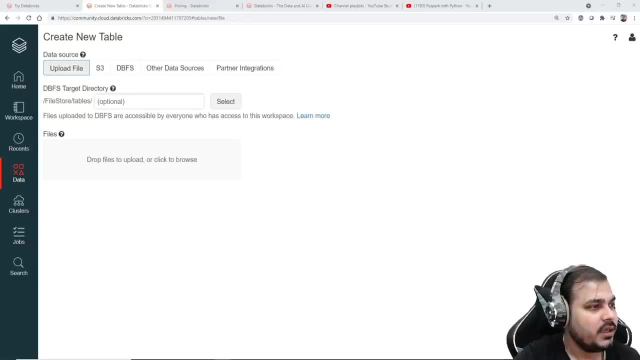 have a look onto this now. what i'm going to do is that i'm just going to click over here and try to upload a data. let me just see, let me just upload a data sets. i'll just go to my pi spark folder. so here is my pi sparks. well, i'm 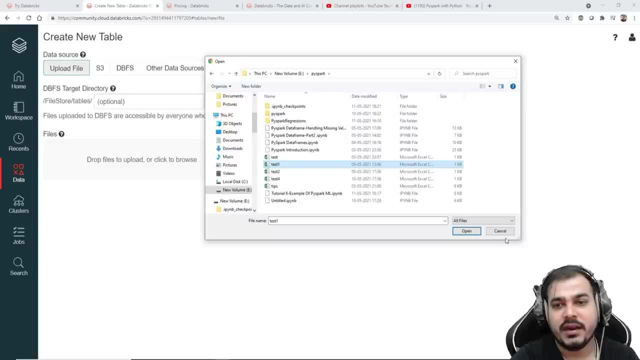 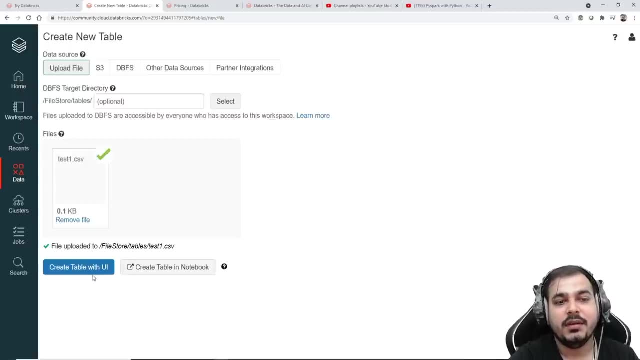 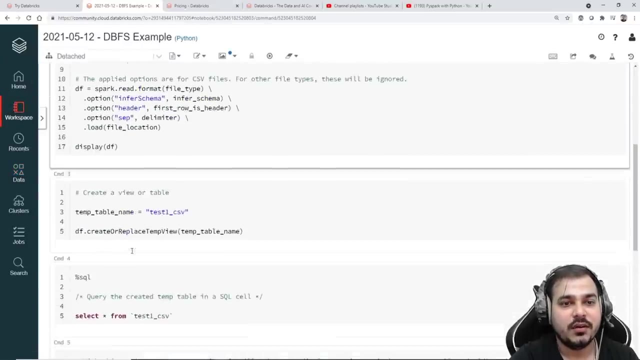 just going to upload this test data set, probably, or i'll try to upload this test one now. here you can see that the data set has been uploaded. now it is saying that: create table with ui, create table notebook, suppose if i go and click this, you know, so here you'll be able to see. this is the code. 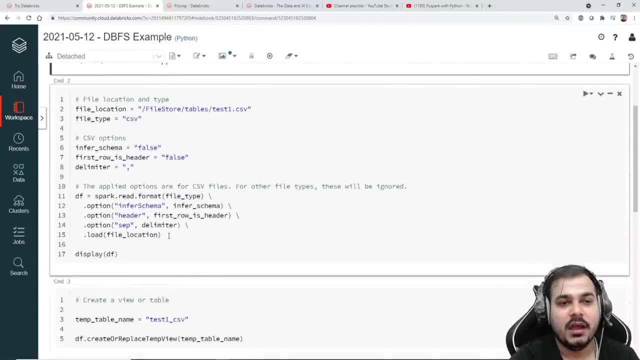 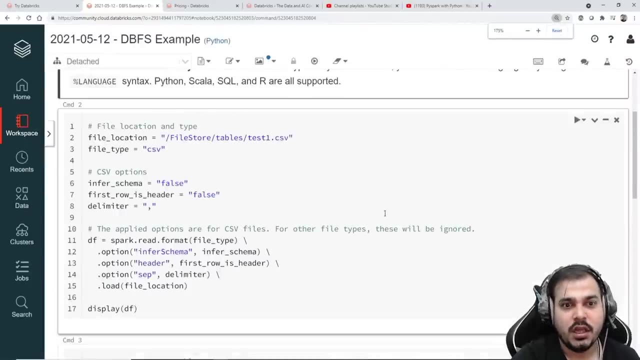 this is the entire code to basically create a table, uh, in the ui. but what i really want to do is that i don't want to create a table. instead, i'll just try to execute some of the pi spark code which we have already learned till now. okay, so what i'm going to do? i'll just remove this. i. 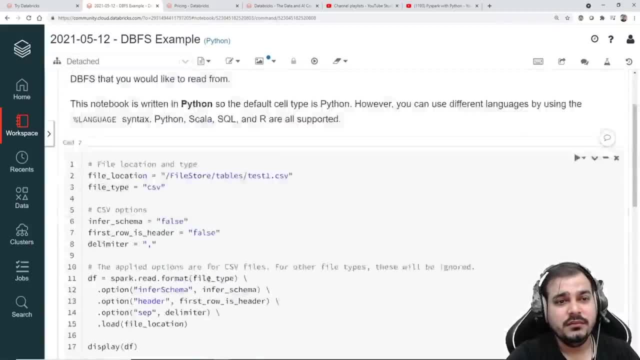 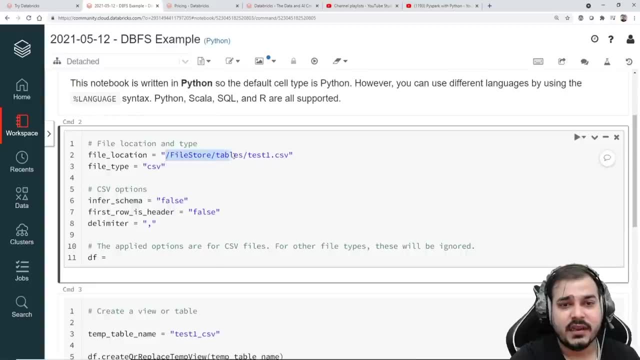 don't want it, i'll remove this, okay. okay, let me read the data set now. for reading the data set, you'll be able to see that my data set path is basically this: it is a csv file, infer, schema, header, schema. all these things are there, so let me remove this also. so let me start. 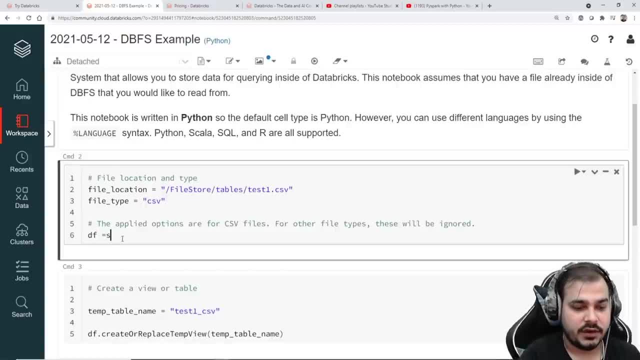 reading the data set. so by default spark is already uploaded, so i'll write spark dot, spark dot read dot csv. i hope so it will work. and for the first time, remember this is my file location. file location- okay, file underscore location. and then i will also be using two more option. 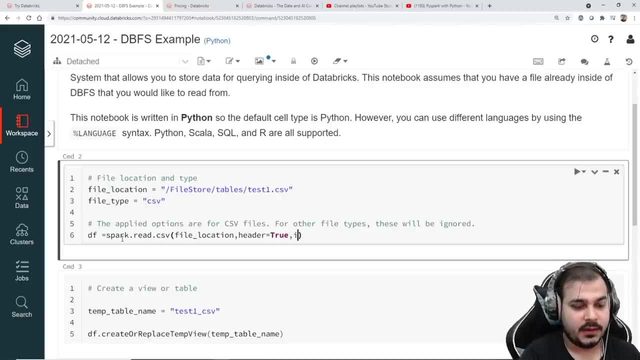 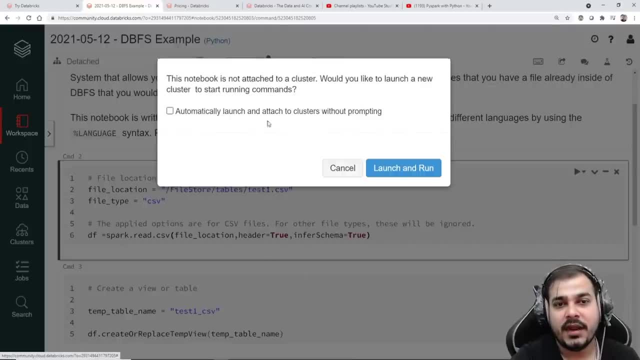 one is header is equal to true and then i have infer schema is equal to true. so once i execute this now, you will be seeing that automatically the first time. when you're executing, it will say that launch and run. so we are going to launch the cluster and run it, so i'm just going to click it. 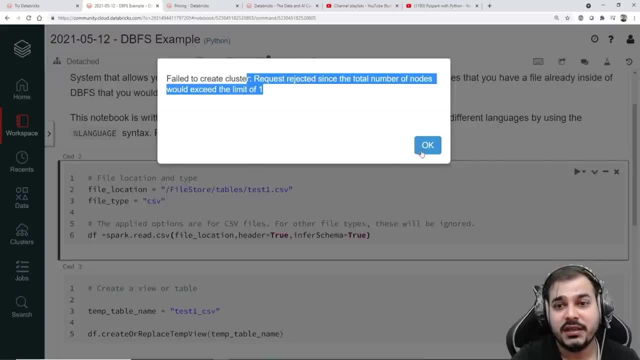 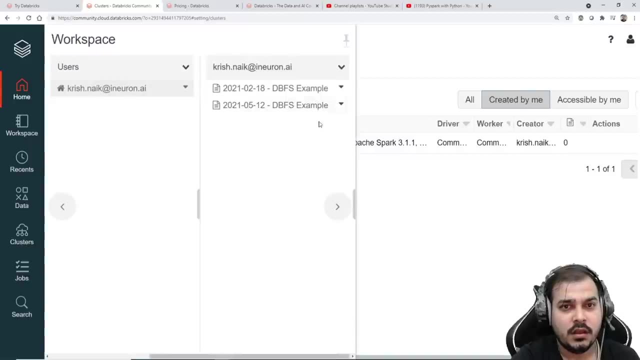 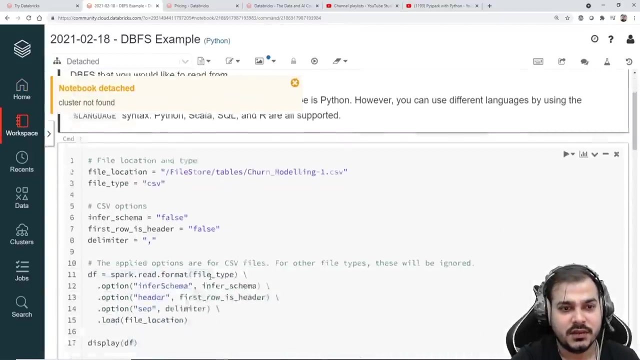 fail to create reject request, since the total number of nodes would exit the limit one. why this is there? let's see our clusters. we just have one cluster, uh. okay, there were some examples. uh, that has been taken over here, so let me remove one of them. okay, let me just execute this. 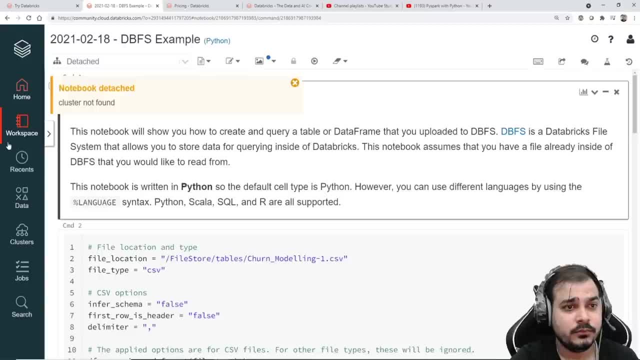 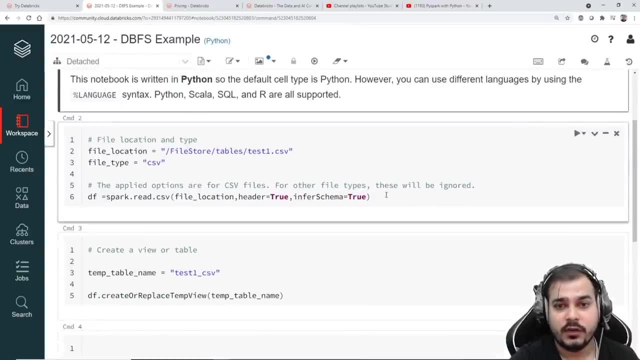 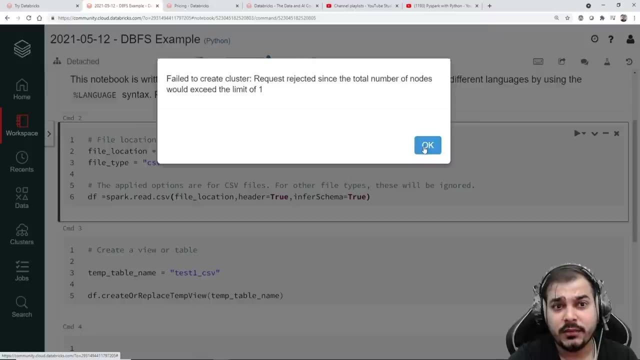 okay, uh, i'll go over here space, let me delete it. okay, perfect, now i'll try to read this. let's see again. it says: fail to create the cluster. reject request rejected since the total number of nodes would exceed the limit of one and it is not allowing us to execute more than one file. i guess. 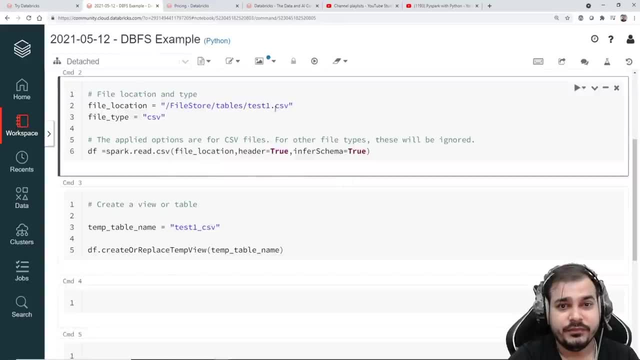 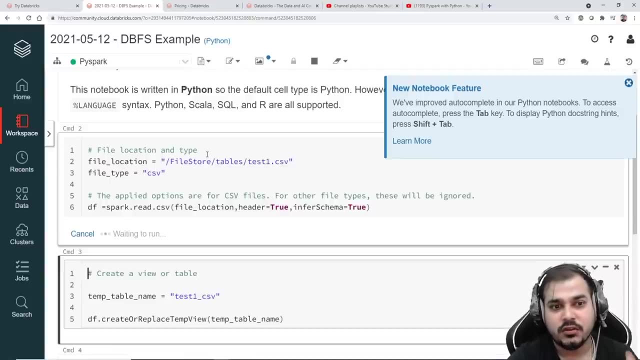 so because of that, i'm just reloading it. let's see now. now it has got executed. see, guys, before there were two files, so because of that, it was not allowing me to run, i just, really, i deleted one file and i i reloaded one file. okay, so now you. 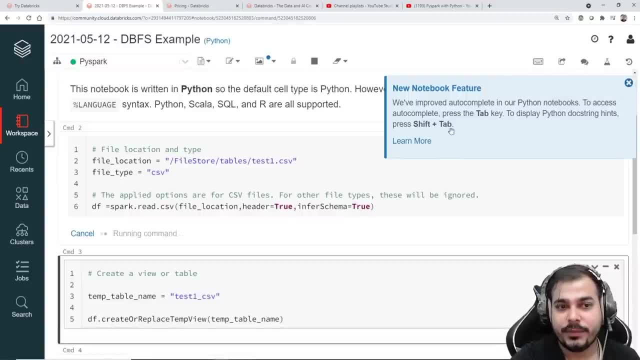 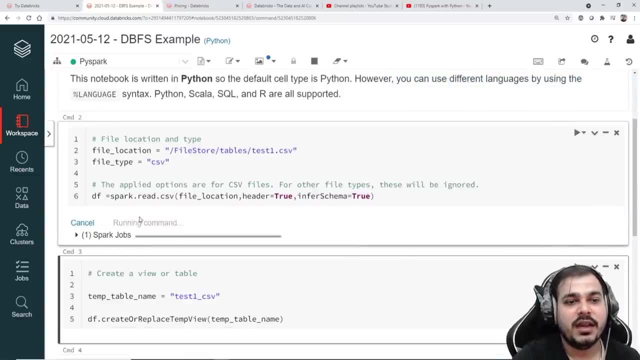 can see that it is getting run. so now you can see that it is getting run. so now you can see that it is getting run. now, okay, you can also press shift tab to basically see some hints and all same, like how we do it in jupyter notebook. now, here you will be able to see that my 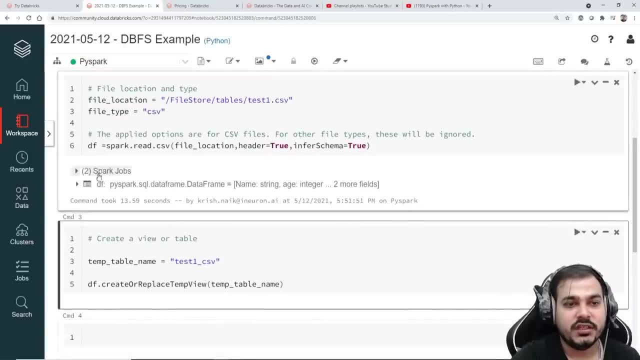 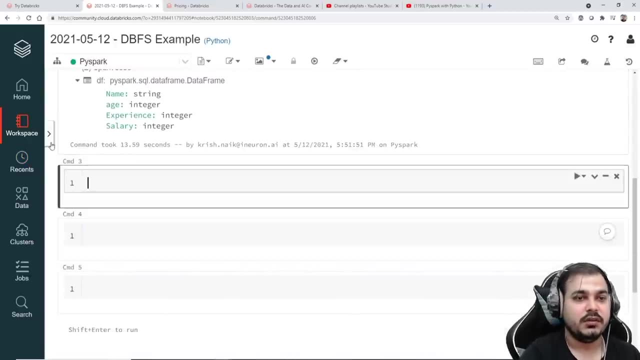 file will be running absolutely fine. and it shows. it shows this df, it shows that, okay, it is a pispark- dot sql, dot dataframedatafil. now let me just execute the other things. now suppose, if i want df dot print- see, i'm just using that tab, feature print schema. if i go and see this, 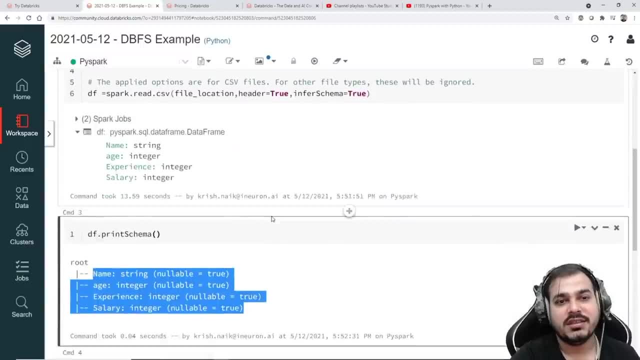 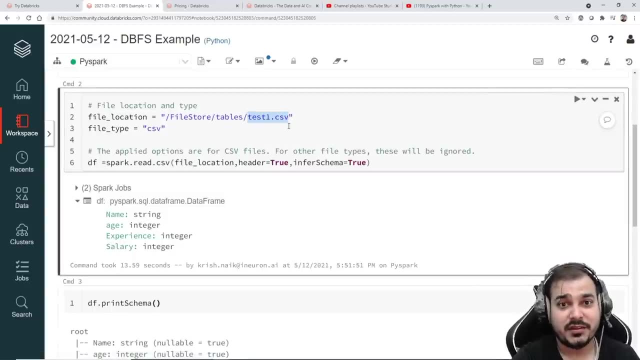 you'll be able to see, find out all the values, right? so, in short, this is basically now running in my instance of the cluster, right, i will be able to upload any huge data set, probably a 50 gb data set, also from s3 bucket, and all right, that i'll try to show you how we can do it from. 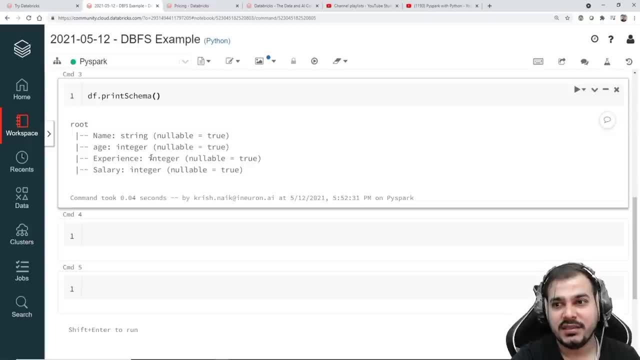 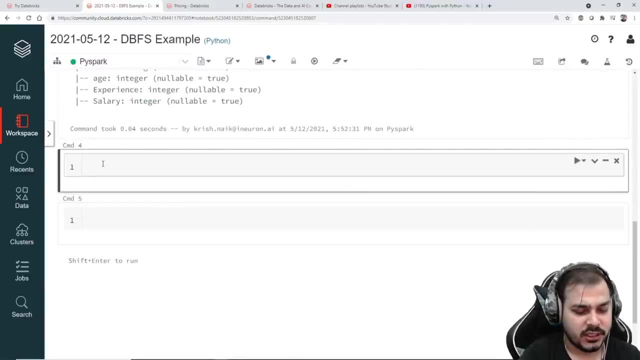 s3 bucket in the upcoming videos. but what i'm going to show you guys in the upcoming future will try to run all this kind of problem statements through the data brick so that you'll be able to learn it. okay, now let me just go and do one more thing. so this is my dfshow. okay, so this is my. 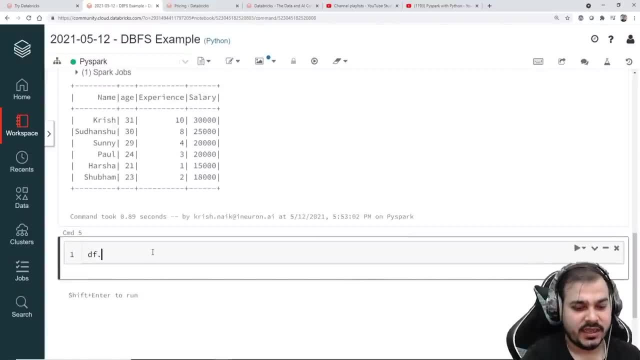 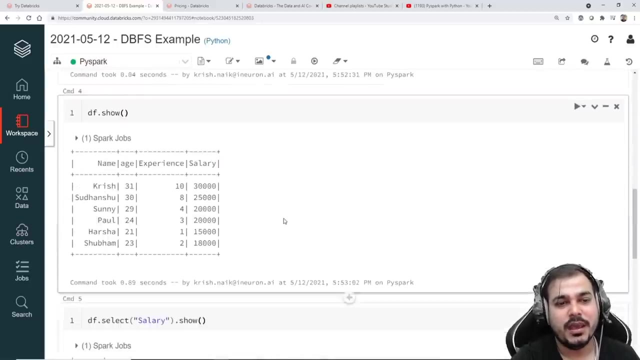 entire data set. so probably i will just want to select some column. i can actually write this dfselect, and here i just want to say salaryshow. i'm just selecting salaryshow. uh, here you'll be able to see. so, everything that you want to do, you'll be able to do it and remember, over here you'll be. 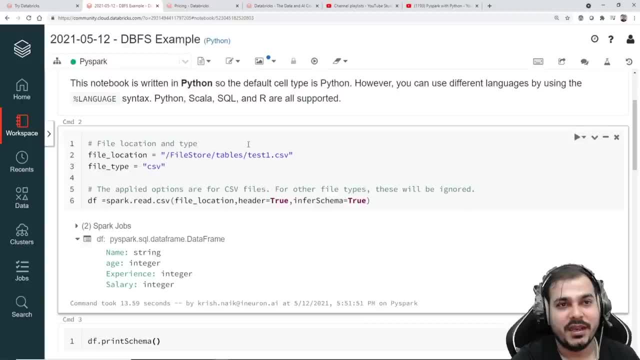 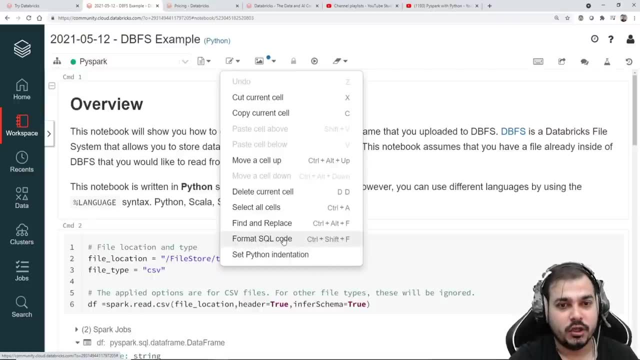 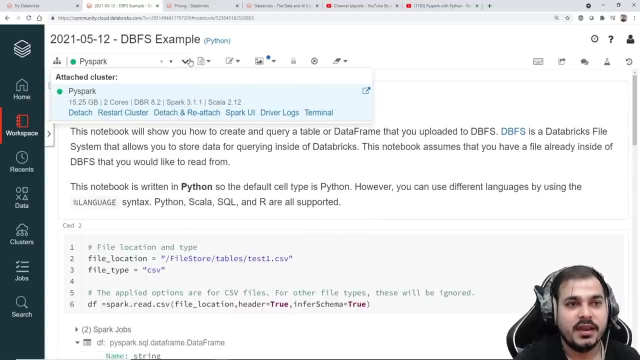 able to find out around 15- 15 and you can definitely perform any kind of things. okay, uh, here also you have same options, like how we have it in, uh, you know, in jupiter notebook. every option is there. you'll be able to find out all these particular options in jupiter notebook also. right, so this is basically running. 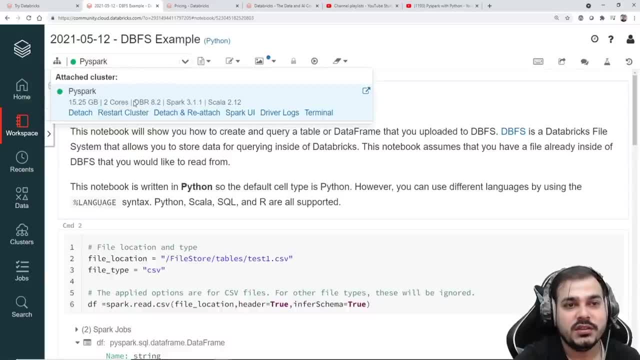 in 15.25 gb. uh, two cores. uh, okay, in that particular cluster you have two cores. then you have spark 3.1.1, spark 2.12 and you'll be able to see all this particular information. so what i would like to want, guys, please try to make a specific environment for you. 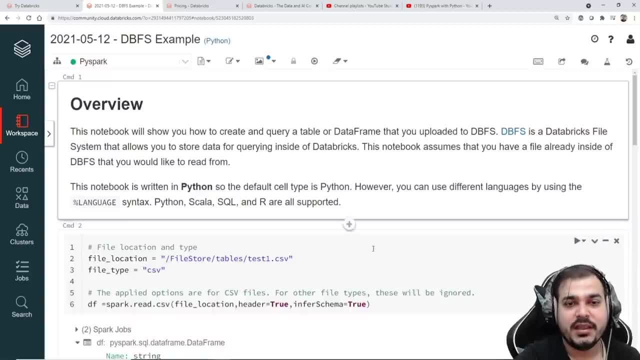 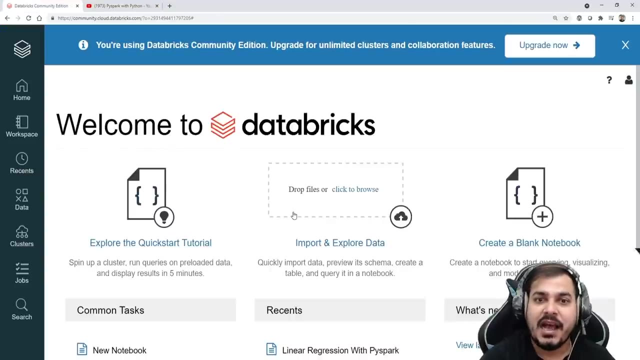 and then try to start it. uh, try to keep everything ready and from the upcoming videos we will try to see how we can execute, how we can implement uh problem statement, how we can implement different algorithms. i have already given you the introduction of databricks in the last class. i hope you have. 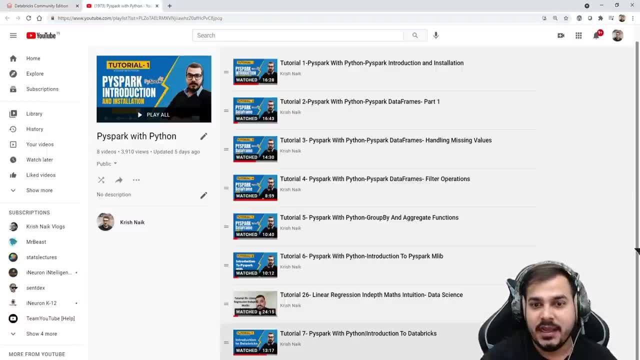 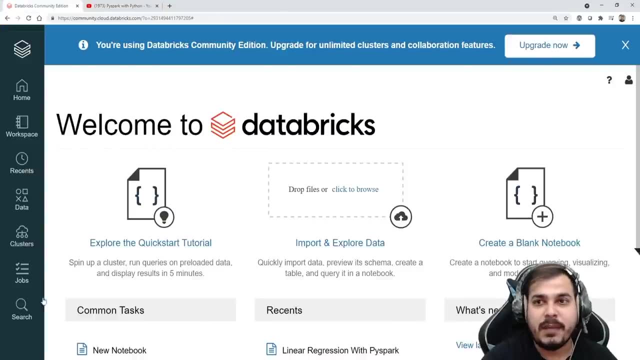 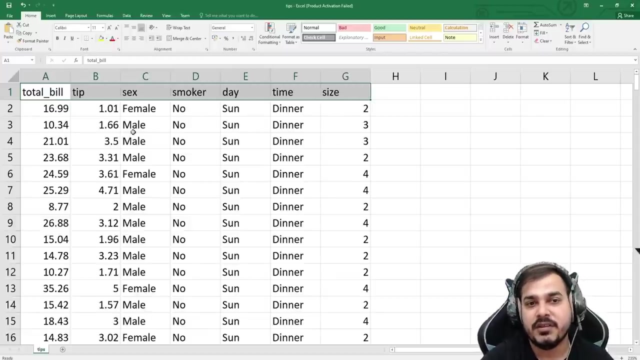 made your account and i hope you have started using it. if you don't know how to make an account, please watch the tutorial 7, the entire video, and i will see you in the next video. bye, bye, bye. so this is a multi-linear regression problem statement. here you have many, many features, right? so let's. 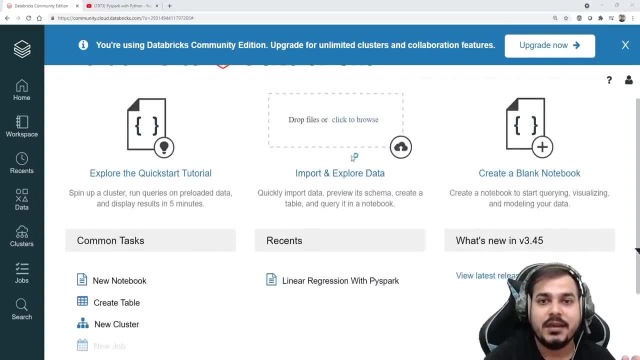 proceed now. first of all, what i'm going to do: i'm just going to click to the browse and i'm going to upload this particular problem statement and i'm going to go to the restaurant: what tip they have in that particular data set. now, in order to upload this particular data set, i have this particular data. 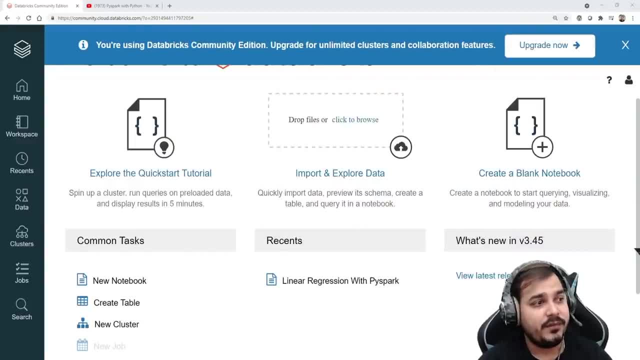 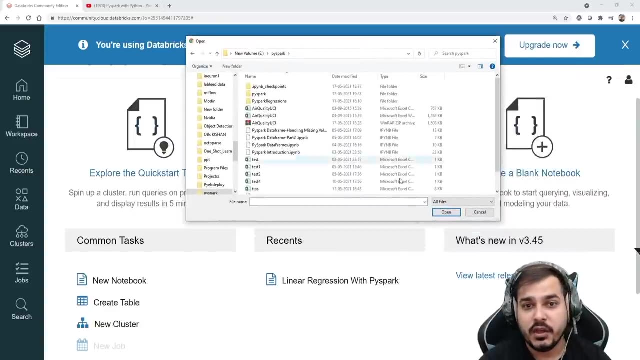 set in my path, so probably i'll also be giving you this particular data set, so don't worry about it. uh, let me just quickly just a second. let me just upload the data set over here, okay, by spark. okay. so here you can see that this is my data set, which i'm actually uploading tips, so let me open it. right now. here you'll be able to see that i've uploaded what's called a resting model. fine, when this is a restoring data set, which is kind of like an Calculator inside of the harvester product border, where everything is différents. so anyway, let's see how we can do the test, test, test, and i will just let you look these. it's like this: 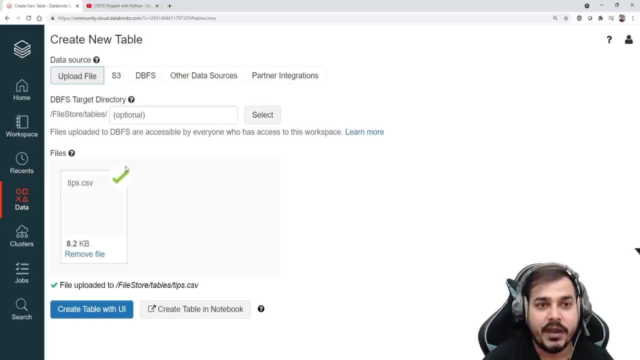 so here you can see that this is my data set, which i'm actually uploading tips. so let me open it right now. here you'll be able to see your tips. data set will get uploaded, you know, in this dbfs directory. so here you'll be having. 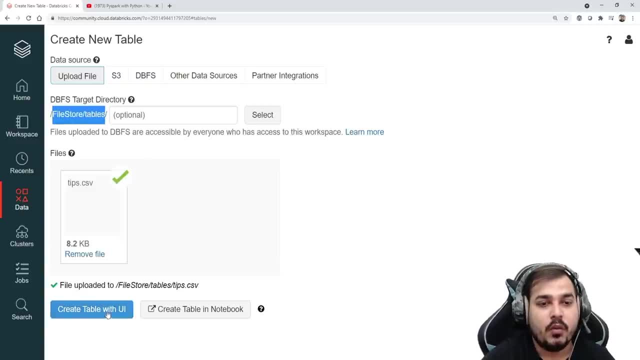 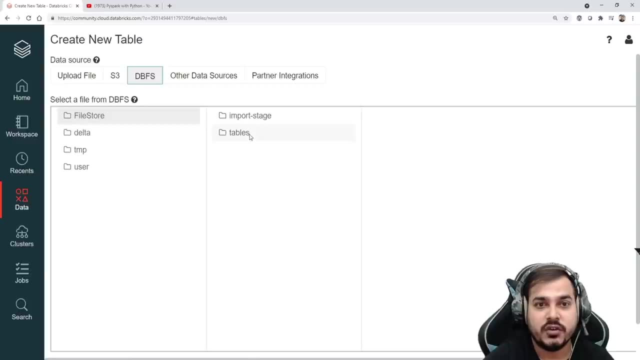 something like file stores, slash tables. okay, now, what you can actually do now. uh, let's go and click on this dbfs and here you can see on file stores. probably you can also click on tables. here you have this tipscsv. i've also uploaded these all data sets in my previous videos. uh, probably i was. 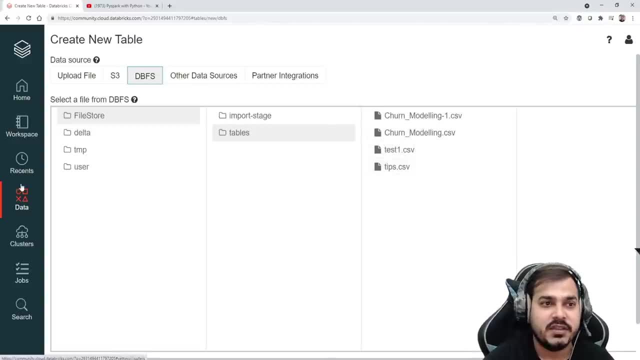 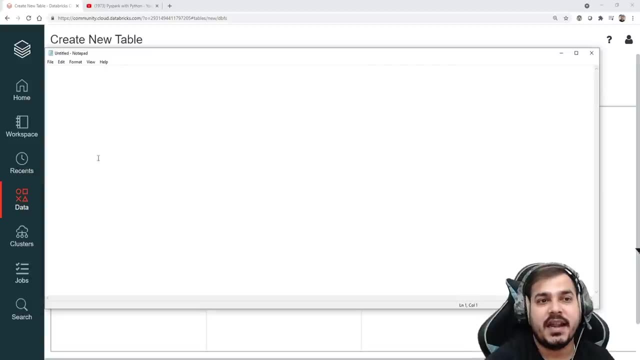 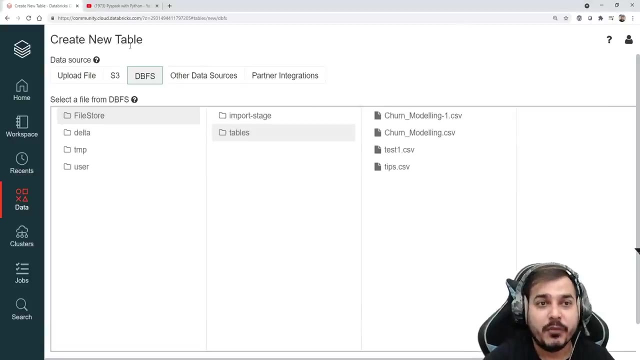 just using this? okay, but here i'm just focusing on tipscsv. now what i'm going to do over here, let's go and do the first step. remember: the first step in databricks is that we need to create the clusters. okay, create a cluster right now, by default in the community version databricks. 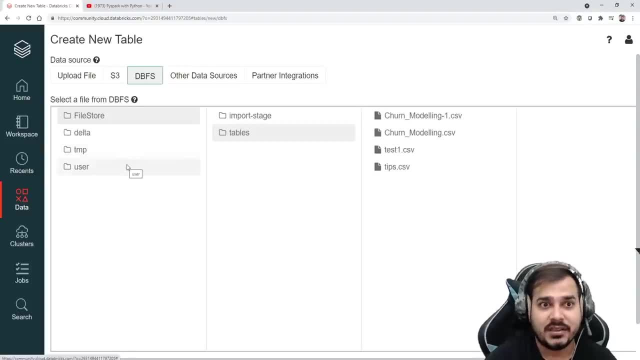 actually helps you to create a cluster. just one single cluster, okay, but if you are using the paid version, the upgraded version, it will actually help you to create multiple clusters if you have the access of adobe s cloud. so i'm just going to click on the cluster. let me create a new cluster. 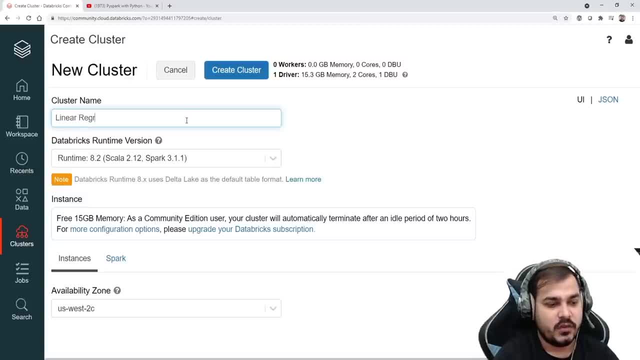 so i'll say: this is my linear regression cluster, okay, and then i'm going to use this runtime 8.2 scalar, this, this is there, and we're just going to click the cluster and remaining all things will be almost same in this cluster. in this instance, you'll be getting 15 gb memory and 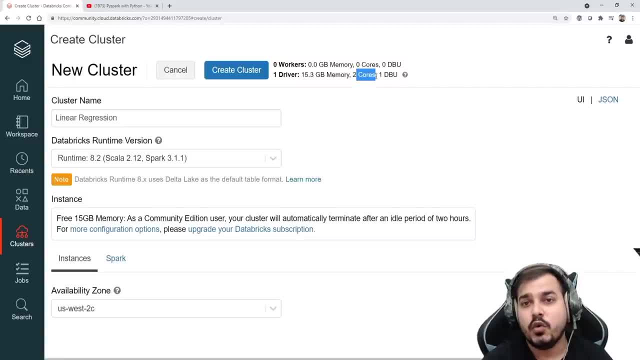 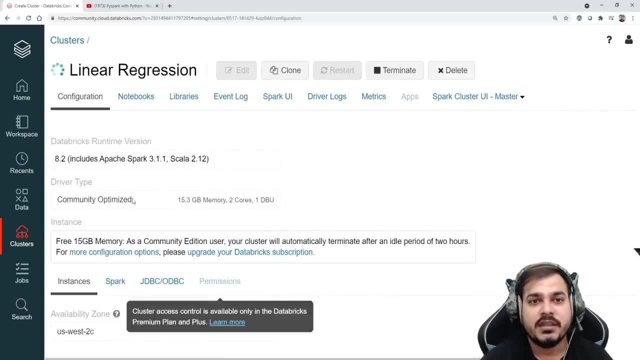 all the other information here. you can check it out. you can also be getting two cores and one uh i dbu okay, so, which i've actually already discussed in my previous session. so i'll go and click on cluster. this will take some time and remember, guys, if you really want to use any kind, 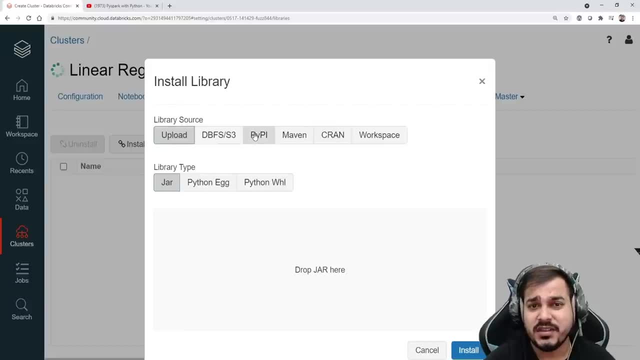 of libraries. just click over here, install those libraries which you want. like suppose, if you want to use seaborn, you want to use keras, you want to use tensorflow, so here you can basically type this along with the versions, and you'll be able to install it. okay, but right now i don't require. 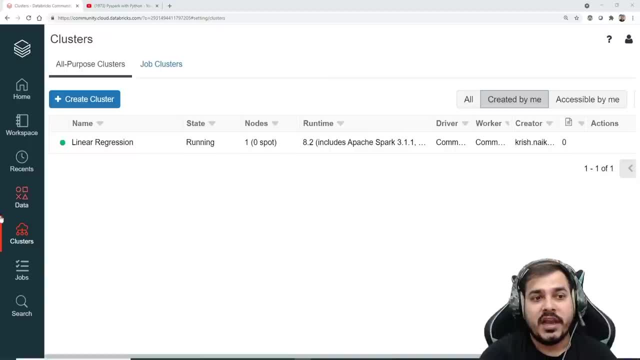 any libraries. i'm just going to use py spark, that is my main name. so guys click on the clusters over here and here you can see that probably after a minute this particular cluster is actually created. so i'm going to go to the home. what you can do: you can create a blank notebook. i've already created. 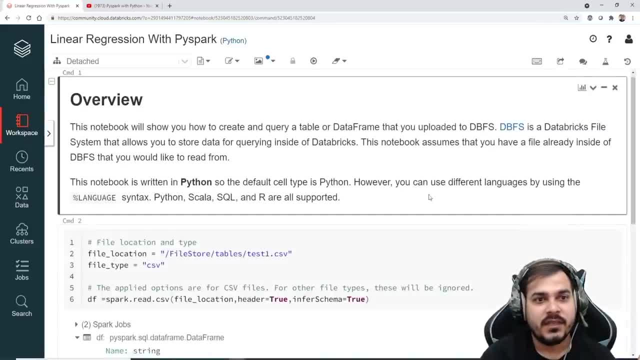 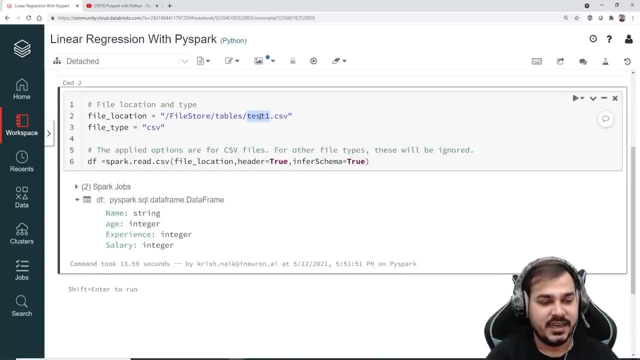 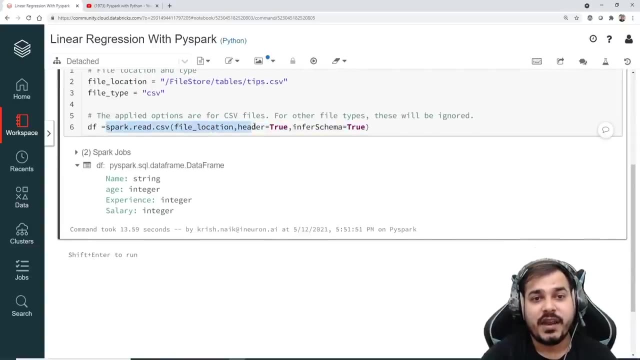 one notebook so that i have the basic code written. so i'm just going to open this and let's start this particular process now. first of all, i have something called as file location. i know my file location is basically tips dot csv, the file type is csv and then i'm just using sparkreadcsv file. 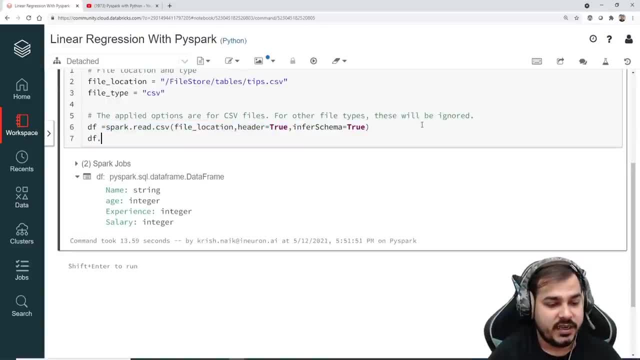 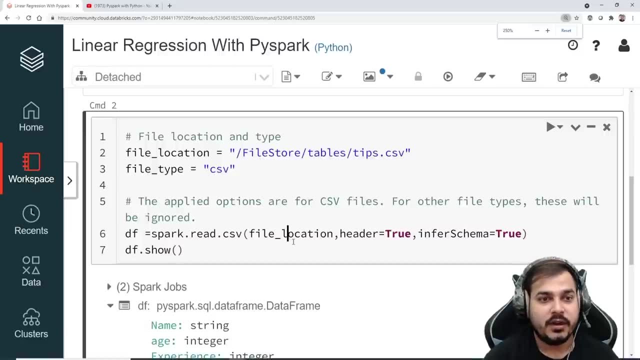 location header is equal to true, in for schema is equal to true, and let me just write dfshow. this will actually help me to check the entire data set. okay, so i'm just going to execute it in front of you and let's make it line by line. i'll try to write down all the all the codes. it will definitely be helpful for you. 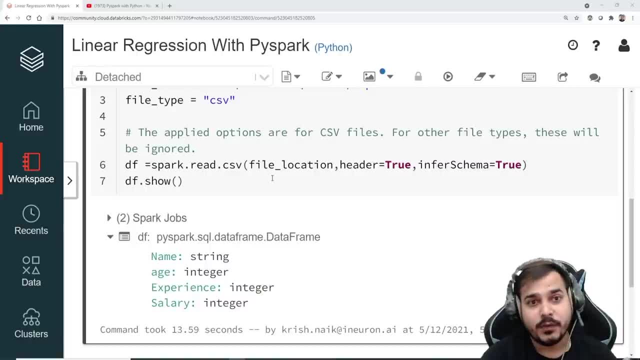 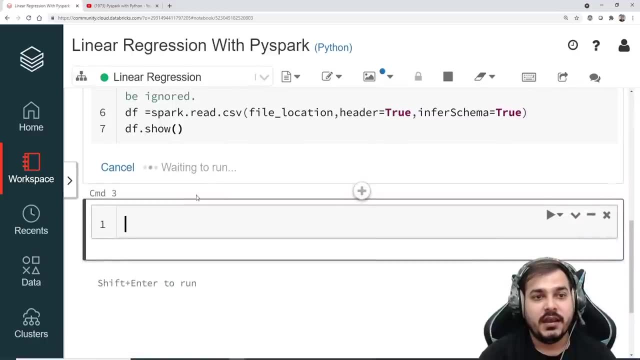 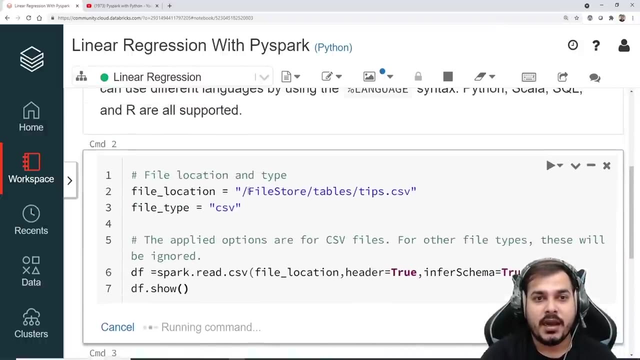 to understand. so please make sure that you also type along with me to understand the code much more better. okay, so here, now i'm going to execute this now here you'll be able to see: uh, my, my clusters will start running, okay, and then you can see waiting to run, running the command. probably we. 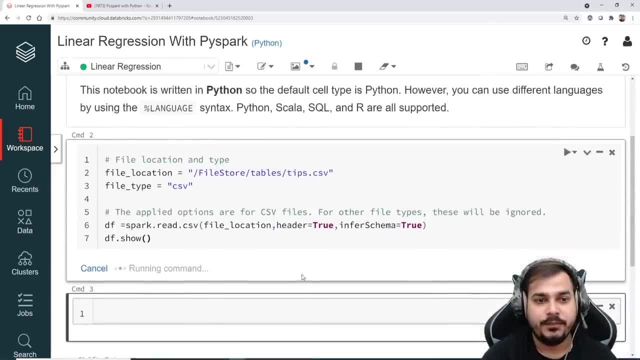 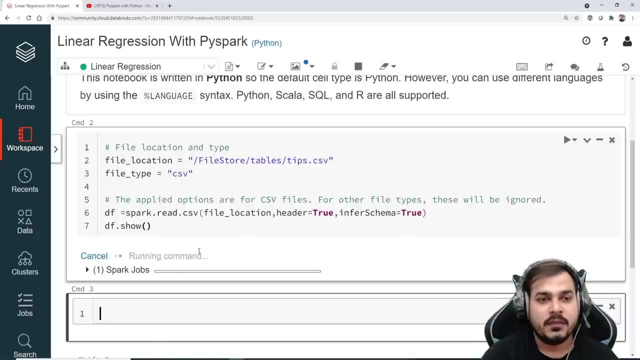 can see it. i'll just zoom out a little bit so that you'll be able to see properly and again, guys, for the first time, if you're starting this particular cluster, it will take time, okay. so spark jobs: it is running and now you'll be able to see my data set. that is, my tips data set which is uploaded in this. 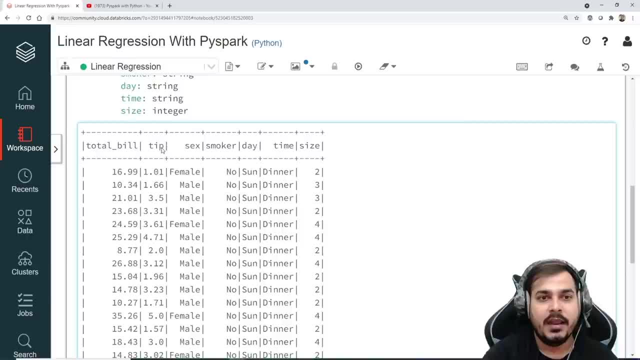 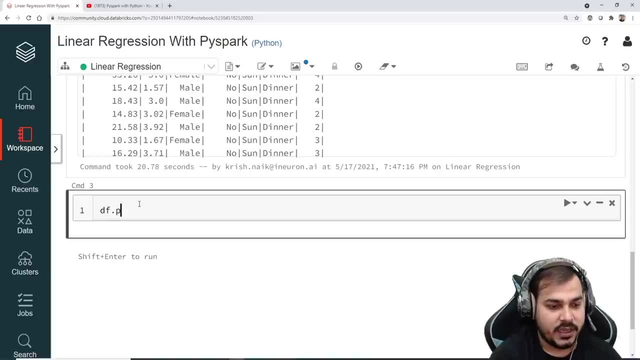 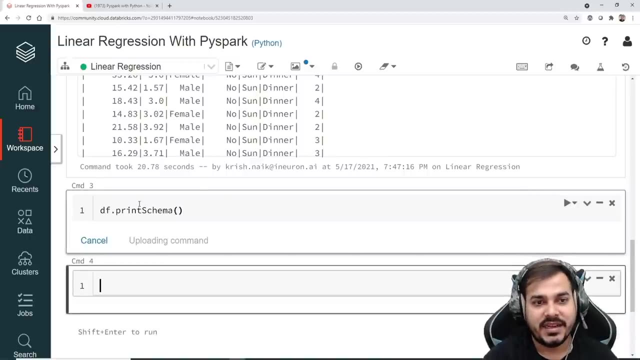 specific file location. so this is my entire data set. total bill tip, sex, smoker, day time size. perfect, now let's go to the next step. uh, what i'm going to do? i'm just going to write dfprint schema. i can also use tab, you know, it will be able to load this entire thing. so now, here you can see. 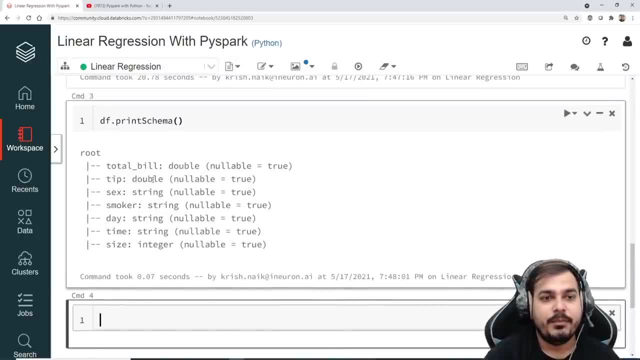 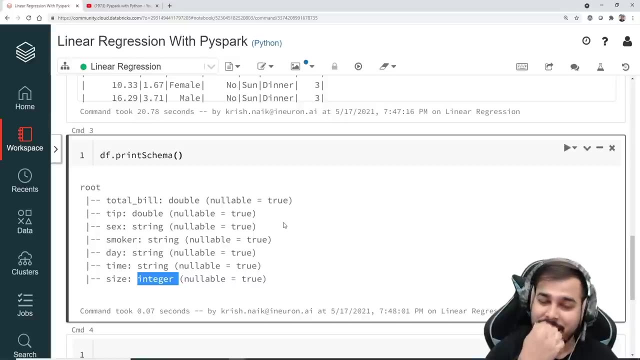 that this is my entire features. total bill tip: sex, smoker, day time. so here is all your features like double double sex is string smoker is string day, string time is string integer. now remember you may be thinking krish- why i am actually doing this in databricks: to just 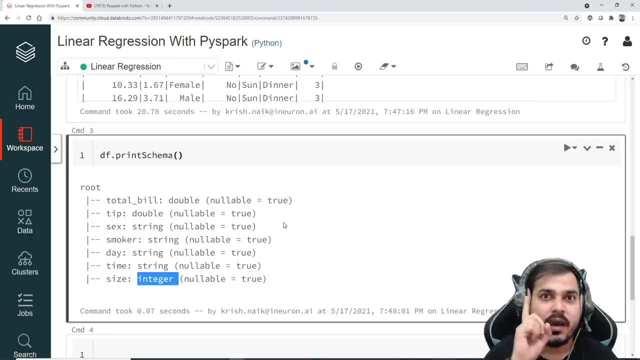 make you understand how this will basically run in the cluster. right now i just have one single guys. that basically means, and the maximum ram in this particular cluster is somewhere around 15 gb. but just understand, if you're working with 100 gbs of data, then what happens? this kind of processing? 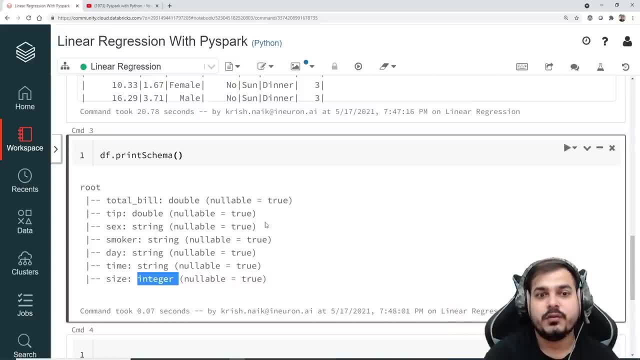 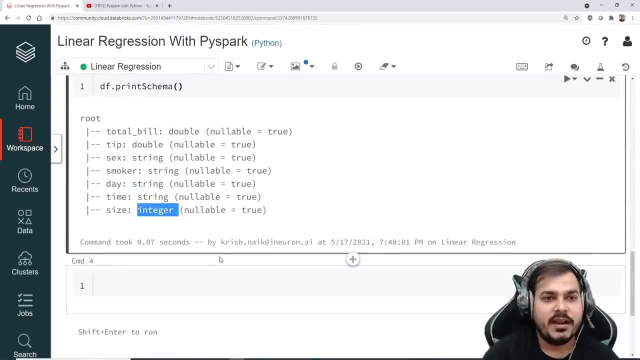 will get uh split in multiple clusters right. so in this way you'll be able to work with big data also in the upcoming things right now. this is how i think guys, right now, let's go and try to understand over here, which is my independent feature. my independent feature is my tips feature: sex. 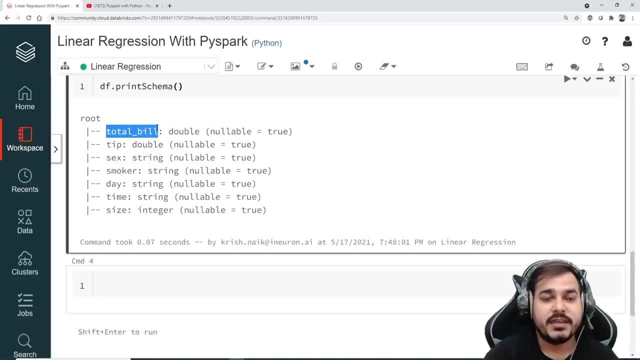 smoker day time and size, and my dependent feature is basically total bill. so, based on these particular features, i really need to create a linear regression algorithm which will be able to predict the total bill. so let's go ahead now. over here i'm just going to write df dot columns. 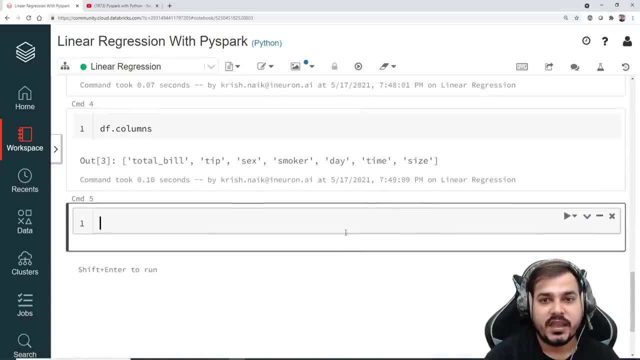 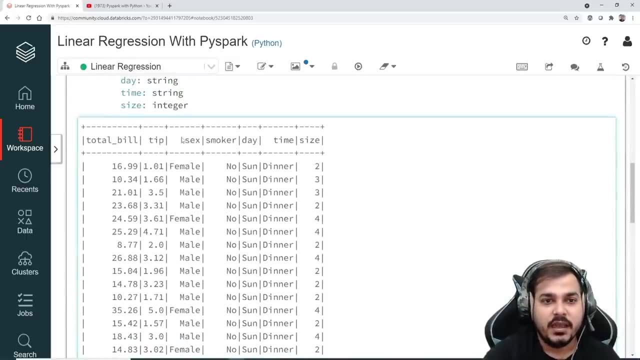 so if i want to check my columns, this is my columns over here, so i can see this is my exact columns, this many columns i actually have now, uh, one thing about this particular feature over here, guys, you have columns like sex smoker day time, right. these all are categorical features, right? 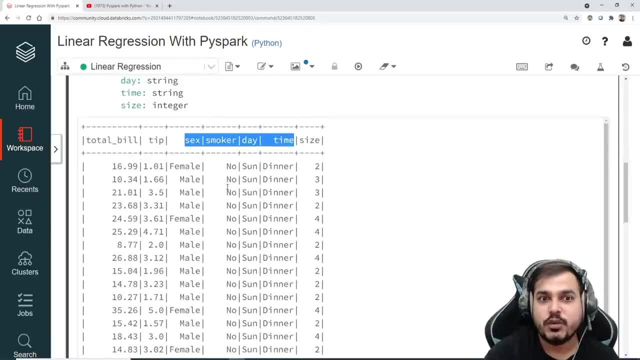 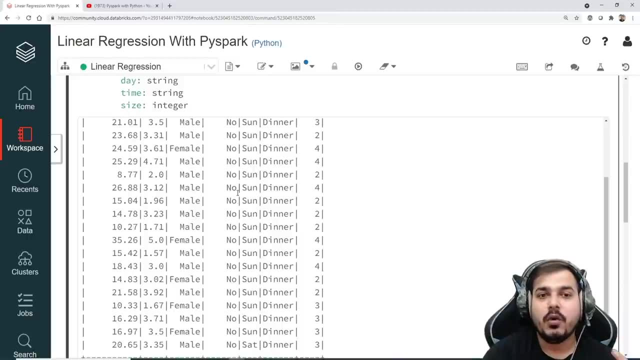 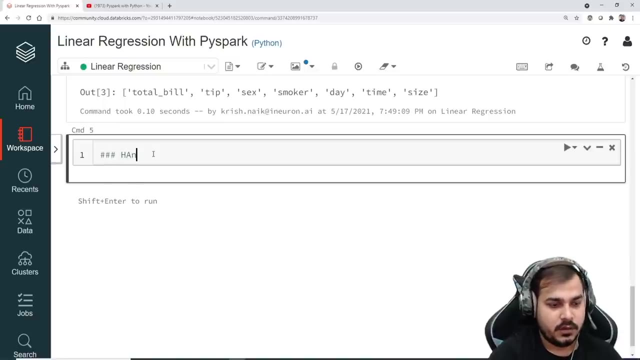 and probably, uh, you know this category features, so let's see how to handle this kind of category features. so here i'm just going to write a comment, okay, handling categorical features. right now i'll try to show you how to handle this kind of category features. now one way in pi spark and obviously, we know, in normal sk: learn, you know we, we try to use one. 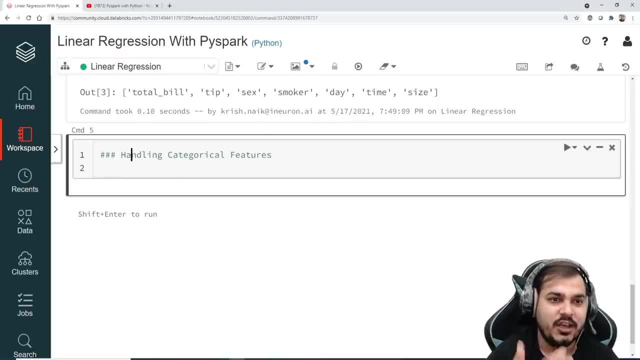 of these kind of category features. now one way in pi spark- and obviously we know in normal sk learn hot encoding- we try to use ordinal encoding, we try to use different kind of encodings in this and similarly we can use that same encoding over here, also with the help of pi spark. 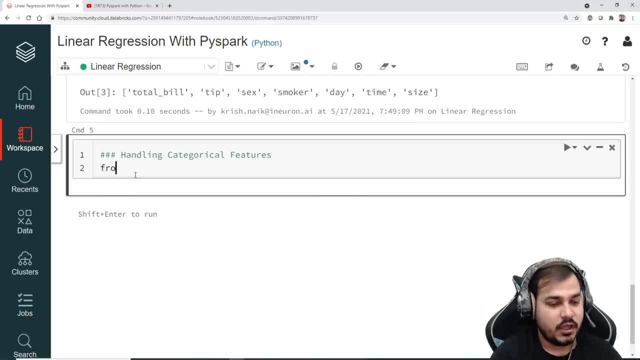 so for this particular process we have something called a string indexer. so i'm just going to say, from pi spark, you know, from pi sparkmlfeature, okay, i'm going to import something called as string indexer. so i will be using this string indexer. this string indexer will actually help us to. 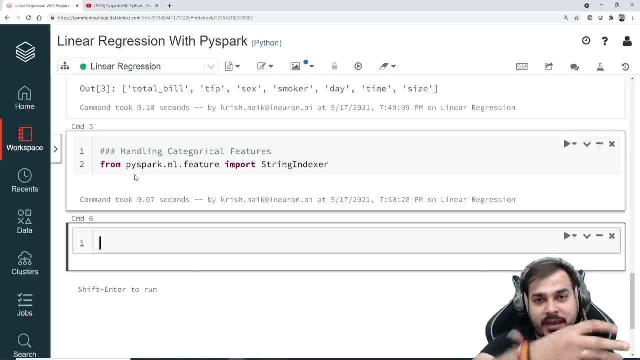 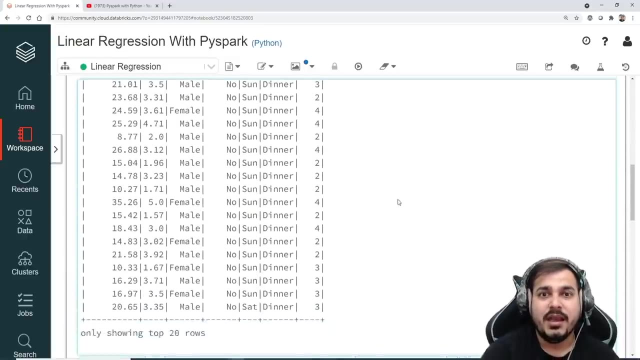 uh, you know, uh, basically convert uh string category features into some numerical features. numerical features basically is ordinal encoding. like suppose, if i have gender, like male or female, uh it'll be shown as zeros and ones. and over here you will be seeing guys, most of the categories over here are ordinal encoding. now you may be thinking one hot. 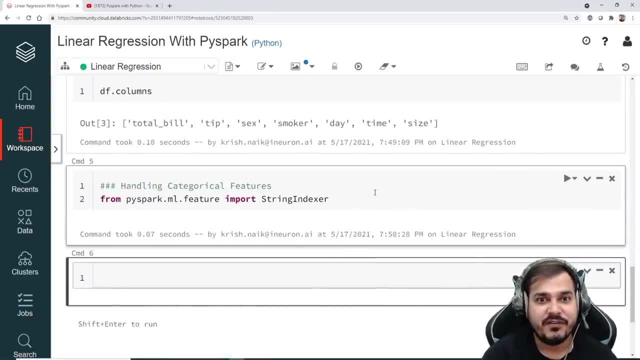 encoding. what is the process that i'll try to show you in the upcoming videos with different different machinery algorithm. the reason why i'm making it? because it is better to learn one thing time right, so we'll. i'll try to show all those kind of examples also. guys, now let's proceed and 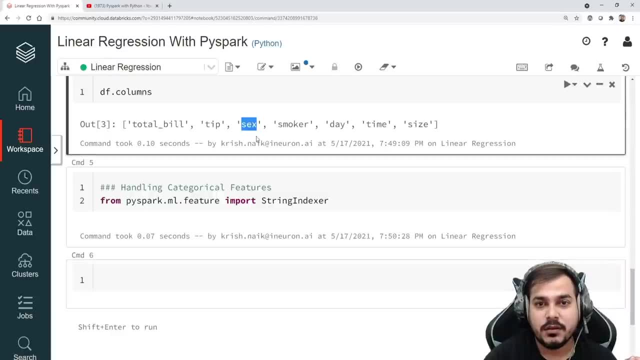 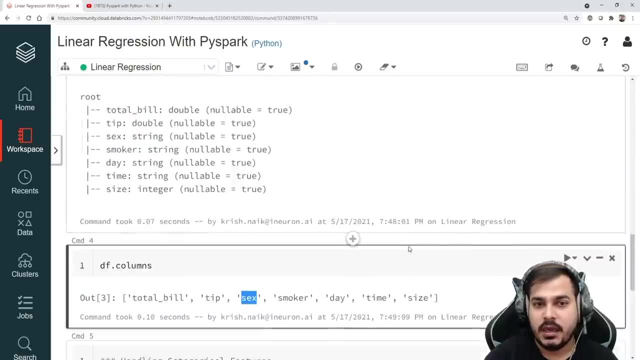 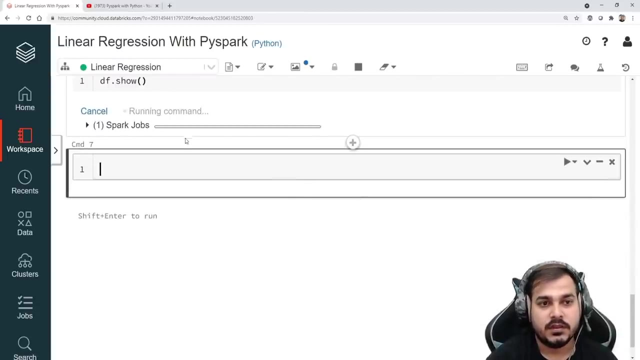 try to see that, how we can convert this category features like sex, smoker day and time- probably time is also a category feature, see over here. so if i see this all features over here, uh, let me do one thing. okay, let me just write dfshow. so this is my entire features. so quickly, if i go and see 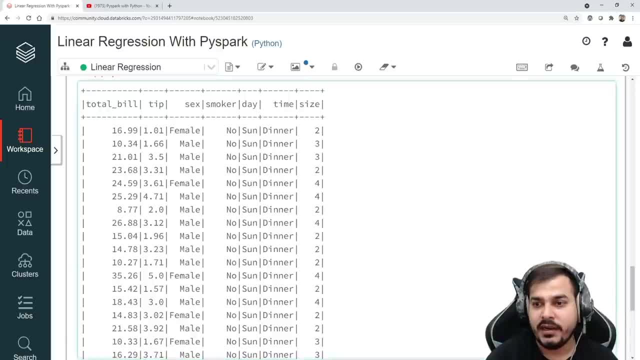 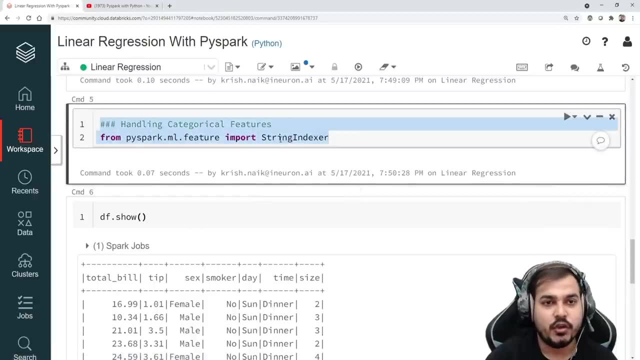 this is time- is also a category feature. so quickly, let's go ahead and try to see how we can basically use this. let me delete this thing also, or let me just write it once again. so i have actually- uh, you know- imported this library called a string indexer. now what i'm going to do over here is that 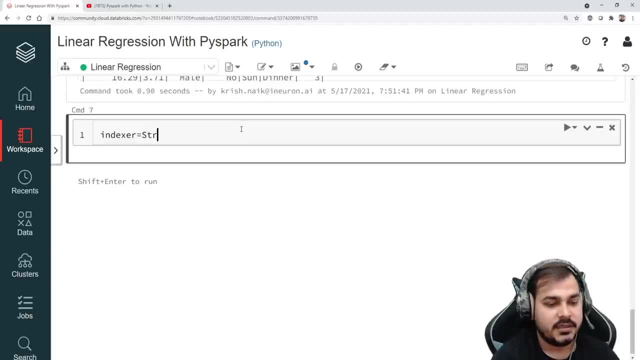 let me write a indexer object saying as this, and i'll write string indexer, and here, first of all, i really need to provide which all are category features. now, remember, uh, in this string indexer, if i go and press shift tab- probably over here here you'll be able to see i have to give input columns. 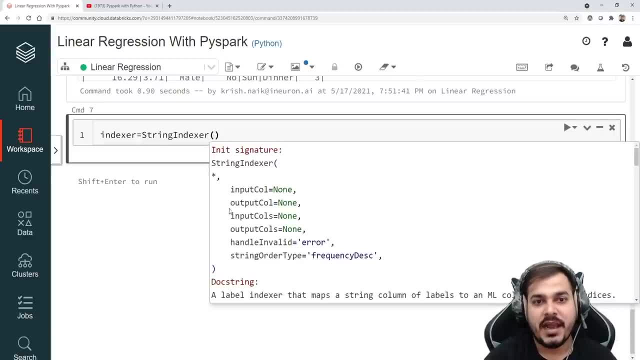 so let me press here. i have to give input columns and i have to give output columns. i also have options of providing input columns as multiple columns and the output columns as multiple columns, so let me try both the thing. okay. so over here, first of all, let me try with input columns. so 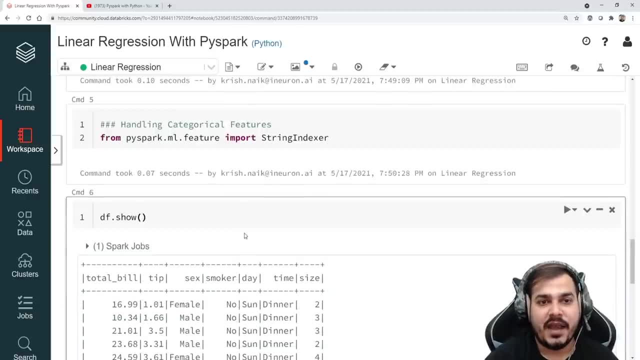 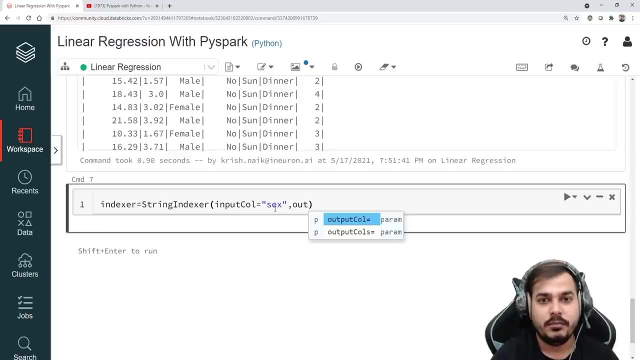 here in the input columns, i will provide my first value. now suppose i want to really convert this sex column into into my category feature. so here i'll write output column okay, and here i'll say: sex underscore indexed. now here what we are actually doing, guys. here i'm actually giving my sex column and this sex column will. 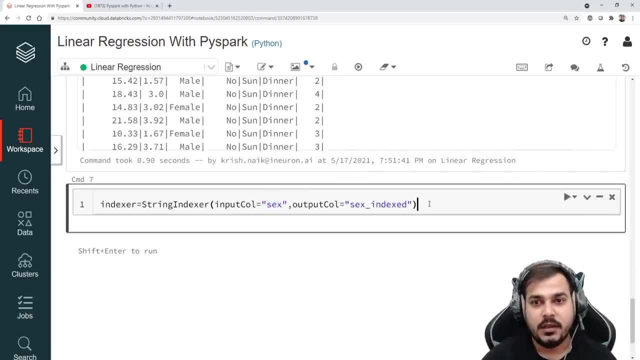 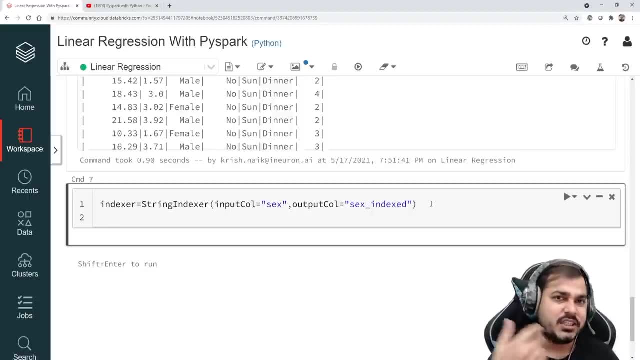 be converted into an ordinal encoding with the help of the string indexer. okay, now in the next step, what i'll do? i'll just write df. okay, probably i'll just use df. or what i can do, i can, i can just create another. uh, probably i can create another data frame. so i'll write df, underscore r, probably. 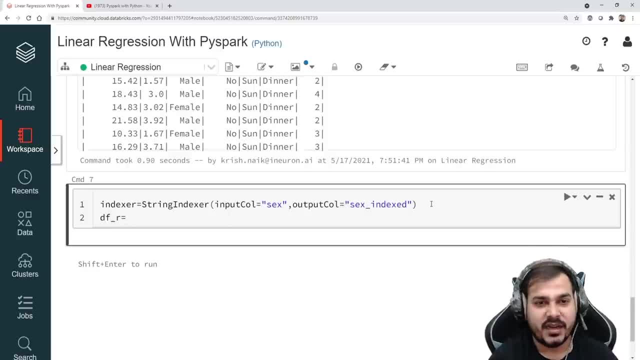 see, because i don't want to change that df and again run that particular code. now i'll say indexer dot fit. okay, so i can definitely use fit, and then i can use transform. so here also it is almost same like that, only guys, uh, fit, underscore transform. and here also i'm going to use this. 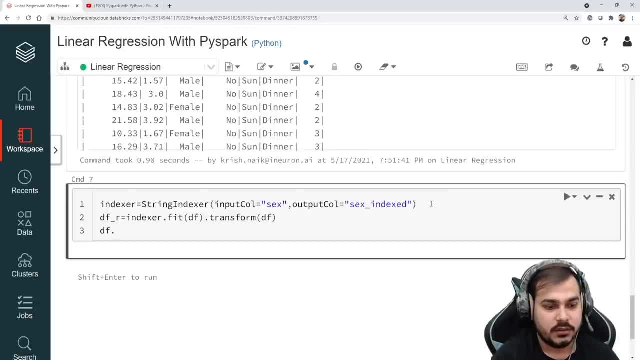 okay, and then if i go and see df, dot, df, underscore, r dot, show here now you'll be able to see that this sex column, one more sex underscore index column, will be created and it will have the ordinal encoded values, uh, in this particular column. so let's go and see this. so once i execute it, perfect, i think it is running. probably it will. 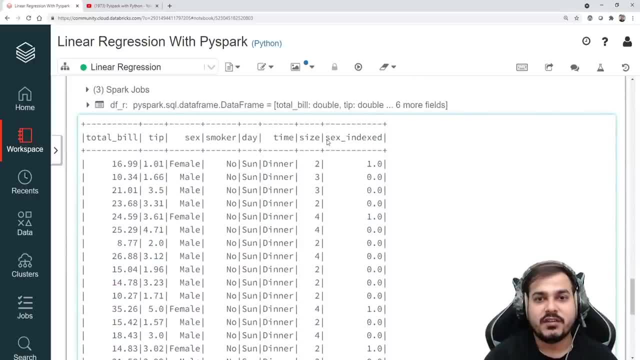 take time. now, here you can see that i am having one more column, which is called a sex underscore index. wherever the female value is that the value is one. wherever the male value is that the value is zero. right. so we have handled this particular column and we have basically converted this. 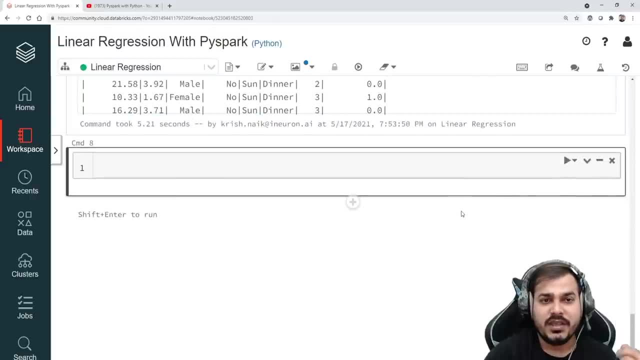 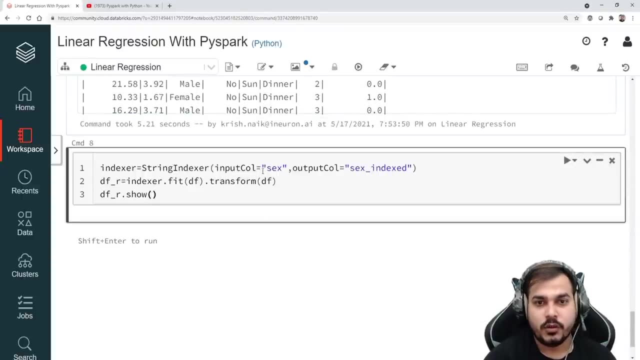 category feature into, uh, the ordinal encoding. now, still, we have any features. so what i'm going to do, i'm just going to use this indexer again, okay, and probably i'm just going to write over here now multiple columns. i will specify. so, first column: i've 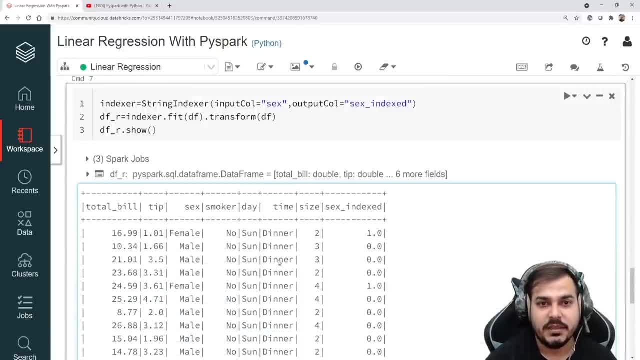 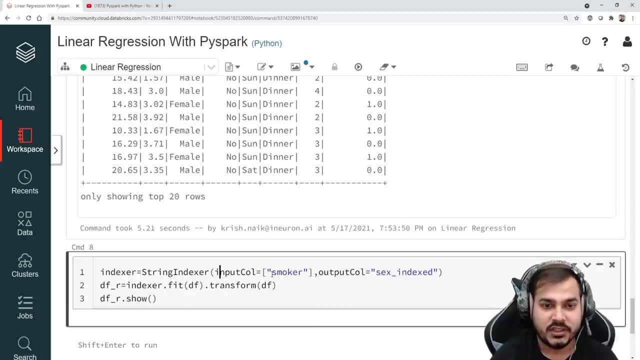 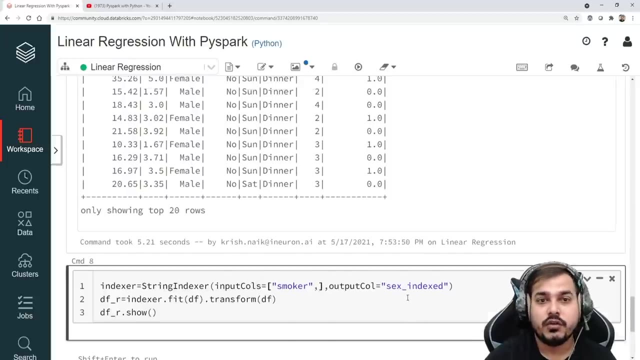 already changed it, so i'm going to change this into something else: sex instead of sex, it will become smoker. okay, smoker, but i showed you guys, instead of writing input columns now i have to write input columns, right? so in this, multiple columns when i'm giving. so this is smoker then. 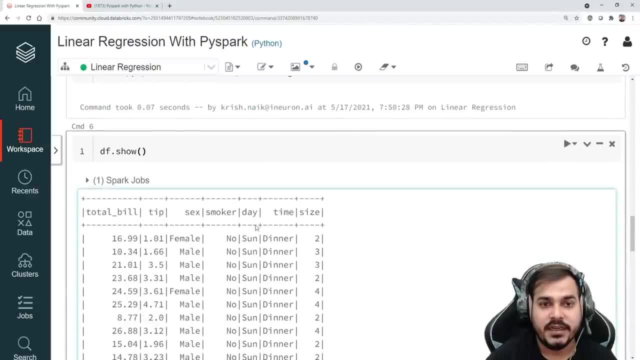 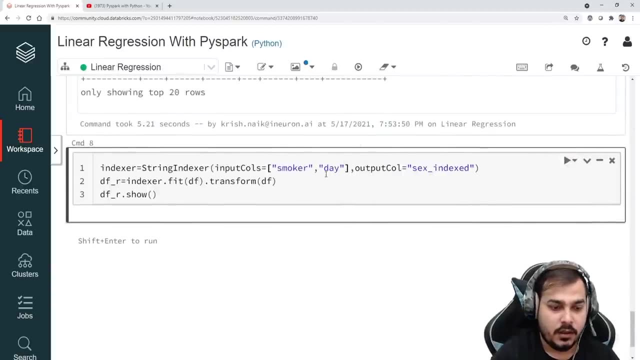 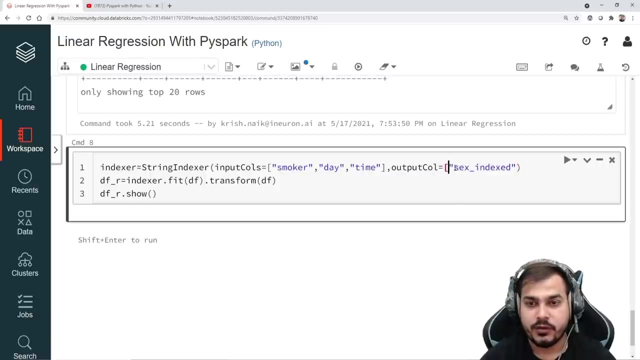 i have one more feature. uh, if i see day, day and time, day and time is more two features, so i'm just going to write over here day underscore. so, guys, now how i've written smoker, day and time. similarly, i will be writing three more columns over here, so the first column should be because: 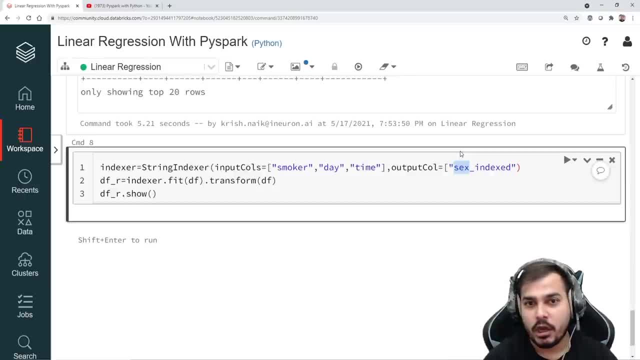 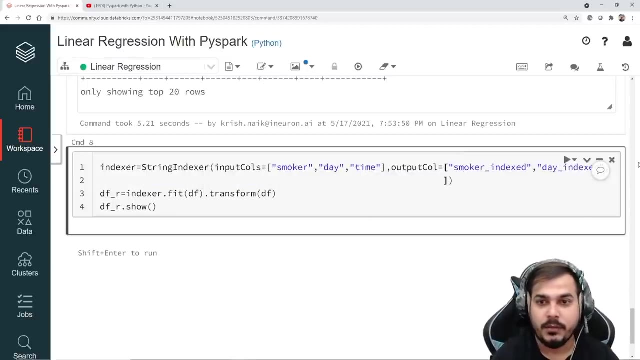 i'm going to create the ordinal encoding and i probably create a new column over here, so this will be my smoker underscore indexed. okay, i'll close the braces over here. my second feature will be day underscore index. right, uh. and my third feature will probably be, uh, time underscore index. 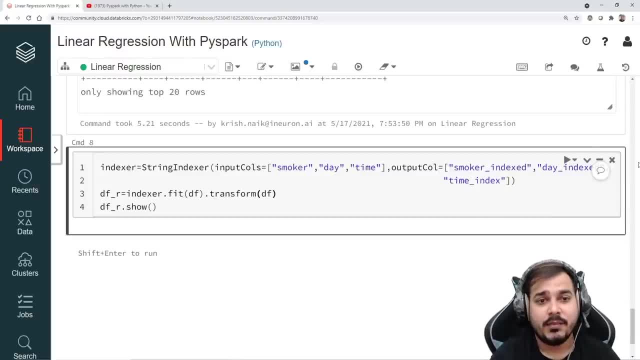 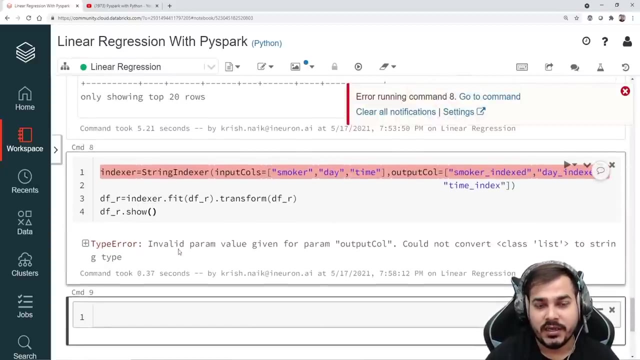 so here i'm just going to create three more features and then i'm giving indexerfit df underscore r- okay, because now i have my new data frame. and then i'm going to say df underscore r, dot show. now, once i execute it, guys, i hope it should not give us an error. okay, it is saying: 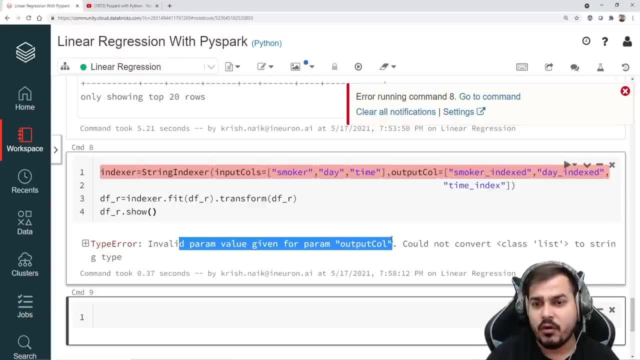 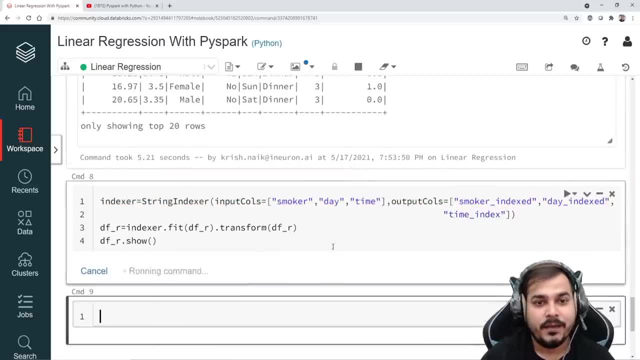 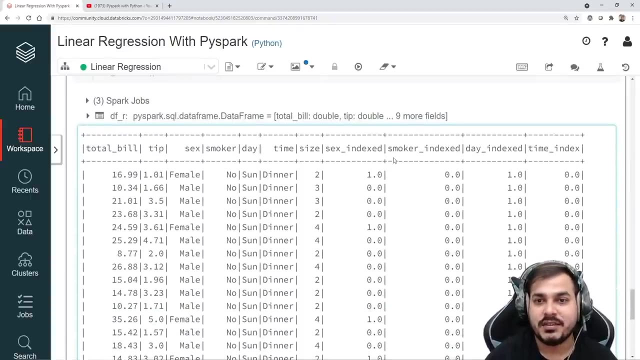 that invalid param value given for param output columns could not convert class bridge to, so i have to make this as output columns, okay? so that was the issue, right? so now you'll be able to see that it's executing perfectly fine. now, here you have all the features available. sex underscore index. smoker underscore index. day underscore index. 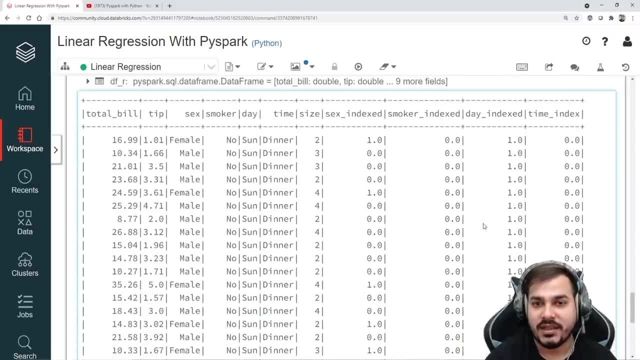 and time underscore index and all you can see over here is ordinal encodings like 0, 1, 2, right, and we have now converted this- all string values- into this kind of all category values that are available, into our numerical values. now my model will definitely be able to understand. okay, now we 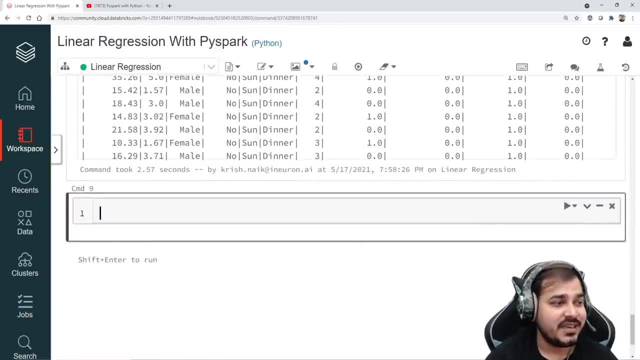 have done this, guys, now let's proceed. what is the next step that we basically do that we are going to discuss now, the now? the steps are pretty much easy, because we have already created this specific data set. now what we have to do is that there is something called as vector assembler- now always. 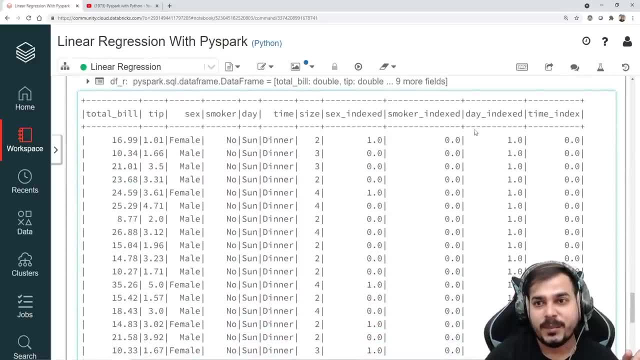 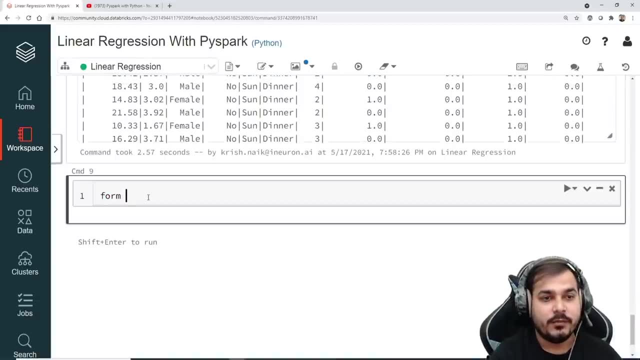 remember, guys, in pi spark, you know, whenever we have all this particular feature, we need to group all the independent features together and the dependent features separately. okay, so, guys, we'll write from from spy spark dot. ml dot. feature. i'm going to import something called as vector assembler, right? so i'm just 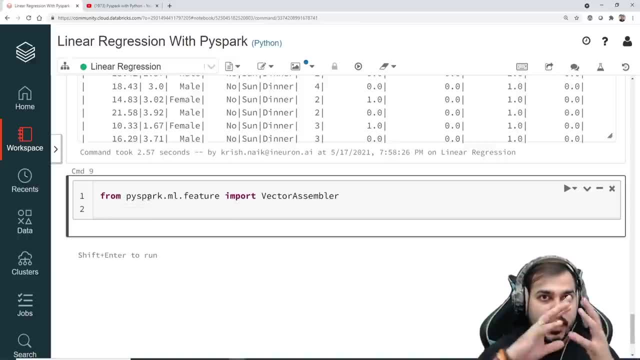 going to use this vector assembler. this will actually help us to group independent features together and the dependent feature separately. so let me just go ahead and write vector assembler and then i'm going to initialize this. the first parameter i have to provide is basically my input columns here, my input columns. what are the input columns i have? let me just see before this. let me. 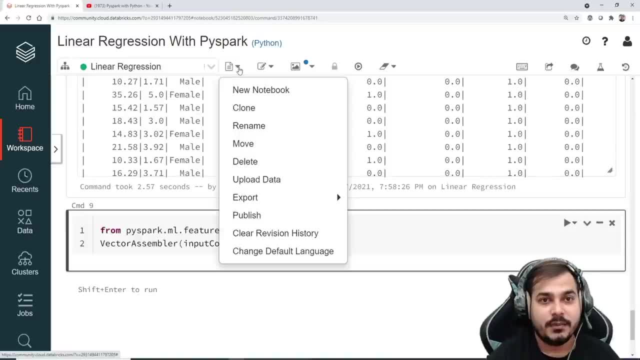 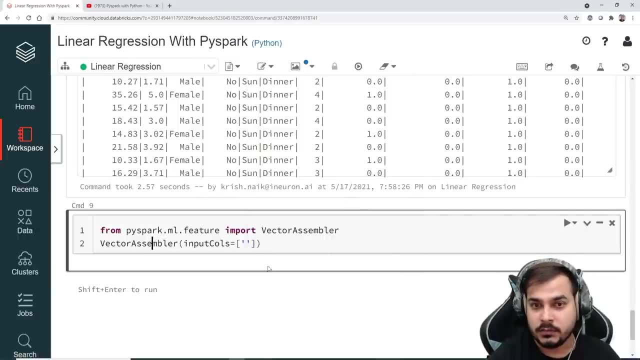 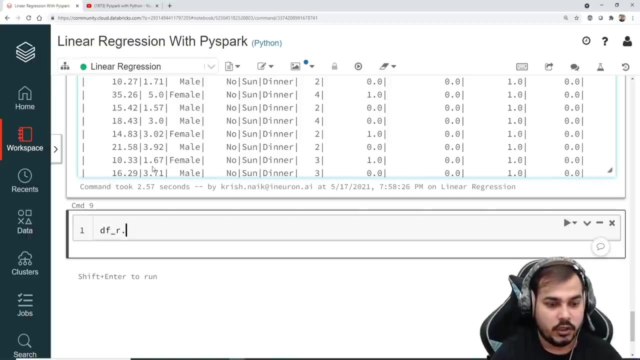 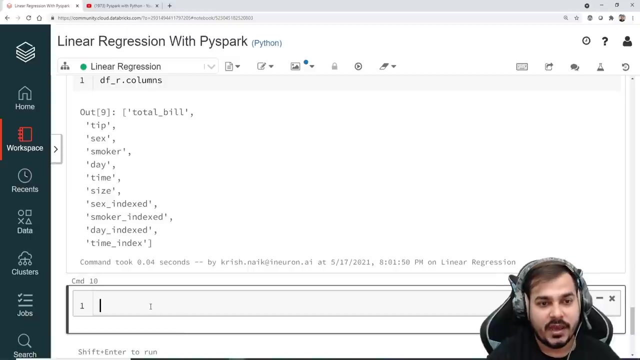 quickly do. one thing is that let me make a cell. okay, move a cell up, create a cell. or let me just remove this and probably just let me write: uh, you know df, underscore, r, dot columns- okay, so how many number of columns we have? so i have all my information with respect to the columns. so my 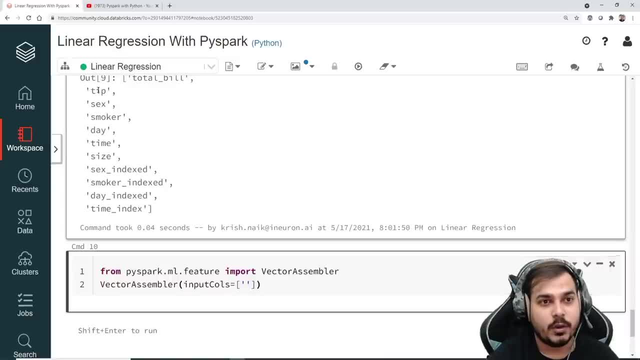 input column over here. the first thing that i am definitely going to provide is my tip column, because tip is required. tip is the first independent feature and it is a numerical feature. then i have something like six underscore indexed. okay, so i'm just going to copy this: 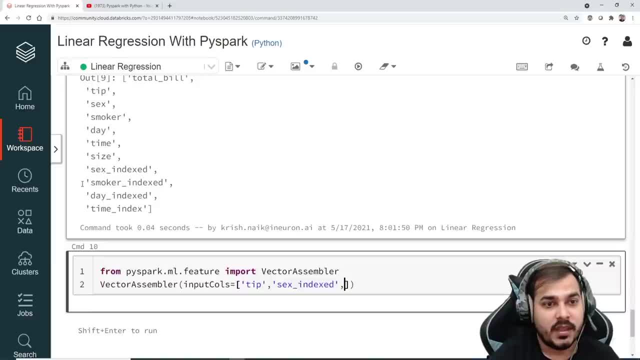 paste it over here. and this is my another input feature. and remember, guys, we really need to follow the order. so now my third feature is basically smoke index and before this also i can also specify size. okay, so i will be specifying size, size, sex index, smoker index. okay, and then 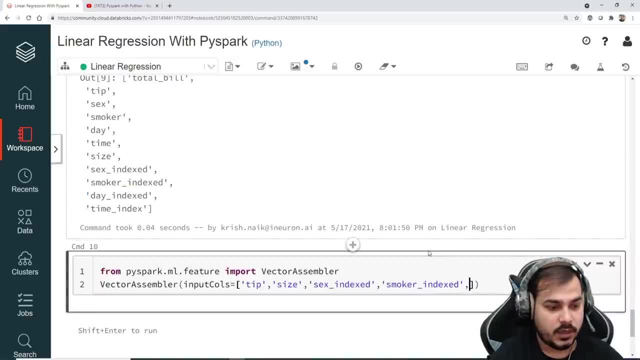 probably i'll also create day index. okay, day index comma. i'm just going to use time index, okay, so this is our. these are all my independent features and with respect to this, now, remember this will be grouped together and i also have to say that if this is grouped together, let's create. 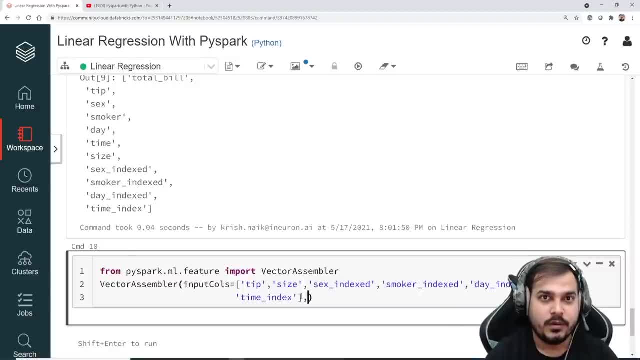 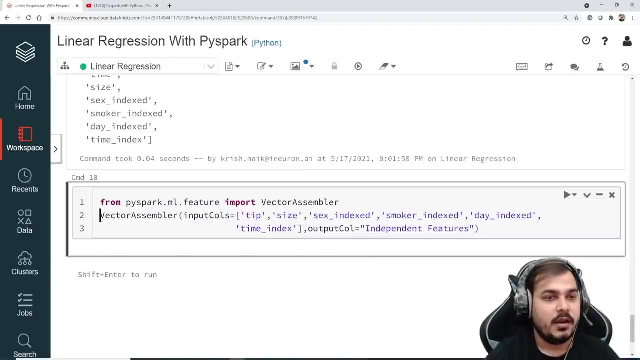 a new feature and entire and name this entire group. okay. so here i'm just going to say: output column is equal to, and here i'm just going to specify this are my independent features, so i'm going to name this entire thing as my independent feature. pretty much simple. now let me do do one. 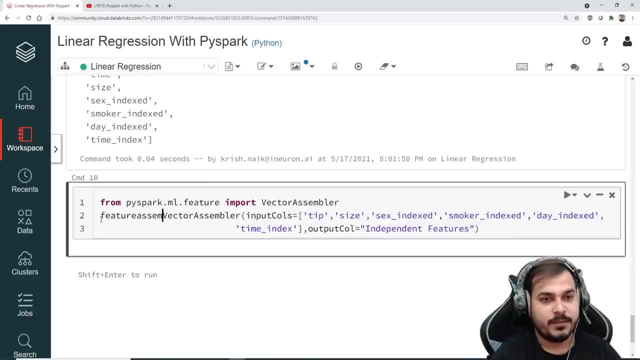 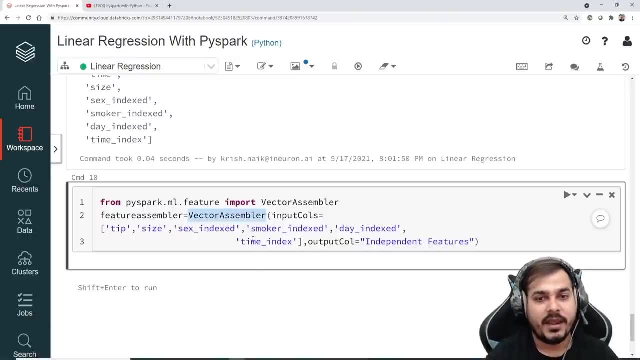 more thing: let me create a variable called as feature assembler, so that we will be able to transform these values. okay so, feature assembler is equal to vector assembler, and here i have to provide my input columns, and here i have to create a new feature and name this entire group. okay, so? 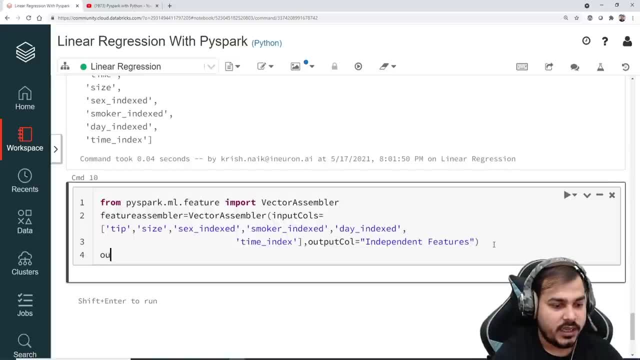 and the output columns. pretty much simple, pretty much easy. now the next step that i'm going to do is that right output is equal to. i'm just going to say, dot transform, because i really need to transform and this needs to be transformed from my df underscore art. okay, so let me just execute it. 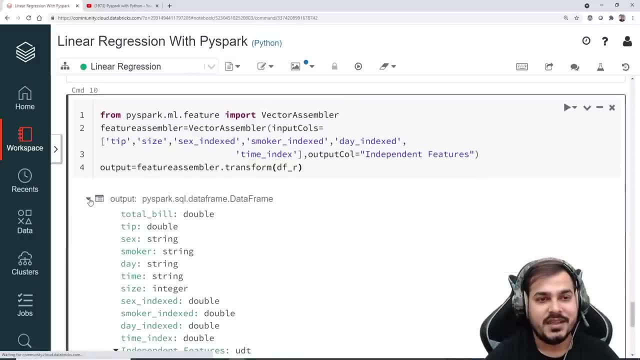 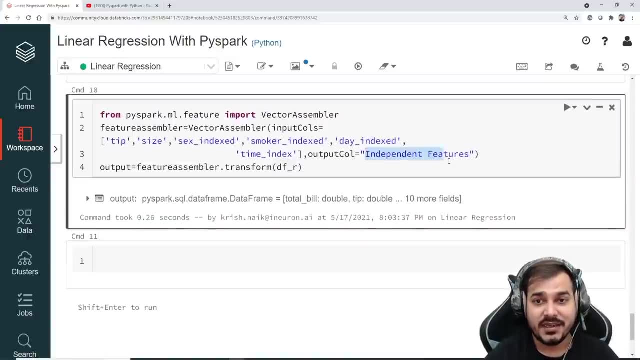 now. now here it has got executed. here you can see the entire output. all these things are created. these are my independent features now in the independent, and why we need to create this. independent features- that is the. that is the specification that is given in py spark. always remember we need to create a group of features in, probably a list. all these: 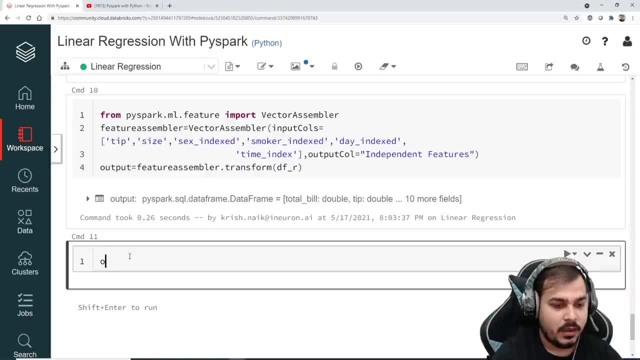 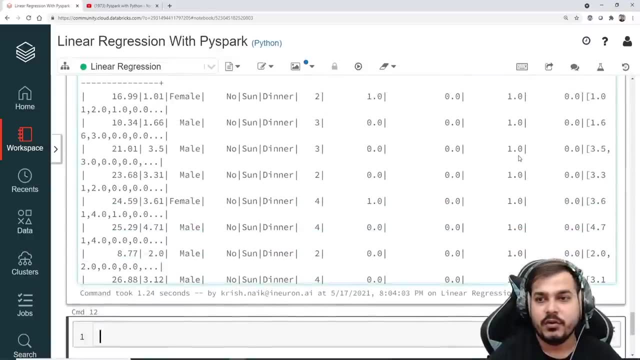 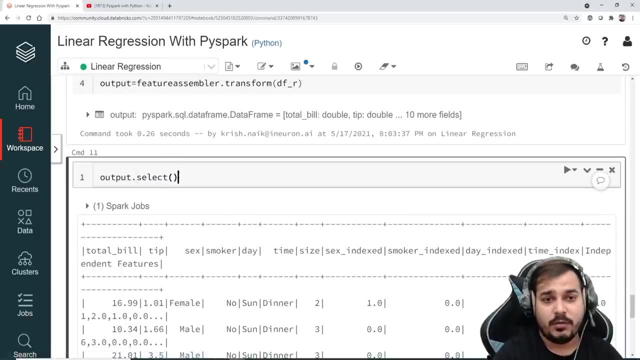 independent features will be done together. now, if i go and see my output dot show here now, you'll be able to see. i will be able to see one more feature which has this: or let me just write output dot select, because probably all the features have been grouped together and it is very 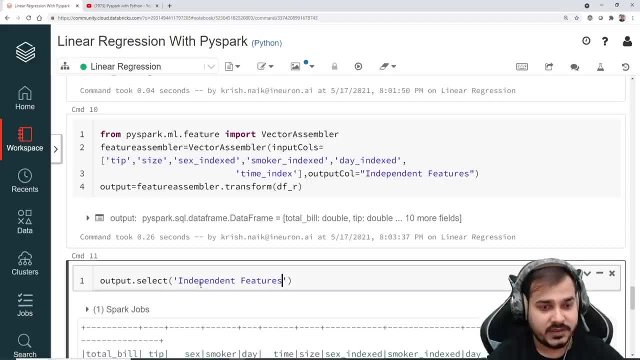 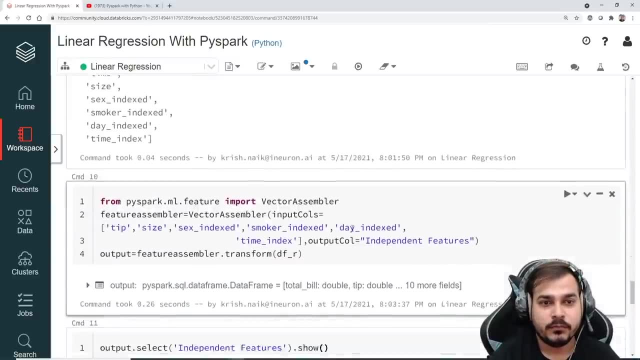 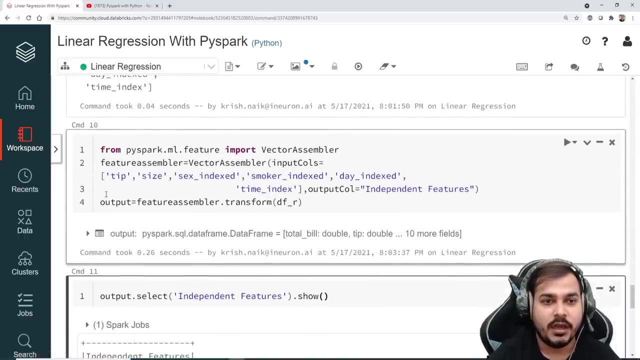 difficult to see all the features in just one screen. i'm just going to take this independent feature and just click on dot show. now, once i do this here, you will be able to see all these particular features are there. remember this needs to be shown in the same order: the. 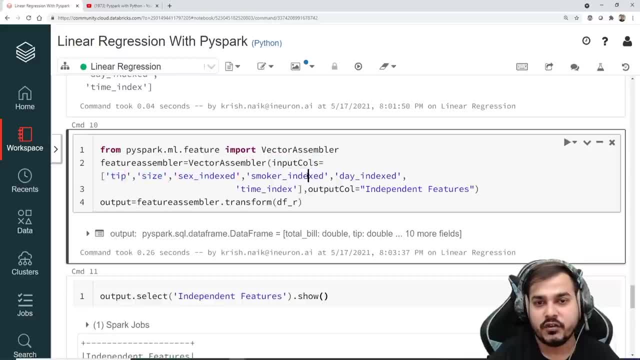 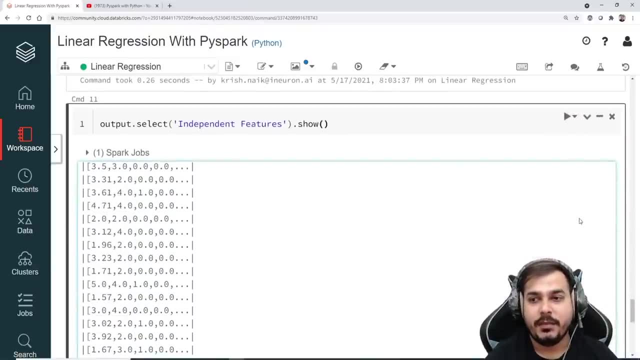 first feature is tip, then size: sex underscore index. smoker underscore index. day underscore index. time underscore index. so these are my independent feature. now i just have one feature, and over here you'll be able to see that it is just having a list of all the features like this. 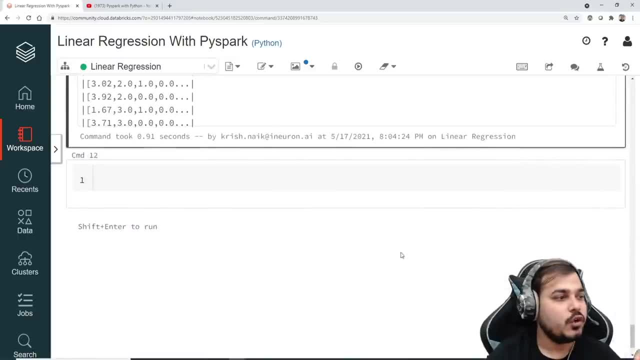 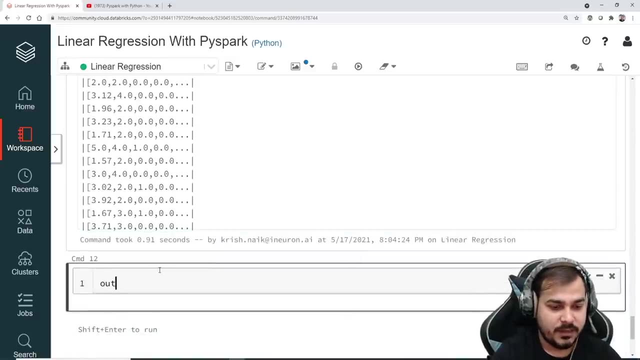 and this is the first major step to create. okay, now let's go to the next one. now i know what is my output. now what i'm going to do is that, out of this entire output, if i go and see my output output dot show here you'll be able to see. 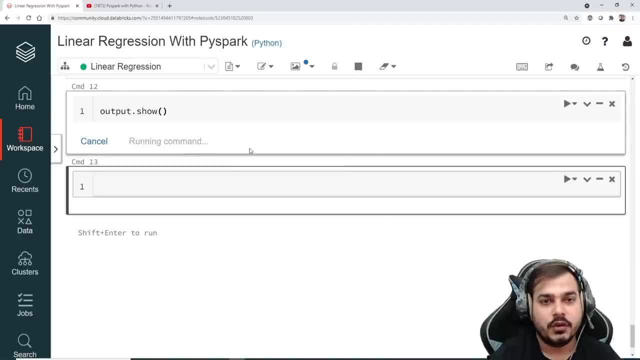 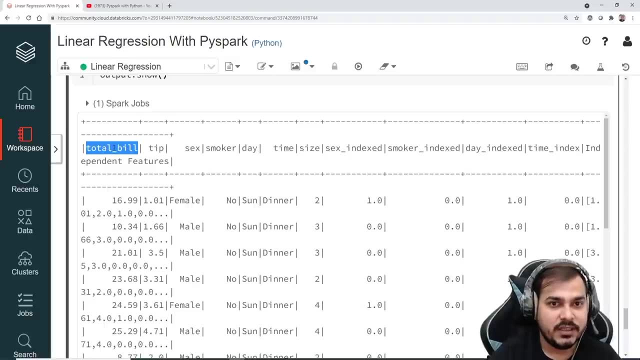 all the features are available right in output dot show. so here you'll be able to see all the features are available. now you know which is your output feature, right? so this is my dependent feature and this independent features are my independent feature. so what i'm going to do now? 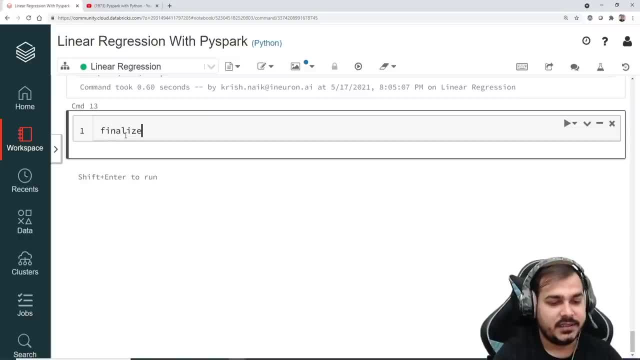 output, or i'll say this is basically my finalized data and i'm just going to pick up two columns, that is, output, dot, select, and inside this i'm just going to give my two features, which i'm going to say one is independent features. okay, independent features. i hope that the name is right, otherwise 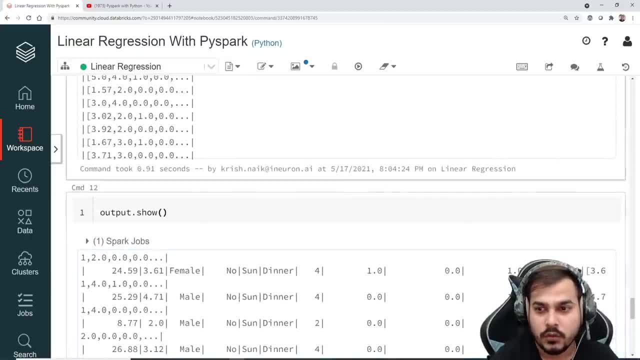 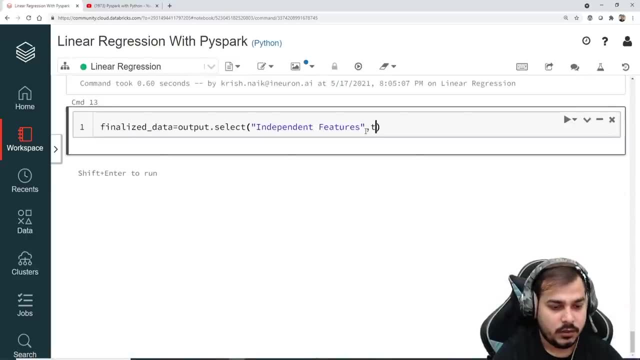 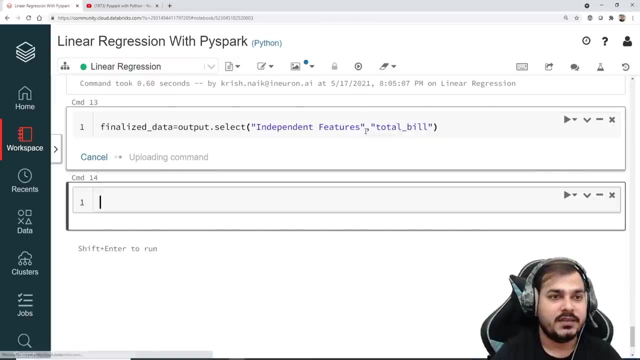 i'll just confirm it once again. so let me click it over here and i'm just going to go and execute this and i'm just picking up two features right from this now, if i go and find out finalized data dot show now, i'll be able to see two important features. 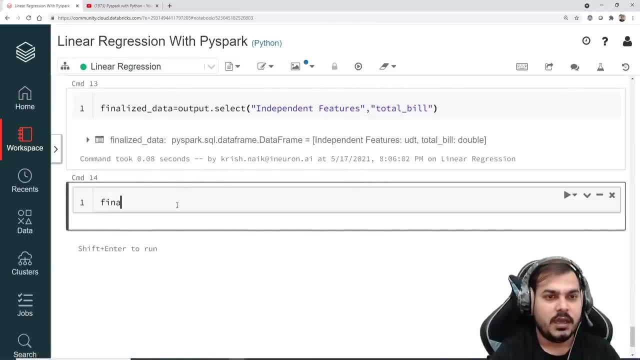 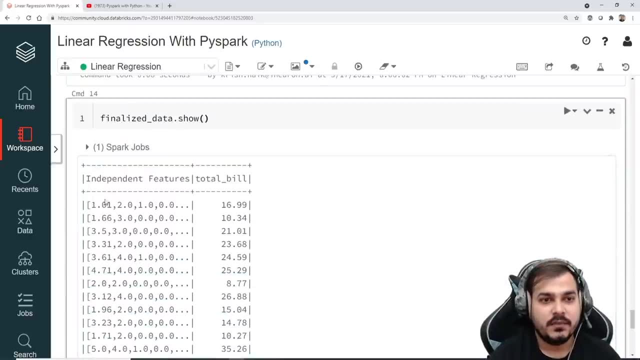 that is, independent features and total bill. remember, this is all my independent features and this is my dependent feature. this is very much simple till you get to the end of this video. i hope you enjoyed this video. if you liked it, give it a thumbs up and subscribe to my channel. 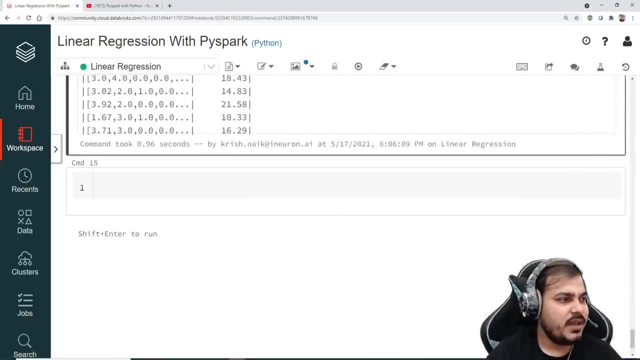 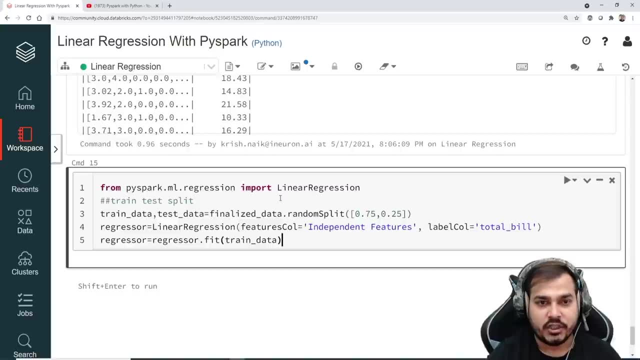 and i'll see you in the next video. bye here, if it is done, guys. the next step is basically, i'm just going to copy and paste some code, i'm just going to apply the linear regression. so first of all, from piesparkmlregression, i'm going 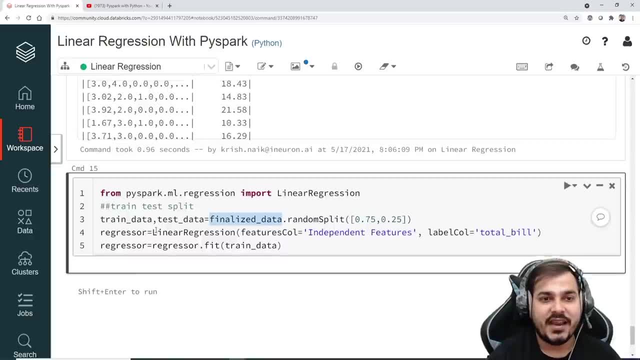 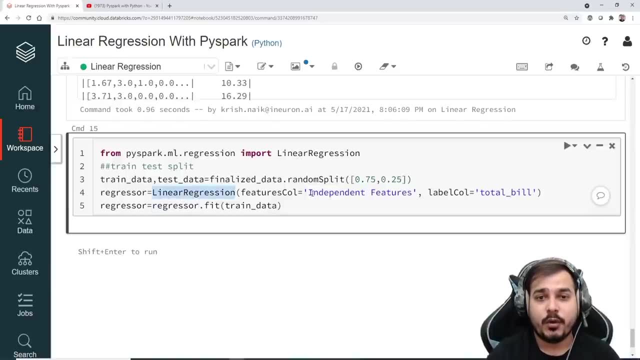 to import the linear regression and then i'm going to take this entire finalized data and then do a random split of 75 and 25, okay, and then in my linear regression i'm just going to provide my independent features as my feature column. this is two parameters needs to be given in linear. 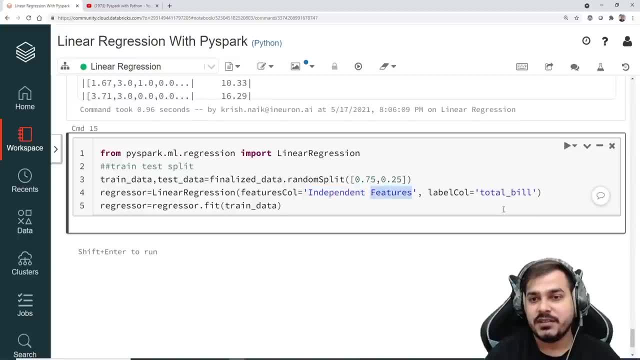 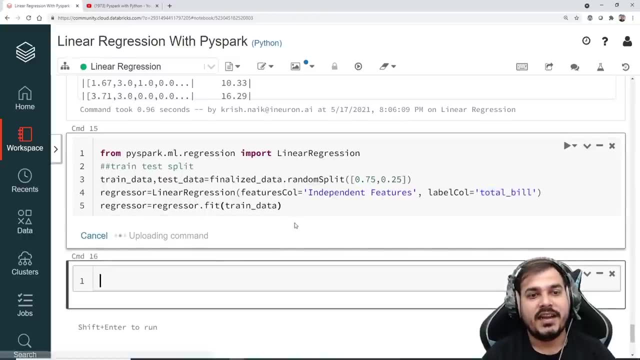 regression. one is feature column. here i'll be providing independent features. the second one is image. of course i'm going to leave this as my total bill, which is my dependent feature, and now i will just do a fit on train data. so once i do it, my regressor model will get created, and probably this: 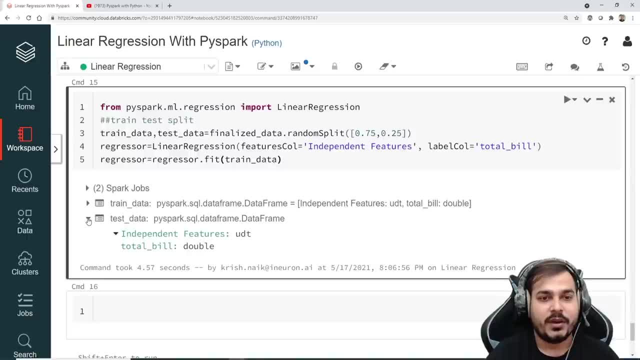 will take time. now, here you can see all the information, amazing information you are getting with respect to train and test. okay, and remember, guys, whatever group we have made this independent feature, this is in the format of udt. okay, you can see the full form of udt. that's not a big problem. 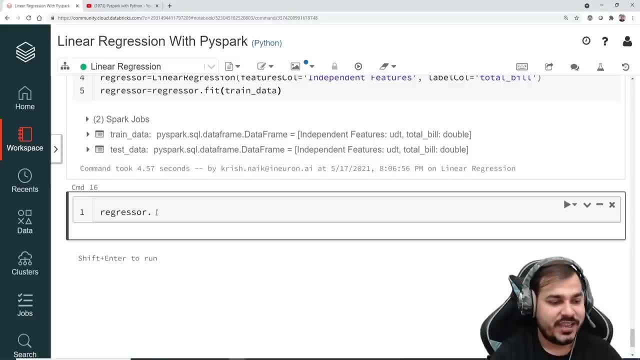 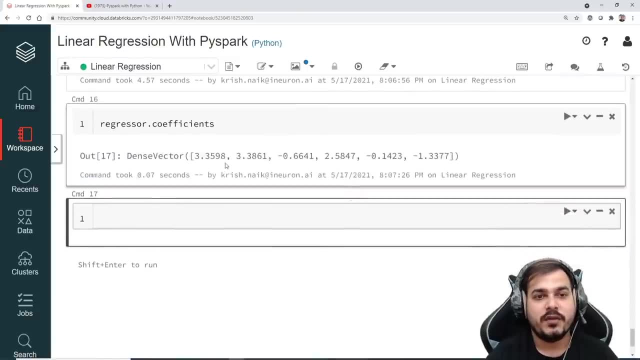 at all. okay, now i have my regressor, um say regressor dot coefficient, since this is a multiple linear regression. so i'm just going to use regression coefficient and these are all my parameters, or different, different coefficients, because i have around six parameters. so these are all the six, uh, different, different coefficients. 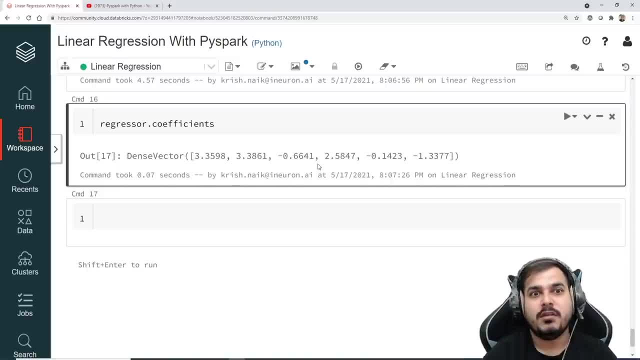 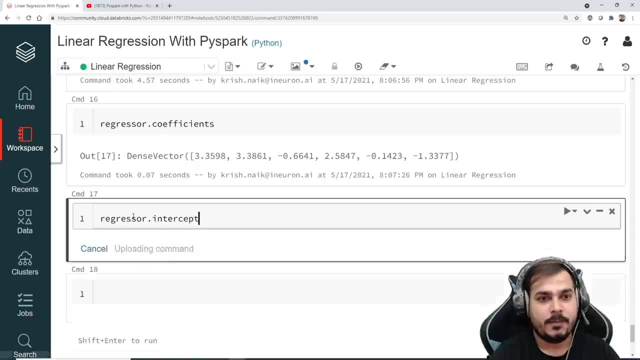 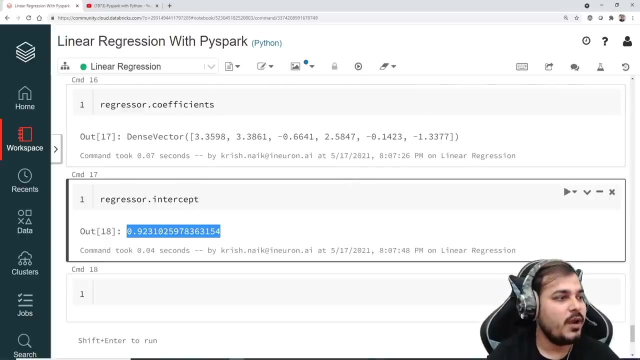 always remember, in a linear regression you will be having coefficient based on the number of features and you will also be having a intercept. so here i'm just going to say intercept. okay, so this is basically my intercept, that is 0.923. okay, so here you have both the information. 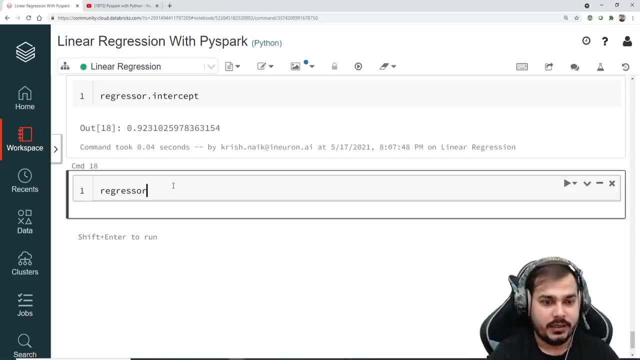 now it's the time that we'll try to evaluate, evaluate the test data. so here i'm just going to say test and this is basically my predictions, right? so here let me write it as something like this: so predictions, okay, prediction, and, and what i'm going to do? i'm just going to write pred underscore results. 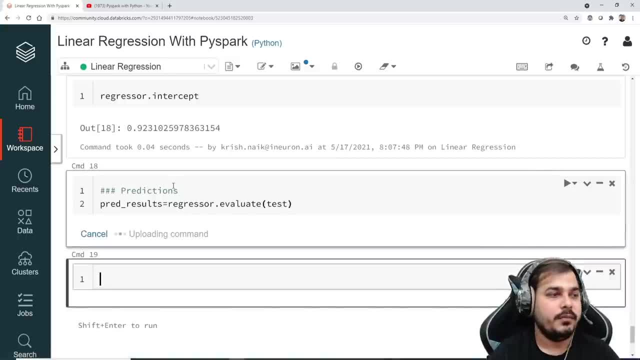 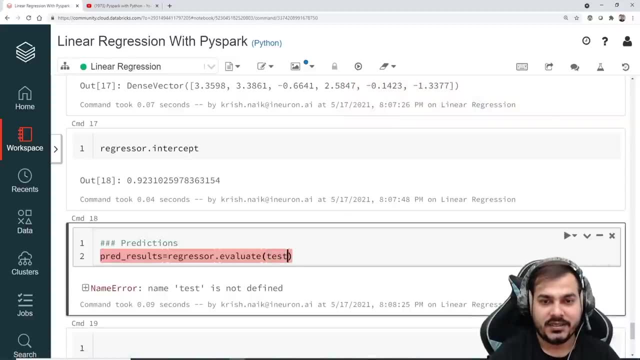 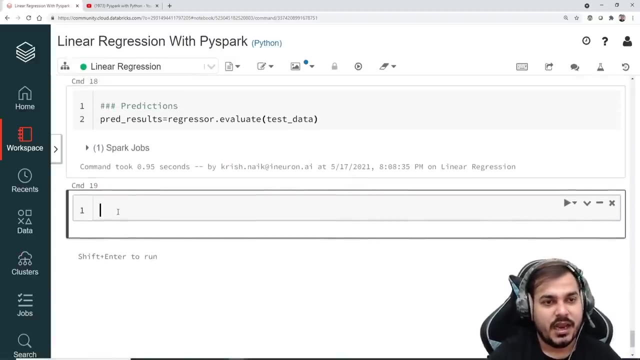 results is equal to this one and this will basically by be my results. okay, or test is not defined. why test is not defined? because this should be test data. i'm extremely sorry. okay, but it's okay. you will be able to get so small, small errors. okay. now, if i really want to see, 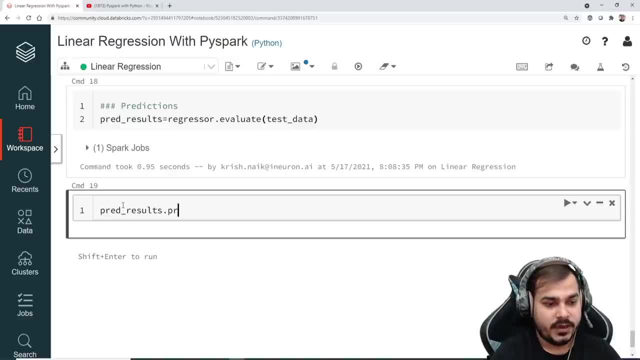 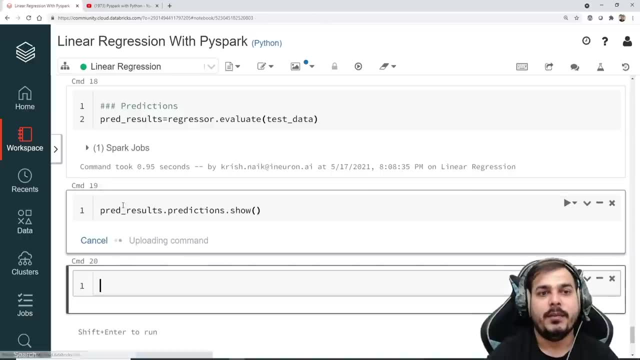 my pred results. just go and see pred dot predictions. there will be something like predictions dot show. okay, if you write like this here, you'll be able to get the entire prediction okay. so remember in this prediction, this is your independent feature, this is your total bill. this. 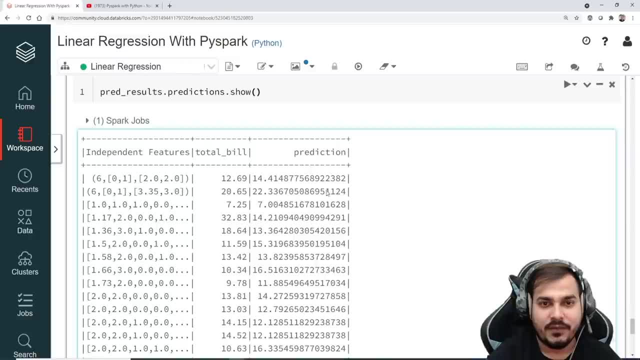 is your actual value and this is a prediction value. actual value, prediction value, actual value and prediction value. here you can actually compare how good it is. you know, by just seeing your total bill and the prediction value. pretty much good, pretty much amazing. you are able to see the data. 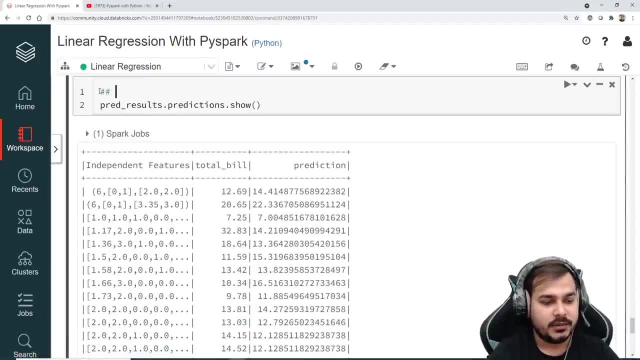 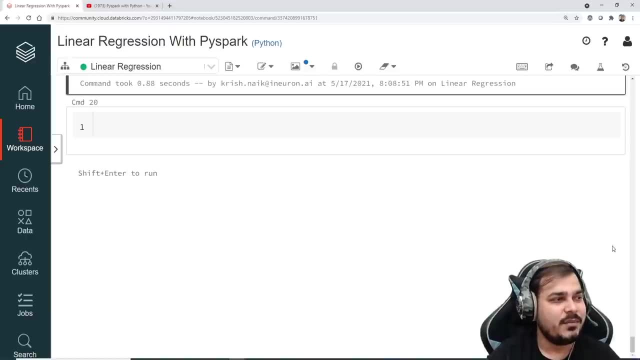 i'm just going to write my final comparison. okay, okay, final comparison, perfect, i'm very much good at it. you can see it. now let's see some of the other information, like what all information we can basically check it out? uh, from this we can we have a lot of things. probably you want to check out the r square, so what you can write, you can. 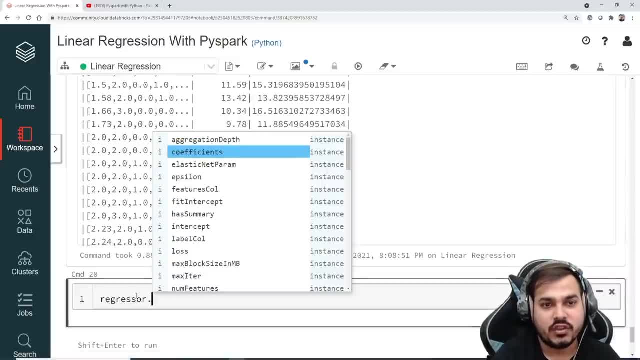 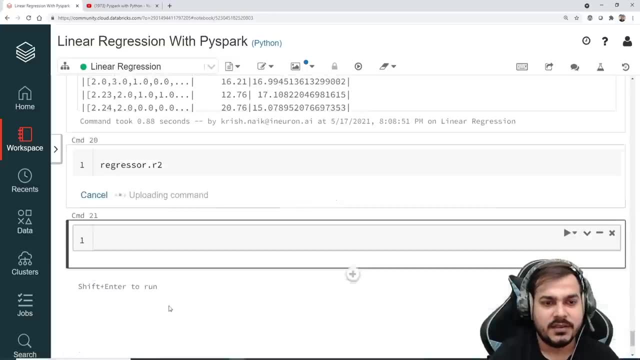 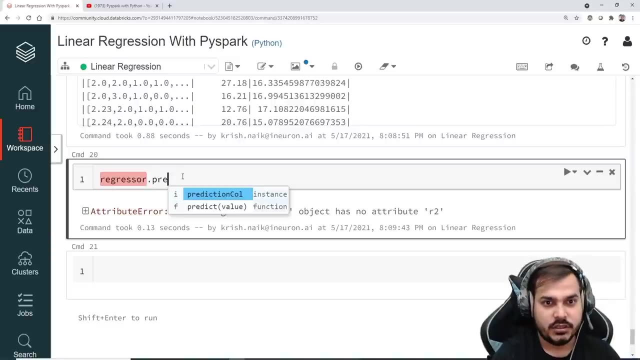 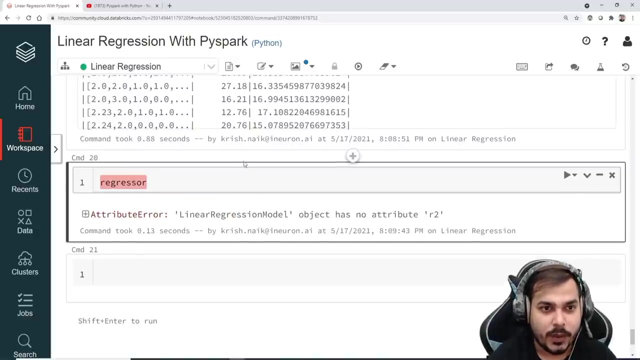 basically write regression dot. if i press tab this coefficient intercept, then you have loss. then there's also something called as r square. if i go and execute this, this is basically my r square, or let me just write it down, i think, the prediction, predictions. i don't think so. r square is where let's see whether we'll be able to see the r square value. 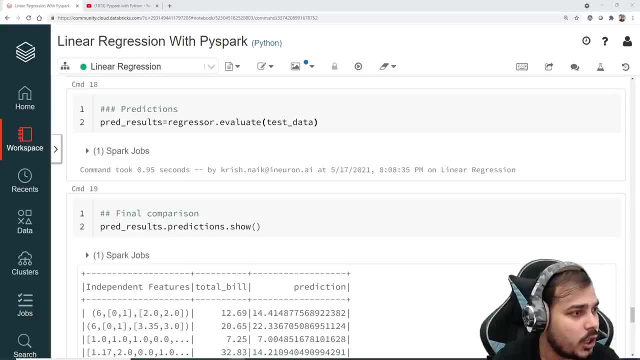 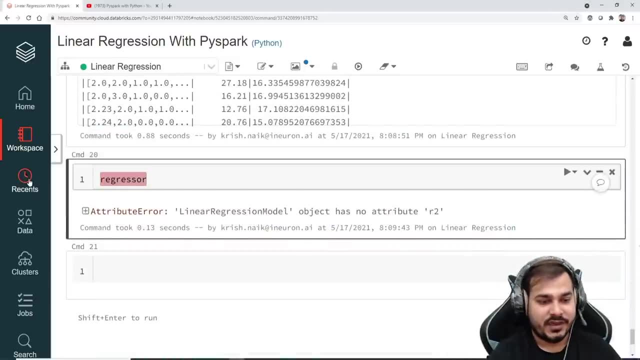 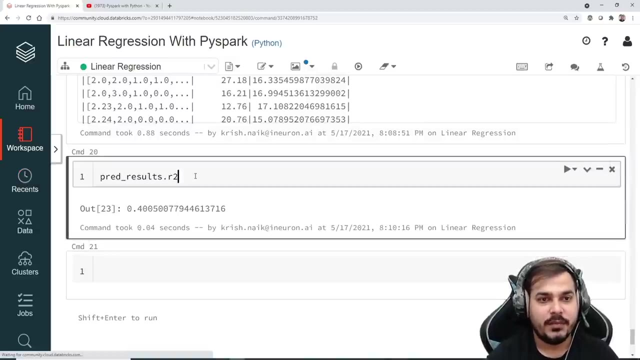 or not. just a second. i'm just checking out the documentation page. uh okay, oh sorry, i don't have to use regressor over here, so here i will be using prediction dot results and let me compute the r square, r square. so this is my r square. similarly, you can also check out prediction results, dot mean. 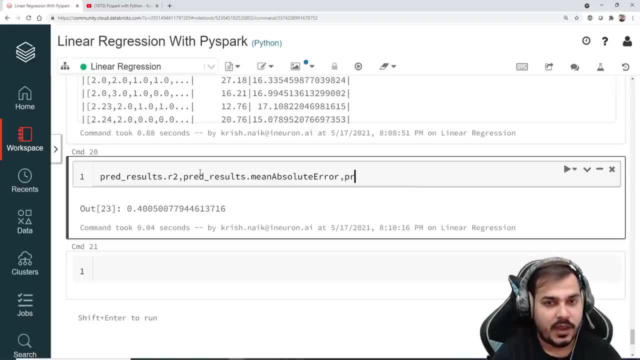 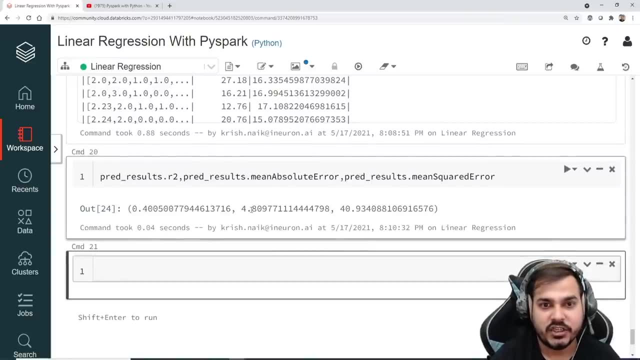 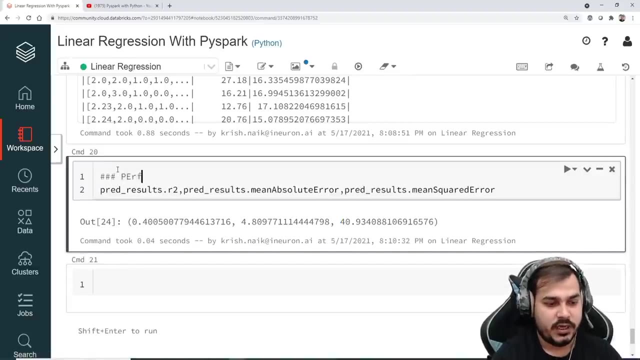 absolute error. so you have mean absolute error. you also have prediction underscore result dot- mean square error. so all these three values you can definitely check it out. so here is your mean absolute error, here is your mean squared error. so these are my performance metrics that i can definitely have a look and whenever you guys, whenever you face any kind of problem, just 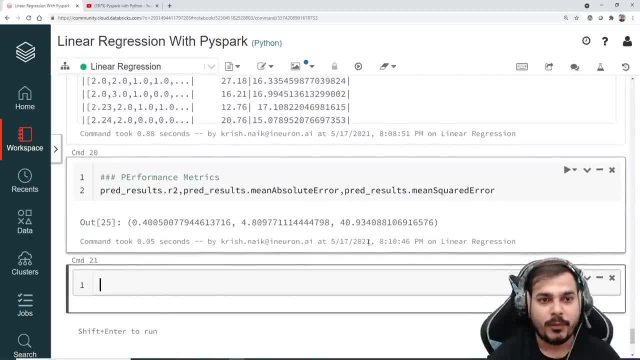 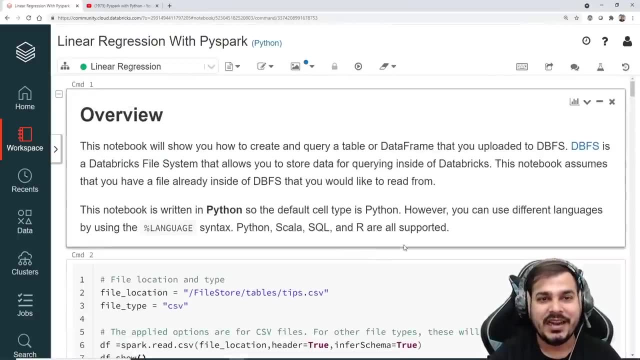 make sure that you check the documentation in apache, spark mlib documentation now. in this way you can definitely do this entire problem statement. now i'll give you one assignment: just try to google it and try to see how you can save this particular file, probably in a pickle format. 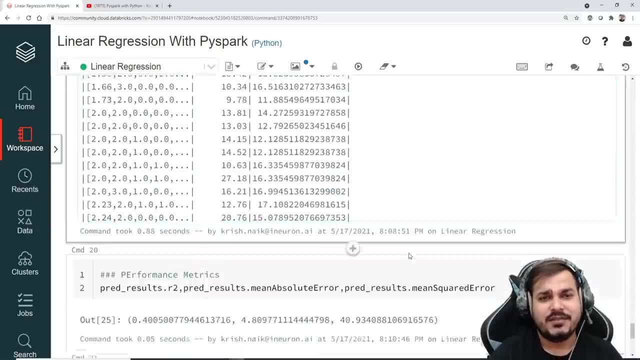 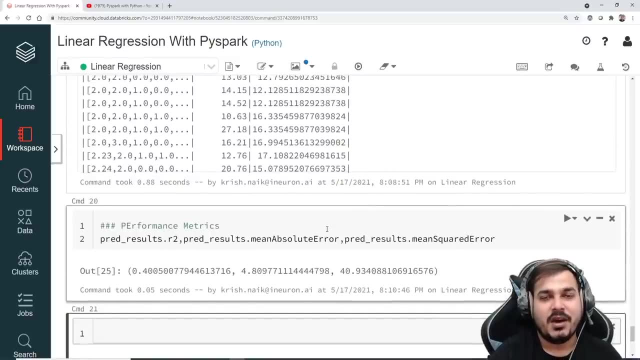 or probably in a temporary model pickle file. you know it's very, very simple: you just have to use the regressionsave. but try to have a look and try to see that how you can save this particular pickle file. now this was all about this particular video. i hope you like this. now just try to solve. 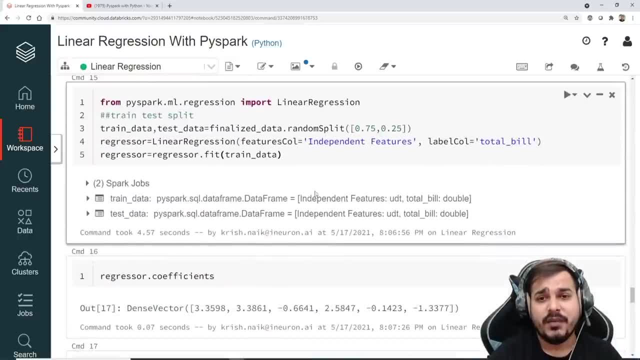 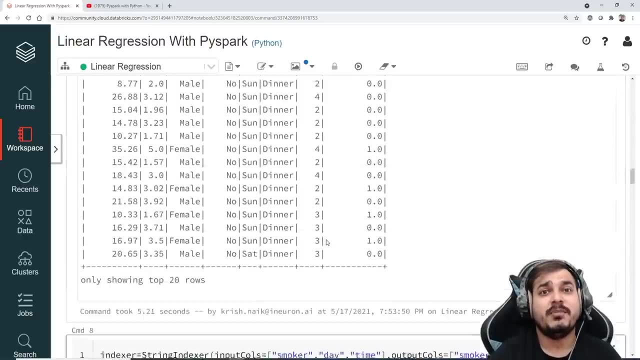 with any other problem state when try to do this. in the upcoming videos i'll also try to show how you can do one hot encoding, and probably you'll be able to learn that too. so i hope you like this particular video. please do subscribe the channel if you're not subscribed. see you in the next video. have a great day. thank you and all bye.